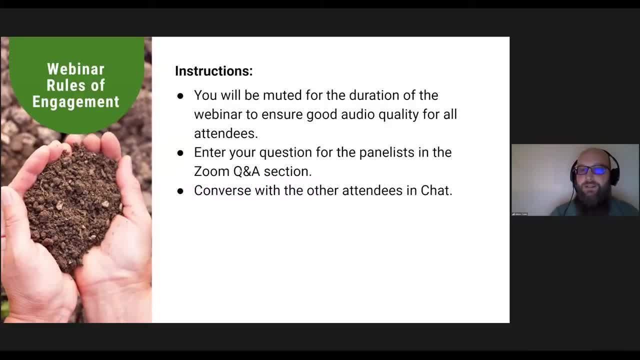 We do invite you to enter your questions for the panelists in the Q&A section of the Zoom links, And so we'll get a little bit more into exactly where that is in a couple of minutes- And I see that people are already filling in per our usual question that in chat you would tell us where you're joining from. 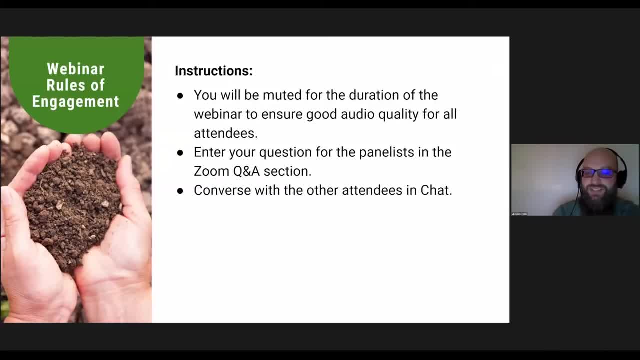 I'm seeing places like Brazil And Puget Sound and Switzerland's coming up, So this is exciting for us to have people joining from all over the world. Feel free to converse with other attendees in the chat And remember that you can ask your questions of the panelists directly in the Q&A section. 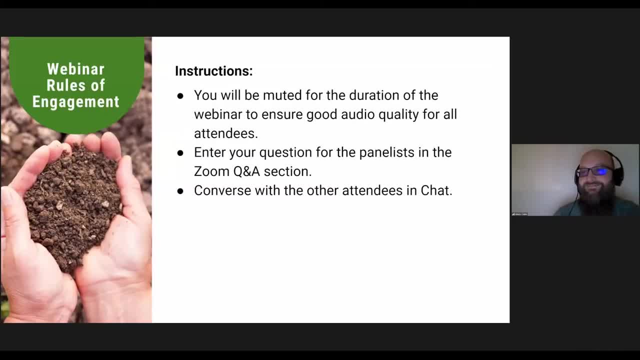 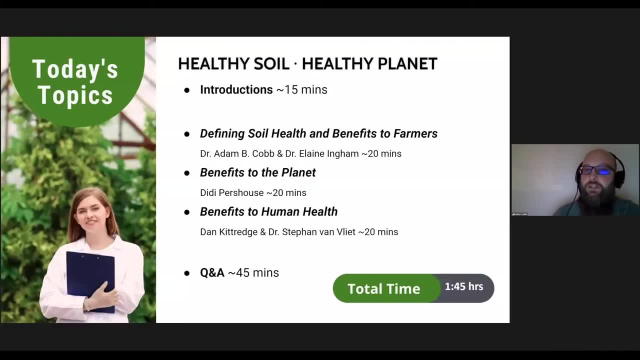 Looks like we've already got hundreds of participants. That's great. Can we go to the next slide, please, Brian? Again just to let you know how the rundown of today's webinar will work. We're going to make some introductions here for a few minutes. 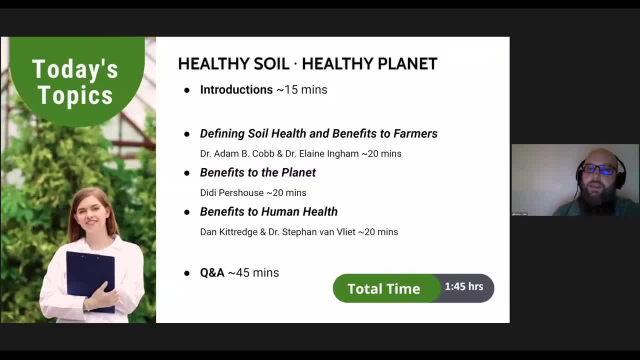 We'll get to all of our panelists today And then I'll give you some working definitions of soil health that Dr Ingham and I have chatted about, as well as defining some of the benefits to farmers if they'll restore their soil health and manage that properly. 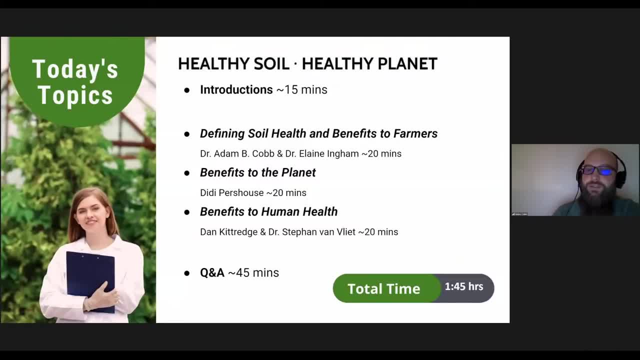 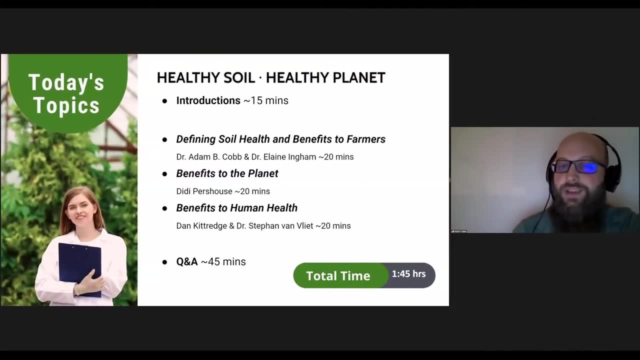 And then we have DeeDee here to give us some of the some information about benefits to the planet. So soil health can extend out to having a lot of environmental benefits and she'll cover those. And then we also have Dan and Steven here to talk about benefits to human health. 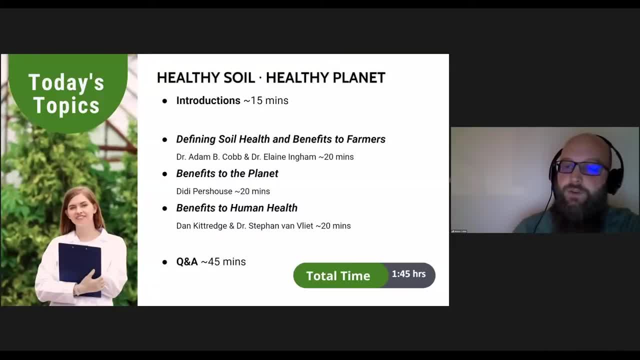 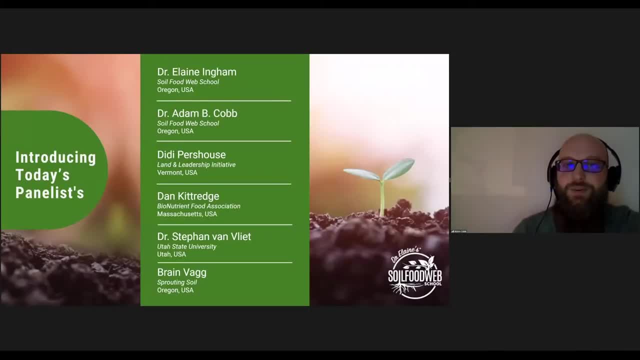 We'll follow that with a Q&A session for 45 minutes, so a total time of just under two hours today. Let's go to the next slide, please. All right, So we're going to go around the horn here and let the panelists introduce themselves, starting with Dr Elaine Ingham. 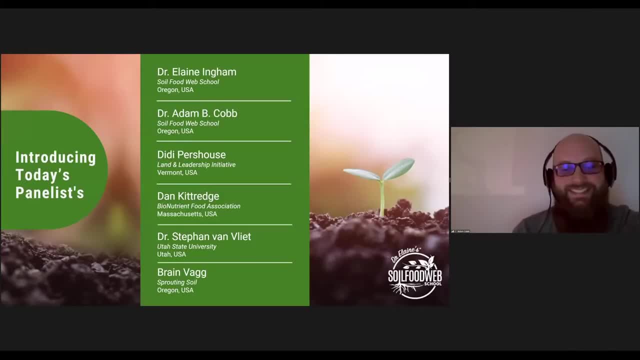 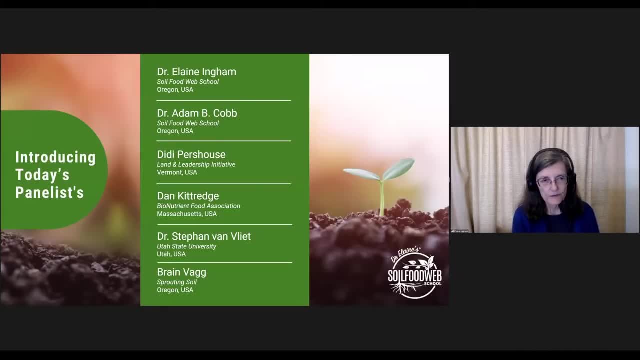 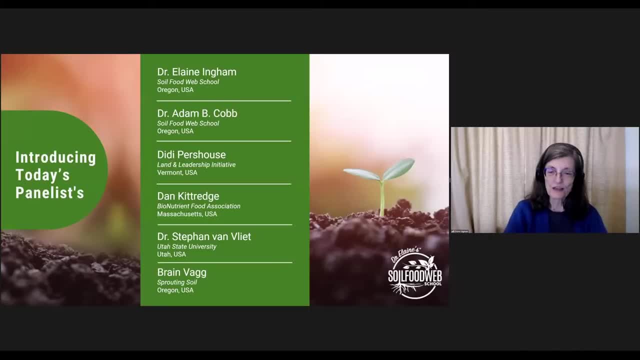 This is what happens when you get to be 80 years old – or 70 years old, Jeez, can't even get the numbers right. So publications in the scientific literature: you know we've done a lot of work and much of it's been published. 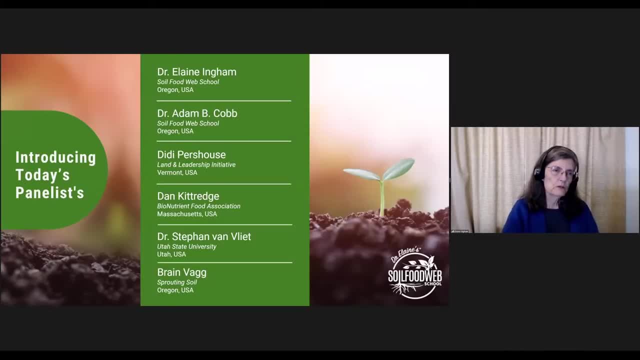 But here at the school we're continuing to do research And we will be writing that data into the manuals and into the information that people learn when they come to get the education here in the foundation courses: learning how to use a microscope becoming a laboratory, that you do samples for other people. 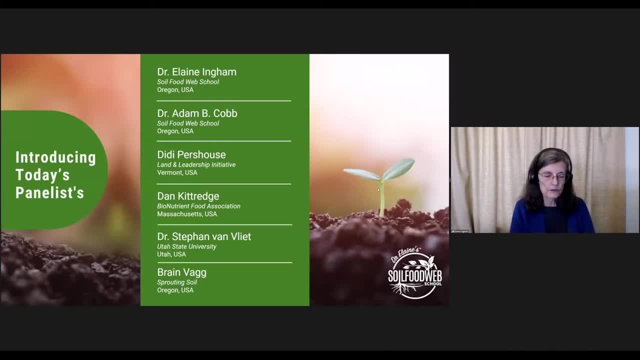 or you become a consultant where you're doing interpretations of what that biology – is or should be for maximum health in your – in your school – in your – in your fields. Thanks so much, Elaine. I'm Dr Adam Cobb. Again. I'll be sort of running the MC portion of today or being the host of the webinar. 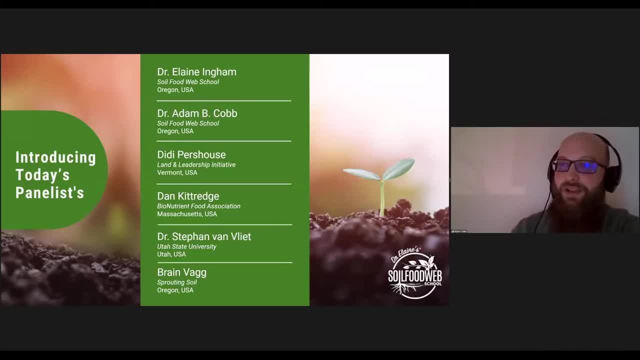 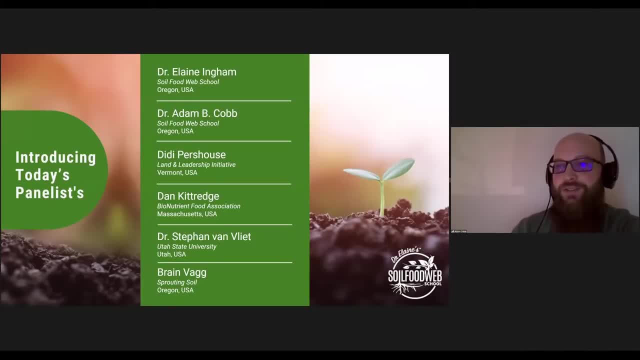 and I do a lot of work in the background as a content creator And also some of the work in the foreground as a science communicator here at the school. So that's just a little bit about me, And then we'll have Didi, who's with the Land and Leadership Initiative, explain a little bit more of her background. 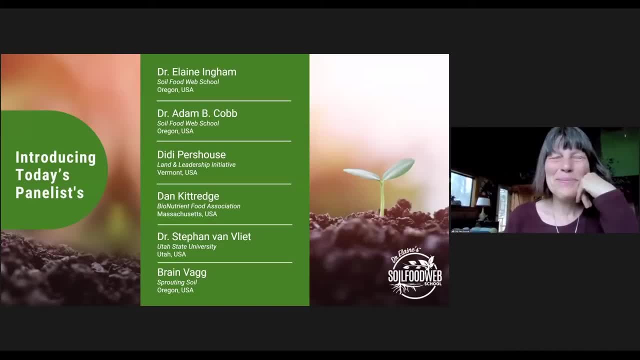 And Didi, you're muted as well. Okay, I am the author of two books. One is called The Ecology of Care, Medicine, Agriculture, Money and the Quiet Power of Human and Humanity. One is called The Ecology of Care, Medicine, Agriculture, Money and the Quiet Power of Human and Humanity. 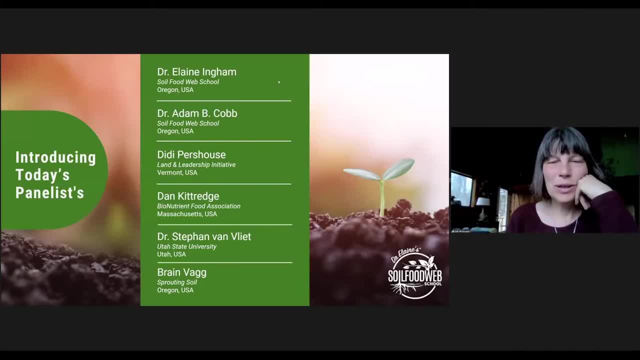 And the second book is called Understanding Soil Health and Watershed Function And that is a free download at landandleadershiporg. And I teach a lot online, including through the Soul Food Web School And, one of the most exciting things, in which we have really deep discussions and design for regenerative projects. 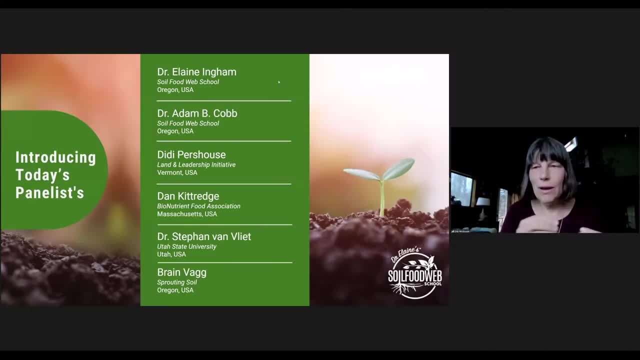 not so much the, Not so much the nuts and bolts of how to make healthy soil- That's Elaine's job- But more thinking about the entire system, thinking about the economic system, the education system, social systems and how we need to work with those to get everything going in the right direction. 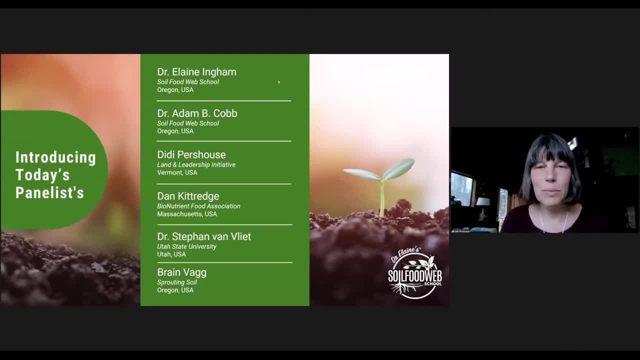 The other project is the Under Pradesh Community Managed Natural Farming Initiative in India that is engaging close to 800,000 farmers in one state in regenerating health And I'll show a little mini video if we have time about that at the end. 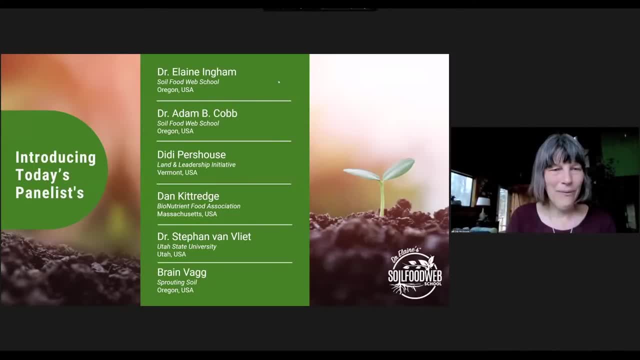 Over to you, Dan. Hi, Glad to be here. My name is Dan Kittredge. I'm the founder and executive director of the Bioinitiate Food Association. We're about a little more than 10 years old now- Nonprofit. 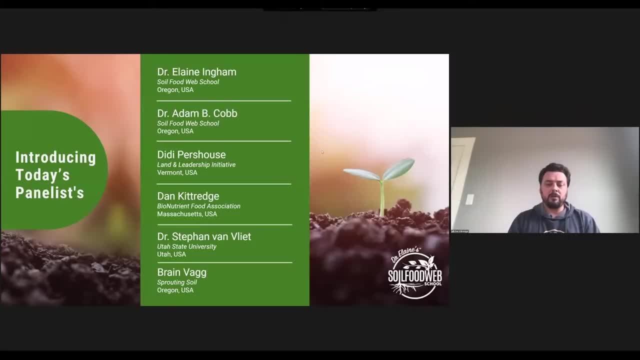 I'm focusing on increasing quality in the food supply, And by quality I mean flavor, aroma, nutritive value, health-giving attribute which we are fairly certain connects to soil health And plant health and human health and farm viability and all kinds of cultural health. 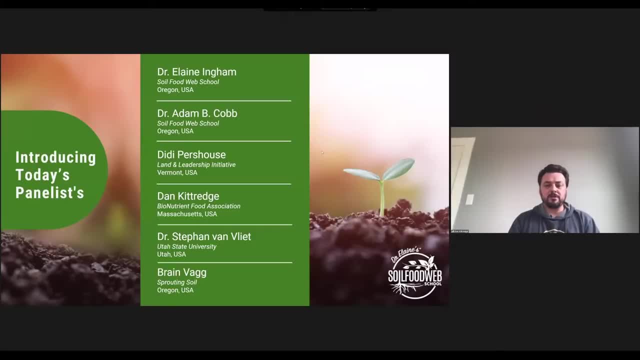 We've been working for the past five years on a research project to sort of define those nutrient variations in food, to connect them through a really broad and thoughtful open source data framework to management practices in soil health And as well, to build a you know instrumentation so people can assess that nutrient variation. 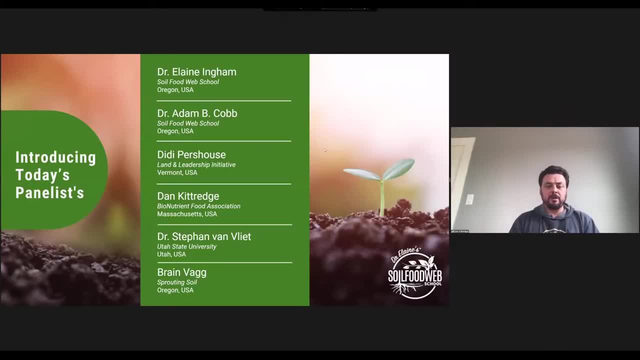 We think that there's a strong connection, Like I said, between nutritional value of food and soil, health and environmental health and human health, And so we think that's a spot where a lot of people can engage who aren't necessarily growing themselves. So I'll be talking a little bit about our work here today. 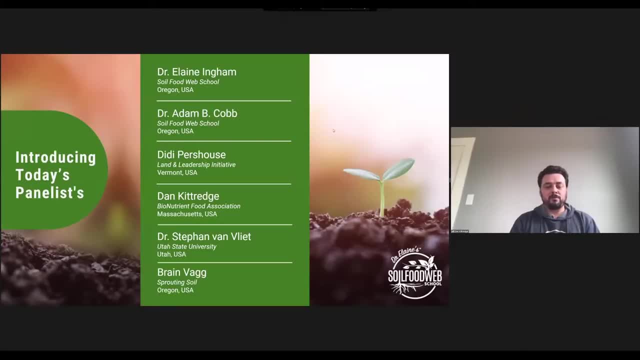 And very excited to introduce Stefan, our partner in our beef project, for that work to this community. It can really be impressive what he's doing. I always Speaking of that. Oh sorry, Yeah, I was just about to say. 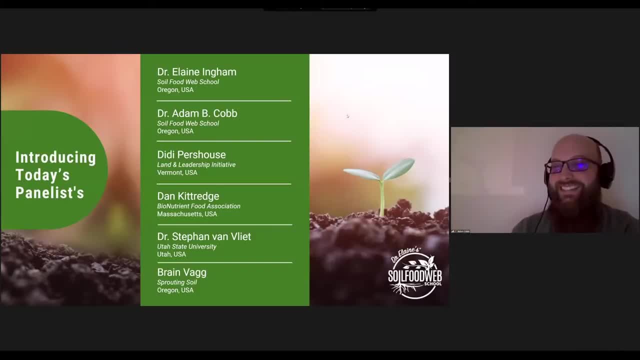 And speaking of that, Stefan, we'd like you to introduce yourself, please. Great. Yes, Hi all My name is Dr Stefan Van Vliet. I'm a nutrition scientist with the metabolomics expertise in the Center for Human Nutrition Studies at the Utah State University. 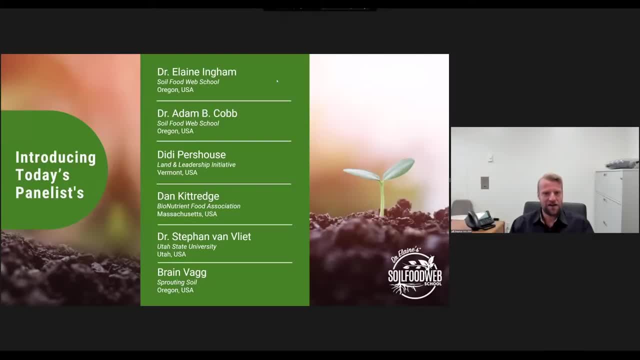 I earned my PhD in kinesiology and community health as an Aspen Fellow and received training at the Washington University School of Medicine and the Duke University School of Medicine. I'm particularly interested in linking agricultural production and soil health, Plant animal health, to human health. 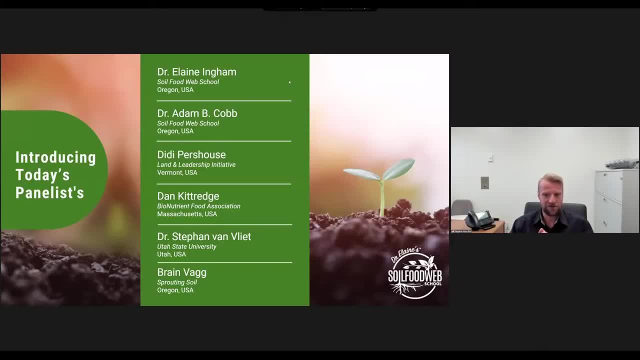 So a lot of our work is performed at the nexus of agriculture and human health, collaborating with farmers, ecologists, agricultural scientists to study these critical linkages between the nutrient density of our food production and human health. And that is, in a nutshell, what I'll do and will present on our beef nutrient density project with Dan Kittredge and the Bionutrient Institute. 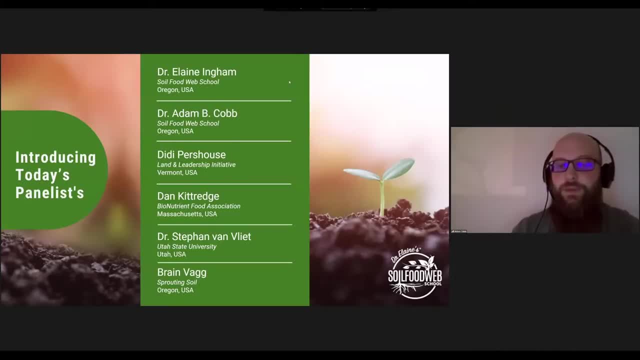 Thank you so much. And last but not least, we have Brian Vag here, who's one of our consultants at the Soil Food Web School. And, Brian, would you give the audience a little information about yourself? Sure, I'm Brian Vag. 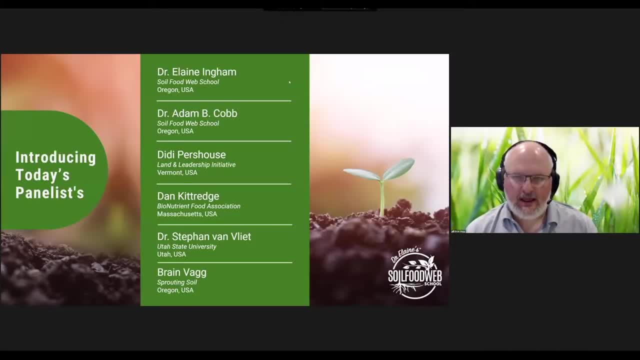 I own a company called Sprouting Soil, based out of Oregon And, as Adam mentioned, I am a Soil Food Web consultant and also a mentor for the Soil Food Web School And really you know my role is to help transition- predominantly agriculture, but other growing systems like landscaping and golf courses and parks and things like that. 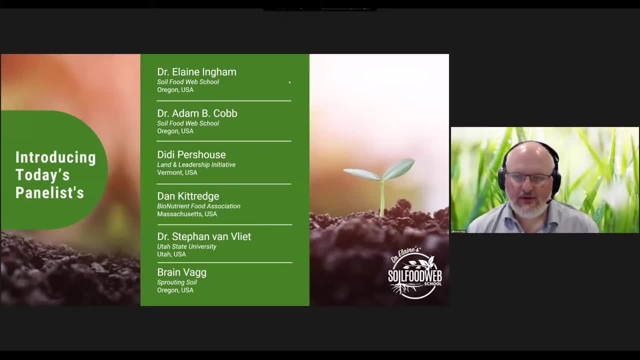 But helping those folks in those growing systems transition from either conventional, conventional organic into growing with biology- And it's definitely, I'd say, in the last two years at least- is really accelerated. There's a lot of challenges that farmers are facing and we have a lot of answers for them. 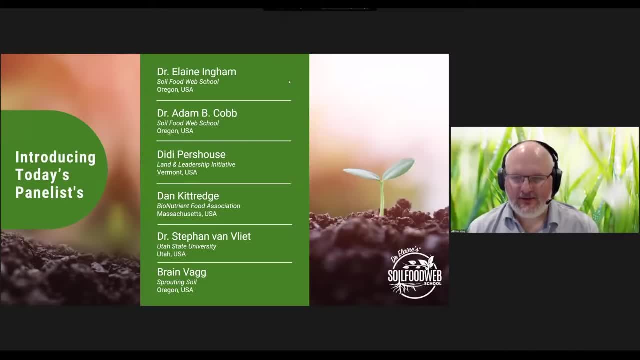 So it's a good time to be in the soil biology consulting business, that's for sure. That sounds great. Now, if we could go to the next slide here, We're going to do a quick poll which will pop up for all of our participants. 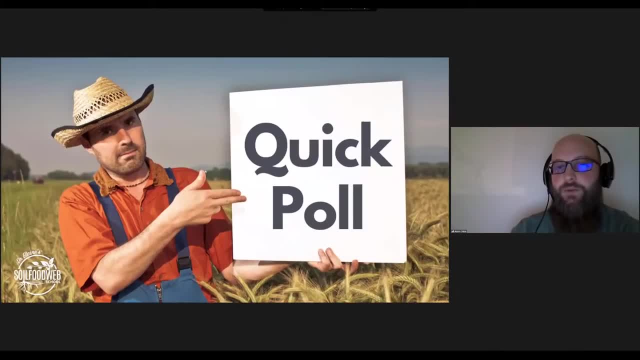 Yes, we're just going to ask that you let us know if you're visiting us here today as a farmer, grower or ag professional, as an environmental advocate, or if you consider yourself both the above or neither of the above. So we already see that there are some answers coming in. 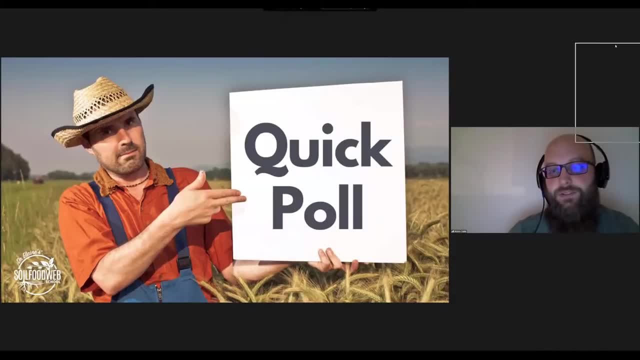 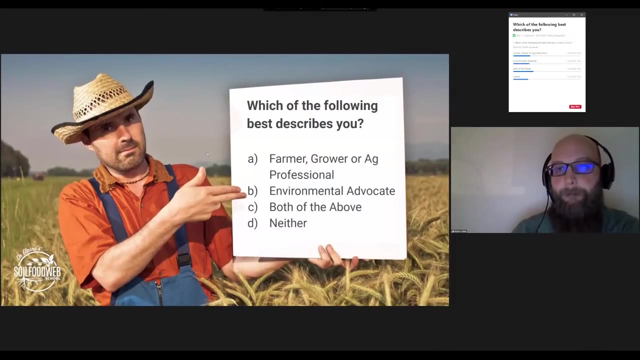 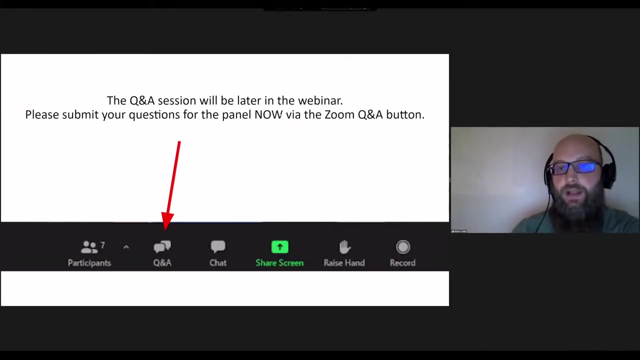 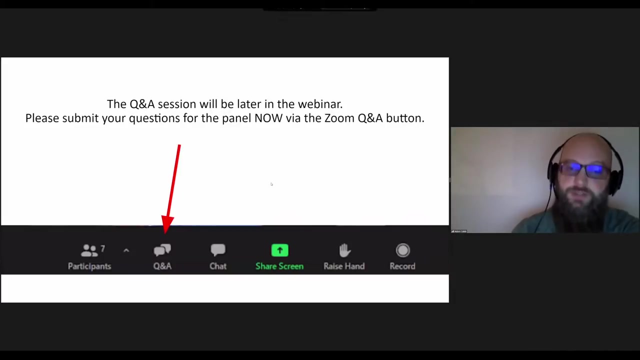 Looks like we have a fair mix of folks. You can take us to the next slide as well, please, Brian. All right, And then this is just one more reminder that we're asking you to add your questions to the Q&A tab so that in our Q&A session at the end, 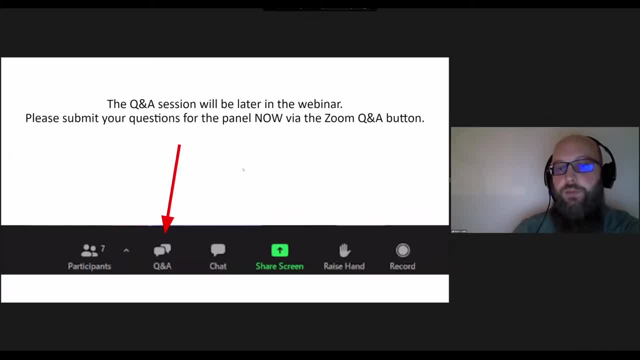 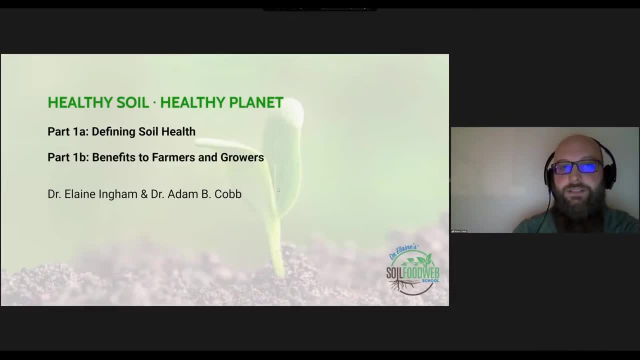 after we've done the presentations, we'll be able to pull those over and answer your questions for you. All right, let's get started. As I mentioned, the first part of the webinar today is going to really be about defining soil health. 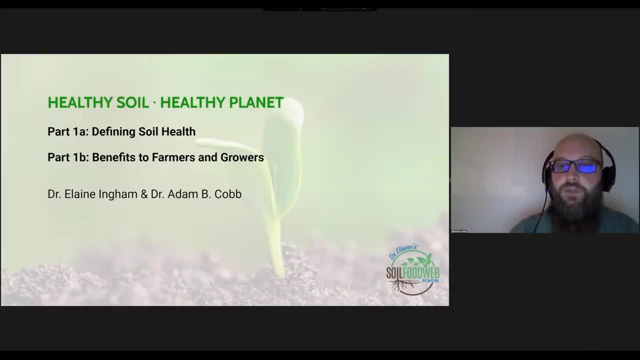 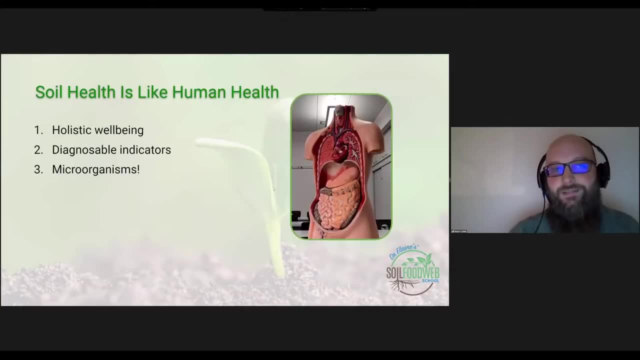 as well as explaining some of the benefits to farmers and growers, And that's going to be a bit of a team effort between Dr Elaine and myself. So, as I was asked to come join the webinar today by the team, I really took some time to survey the literature and ask a lot of my friends who are working across academia and governments what they define soil health as. 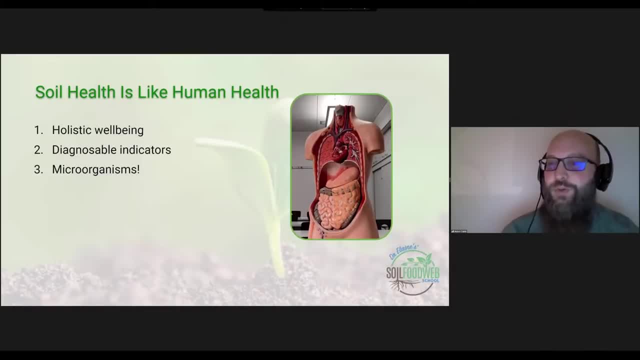 And in my opinion there's not one true, great, perfect definition for soil health out there. Most often we see something to the effect of the ability of soil to act as a living ecosystem and supply the nutrient needs of plants and animals and humans. 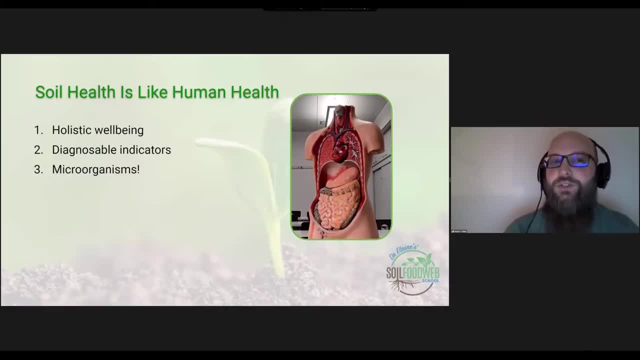 So I actually wanted to go a little bit more into a metaphor today and set the stage for our discussion. So I like to think of the human body and human health, which is something that we're all intimately familiar with, and the ways in which soil health is like human health. 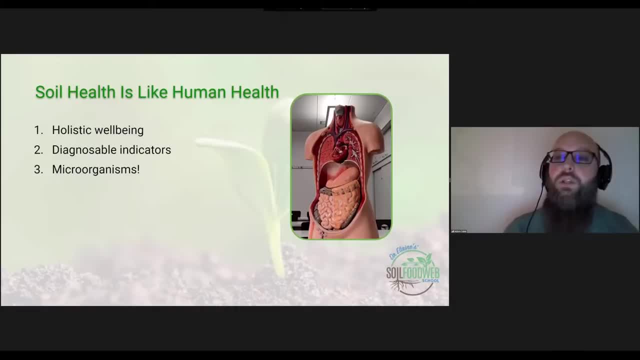 The first way is we're really holistic beings, Even though you can look at the human body and consider different organs and different functions within the human body, it's a whole well-being, not just somebody hanging on by a thread as technically alive but truly thriving. 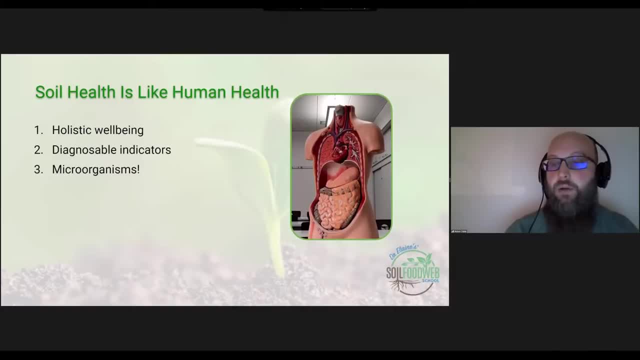 is about a whole Holistic connection and health across the entire human body. Now with point two, here, just like with the human body, soil has these different diagnosable indicators. So if you go to the doctor, they're going to check your blood pressure, your pulse. 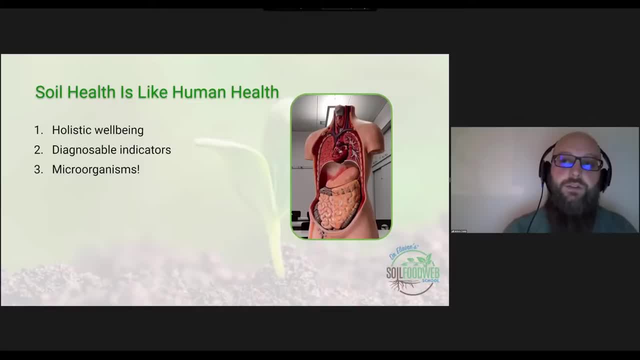 your breathing. Those are indicators of health And we can start to see now if something's not quite aligning with the normal range. that tells your doctor that they need to do something about it. They need to do some diagnosing to dig down and find the root of the problem. But we all know. 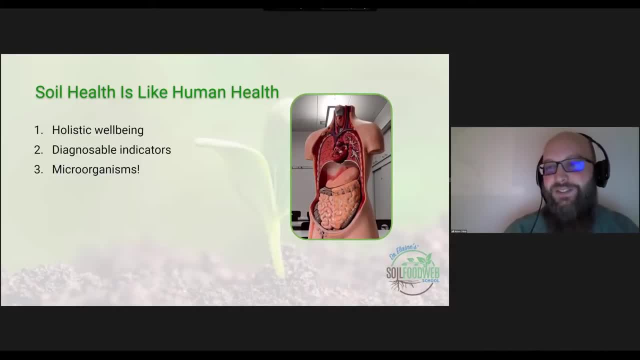 that modern medicine can sometimes just mask the symptoms of what people are facing when they're unwell. And in the same way, we'll talk about how many of the agricultural practices that are used in industry are just masking symptoms that are happening when the soil system is not fully. 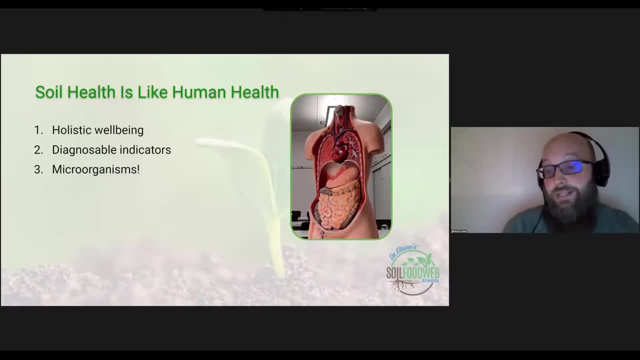 healthy, And so the final point I'd like to make is about the role of the human body in the microorganisms, because this is similar between soil health and human health as well, that we're finding more every day. There's more literature being published about how important the human 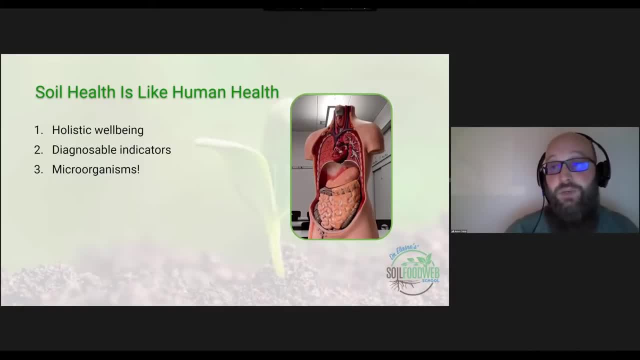 microbiome is to our health. I actually was reading a paper recently that tracked populations- aging populations- and found that there was a connection between the microorganisms in their gut and their sense of loneliness right. So if you look at the microbiome you can see that there's a connection between the microorganisms. 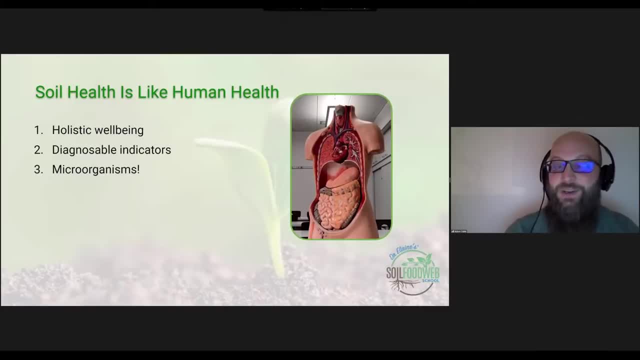 and that we can tell if you need a boost to your, to your mental well being. your microorganisms may play a role in that And really microorganisms are- are the key to soil health, if we're. we'll go into this in a little more detail as we, as we move along. 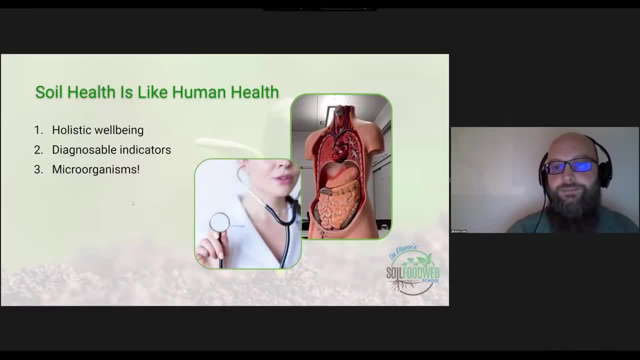 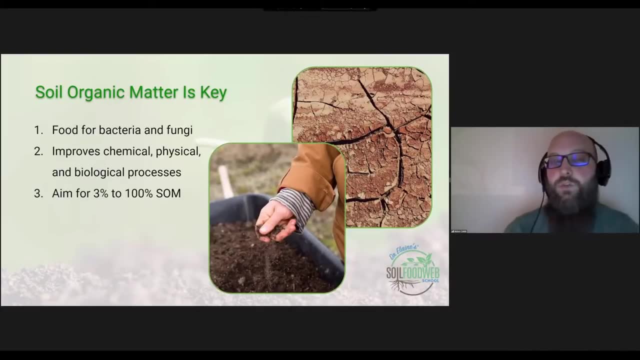 If you could take us to the next slide there, Brian, please. So one of the key indicators that we do want to make sure to talk about is soil, organic matter, And I mean as a scientist- I'm not supposed to use the word magic, but if there's a magical, 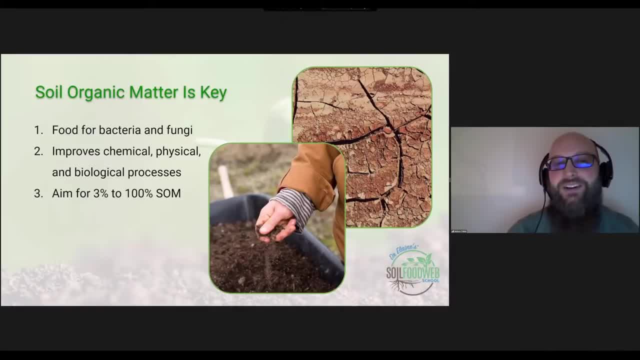 component of soil. to me, it's the soil, organic matter, And that's partially because it serves as a food source for bacteria and fungi, and bacteria and fungi consuming organic matter as well as minerals in the soil and taking them into their bodies is one of the basic functions. 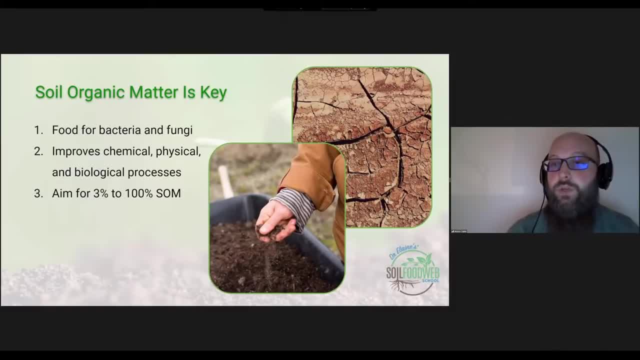 of the soil food web. Of course, those nutrients are released as the bacteria and fungi are consumed by organisms across the soil food web, So it's an important food source for the base of the food web. Soil organic matter also can play a very direct role in improving chemical 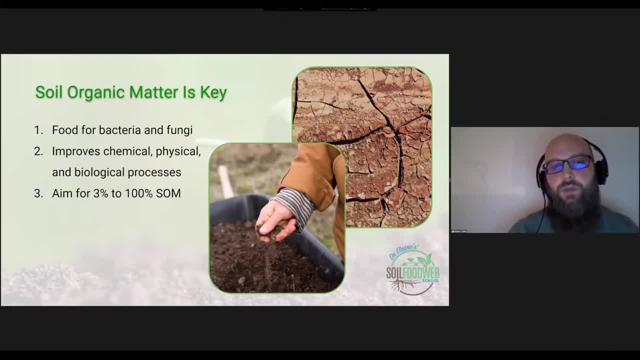 physical and other biological processes in the soil. So let me give you an example here of chemical. Greater organic matter content in the soil tends to keep the pH of the soil more stable. That's a very basic chemical indicator that's almost always tested by soil testing labs. 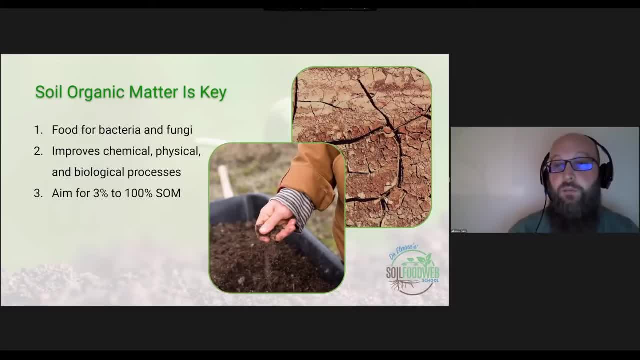 And we see- you know sometimes we use the word a buffer- that a lot of soil organic matter can keep that pH from moving too high or too low right. So that's a very basic chemical indicator that's almost always tested by soil testing labs. 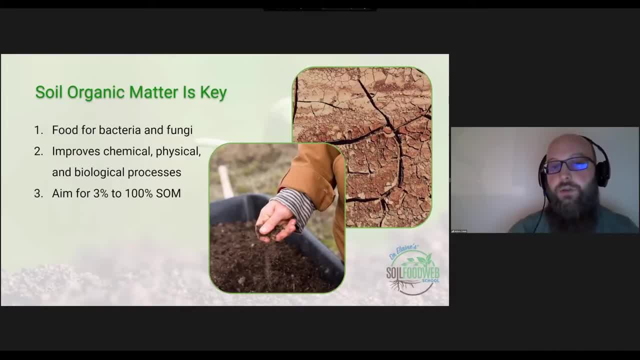 Additionally, there are physical characteristics of the soil, such as- for lack of a better word- the fluffiness of the soil, the tilth- You can pick it up with your hands and you can get scoops of it with your hands. and more organic matter tends to create better physical 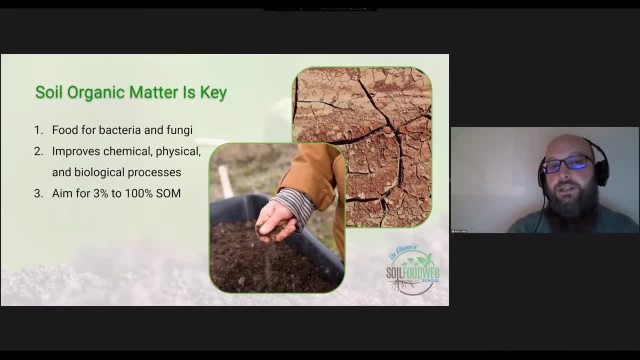 characteristics in the soil like that And then, in addition to the food source for bacteria and fungi, that would be a part of the biological process of the soil. So that's a very basic chemical indicator that we can use from soil testing labs. So there's different ways we can use organic matter to create pigments. 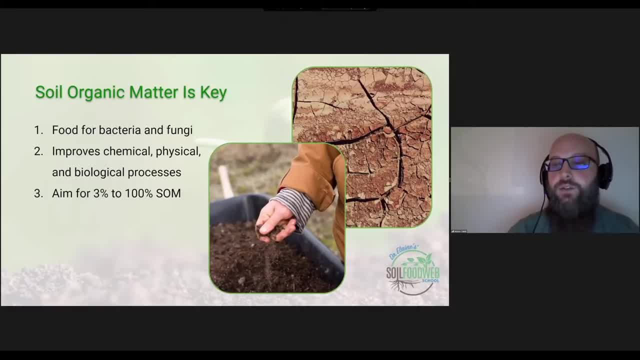 Other organizations also. there's this again. I don't want to talk about the word or it's just one way, but this is the way we can use organic matter to create pigments. We would call it agravim. This would be the way we would use organic matter to create pigments. So we would say, for the sake of this video today, let me just E E, E, E E. So organic matter is a tributary of chemical substances and soil. Soil, organic matter tends to improve things like the infiltration of water and air into the soil. 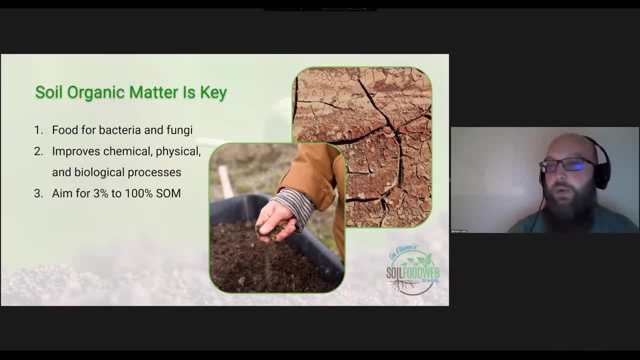 system and tends to provide little habitats for different organisms to connect with. so they will see hunting organisms that are predators actually hunting in soil. aggregates near organic chunks of organic matter in the soil, And so it has a wide range of positive effects on biological processes in the soil. 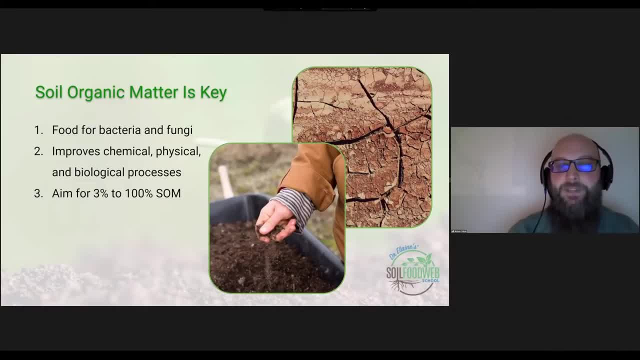 Dr Elaine and I talked about this just the other day in our foundation courses. She mentions that you really want at least 3% soil organic matter just to serve that basic function of food for your microorganisms. But really you could go up to 100% soil organic matter. 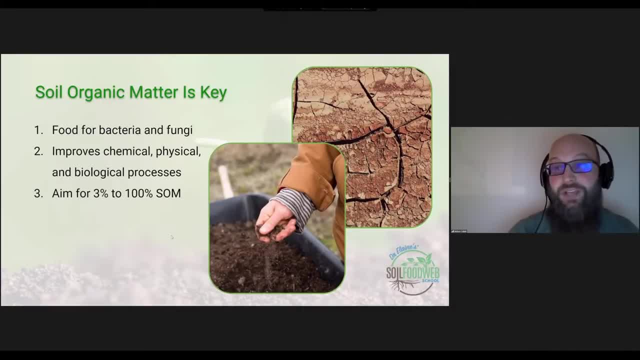 Plants grow very well And you know, if you could have a deep garden bed that went two meters deep and it was just full of compost, your plants could theoretically grow very well, in that if the compost was biocomplete and the organisms and other components were there, 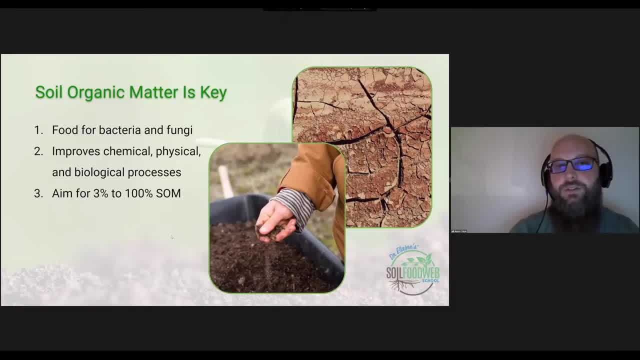 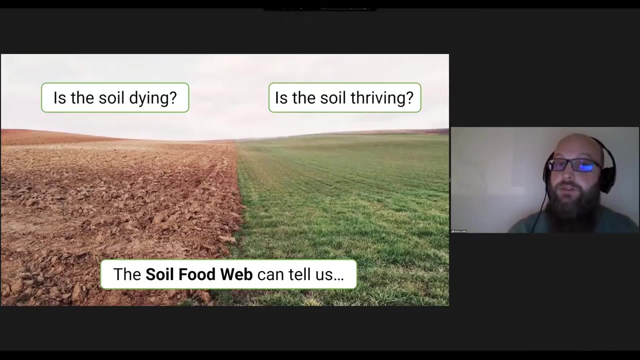 So soil organic matter is just one of the key indicators. It's like a heartbeat or a blood pressure reading for the soil. You can take us to the next slide please. So I'm going to ask Dr Elaine to speak on this in just a moment. 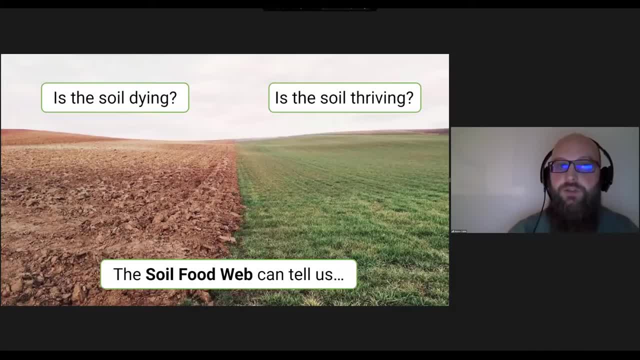 But I wanted to ask this question so that we can all think through. if you were actually to ask yourself the question from looking out at a field that you pass in your car And you said: is that soil dying or thriving? Is that soil degrading or is it improving the soil health over time? 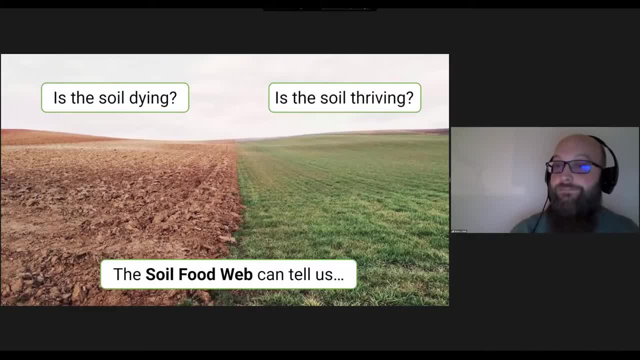 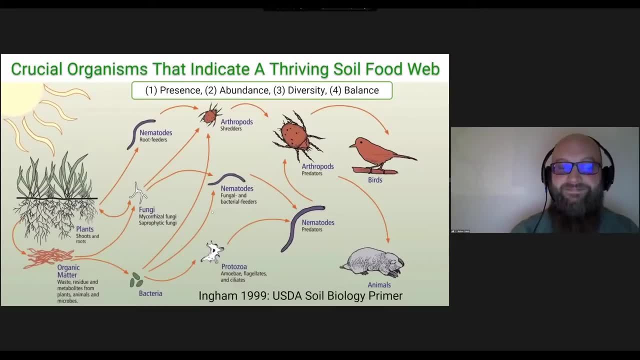 It's really the soil food web that's going to give us the answer. So we'll go to the next slide and have Dr Elaine explain a little bit about the soil food web. Unmute myself, All right. So when we look at the soil food web, this is the web that we talk about all the time and the position of different organisms in this food web. 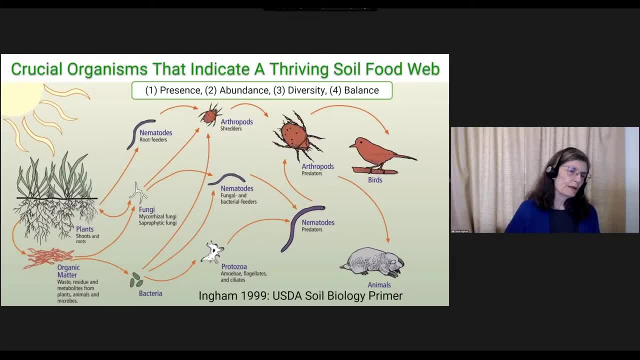 It's a web because It's not a single straight line through. We always think of above ground, as it's. you know, bunny rabbits are eaten by, foxes are eaten by, you know, whatever the next bigger predator? And that's the food web. 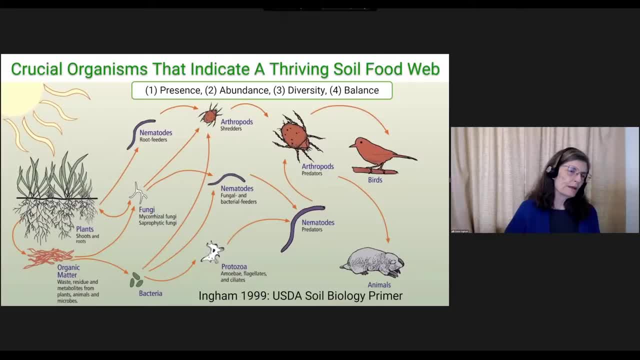 Well, yeah, the straight chain, the food chain, is where you only have one group of organisms occupying each stage in that successional system Or food chain. When, in fact, when we look at soil and above ground, it's a web that we should be talking about. 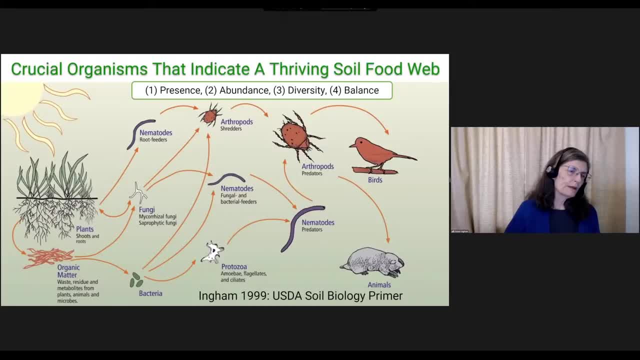 So you know, sunlight energy has to be fixed and that process occurs through photosynthesis, Just as Adam said, we don't tend to like to use that term magical when we're scientists, But if you want, If you want to talk about a magical occurrence going on all the time, it's the process of taking sunlight energy and being able to store it through the process of photosynthesis. 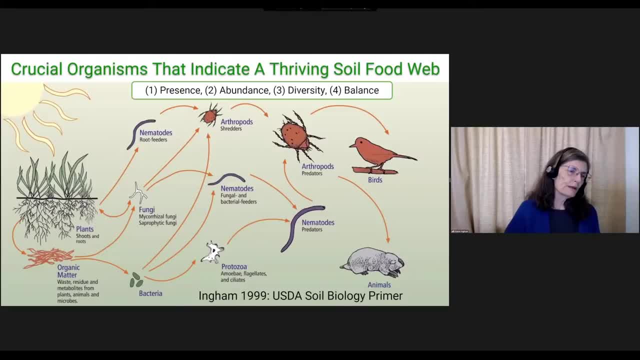 So fixing carbon, taking a carbon dioxide molecule from the atmosphere and removing the hydrogens and the air oxygen And getting the carbon chain started. It's that connection between the first carbon chain and the second one and the third one, The fourth carbon dioxide, the fifth carbon dioxide. 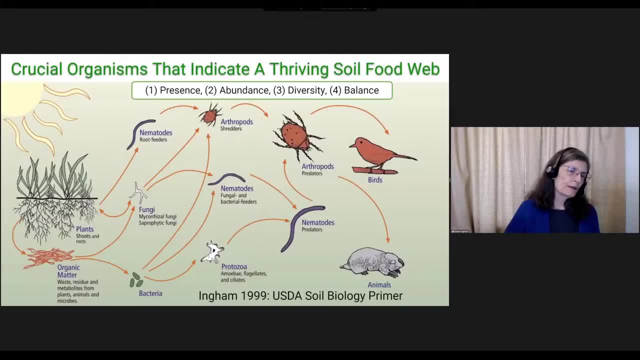 Pulling, holding that energy in that bond, And now we have energy that can be used through the whole rest of this food web. Well, you know, think about your plant. It's now got the energy that it needs to run everything. 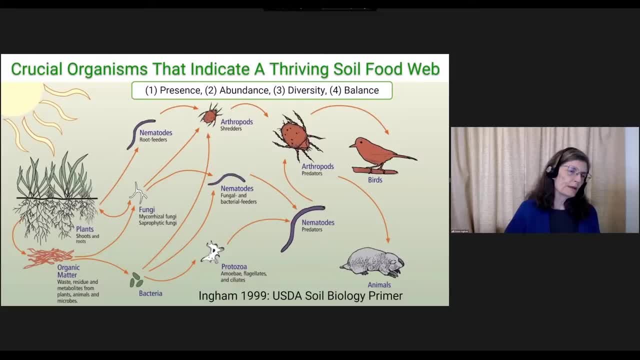 But in order to To stay alive, you have to be able to pull all the other nutrients into your body, And the cells of grasses are not that different from cells of fungi or cells of micro arthropods or cells of human beings. 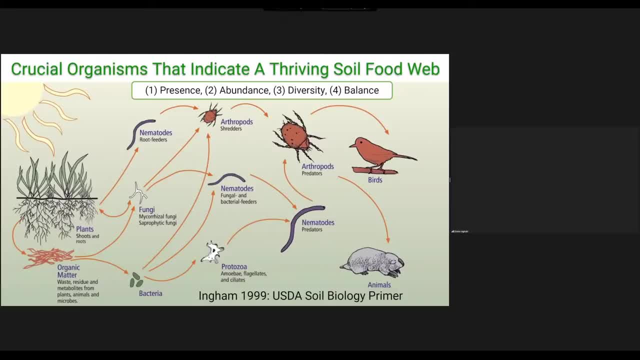 We all require more or less the same amounts of nutrients, And where is your plant going to get that? And I always have to know the mechanism. It doesn't work. you know, I'm just going to: I put my plant in the soil and it's going to magically start growing. 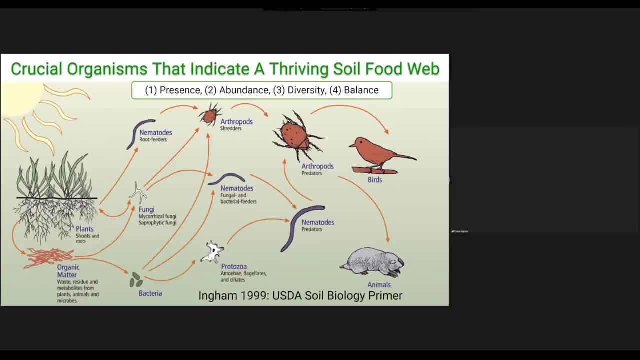 Well, why do some plants not grow? You have to understand the mechanisms going on in your soil. If you can't figure out the mechanisms by which the plants are getting the nutrients, or getting protection, or holding water in the soil, fixing compaction problems, 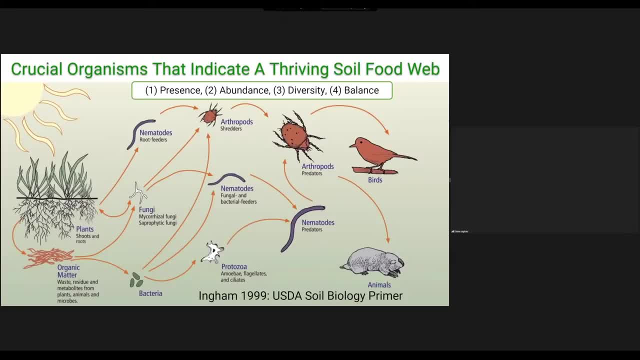 If you can't, If you can't figure out how to do that work, who is it in here that does all of the particular jobs? you're not going to be successful. You have to know what you're doing. You have to know what these organisms are present in order to do the jobs they're supposed to perform. 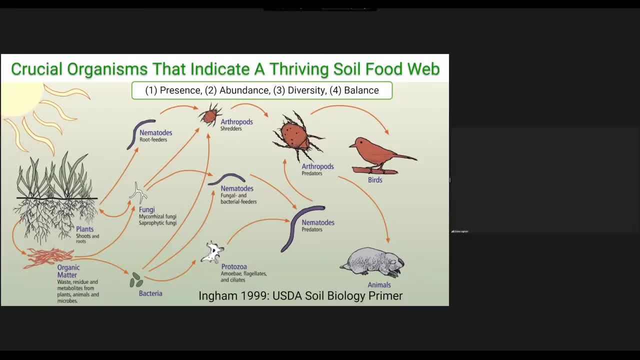 And so that's kind of been my career is putting all of this together. So energy from the above ground part of the plant, But the plant has to get nitrogen and phosphorus and sulfur and magnesium and calcium and sodium and potassium and iron and zinc and, oh yeah, some water and some oxygen. 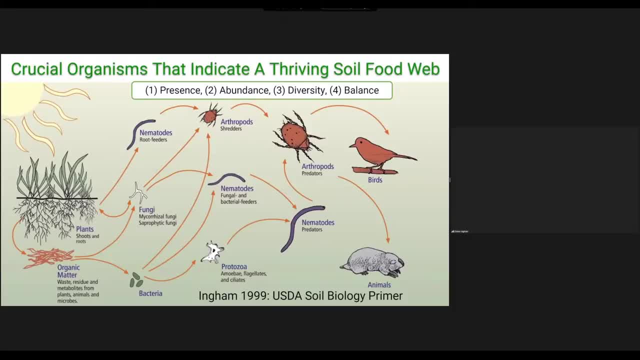 And so your plant is putting that root system down into the soil in order to get those nutrients. But those nutrients are tied up in plant not available forms, in the sand, the silt, the clay- If you look at rocks, pebbles, parent material. 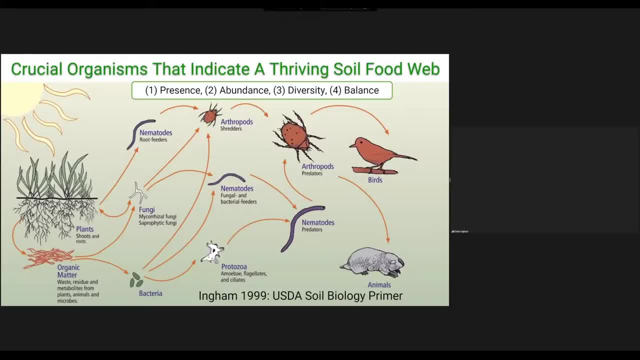 Material boulders, things like that. those are all the precursors to sand, silt and clay. Well, how do you break down the big boulders, the pebbles, the rocks? How do you break that down into something that a bacterium or a fungus could approach and pull the nutrients out of the silica bilayer in the sand, silt and clay? 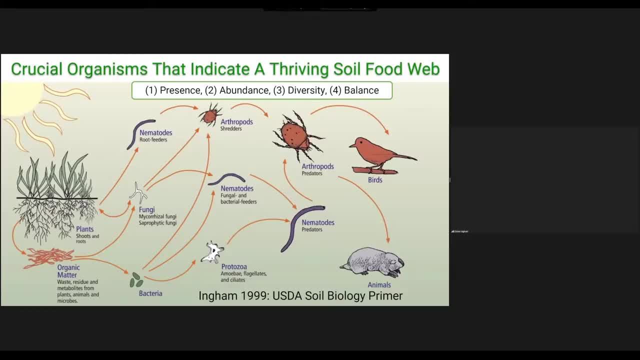 How do you convert parent material into sand, silt and clay? Well, most people would say, oh, it's weathering, It's freeze-thaw, wet-dry cycles, And those are insignificant amounts of breakdown of the rocks, of the boulders, into something, into sand, silt and clay. 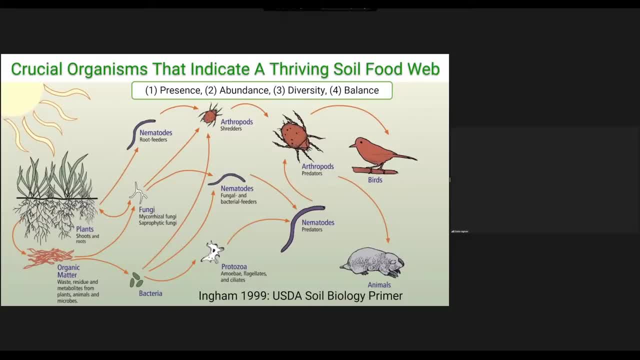 Because what does the greatest amount of breakdown of those inorganic nutrients not available nutrients are the bacteria and the fungi. So right away we're looking at bacteria. I hope you can all see my pointer. The fungi are right above it, in that second trophic level, if you will. 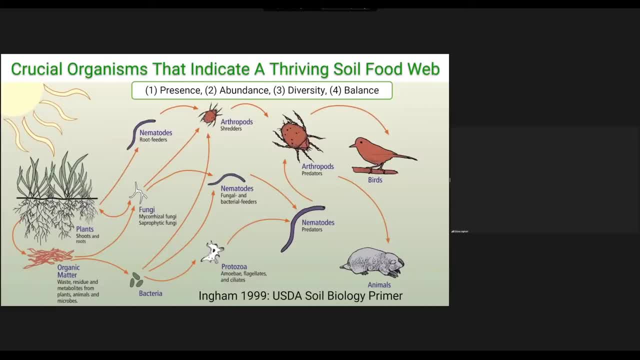 So the plant is actually putting out sugars, proteins and carbohydrates- high-carbon-containing materials- and using that as food to get the bacteria and fungi growing. The plant will actually put out a specific exudate when it needs calcium, or when it needs potassium, or when it needs. 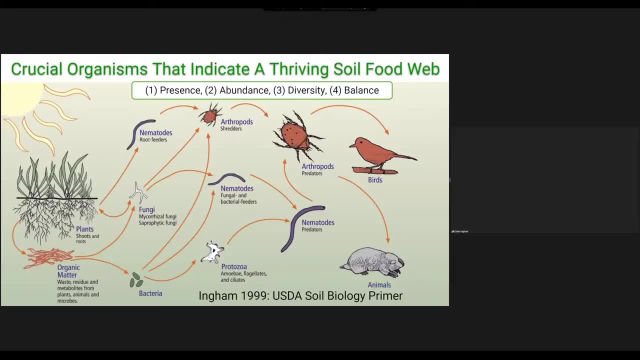 It's a message to the bacteria and the fungi here that those bacteria and fungi better start growing. Here's some food to get you growing. But make the enzymes to pull those nutrients that the plant requires from a plant-unavailable source, Such as in soil, organic matter. 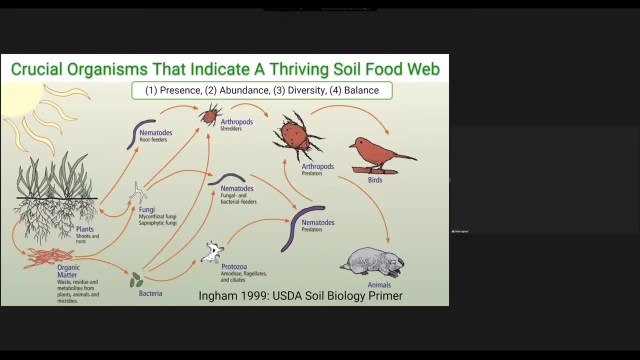 Most of the nutrients in soil, organic matter, are not available to your plant. Your plant can't take them up. Sand, silt and clay Plant can't take up those nutrients. You've got to have the fungi and the bacteria doing the next step of using their enzymes to pull those nutrients from the organic matter. 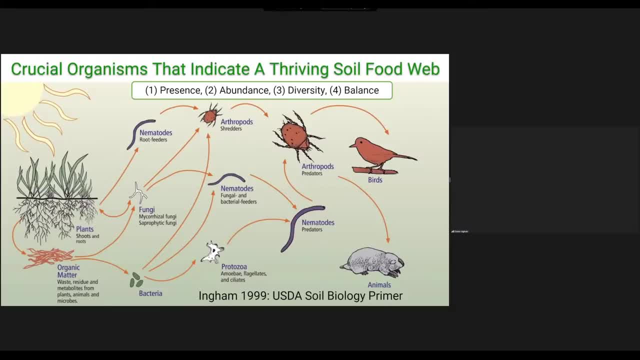 Pulling that out and storing Those nutrients in the bacteria and fungi? And where do most of the bacteria and fungi grow? In your soil? Well, right around the source of their food, Right in the root system of your plants. Yep. 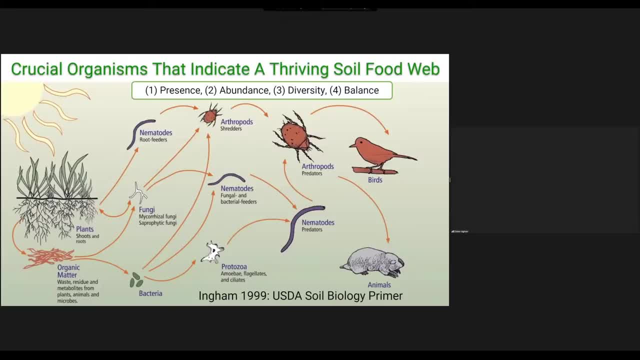 These organisms will also be carried above ground to protect the above-ground parts of your plants, And so there's another whole set of information that we have to know and understand. So bacteria and fungi are holding these nutrients in their bodies, but they're in plant. 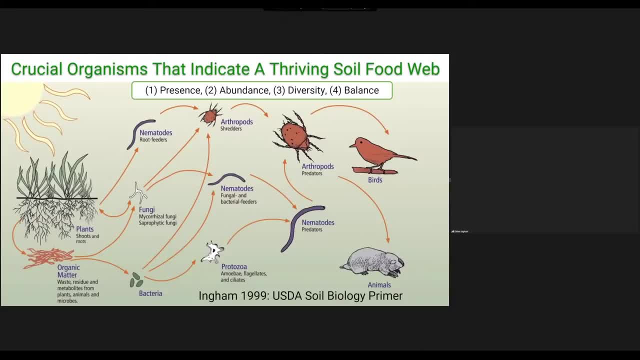 Not available forms. They're organic matter, but they're not available to the plant. So the next step has to happen. The bacteria have to be eaten by the protozoa or by bacterial feeding nematodes. The fungi have to be eaten by micro arthropods or fungal feeding nematodes. 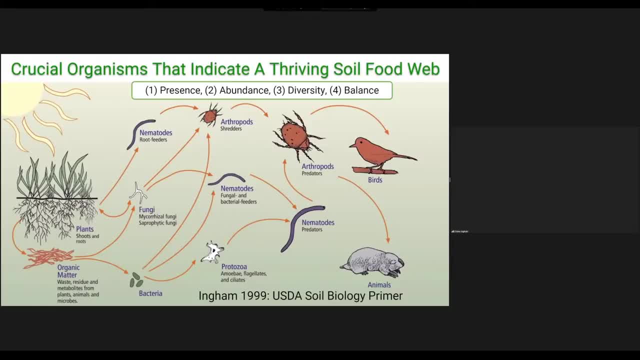 So that, when these organisms consume their prey, The concentration of nutrients Inside the fungi or inside the bacteria is so much greater, So much more than their predators require, That these predators are going to either spit out or poop. Here we go, Here's the poop loop. 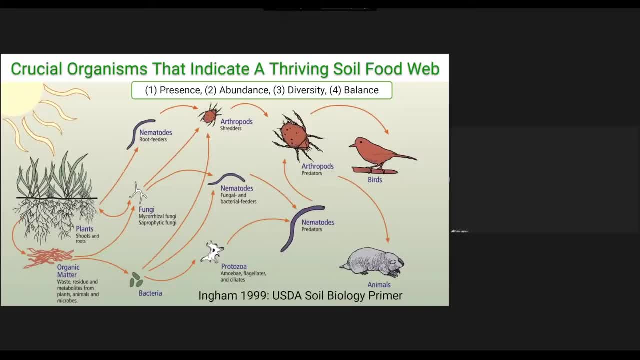 The poop that they produce is exactly the form of nutrient that your plant can take up, And so, As the bacteria and fungi are eaten by their predators, The nutrients for your plants are released right there, next to the root system. No need for diffusion to be pulling things from feet away. 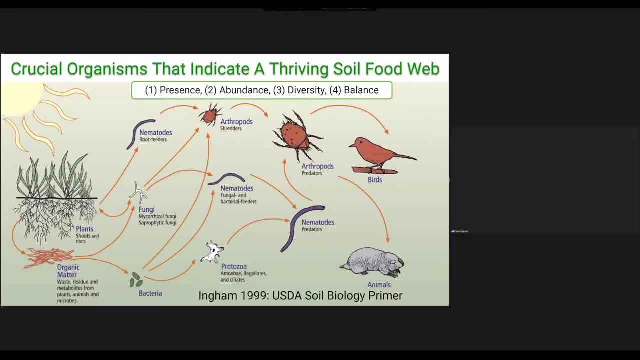 An operating soil food web is going to deliver those nutrients to the surface of the roots. It's kind of like the pizza delivery guy. When you want a pizza, you call up The pizza house And you say I want a cheese pizza with pepperoni on it. 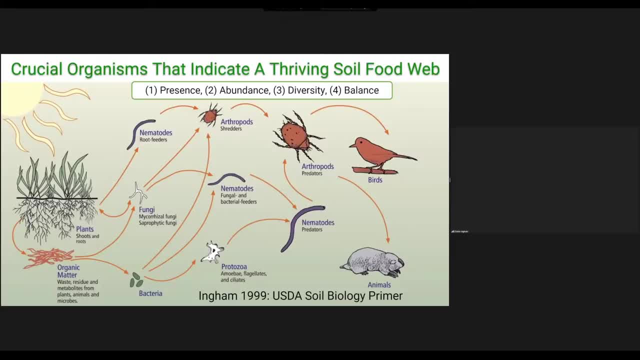 And the root at the other end says: okay, You know, we're going to send out the delivery guy to pick up those nutrients. Make those nutrients available In the shop. Yep, Okay, We've got to make those things into plant available nutrients. 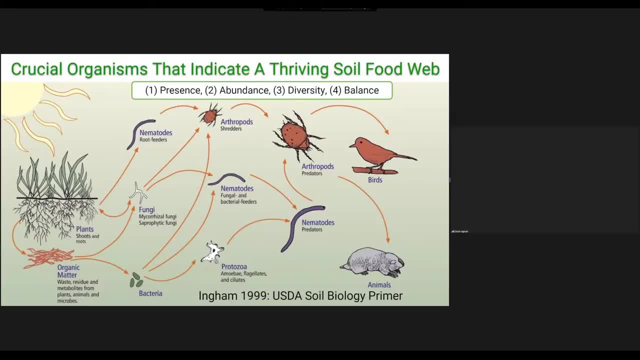 And then here comes the pizza delivery boy, Comes back and delivers the pizza right there at the surface of that root system, So this whole system operating together to be able to feed your plant at the time. And you know then- and I always think of it, as these processes are going on every second of every day, 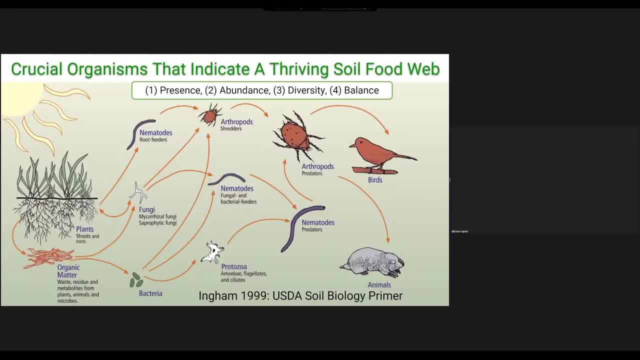 Through the whole growing season for your plants, Making available to the plant, And that's not precisely what it needs, Because the plant can tell the bacteria and fungi what it needs And the enzymes they're supposed to make. And so if you are destroying your fungi, 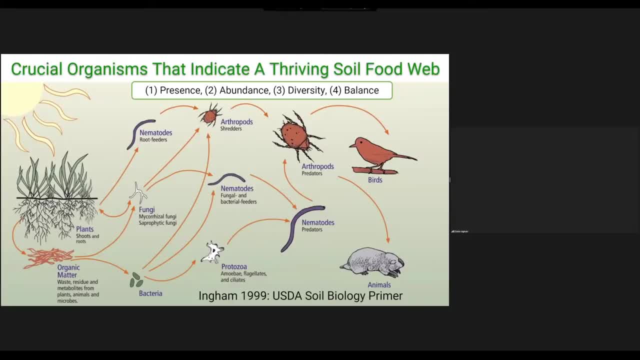 If you're destroying the beneficial bacteria and fungi- Nematodes, microarthropods, protozoa- Your plant's going to be in a lot of pain. You're not going to be able to get all the nutrients into that plant. 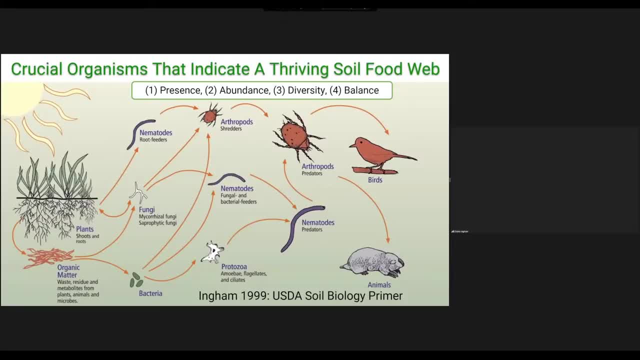 That it requires to prevent- Prevent- diseases from attacking it. The immune system in a plant is very dependent on the nutrients that the plant is getting. Well, human beings are exactly the same. If you're not getting the nutrients that are needed to attack and consume all the bad guys. 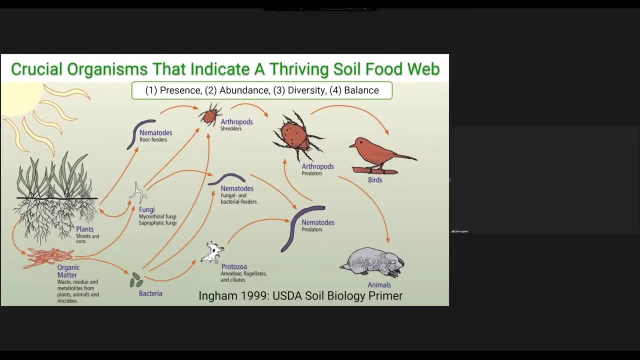 You know getting breathed in Or that you might be eating on your food surfaces. If you don't have the nutrients to build your immune system, You're going to be very susceptible. So, as human beings, so like plants, Or is it so plants, so are the human beings. 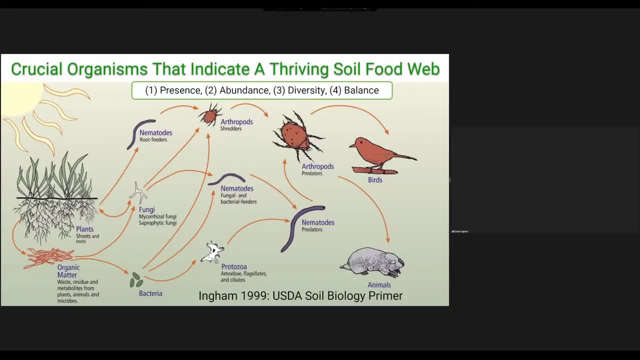 We're shared systems Because Mother Nature found systems that worked And then she repeats them over and over and over again In various places. So when we're looking at this food web- Protozoa, Bacterial feeders, Nematodes that are bacterial feeders. 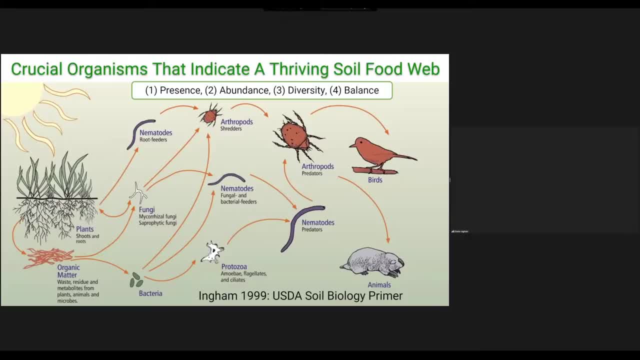 Nematodes that are fungal feeders, Micro arthropods. You can understand their need, Why they have to be there. But why do we need higher level predators? Because if something wasn't controlling The arthropods, the nematodes, the protozoa? 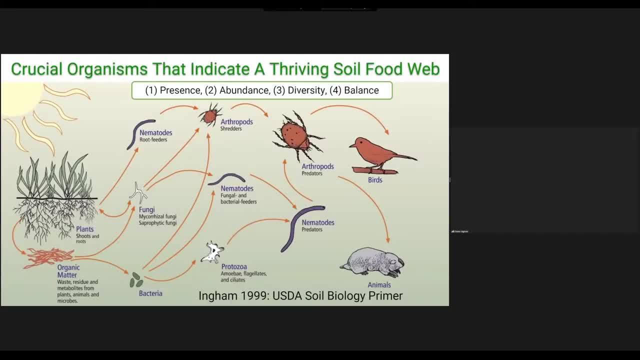 And preventing their numbers from getting too concentrated, Which means then they would overeat And wipe out most of the fungi and bacteria And your plant wouldn't get the nutrients that it requires As rapidly as it needs them. So something's got to maintain the balance. 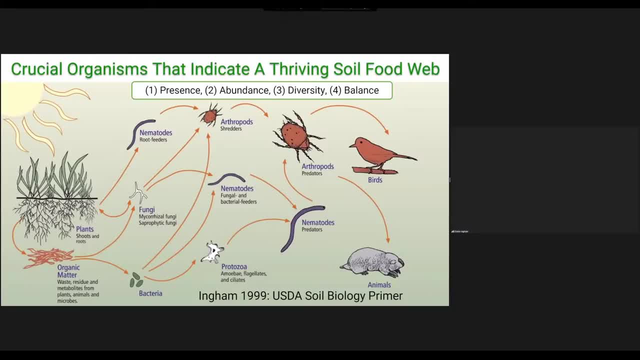 And so protozoa, the micro arthropods, The predatory nematodes, The nematodes that eat these other guys- Yes, there are cannibals in the soil- Because these nematodes eat those nematodes. Well, what keeps these macro arthropods and the predatory nematodes 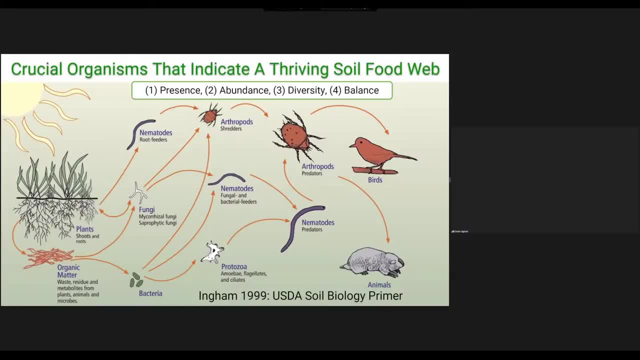 What keeps them in check? Well, you have to have the next layer in the food web And the next, and the next. So who's at the top of the food chain, The top of the food web? more correctly, right, It's human beings. 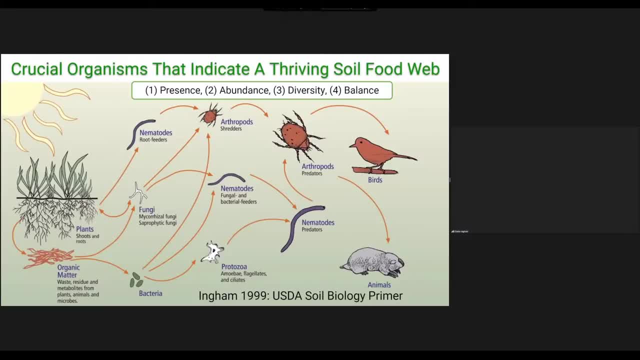 We're here to make certain that this is all functioning the way it should, And instead what we've been doing Is destroying all of these organisms in the soil With the toxic chemicals that we use Inorganic fertilizers. They all kill these organisms. 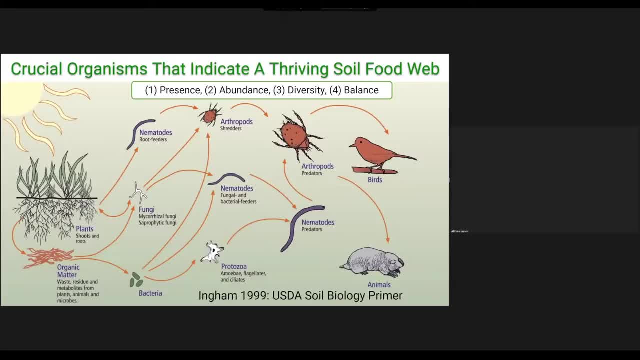 Too high a concentration. The levels of inorganic fertilizers we're putting out Is killing all of this biology. And then you can't get the root systems grow down deep into the soil, Because it is the microorganisms that produce the aggregates. 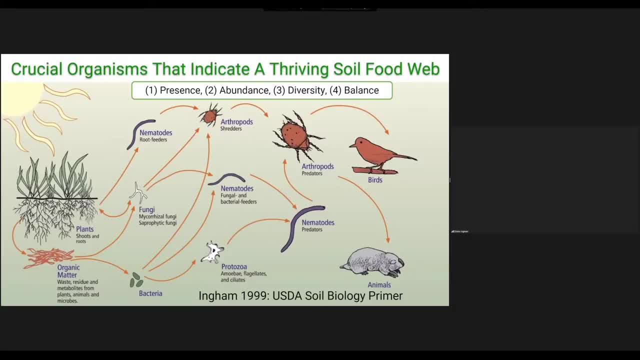 Without the bacteria and without the fungi, Without the higher level guys here building airways and passageways- And even these guys building airways and passageways- We wouldn't be able to survive. We wouldn't be able to get oxygen down into the soil. 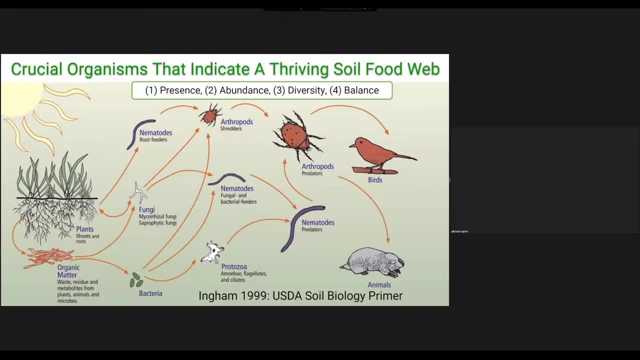 Water wouldn't infiltrate, You would have erosion. Most of your soil would be washing away into the rivers and lakes and streams And the oceans. Oh, wait a minute, That's exactly what we've done. Well, thanks so much for bringing that part up, Elaine. 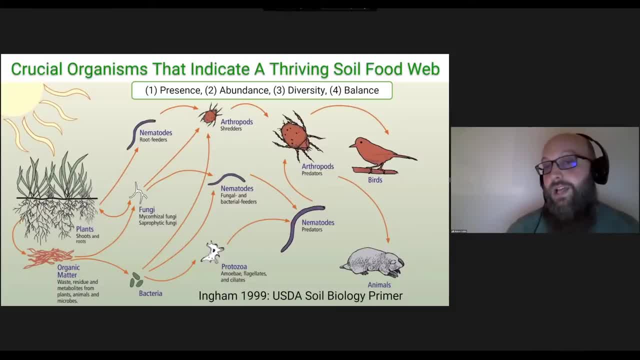 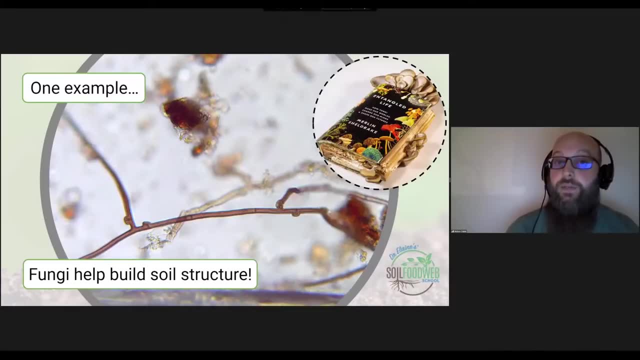 Because I want to move us forward on the slide Just for the sake of time here, Because we've got to get to all of those benefits that are coming up, And just you know one example That you brought up that's so critical. 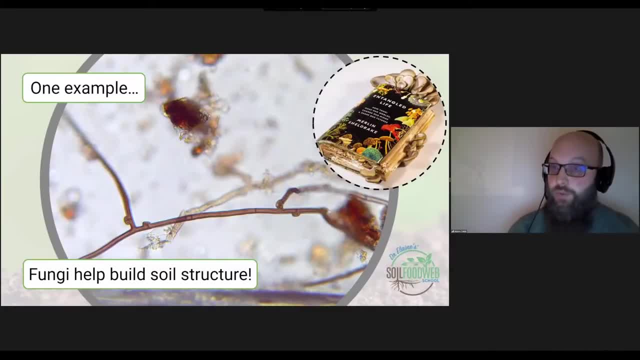 Is the way that fungi can help us build that soil structure directly. And I've put in just a little plug for Merlin Sheldrake as well here In his book, Because we recently had him at our soil summit in a panel And it was a lot of fun to see. 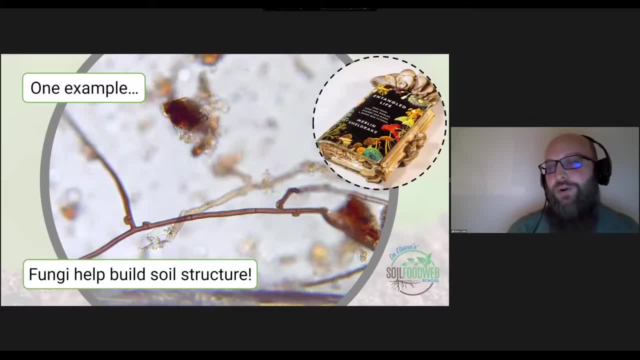 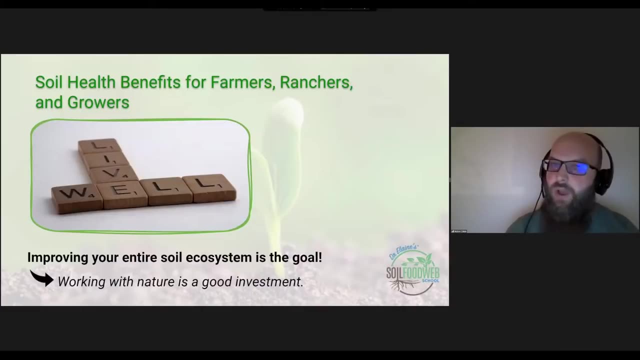 We called it the mycology mind meld, Just to go over all the benefits of this one group of microorganisms in the soil. But let me progress the slide here again And mention the range of benefits You know, starting just with again that idea of wellness. 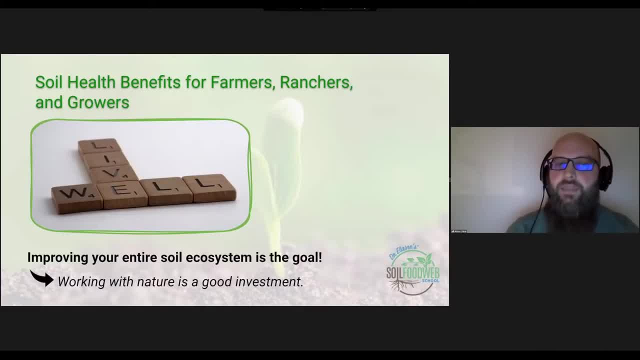 That we have a holistic soil ecosystem And that improving that entire ecosystem is our goal. It's why we work on restoring anything that's missing from the soil food web. As Dr Elaine has explained, Each organism has a purpose, And it would be. 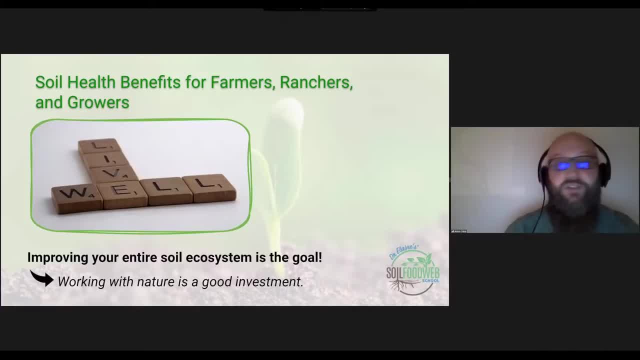 A complete folly of us to assume that none of them is needed in the soil ecosystem. So working with nature is a good investment: Having our growers and our gardeners, our farmers and ranchers, our land managers Make the investment to get anything that's missing from the soil food web right back into there. 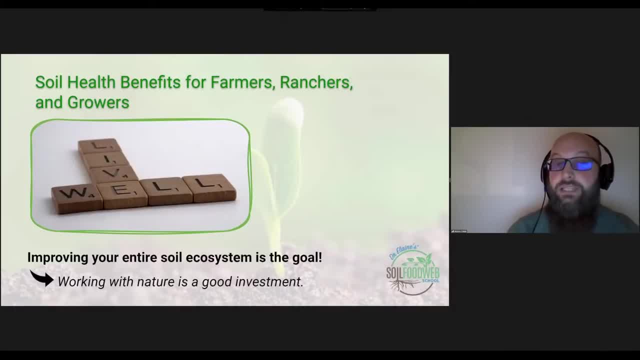 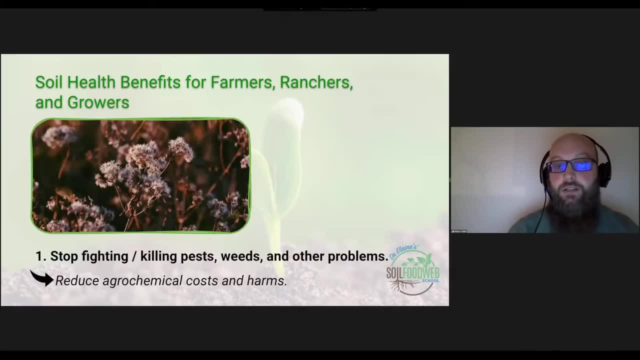 You know, this is the way that we have a healthy, functioning, complete ecosystem. To dive into a more specific example, Brian, if you'd take us forward on to the next slide, What we see a lot of times is that every day, food producers are waking up and thinking. 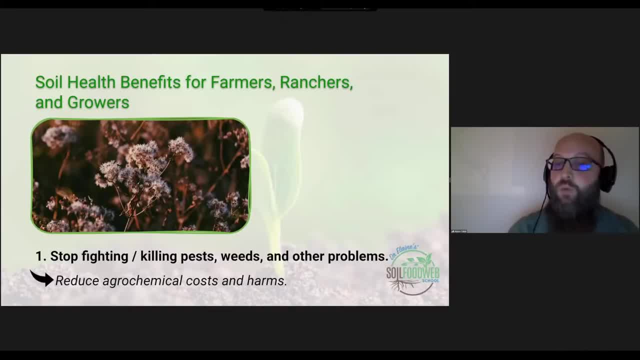 What do I have to fight and kill today? What pest, What weed, What insect? What other problem am I going to have to tackle today And, in reality, these agrochemicals that are being employed so often to solve these problems? 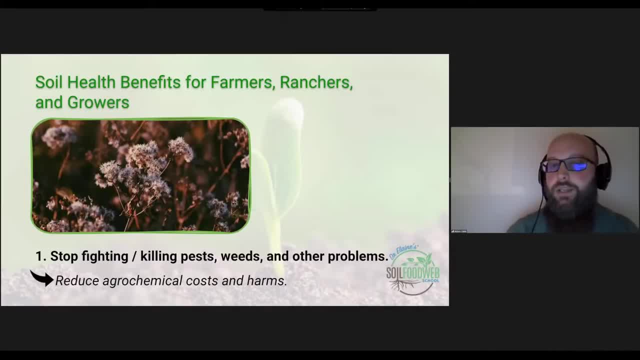 Are just creating more problems. As Dr Lane mentioned, they're wiping something out of the soil food web So that the system becomes unbalanced and incapable of maintaining its own processes. So when we focus on soil health and when we put the soil food web at the center, 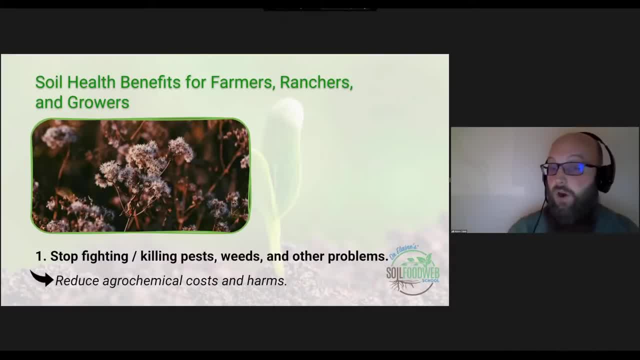 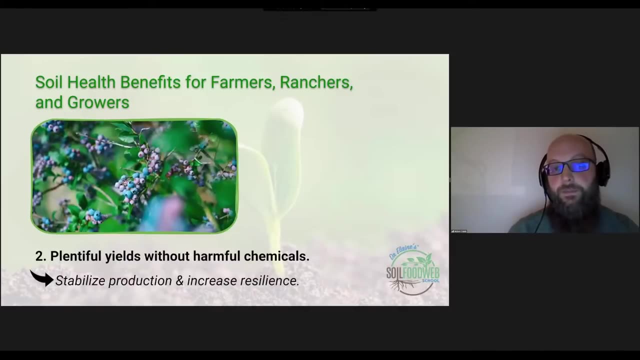 We can eliminate the use of these harmful substances And actually see that pests, weeds, insects and other problems diminish over time As we transition that lane. And Brian, if you'd take us forward to the second example? Everybody cares about yield. 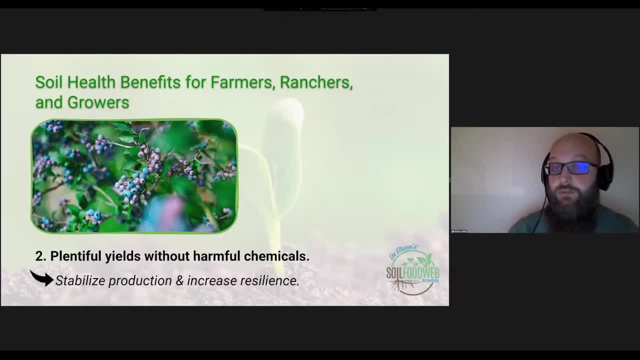 And in fact you know we're all anybody who's involved in an agricultural business. They have to consider their production, their profits, But longer term, not just every year making enough yields to keep the farm going, But longer term. this new idea is arising. 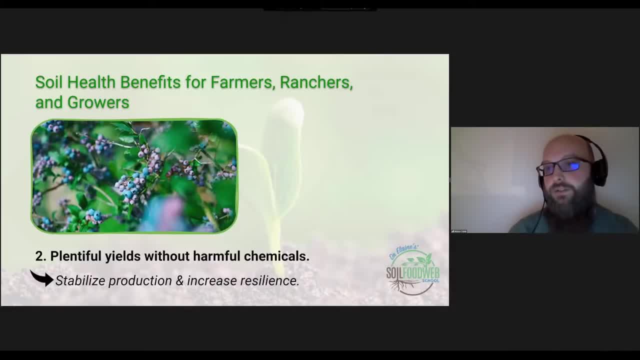 Everywhere in the agricultural sector of resilience- The ability of these systems to recover from stress, Whether that's periodic drought and extreme weather events, And so stabilizing the production on the farm is one of the things that we can do without harmful chemicals. 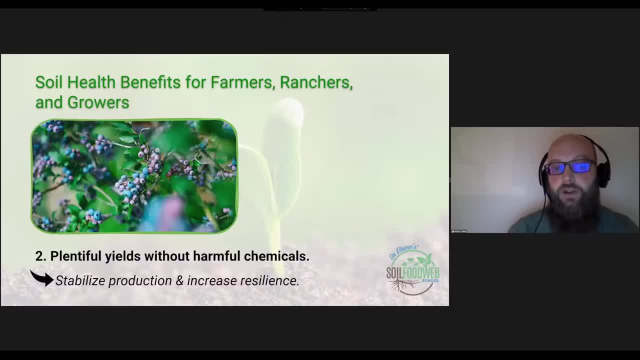 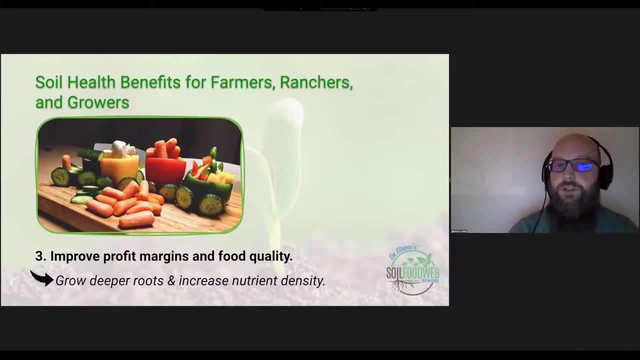 If we have a complete soil food web And our next example or benefit is that we can improve those profit margins. As I mentioned, But not just you know, in the last maybe 50, 100 years of human history, It's been sort of a game of saying: increase the yields, increase the yields. 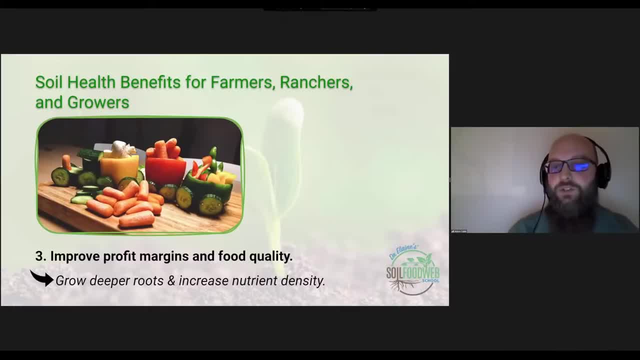 This is what most of the agronomists out there are researching. But today I'm really excited that we'll hear about food quality. You know that's a huge function in terms of increasing that nutrient density of foods, So that the societal costs of poor human health are tackled by the very food we eat. 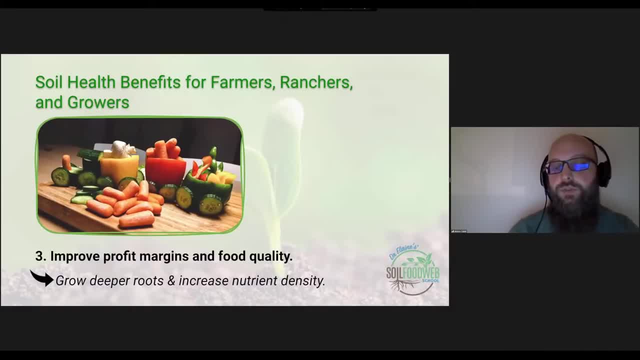 The food can be the medicine, And that's because these roots on our crops will grow deeper. They'll get more access, through the soil food web organisms, to nutrients So that they can collect those nutrients into the food products that we consume. And the next slide talks about the soil sponge. 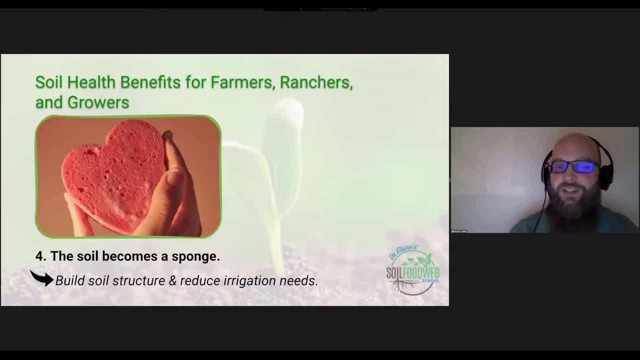 Which is a huge part of what DeeDee talks about as well- That as we build that structure, our irrigation requirements can be reduced And, as Dr Elaine mentioned, we can see less of a problem with erosion over time, Because that water that falls into our food system soils will actually percolate into the soil. 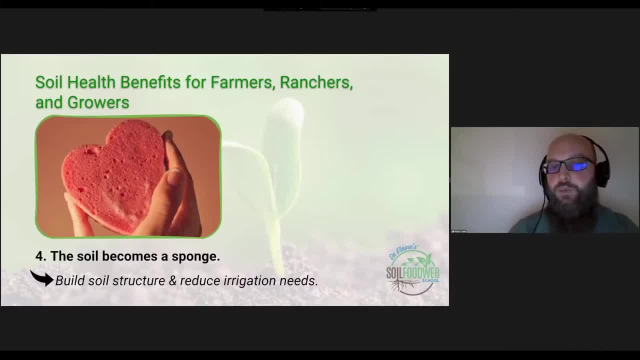 It will infiltrate and go to those deeper layers, Nourishing the life deeper and deeper into the soil, Instead of running off the field and taking a bunch of eroded soil with it. And so this will lead us to the next slide. 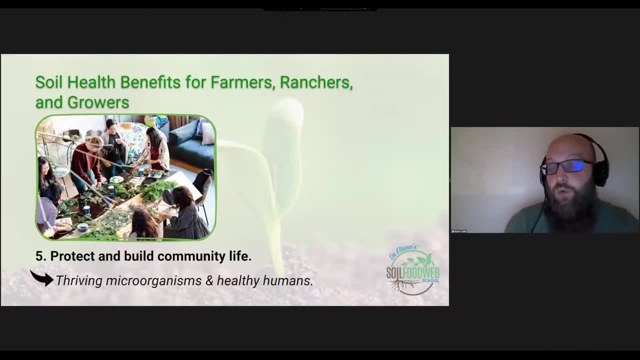 Which leads us to our final example here, Which is that we'll protect and build community life, And I mean that two ways: The life of the community, of the soil food web, will be protected with soil health improvements, But also human community Right. 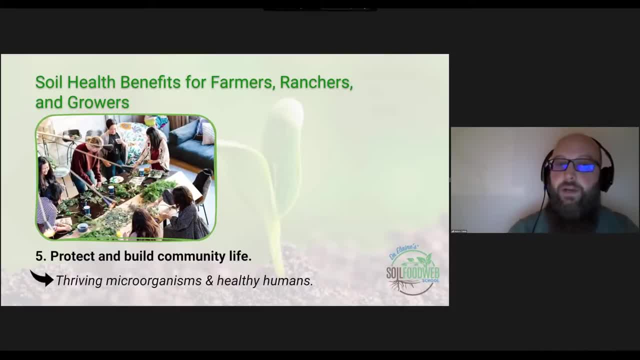 That we can have these thriving microorganisms And through the services that they provide to plants and the food- ultimately, The quality of the food that's produced- We eventually arrive at healthy humans. As Dr Elaine said, we could think of ourselves as the top of the food web. 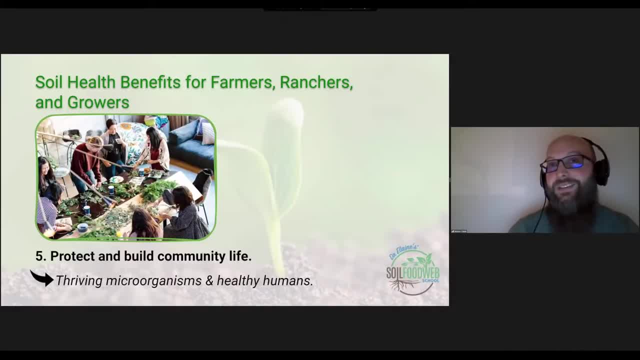 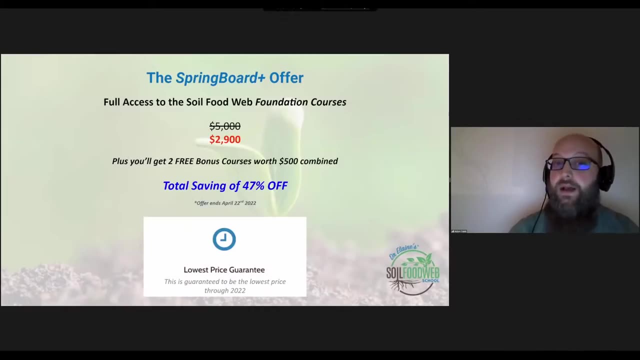 But also, I think, of how the food web is this miracle that gives so much to us And we should be grateful for that miracle. So, if you'll take us to the next slide there, Brian, We're going to talk a little bit about the special 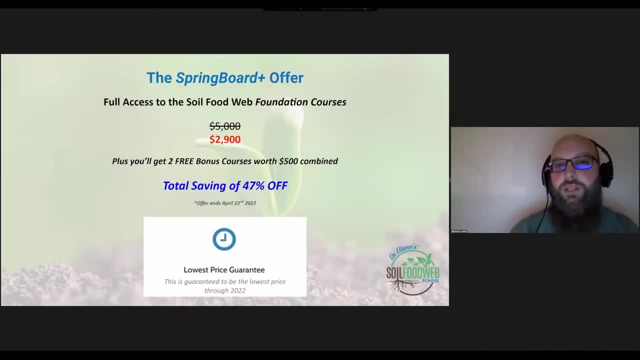 We're calling it the springboard offer, Where anybody who is interested in taking our foundation courses can get a huge discount, Which we guarantee will be the lowest price available for this package of courses in 2022. Representing a total saving of 47%. 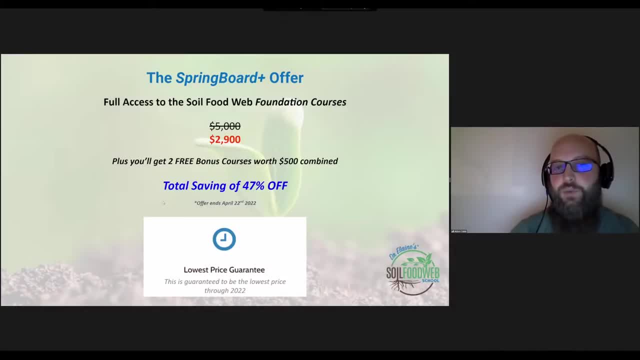 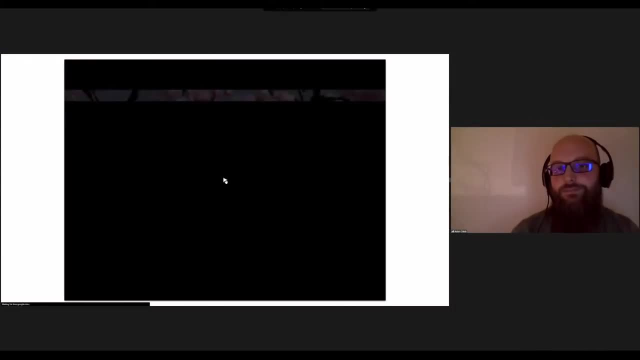 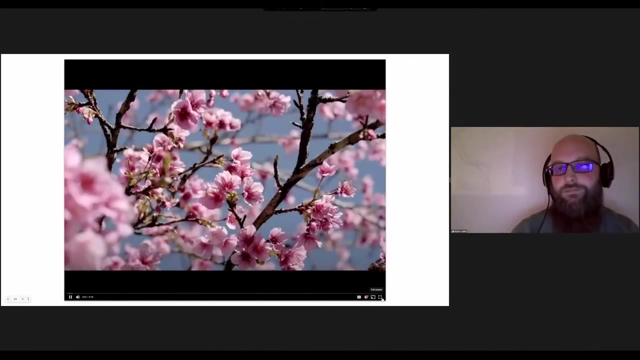 We actually have a video that we're going to show, Just a brief, three minute video about this offer. Spring is in the air And there's never been a better time to launch your career in soil regeneration than right now, With the springboard plus offer. 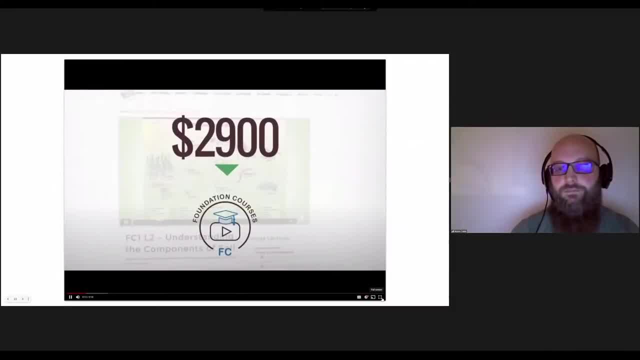 You can register for the soil food web foundation courses for just $2,900. And you'll get two free bonus courses, Saving an incredible $2,600.. Or 47% off the regular fee price. This is guaranteed to be the lowest price. 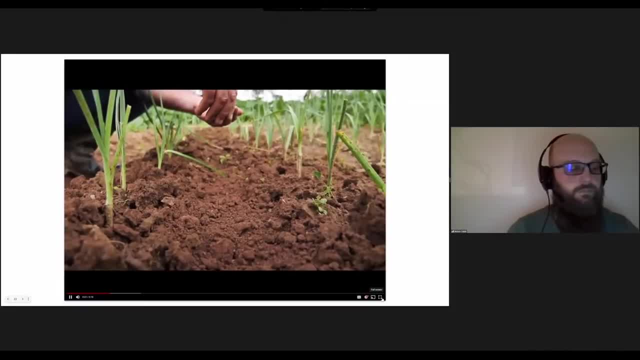 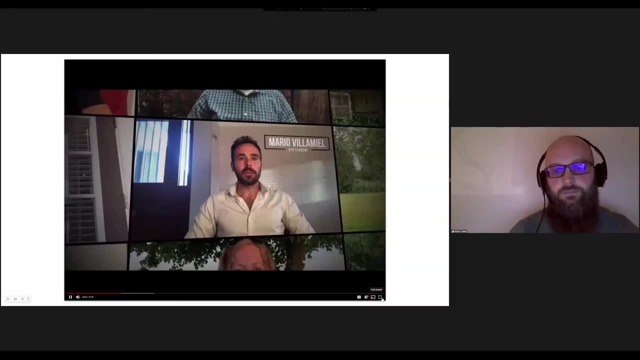 That's through the rest of the year. Whether you're a farmer, Rancher, Market gardener Or just someone who's passionate about the planet, Looking for a way to make a big impact, This could be for you. Here's what some of our students are saying about the soil food web training program. 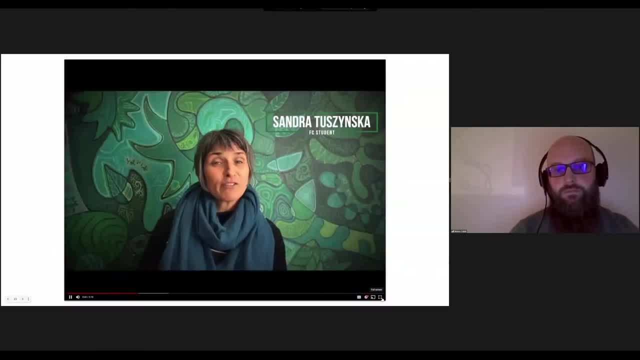 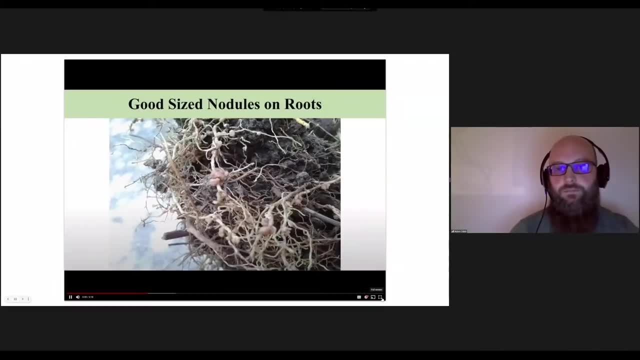 I find that this information hasn't been taught to me And I had to get off my high horse And, even though I have a PhD, I feel like I'm totally under trained. I feel like I'm learning more with this program Than I have with in-person classes in the past. 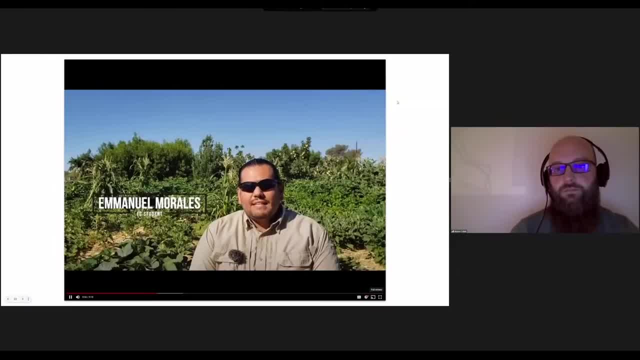 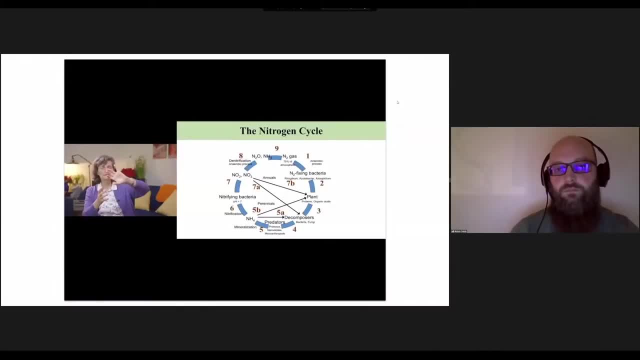 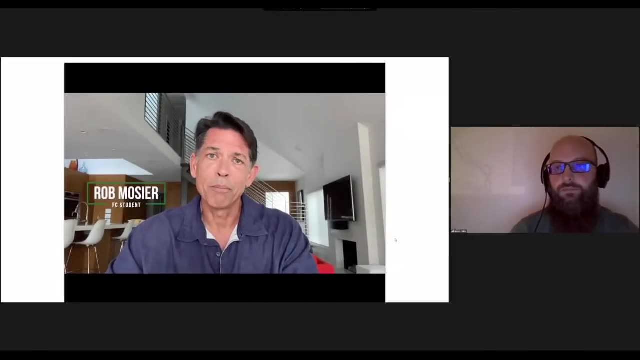 I've taken classes on microbiology before, But this course really makes a difference In the way that a story is put together That unveils the relationships between plants And all those beneficial organisms that we just cannot see without a microscope. If you're looking for something that does a deep dive into soil biology, 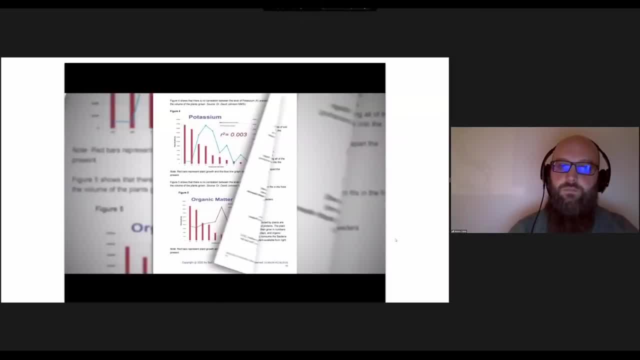 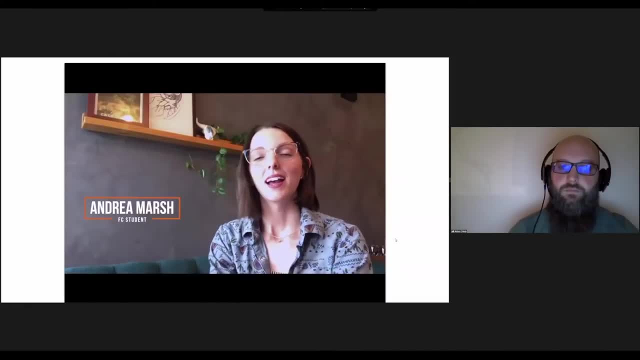 This is it. It is just an incredible knowledge base, And it's really relevant to what's going on right now In the world. Without it, the only way I could have gained this knowledge Would have been by dropping my life And going to graduate school. 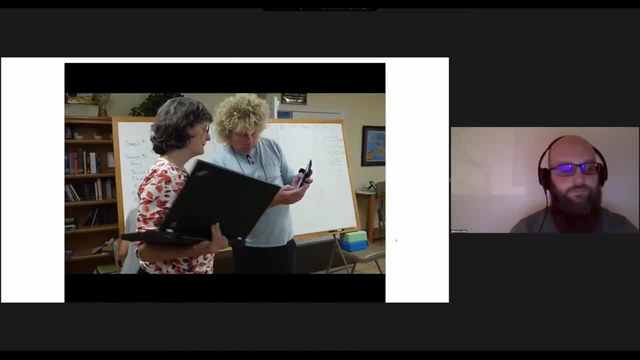 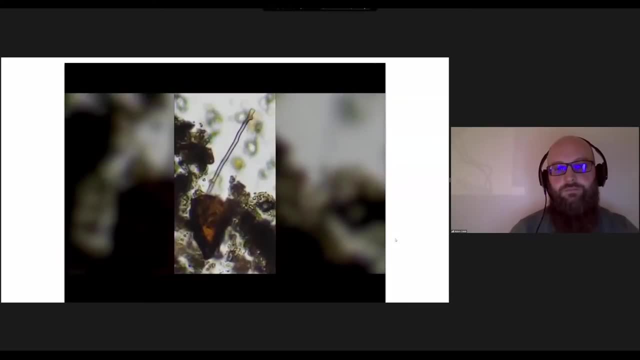 And that just wasn't realistic for me. But soil food web has made it possible For me to build a meaningful career in land restoration. I was really nervous that I was going to put quite a bit of money down And not get that bang for my buck. 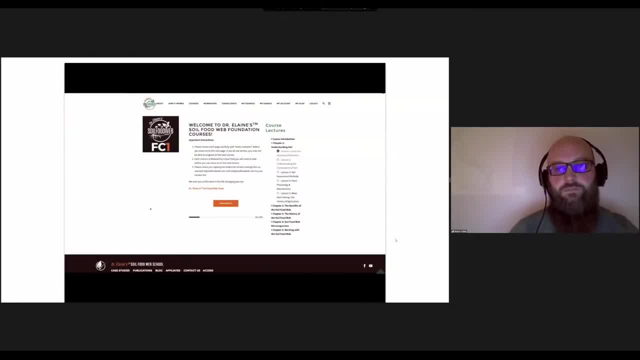 But once I actually got into the FC courses I was incredibly impressed with how professional they are And actually the level of education you get That you receive. This is the career path I've been looking for In the biological community And I was having trouble finding. 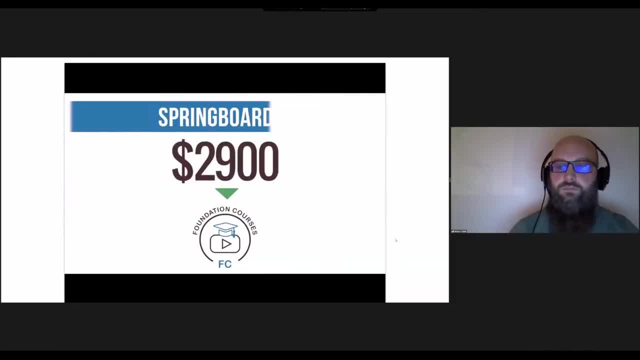 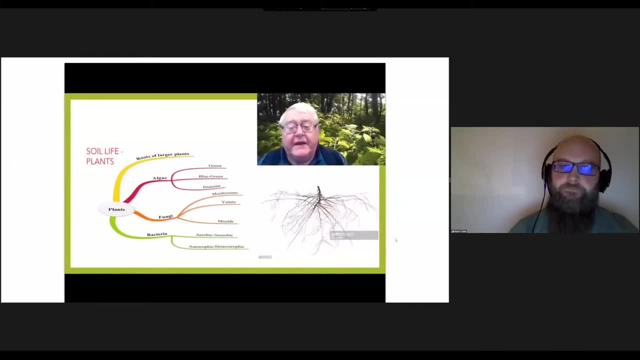 Remember, with the Springboard Plus offer, You're not only getting the foundation courses for $2900. But you're also getting these two free bonus courses. The Introduction to Permaculture is an 18 lecture course That covers a wide array of permaculture principles and themes. 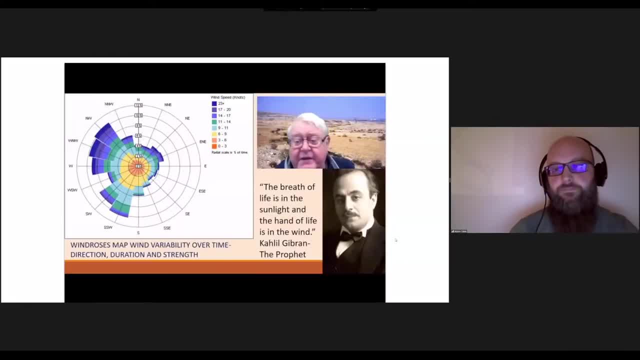 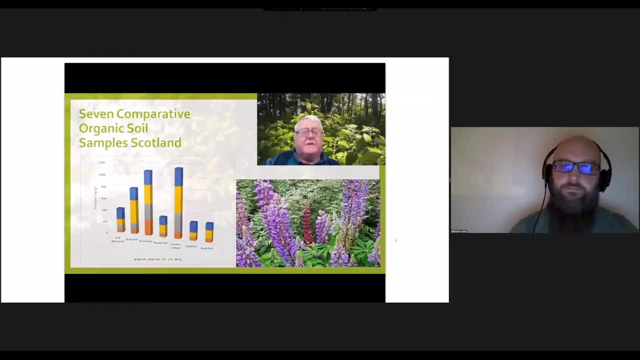 Delivered by Graham Bell, Chair of Permaculture, Scotland And longest serving permaculture teacher in the UK, With 31 years experience Teaching on six continents. Permaculture is a regenerative design approach That can be applied to just about anything. 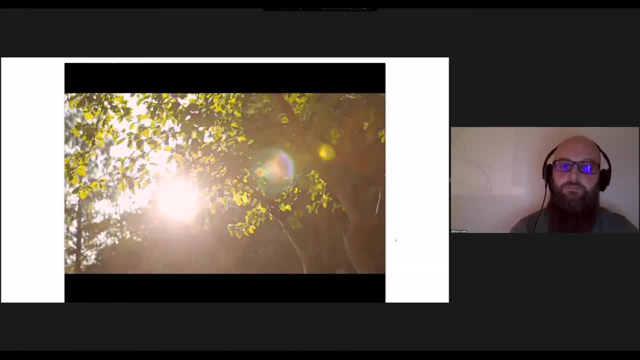 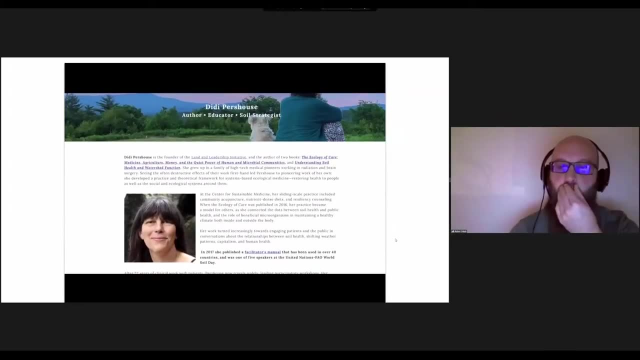 From water management, Growing systems, Dwellings And much more. The Soil Sponge Regeneration Workshop Is delivered by educator and author Didi Persaus. This five session course Is all about regenerating the soil sponge For flood, drought and wildfire resilience. 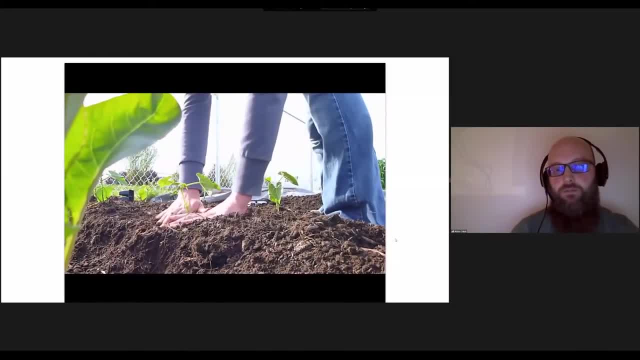 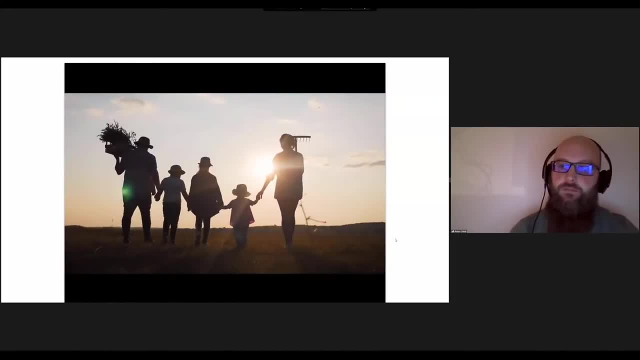 It builds on the successes of innovative land managers Around the world Who are saving huge sums and damages From extreme weather events and crop diseases, While restoring the dignity and profitability of farming. Didi teaches participatory workshops Both in person and online. 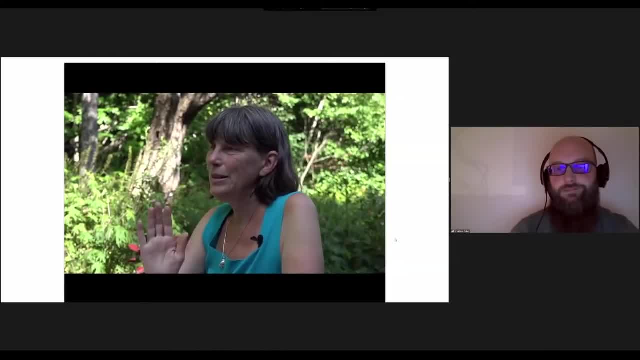 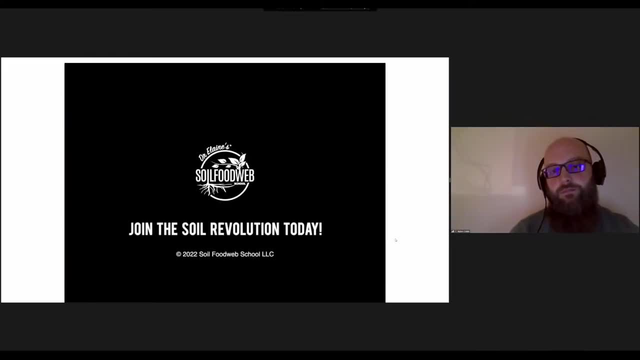 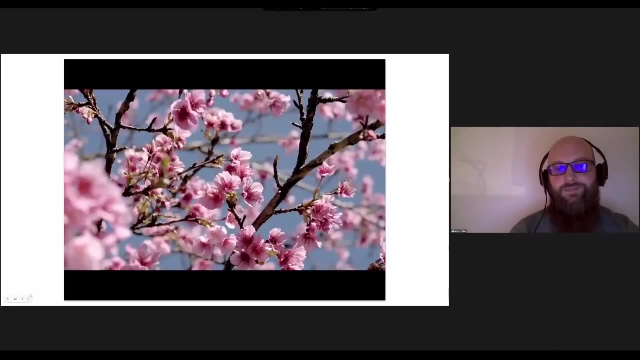 Helping to show the nested relationships Between soil health, Human health, Water cycles And climate resiliency. Sign up for these amazing courses And join the soil revolution today. Okay, So we're going to actually switch gears a little bit here. 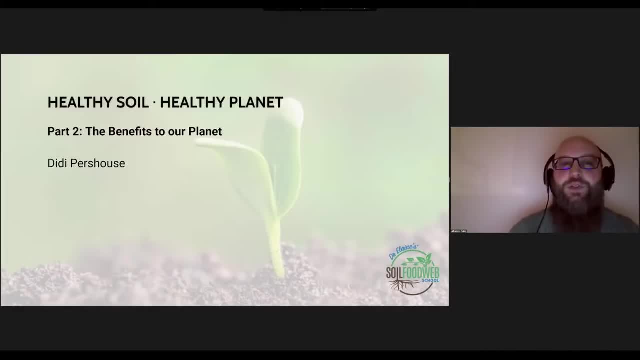 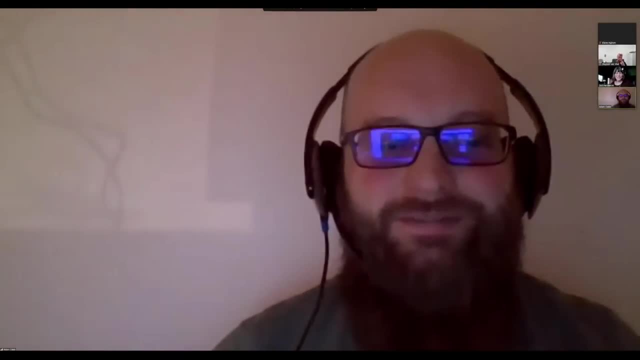 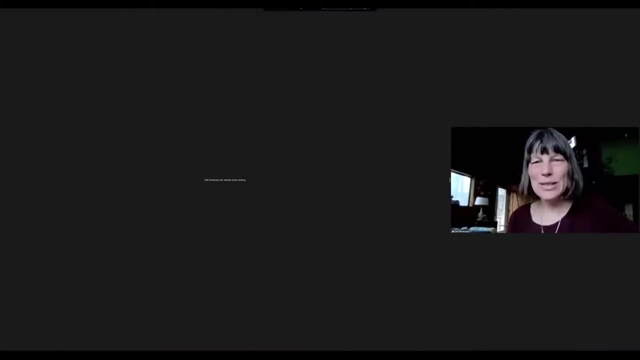 And hear from Didi About the benefits to our planet of healthy soils, And she's got her own slide deck, So we'll turn that over to her. Great, That was exciting to listen to And it was also- It's fun to read all what's going on in the chat. 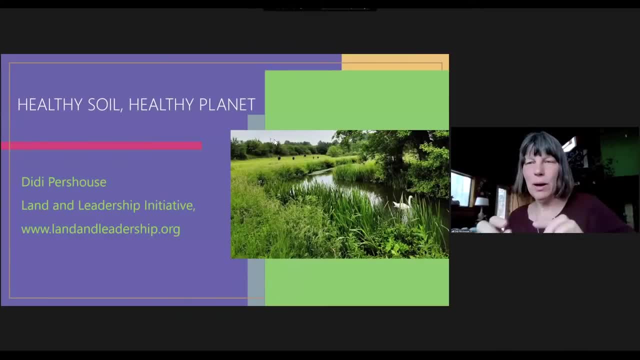 Those who are being distracted by the chat. You can open it up And it'll be a box And you can drag it off to the side, Because I know sometimes you can't see a slide When it's going there. So I am from the Land and Leadership Initiative. 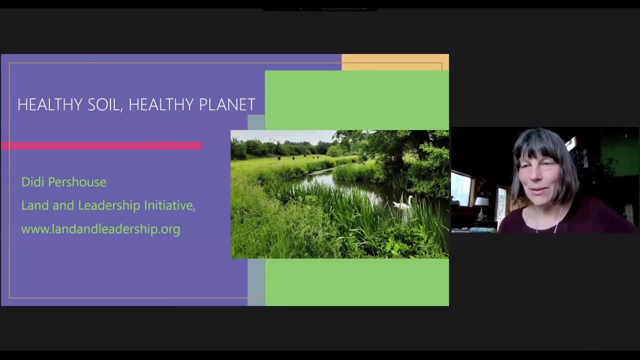 And, as you just saw, I'm also really excited to be teaching a course Alongside the Soil Food Web School And I saw a question in there somewhere About how is the Soil Food Web School building community And one of the ways they do that. 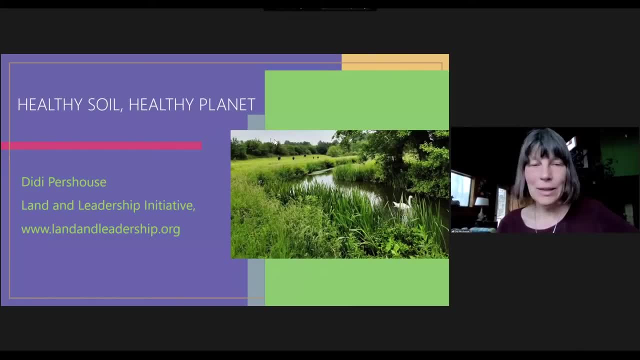 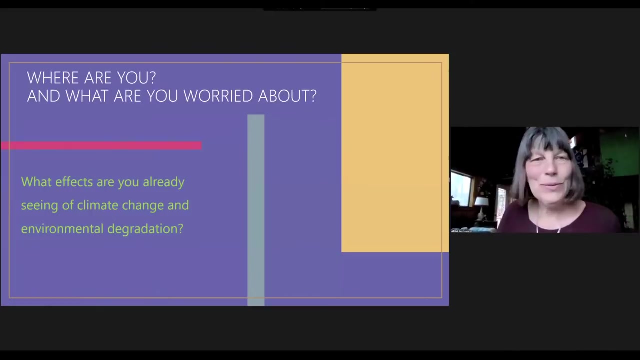 Is through this live five session course Where we do lots and lots of breakout discussions. So you'll get to know people from all around the world, And that's fun for me as well. Okay, So you've already typed some into the chat. 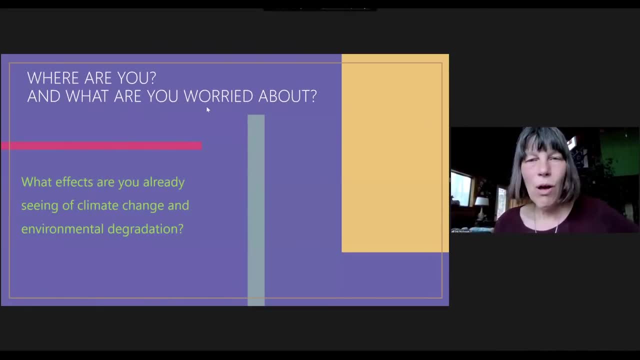 About where you are, But put that in again Along with: what are you worried about? What effects are you already seeing of climate change And environmental degradation? So go ahead and put that right into the chat, Just whatever you are seeing. I know in Vermont. We've had horrendous flooding, Lost hundreds of miles of roads and bridges. I'm seeing pests, Erosion, Increased drought, Fire, Freaky weather, Impacts on human health, Missing food in the future, Algae blooms, Birds dying. 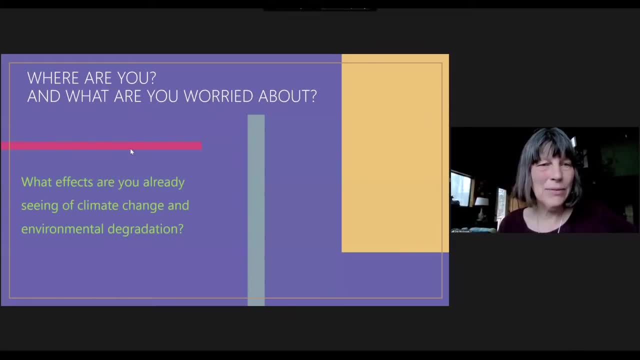 I can't even read these. It's going so fast: High winds, Much less rain, Storms, Yield drop, Erosion, Desertification. And then how about the social effects? Social effects of environmental degradation, Social Yeah. 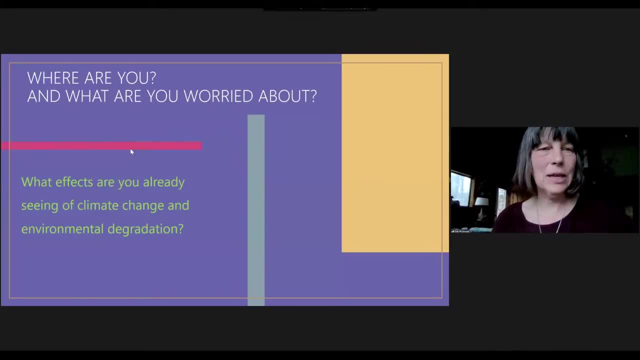 In terms of biodiversity Right Insects Abandoned pastures. I know there's a lot of people having to move Because there's not enough food and water in their area, And then, of course, we get into conflicts over resources. Okay, 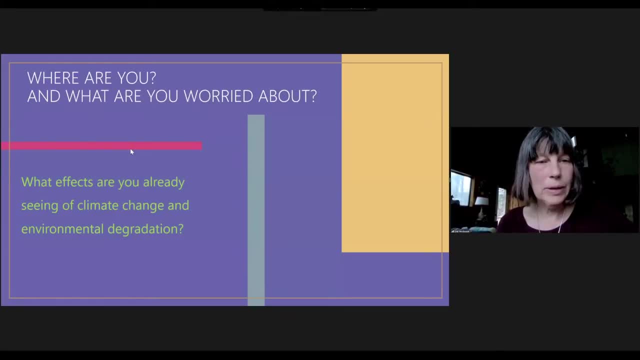 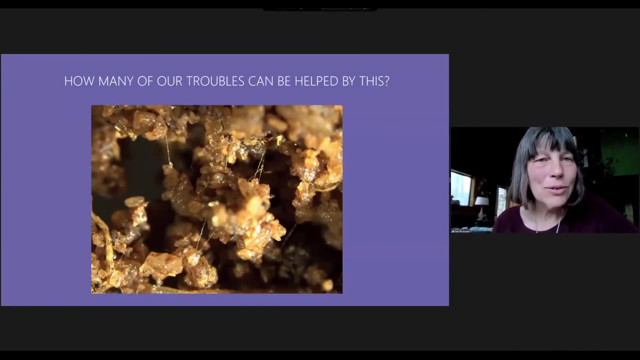 So I'm going to keep going, But note all of these things that are going on, Including depression, that I just saw flash by there And, sorry, My controls are covering my slides, Let's see. So the question I want to get at here today is how many of our troubles can be helped by this. 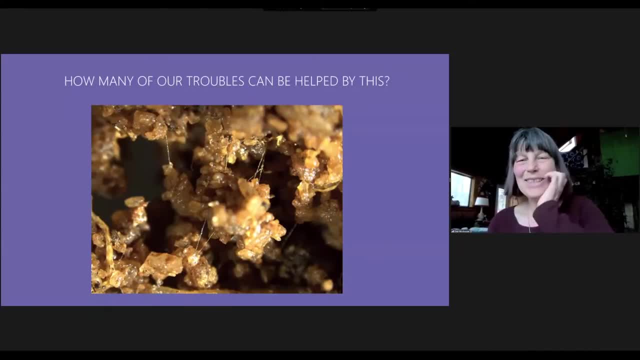 What is this funny thing on the screen here? This is a soil aggregate. You heard Elaine make reference to it. This is sand, silt and clay, Little broken down rocks. It's made together by biological slimes and glues. 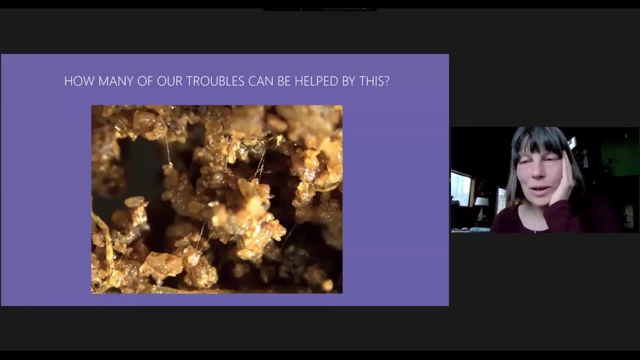 And the little threads of life, The fungal, hyphae, plant root hairs, et cetera. So it's like sticky and also tied together, Little bundles of tiny rock particles, And as you can see there are. it makes space. 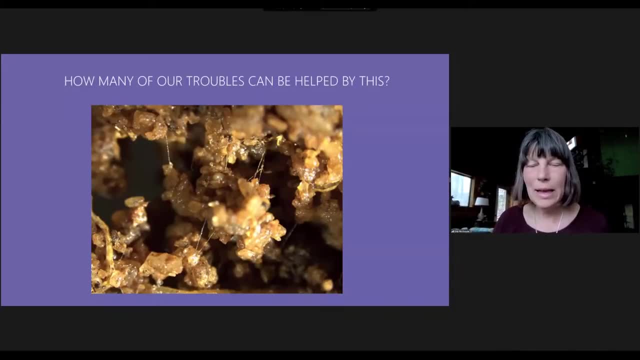 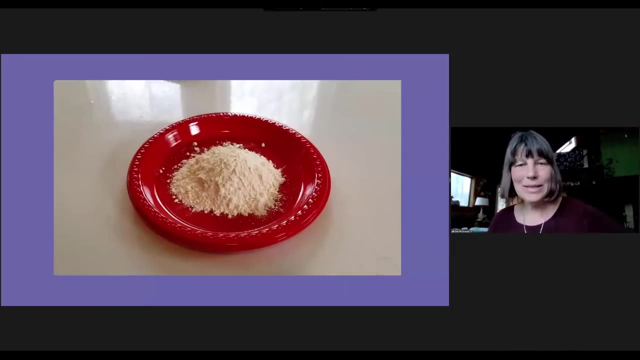 So what would be just a pile of sand, silt and clay suddenly has structure to it, And I, as an educator developing curriculum, this was something I came up with. Now, people around the world are using this as a teaching tool. 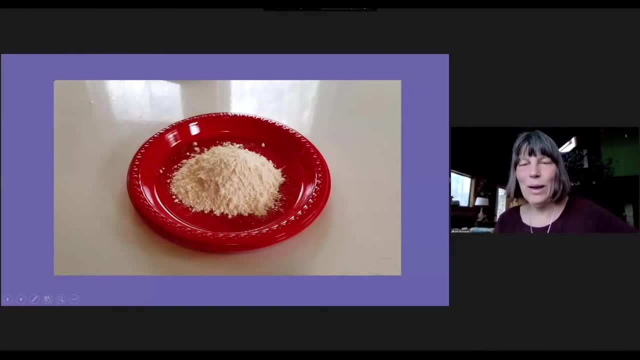 But it's a really, really visual, quick way of getting across degraded soil or unhealthy soil versus healthy soil, And it's a comparison between flour and bread. So if you think about soil, Unhealthy soil is just individual particles of sand, silt and clay that are not held together. 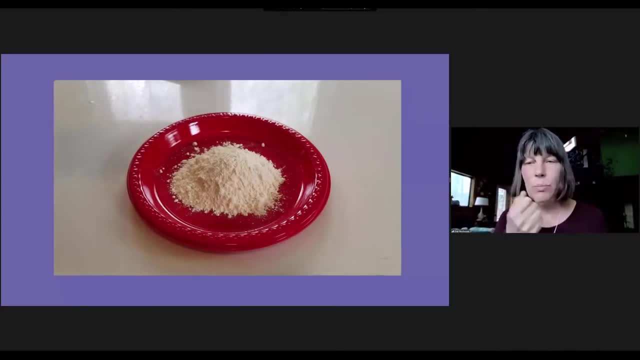 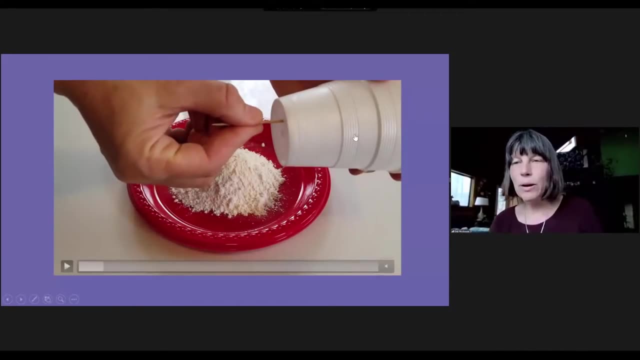 It's like a pile of flour on the ground, And if you pick this plate up before we rain on it, If you picked it up and blew on it, those soil particles would go all over the place, Right, And so that's one thing is that there is no soil structural integrity to wind. 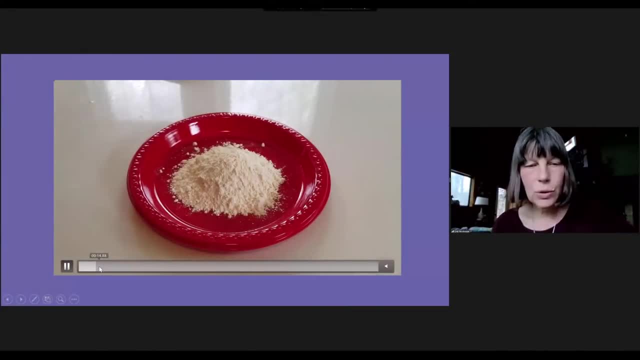 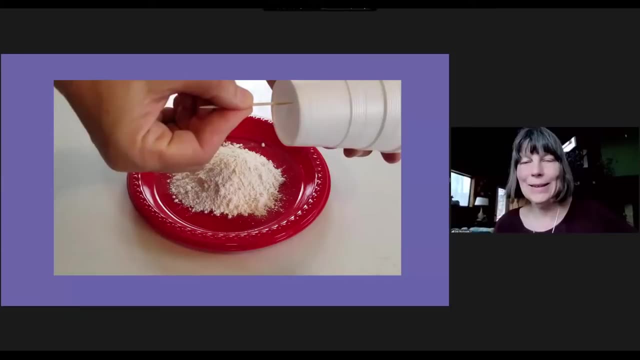 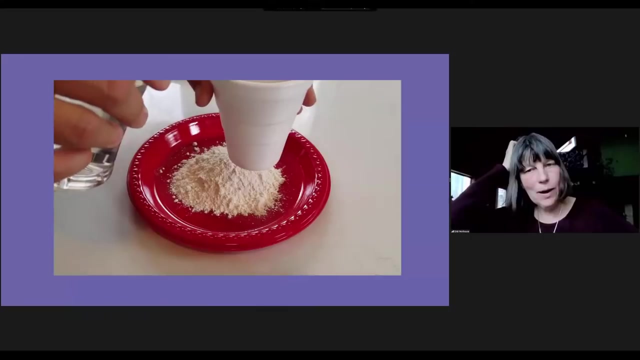 And we see that on the land. So but what happens if you rain on a degraded soil or an unhealthy soil, Or soil that I would say that does not have the structure and function of a sponge? So we can do this experiment: Make a few holes in the bottom of a cup. 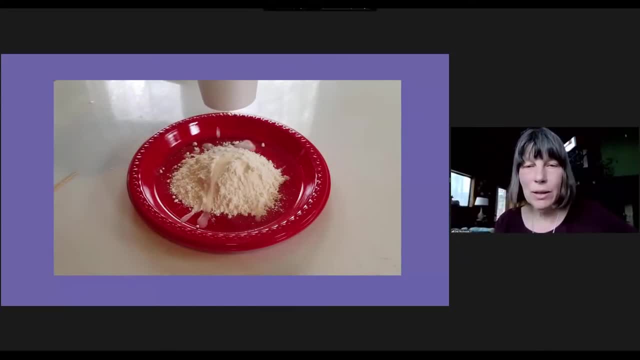 Pour the water on that degraded soil, And of course you can do this out on the land as well with soil itself. But what are you seeing? You start to see erosion Mudslides Flooding, And anyone who's done any baking knows that. if you were to dig your finger down there. 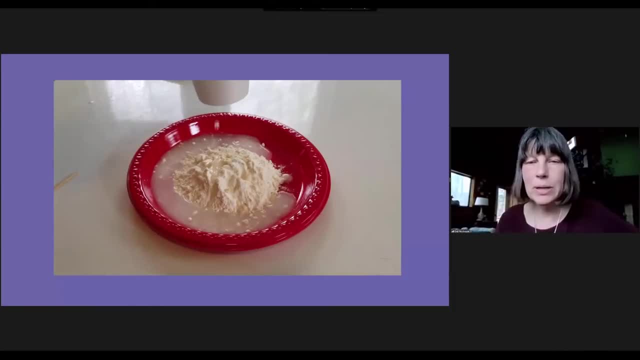 All that water. it's making something sticky on the top, But it's completely dry underneath. There's no water getting down to the plant roots, There's no water getting down to refilled springs or groundwater, But you are having flooding. So this is why flooding and drought are actually two sides of the same issue. And for more reasons than that, Because actually, when we have water that gets down to the plant roots, The plants can then photosynthesize and transpire, Which is like sweating, And that's how the water cycle gets going on land And kick starts the rain cycle. 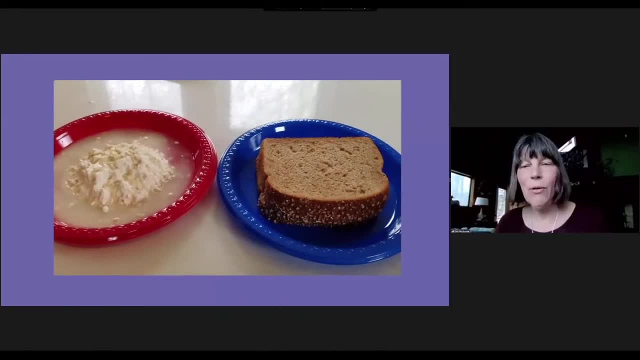 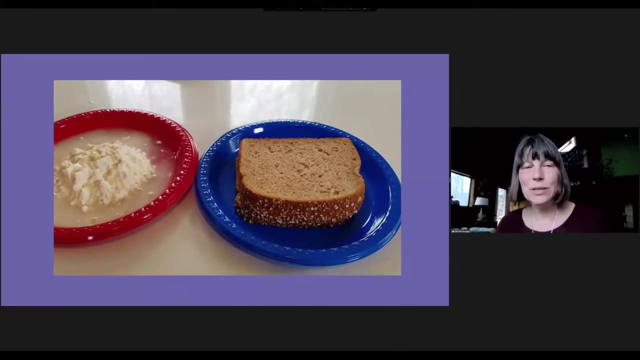 So what is the difference? How do you take flour and turn it into bread? Well, you add biology, And that's what we're here about today. So biology takes those little individual particles And sticks them together into something that has a different structure. 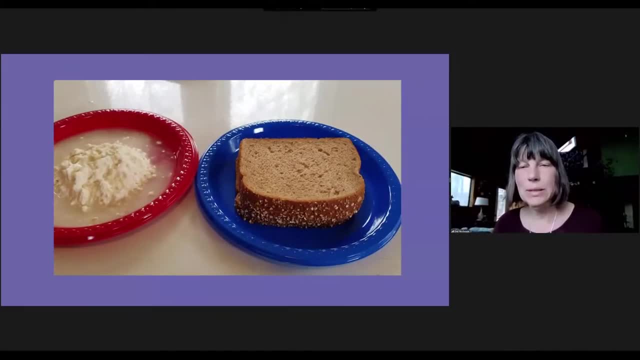 It has holes in it Has pore spaces And the sticky stuck together parts are called soil aggregates. First of all, if you blew on this bread, You wouldn't have anything going into the air, But if you rain on it, Something really magical happens. 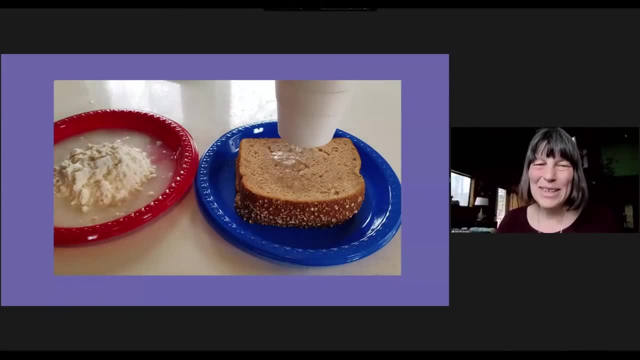 I guess that's our word for the day, Because here at this point, on the other plate, Everything was already falling apart, Right, But what's happening here is it's going sinking in, Percolating down And it's refilling all of those. 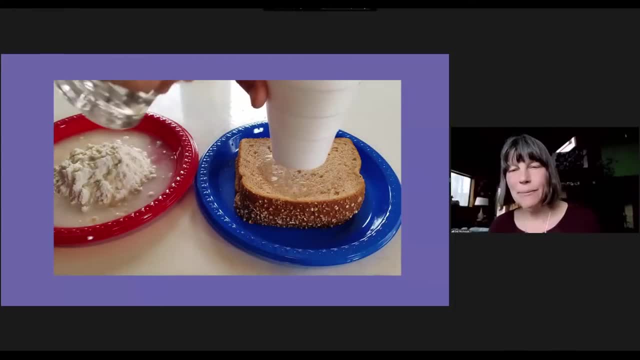 The groundwater and the springs And the streams. It's getting cleaned as it's going through there. The plant roots are happy Drinking it up. It's protected from evaporation. There's no erosion happening, There's no flood happening, Because in a real landscape, 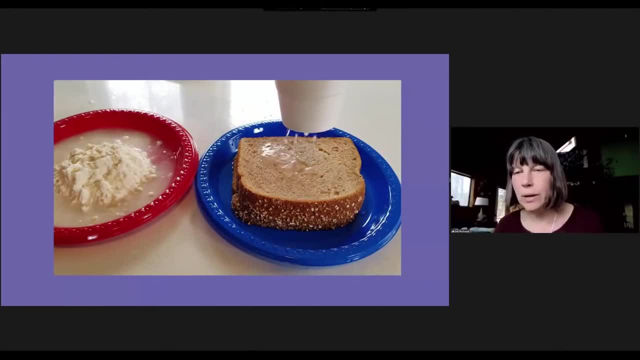 What you're seeing seeping out down below Is that clean, abundant water That's refilling the springs underground, That's refilling the groundwater. That's there for plant roots, That's there for all the life underground That needs that air and water. 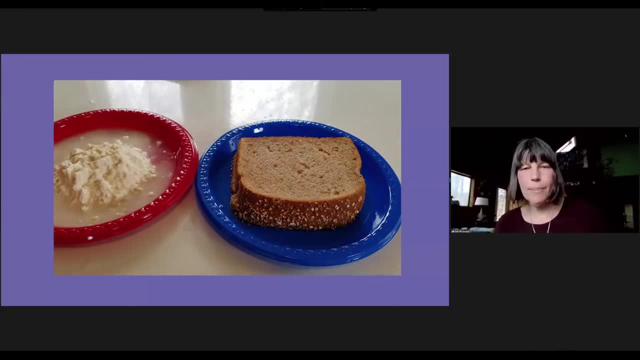 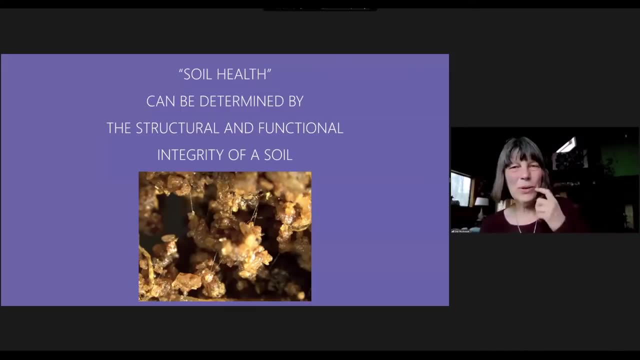 That those pore spaces make possible. Okay, So We're talking about definitions of soil health. One way that I like to think about soil health Is that it can be determined by the structural and functional integrity of a soil, And that's what I call a soil sponge. 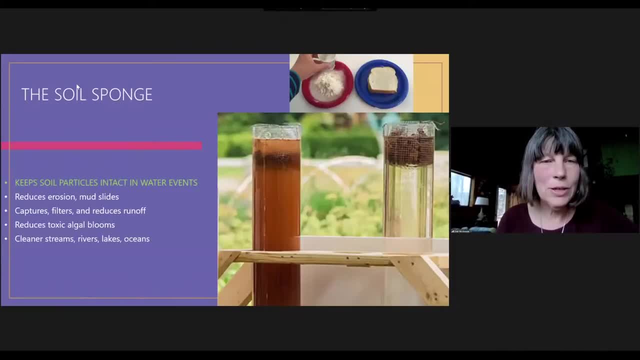 So The soil sponge, Which is just a little review with some different ways of looking at it And a little more information. It keeps soil particles intact in water events And you can do this experiment. You can take a little screen or an onion bag or something. 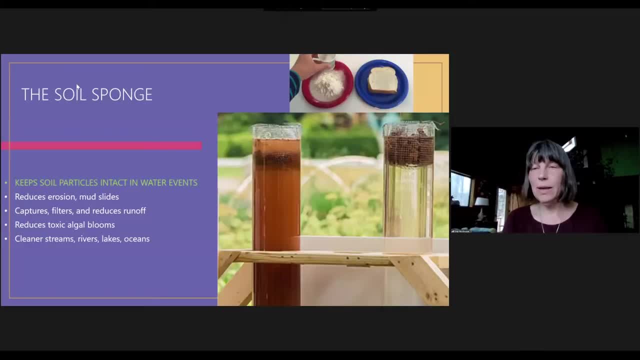 And take some soil that you think is maybe not so healthy, And some soil that has that nice like bread like or cake like structure, And very gently immerse it in a cup of water. It doesn't have to be a fancy tube like this. 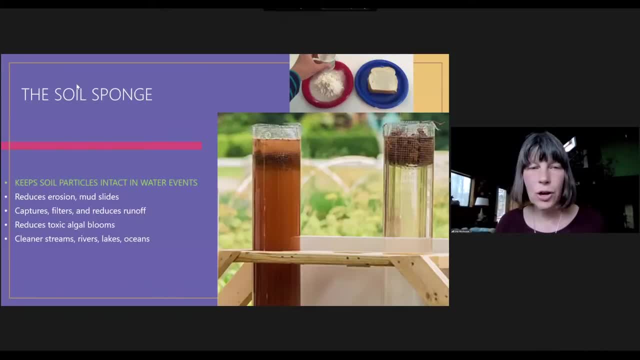 It could be just a any sort of a clear jar And you'll see that those slimes and glues, Those little threads Keep that healthy soil together. Even if you leave it there for hours, That water is going to stay clean and clear. on the right. 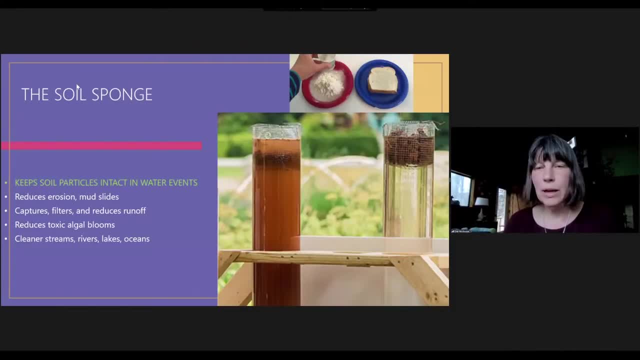 Whereas the unhealthy soil just explodes And fills in the water. You'll see this in rivers after a rain. After a rain, does the river run clear Or is it brown and muddy? So a really key piece of this: The structural integrity of healthy soil. 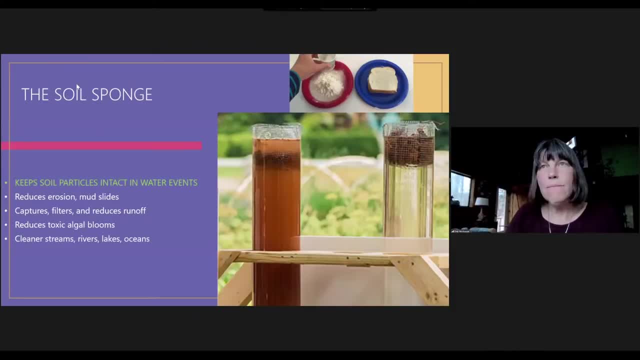 Is that it is filtering Anything that's going through, It's holding it together. It's also biologically breaking down anything that shouldn't be in the water system And it is capturing things that might go into ponds and rivers and lakes, Etc. 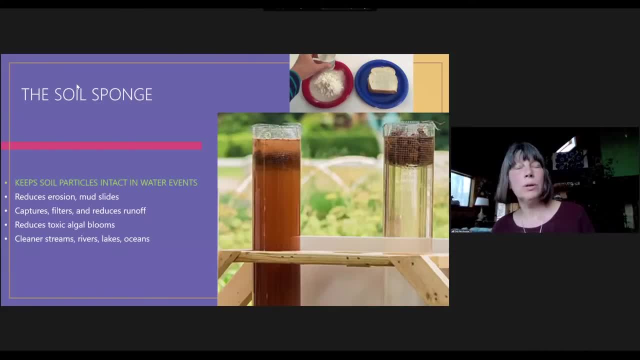 And what we know is that when there is too much manure or too much fertilizer used, We get these dead zones. I don't know those of you who have flown recently. When you look down Over an agricultural landscape, The ponds and lakes are often bright green or bright turquoise. 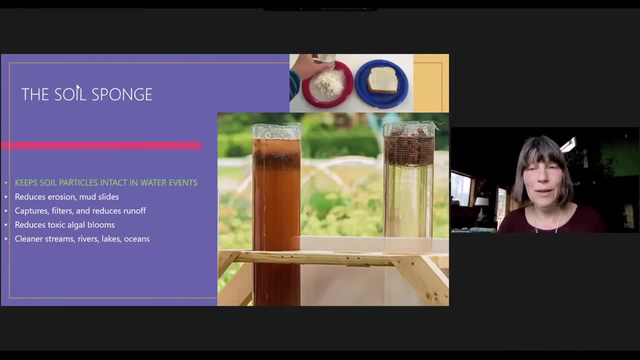 It's kind of pretty from the air But it's really not a good thing. Those algal blooms in ponds and lakes And in small streams, Those are toxic to fish, They are toxic to humans. They are causing things like ALS. 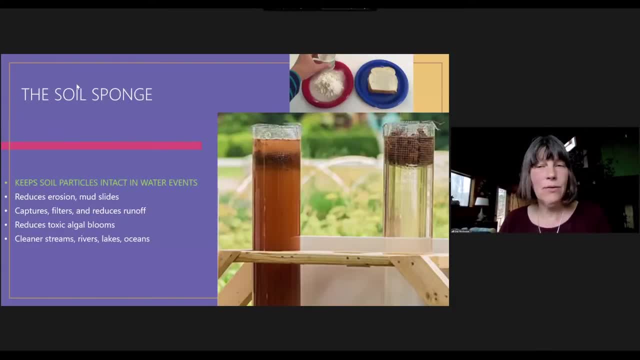 And Parkinson's and Alzheimer's And also very acute illness. So when a dog swims in a lake that is bright green With that kind of toxic algae- Not all algae are toxic, But particular ones- They can die very quickly from that- 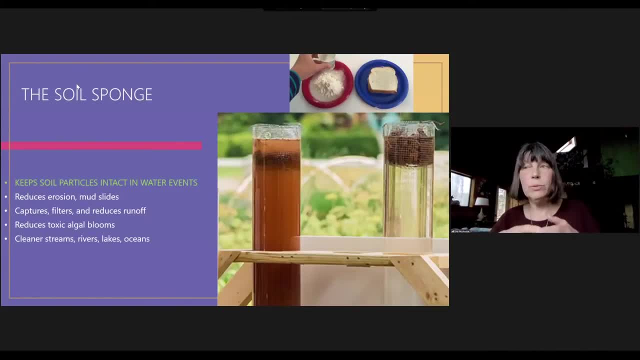 So when we are also seeing that those algal blooms And those dead zones moving out into the ocean From where big rivers empty out into the ocean, When the big rivers have had unhealthy soil And a lot of fertilizer use along the edges, 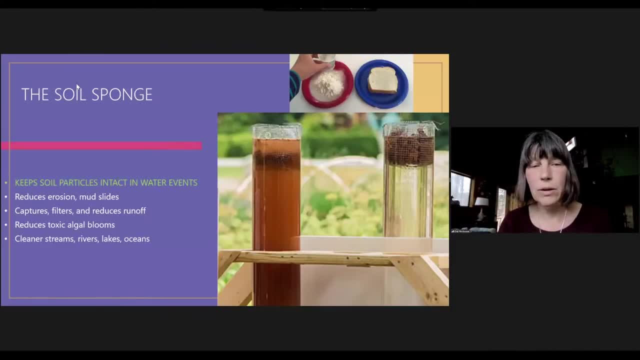 So rivers that go through big agricultural areas That are not practicing soil health. But if we practice soil health principles, You will find that the rivers and streams And everything gets cleaner And people will be healthier long term As well as, of course, all of the life. 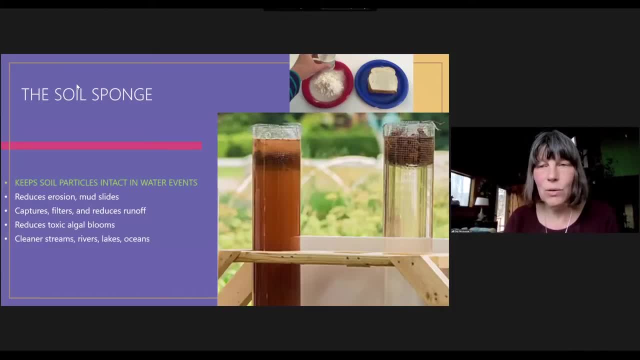 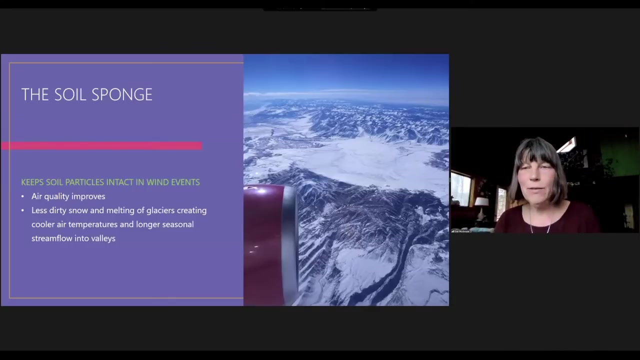 That lives in those waterways, So all of the fish, All of the insects, All of the animals that drink from that. Okay, So then that is the water. But what about air? As we said, If you pick up that plate of flour and blow on it? 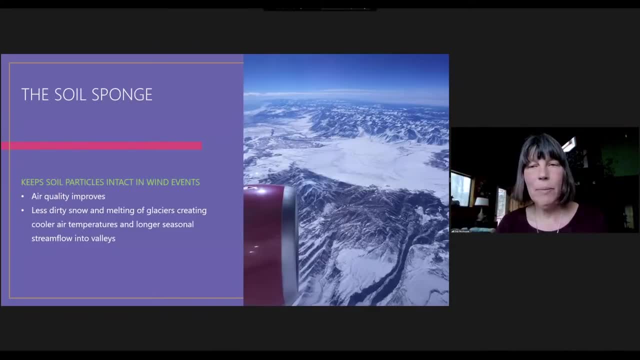 That soil is going to blow all across the landscape, And airborne soil is a huge problem. One of the things is that it lands on snow fields, Like on glaciers on top of mountains, Which darkens the snow And means that the sun can melt the snow much faster. 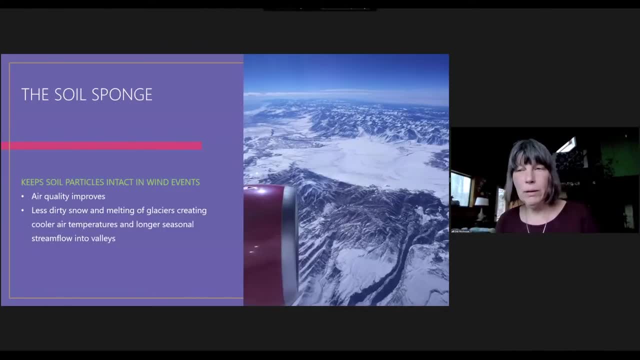 And what you get is a very quick melt And you don't get that long seasonal stream float down into the valleys Where people are typically trying to grow food Or need their wells and rivers running, So that airborne soil is very problematic In terms of climate change in that way. 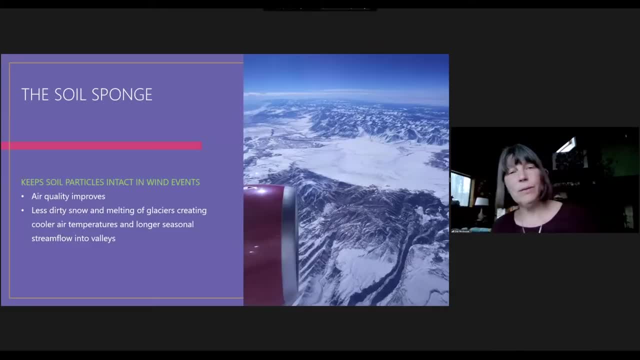 But the other thing with airborne soil Is that it causes lots of respiratory problems For humans and animals And everything that lives, And it also can carry the chemicals that are used in farming And antibiotic resistant bacteria from feedlots et cetera. 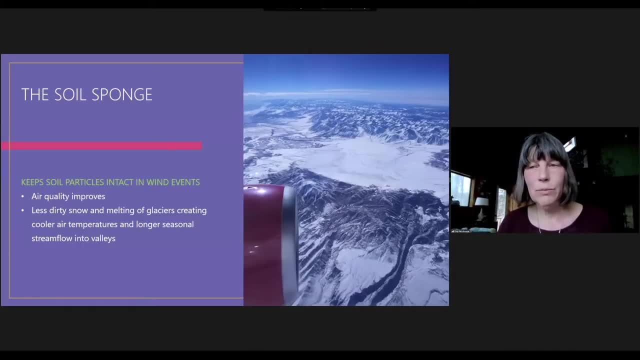 So we really don't want that soil to go in the air, And the soil sponge keeps those soil particles intact, Even when the wind blows. So having plant cover on top of the soil is part of that intactness, But it's the soil itself that has that structural integrity. 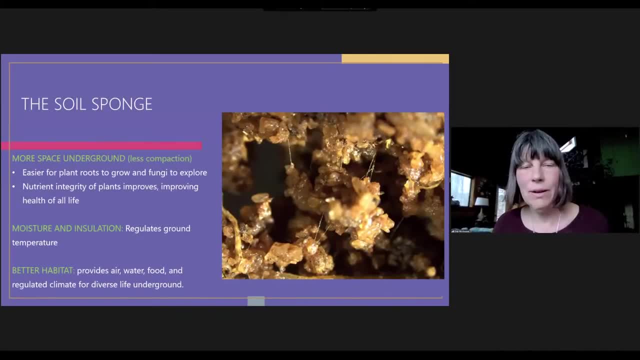 So the other thing is that there is more space underground, There's less compaction, So it's easier for plant roots to grow And for fungi to explore, Which helps to improve the nutrient integrity of the plants And improves the health of all of life. 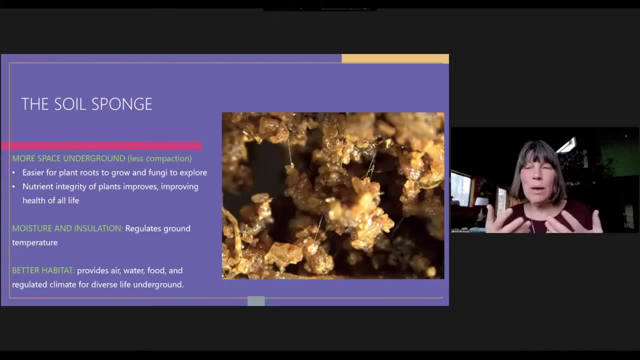 Right, Because plants photosynthesize And they make themselves, And then they make food for all of life, Both above ground and below ground. They're kickstarting the soil food web. So everything that's alive is either eating a plant Or eating something that ate a plant. 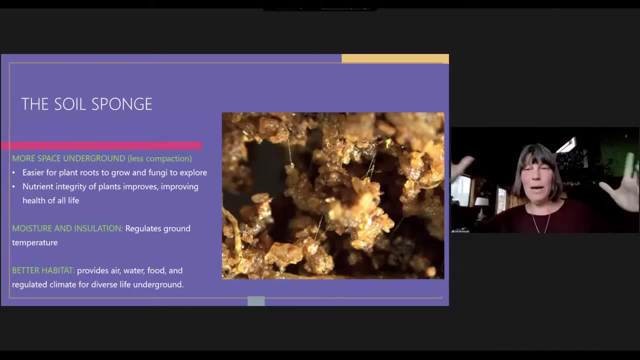 Or eating something that ate, something that ate a plant, And some of that is the plant matter that we see The roots and leaves, et cetera, And flowers and berries, But some of that is the soil, Is the exudates that go out underground. 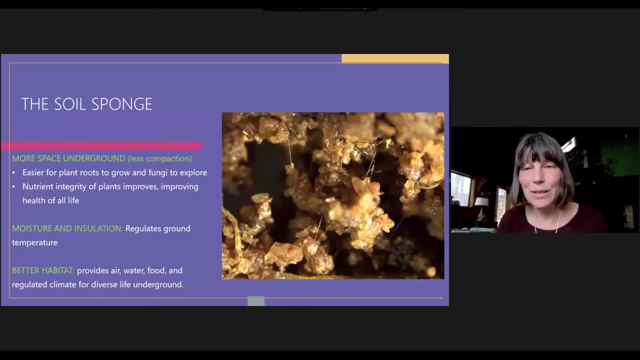 To feed things that we may not even be able to see, Like those mycorrhizal fungi That you can now see here, Because this is a microscopic picture Taken by our friend Phil Lee, Who is in Australia. That space underground also makes it possible for there to be soil moisture there. 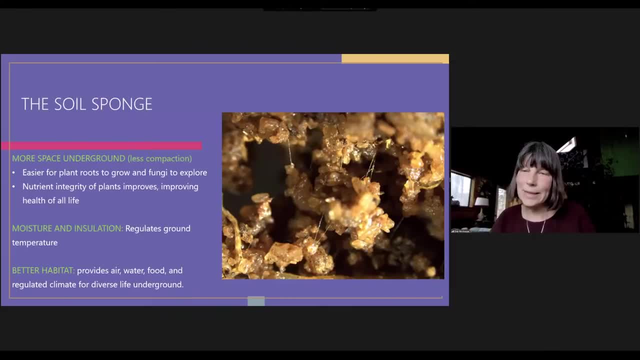 Even during a drought, And also it's like a big insulation. So if you think about insulation in the walls To keep a house cool And also to keep a house warm, It's the same thing with the soil When there is those void spaces. 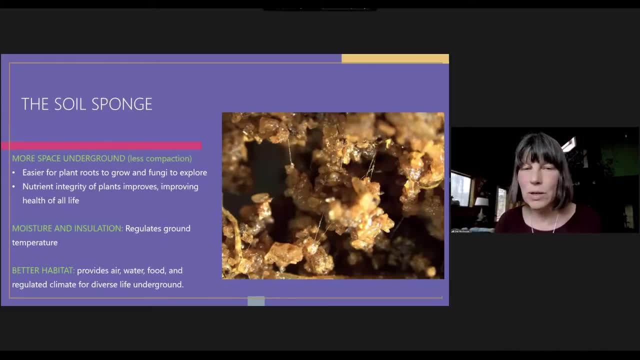 Those pores And that fluffiness of that soil sponge. It helps to regulate the ground temperature. So you have That's easier for plants And also for the life underground. So all of that together makes better habitat Right. You get air, water, food. 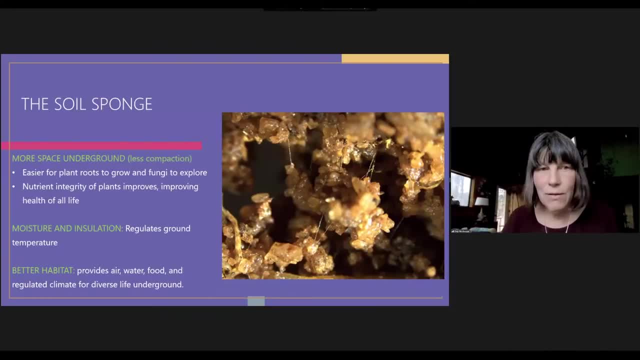 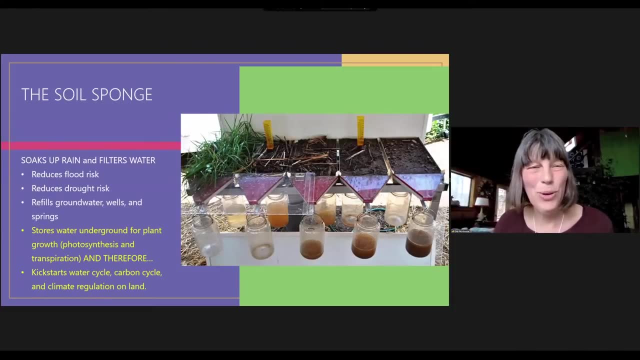 And a regulated climate For all of the diverse life underground. And my favorite part of all of this Is about it soaking up rain And filtering that water, Which reduces flood risk. It reduces the drought risk. It refills groundwater wells and springs. 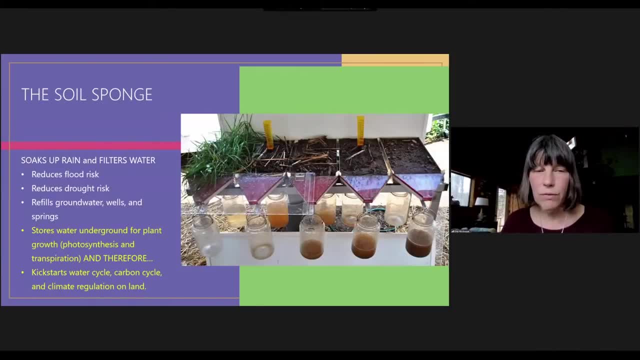 And it stores water underground For plant growth, For photosynthesis And transpiration And therefore it kick starts the water cycle, The carbon cycle And all of climate regulation on land, And we'll talk about that in a minute, About how having water for plants. 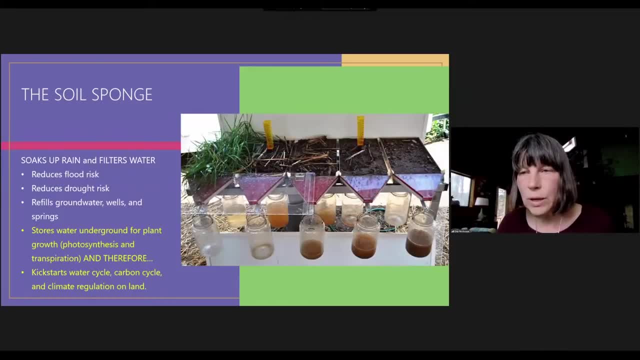 Regulates the climate, But I just wanted to take note Of this picture for a moment, Because this is something called- Oh, I'm forgetting what it's called. It's called a rainfall simulator And in the United States, The soil health team. 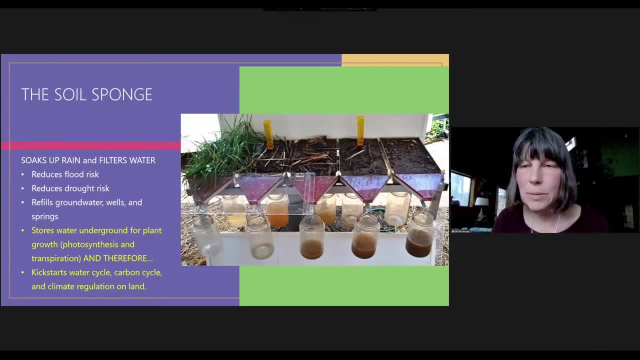 Of our US Department of agriculture Has been going around And showing this to farmers As a way Of helping them understand The benefits of soil health. So these are five pans That they're like a cookie cutter. They're open on the bottom. 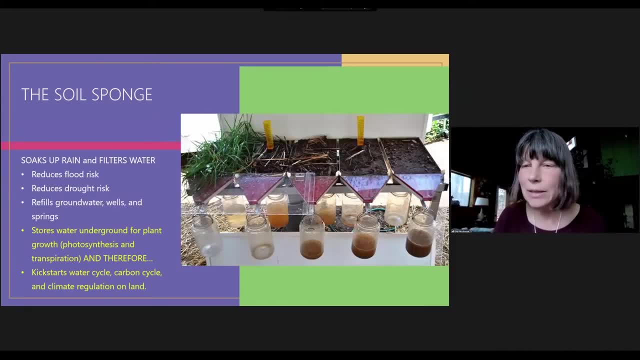 So you press them down And get a soil sample That is intact, And then there's a little screen on the bottom So the soil doesn't fall out, And then they have like a shower head That goes across the top That rains on all of this. 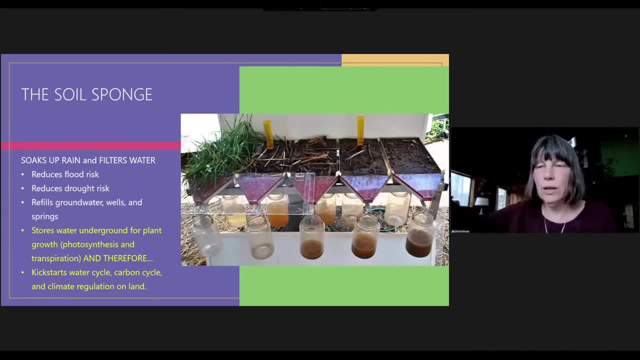 So we've put about three or four inches of rain On three or four inches of soil here, So quite a lot of rain For that small amount of soil. These five soil samples Are all from the same farm. They are all the same soil type. 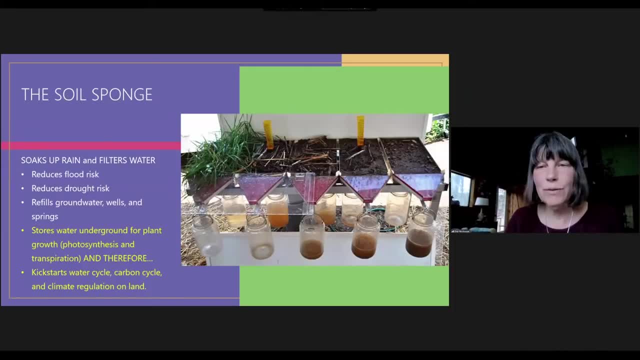 So the same ratio Of sand, silt and clay. You may have heard That a soil's ability to absorb water Is determined By the ratio Of sand particles, Silt particles And clay particles By the particle size. 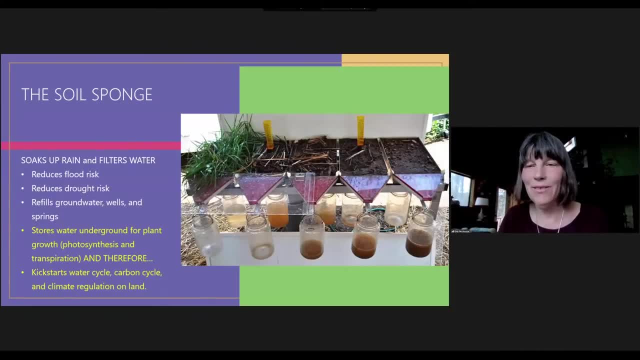 Onto the sand, It sinks in really quickly. If you poured it onto clay It would sink in slowly, But in fact Any type of soil, Any ratio of sand, silt and clay Can be improved By using soil health principles. 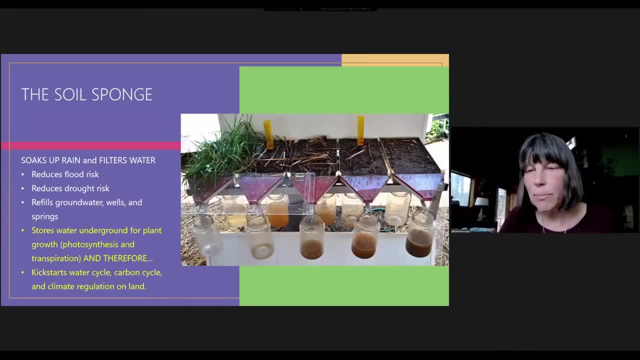 And if you look at the jars underneath On the far right, Those jars in the back, No water has gotten down Three inches into the soil And it's taken all that soil with it, Whereas if you look On the far left, 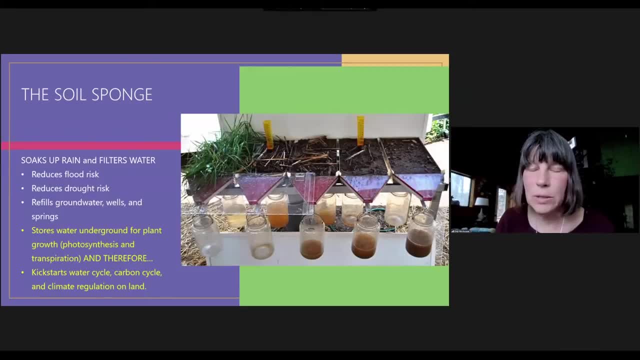 Where all the soil health principles Are being used. Where there's not, The soil is not being disturbed, There's living roots and plants, There's diversity, Etc. And not using biocides And not using fertilizers. You see all the water has sunk in. 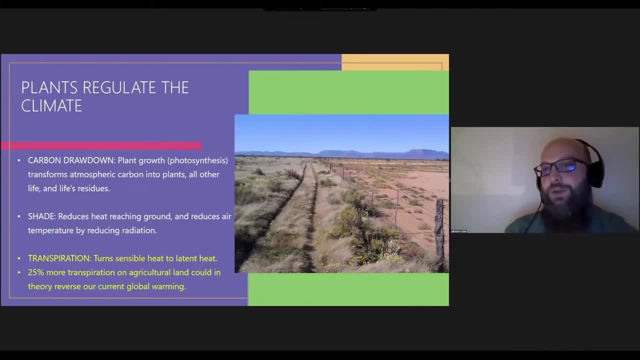 And nothing has run off. I just wanted, As you had asked, To let you know That you've got about three or four minutes left. Okay, I've actually got a timer going myself too, Thank you, So let's just talk quickly. 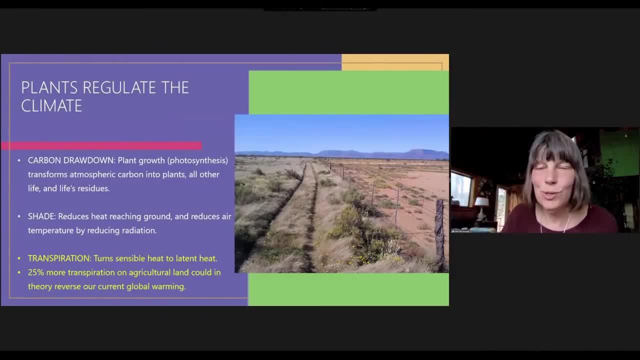 About how plants regulate the climate, Because it's not just plants themselves, It's plants that have their feet In a sponge. So if plants can transpire water, Then they And they can photosynthesize. When it's regulated And it's a. 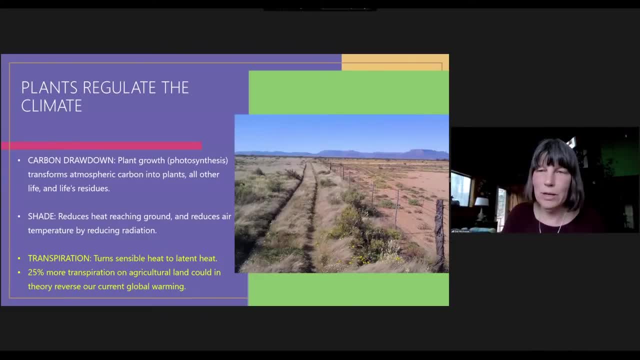 It's a beneficial cycle Because plants grow the sponge And plants benefit from the sponge, So it's a very symbiotic relationship. So the first one That you've probably heard about Is that plant growth, Or photosynthesis, Takes atmospheric carbon. 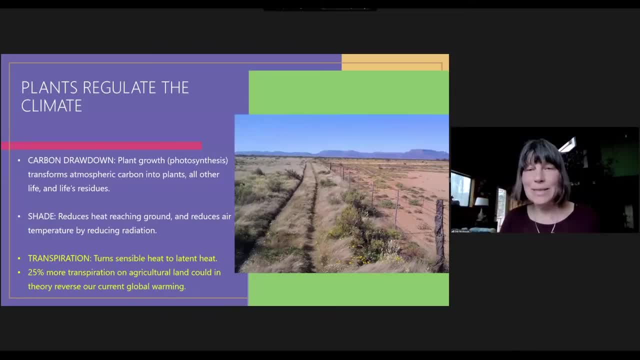 CO2.. Same carbon we're worried about with climate change And turns it into themselves, But through that, And life's residues, So like soil, organic matter. So we can think of that As like living the dead And the very dead. 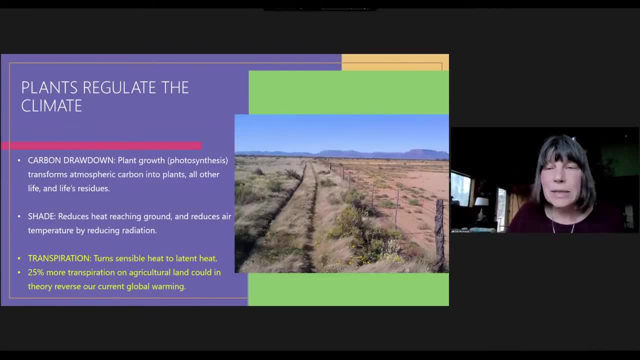 And it's all full of carbon. So drawing down carbon Into living systems Is one way that plants regulate the climate. And just remember, We need a greenhouse. We need a greenhouse effect To keep us warm enough and cool enough. Without it, we'd be in trouble. 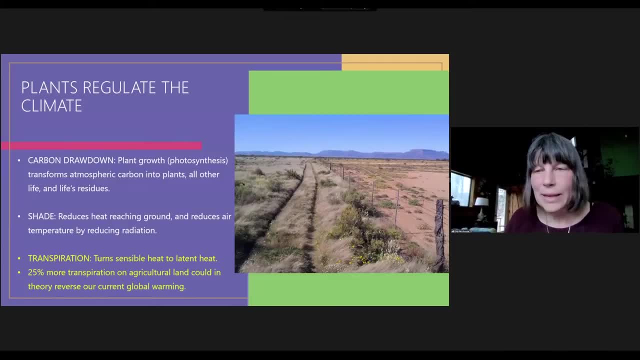 We just have a little too much. The second thing Is that plants help shade the ground, So it prevents heat from reaching the ground And it reduces the air temperature By reducing how much of that heat Is reradiating back into the ground. 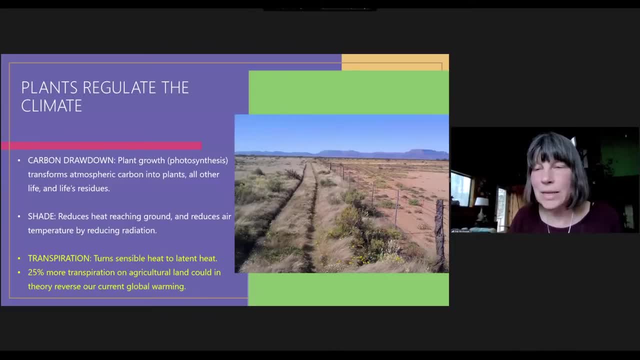 You can imagine If you were standing on the right side of this fence Versus on the left. Your feet would be hotter And probably the air above that bare soil Would be hotter as well. But the third one, That's really exciting. 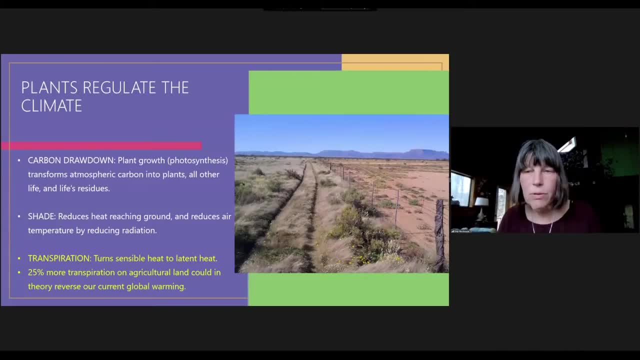 Is transpiration. They take that water Up through their feet- A little different than us- And as they're growing They sweat it out, So that water evaporates from the plants And changes from liquid water Into a gas, Into water vapor. 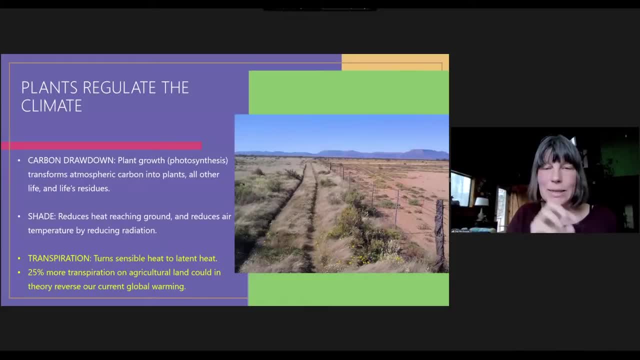 And in doing that, It takes something called sensible heat, Which is the heat we can feel, And it turns it into latent heat, Which is no longer warming the air. And so I remember, And Sophie is here today Standing under tents in India- 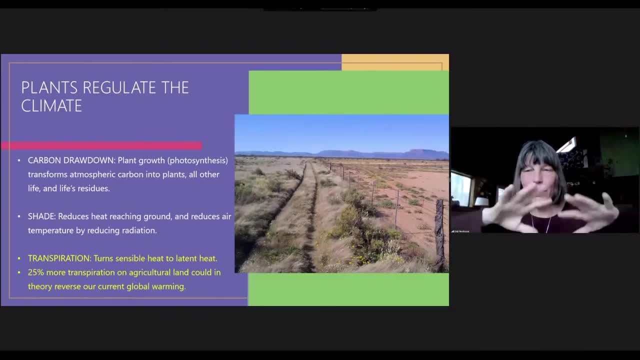 Where there were no plants, That it was hotter in the shade Than it was going, Standing out in the full sun Among those beautiful tall cover crops. That was where I really started to get this. So two of the scientists I work with, 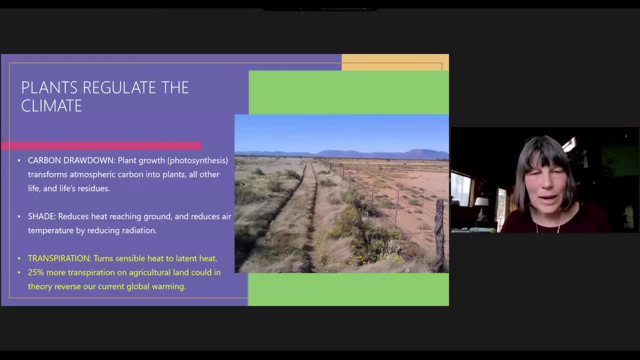 Walter Yena and John Norman Have figured out that transpiration alone Is not as important. But transpiration alone In theory Could actually reduce Reverse the global warming We've already experienced. So if we could have 25% more, 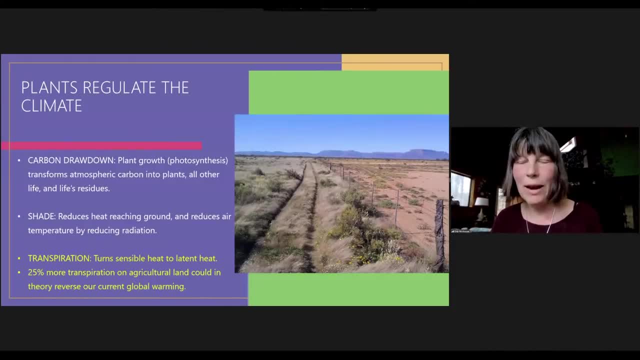 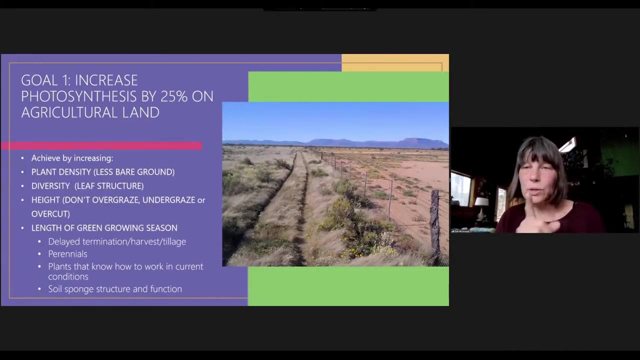 Photosynthesis and transpiration On agricultural land, That could, in theory, Reverse global warming. That's already happened. That's amazing And that's something we could do Probably in one season. Okay, So two goals here. One is to increase photosynthesis. 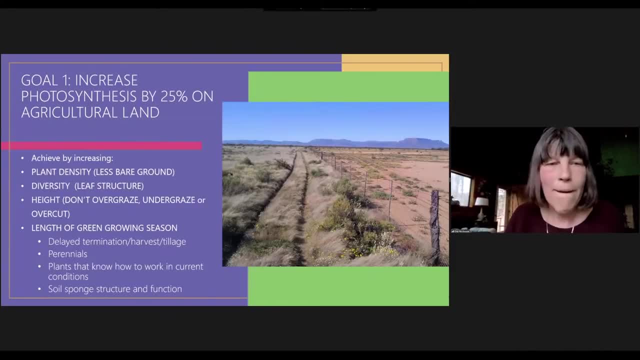 By 25% On ag land, That's worldwide. We can do this with more plant density, So less bare ground. More diversity, So more complex leaf structures, More height, Not overgrazing, Undergrazing, Overcutting. 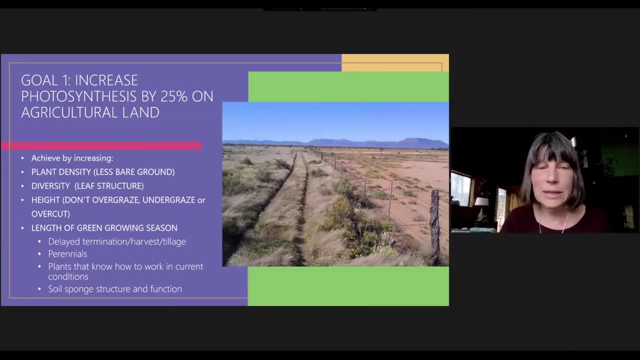 And, of course, we're not even talking about lawns here, But lawn policies, So delaying the harvest Or tillage, Having more perennials, Using plants that know how to work In current conditions, And having more soil sponge structure and function. 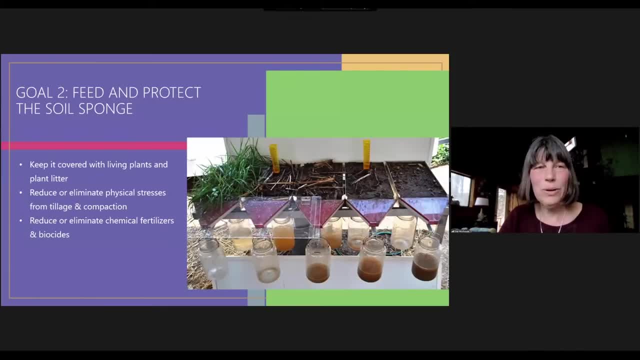 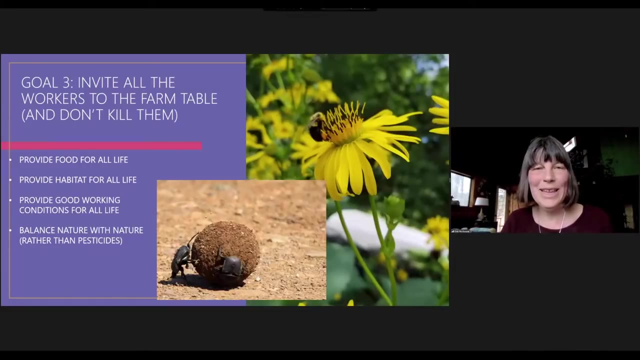 We'll lengthen that. Goal two: Feed and protect the soil sponge, Keep it covered, Reduce or eliminate stresses, And reduce or eliminate fertilizers and biocides. Goal three: Invite all the workers to the farm table And don't kill them. 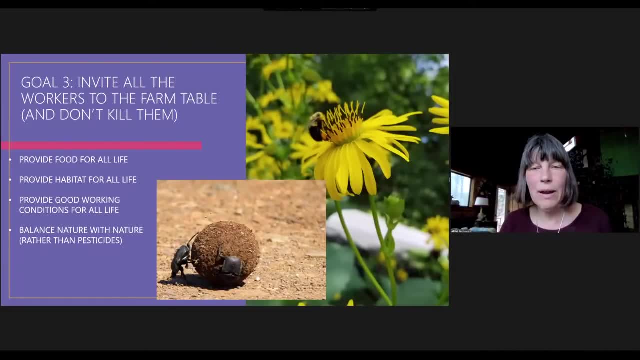 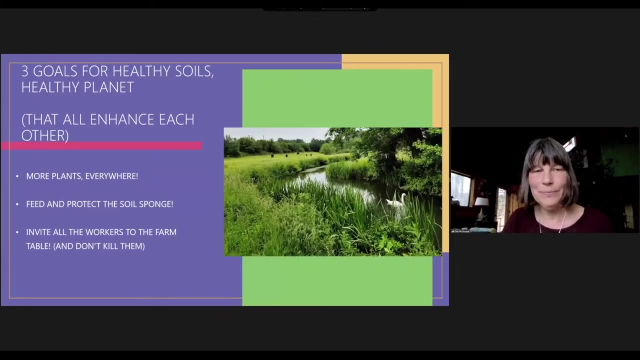 There's this huge web of stuff going on, Both underground and above ground That all makes this whole thing work. So provide food for everyone, Habitat for everyone, Good working conditions And balance nature with nature Rather than pesticides. So those are those three goals. 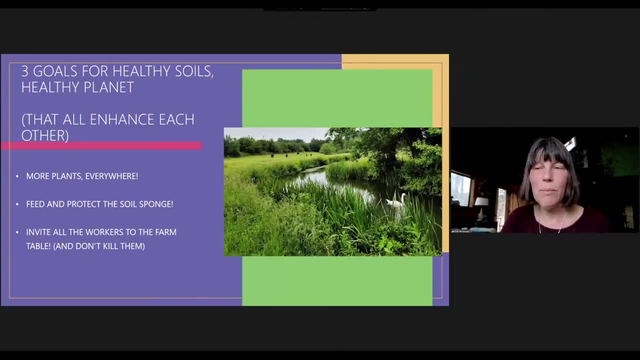 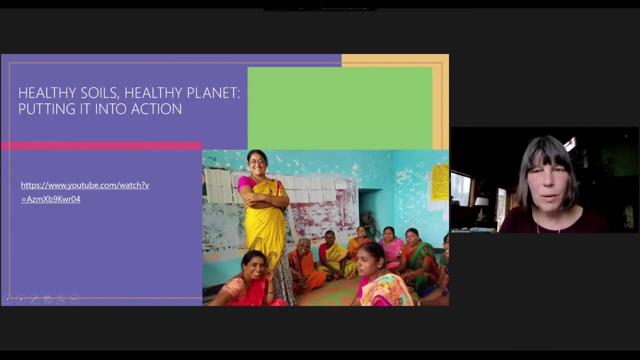 We can actually do this. We can make all of these things that we're worried about. We can address them Through healthy soil, Healthy landscapes. So I wanted Sammy. If we have two minutes, I would love to just bring up that video. 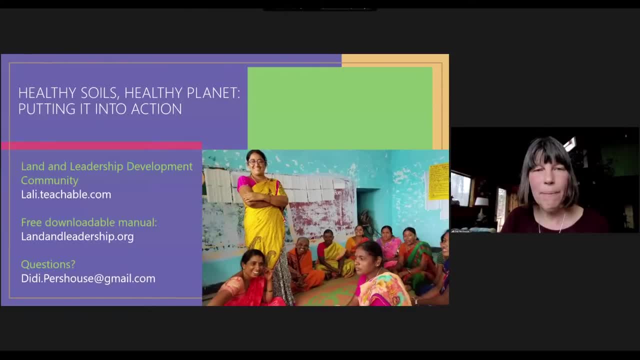 Of how this is being put into action in India, And while we're waiting for that, I'll just invite people. If you want to download the free manual Understanding soil health and watershed function. You can find that at land and leadershiporg. 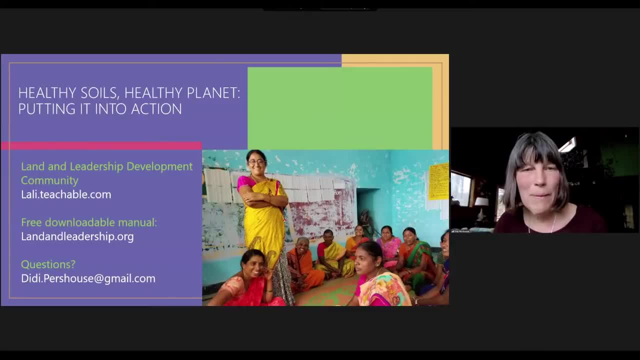 I think it's under resources And if you're interested in joining the land and leadership development community, You can read about it there Or send me an email And I will tell you more about it. If that's, I can share it. 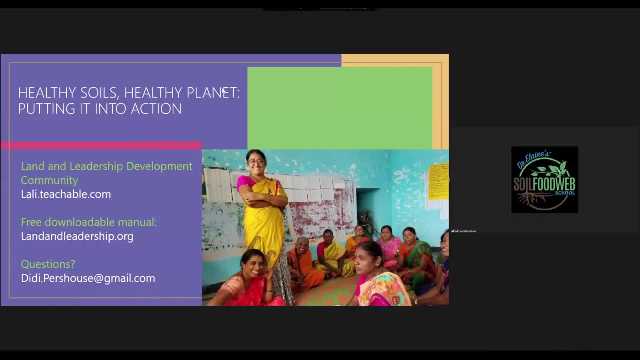 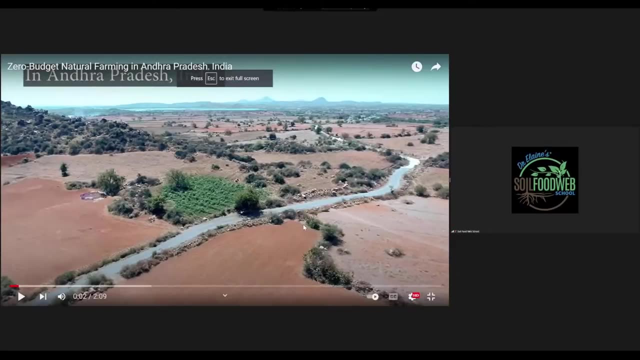 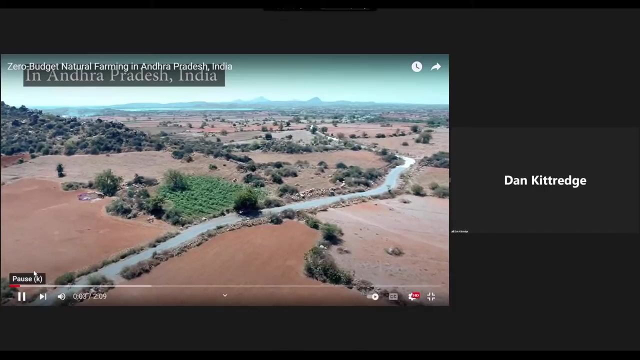 If you don't have it, My PowerPoint closed down So I'm having to restart. If you have it available, Here we go. So there's my timer, But I think Are we okay with me just going to? This is two minutes or less here. 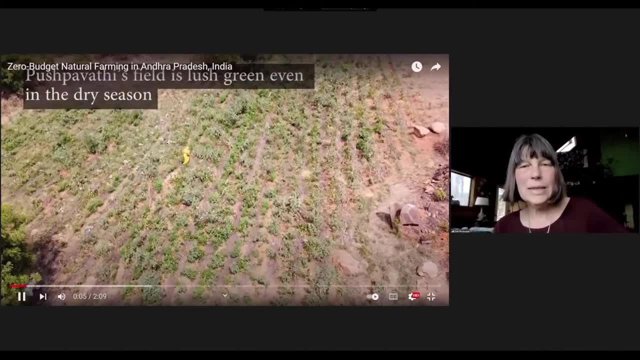 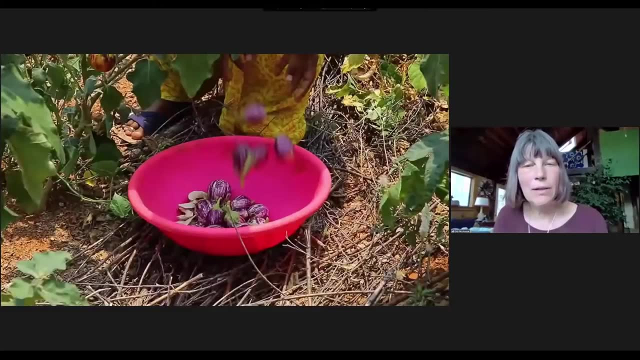 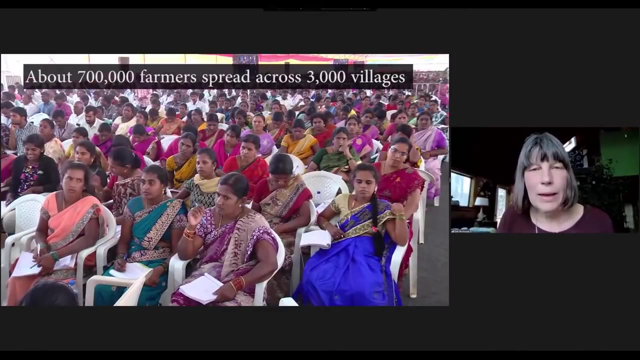 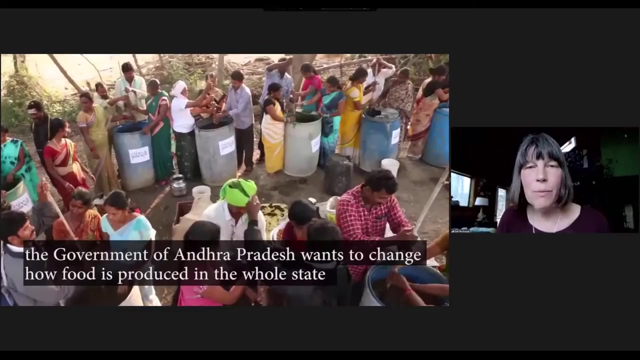 Go for it. Yes, So this is in Andhra Pradesh, India. This is this amazing project That the women's self-help economic groups Are really spearheading Of getting Thousands of farmers to adopt natural farming practices, And they are. 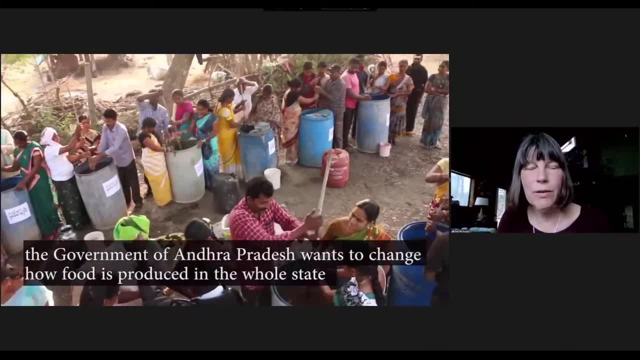 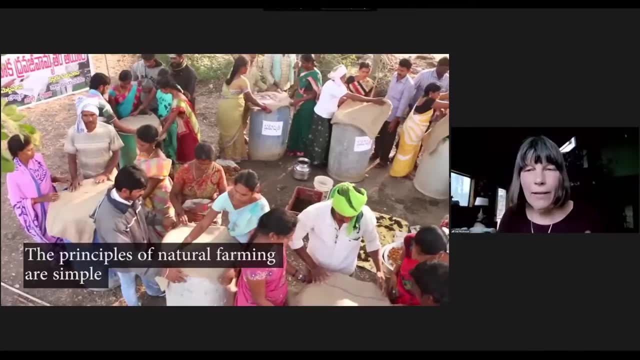 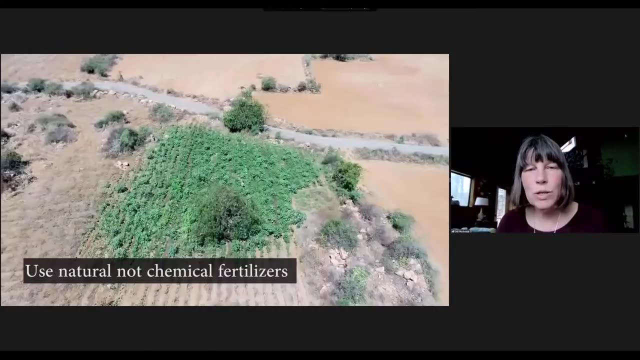 Working with the United Nations Food and agriculture organization, Which helps farmers To work together, To do research together. But what I wanted to Show you here Is just imagine When we talk about 25% more On agricultural land. 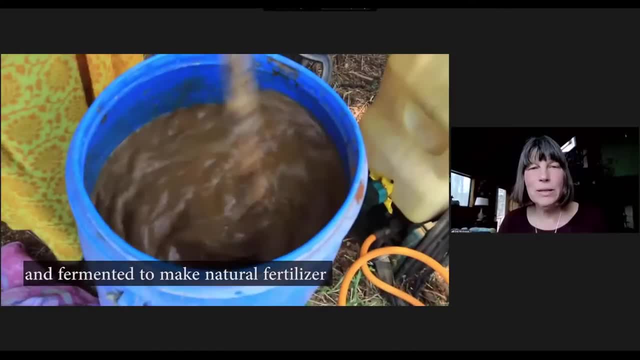 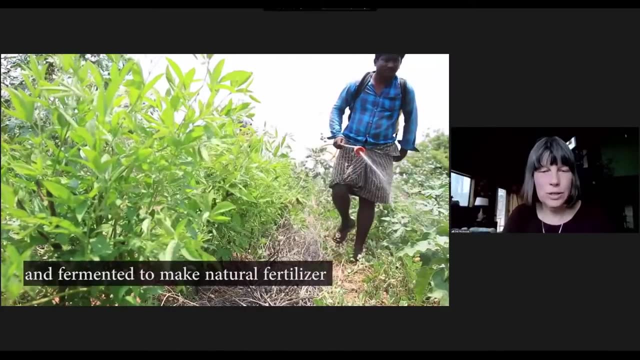 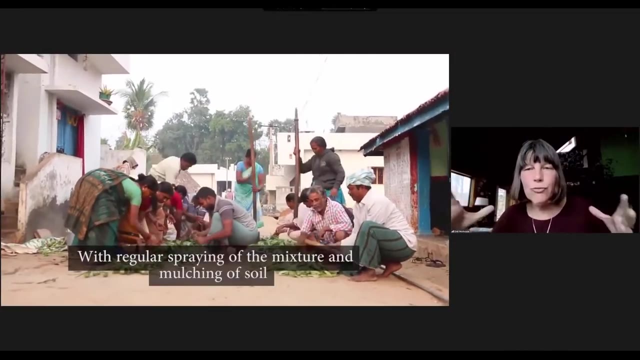 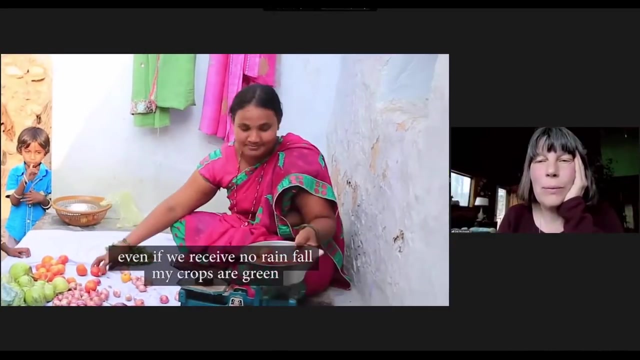 And we talk about all those effects Of building this, Of cooling, Of feeding all of life. Those drone pictures You can see Are just extraordinary: Of this green Carpet in the middle Of a big, dry, Dry area, And what they started doing. 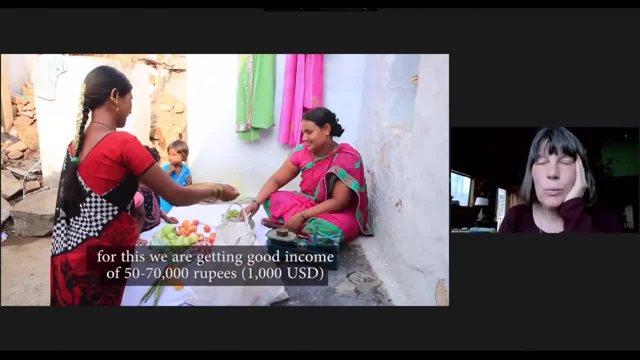 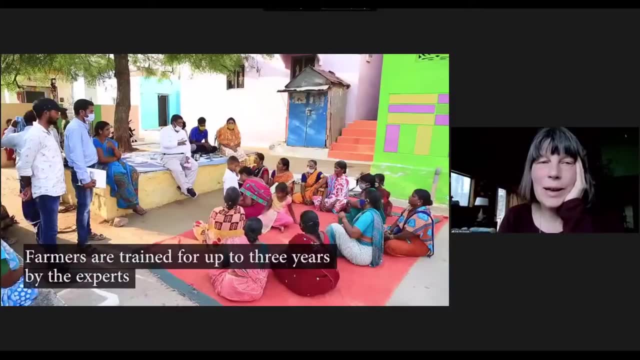 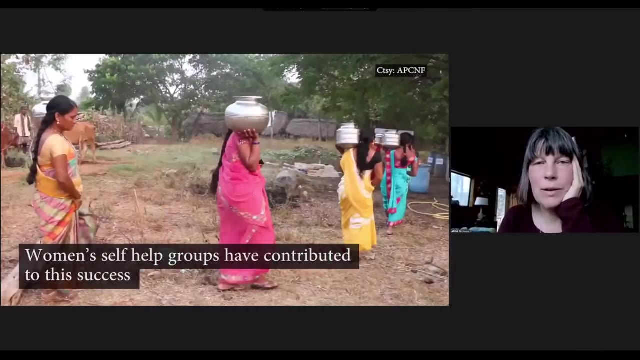 Is something called Pre monsoon dry seeding, Where they are growing Crops Before they even get the rain going, By understanding How the soil sponge works And how it can help Wake up the soil. food web Underground: How using herbal. 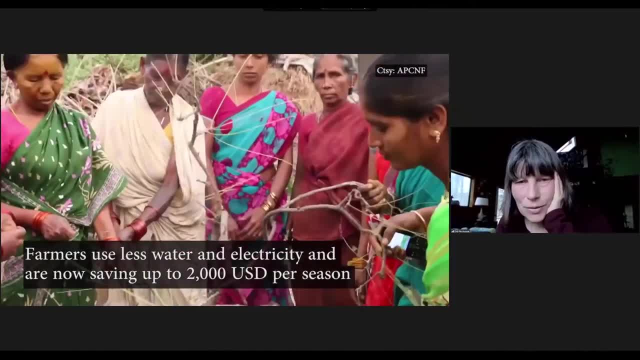 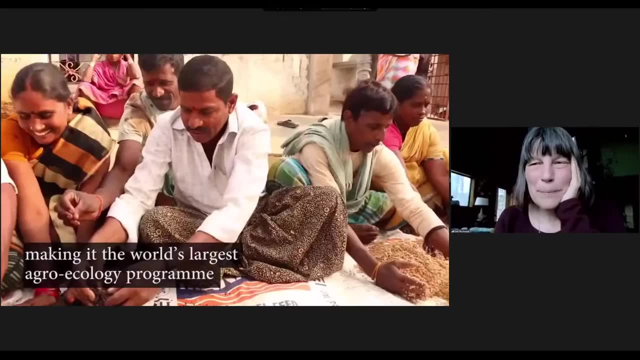 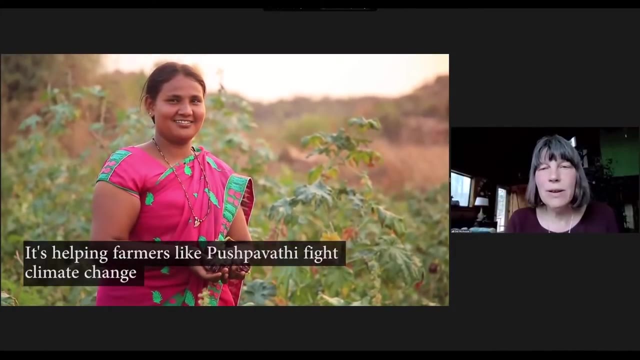 Herbal insect repellent. Here is this. I just think It is amazing. No, that is not the one. And And farmers are Not using any inputs From outside of the village, So they are everything. There is 25% more. 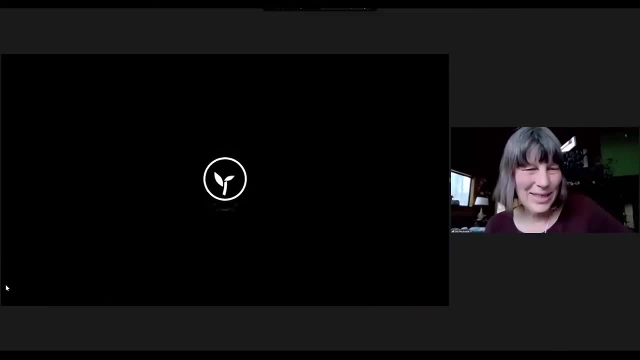 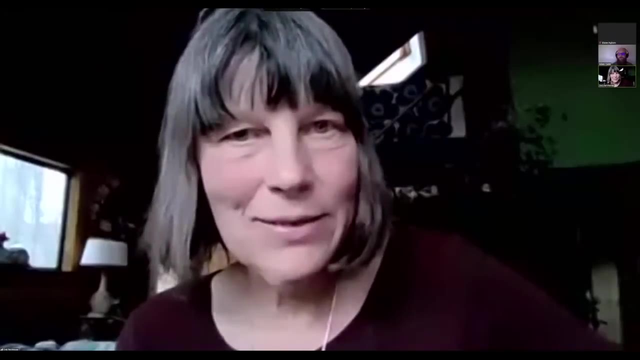 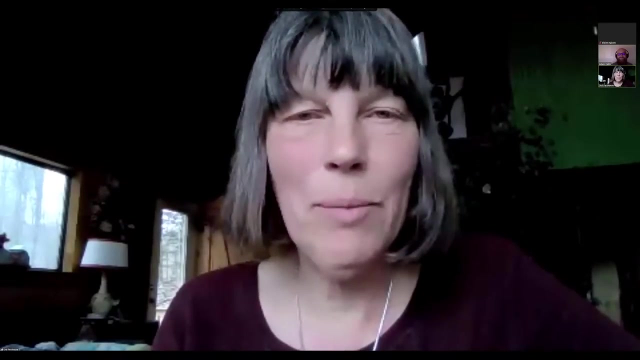 Photosynthesis And transportation. So Let me stop Share So I can see you all for a moment. That is so exciting. I just find that incredibly inspiring. I am really delighted To be working with that program To develop yet another training handbook. 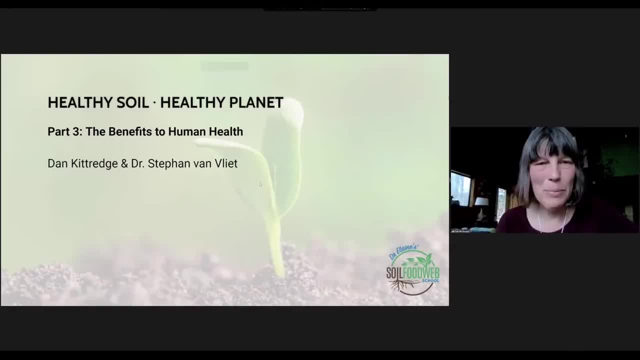 On soil and water And the soil sponge. I am happy to talk more about that During the Q&A. Thank you so much. I want to go ahead and turn over To Dan and Stefan For part three: The benefits to human health. 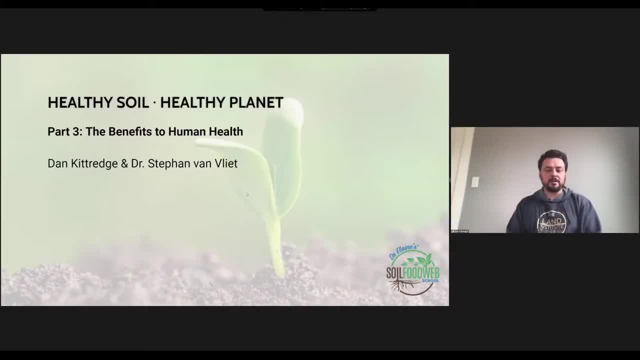 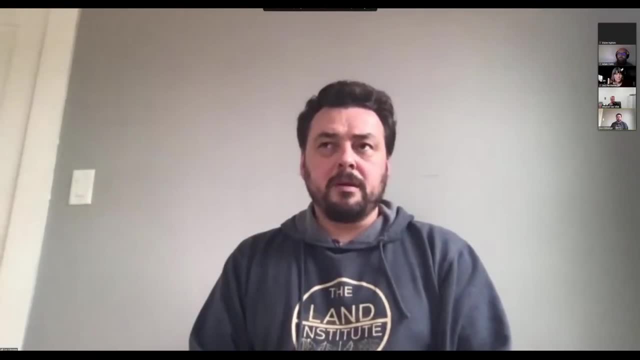 All right, Great, I think you can turn the slides off for a minute, If you want, at least. But my name is Dan. The BFA has been doing What we call principles of biological systems course Working with growers for the past ten years. 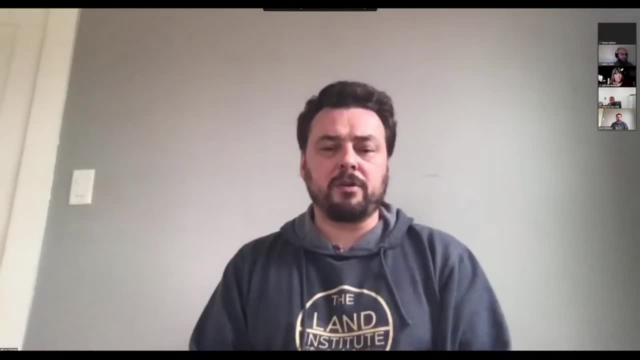 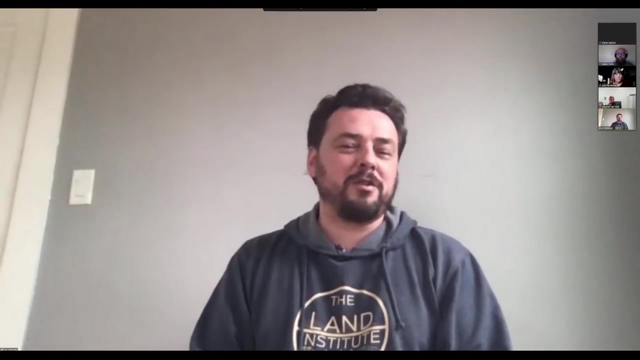 Helping them understand The foundational dynamics For life to function. The whole food chain Food web, To Elaine's point, And foundational to it, of course, Is the microbes. The bottom of the food chain Food web, The center of the food web, 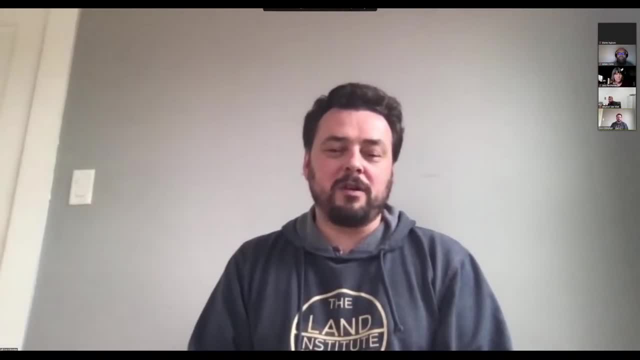 How shall we The center of the evolutionary biological Pathway? Really, it is the microbes that evolve the plants And evolve the animals In micro outcomes And contribute to growth. ALONE Yani, I think I'm not sure if people appreciate what she has been doing. 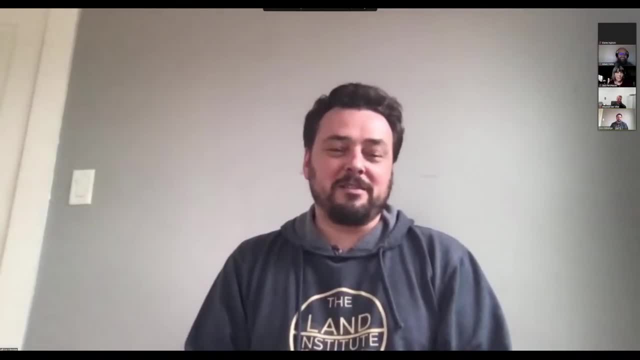 For how many years? But 40 years ago or so, when she said Maybe fungus in the soil lor not all bad And people said no, Now people know about this stuff. She has really been a leader in this Total space. 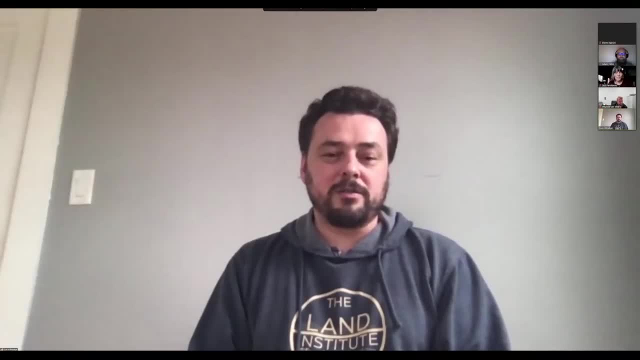 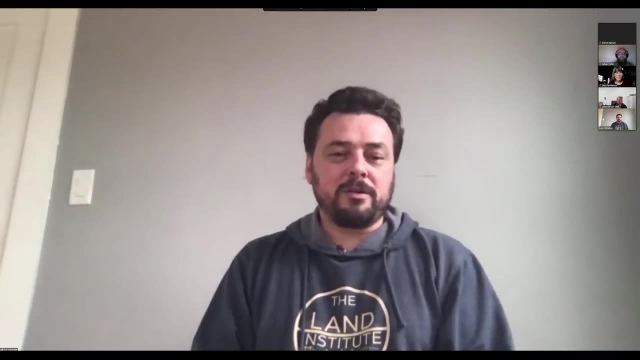 to view that video. it's really so impressive what's being done in the global community with these principles and insights. We think here in North America that we're, you know or not, everyone's here obviously from North America, but we really are, you know. on the 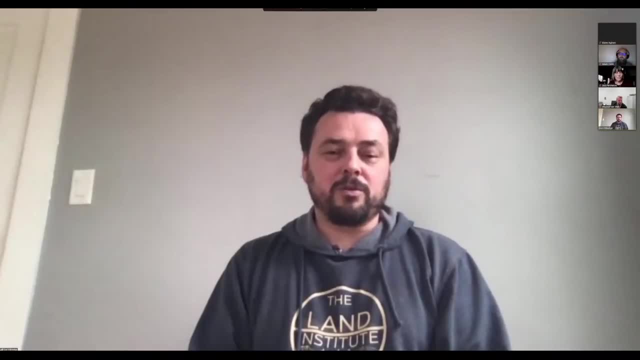 cutting edge, but we have a lot to learn from other parts of the world. So, yeah, it's great. My part, the VFA's part, you know, formally we're an organization, a nonprofit, focusing on food quality, and we're saying the point where you know we can actually have some. 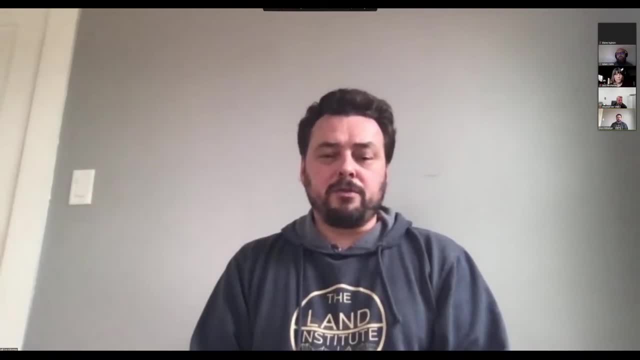 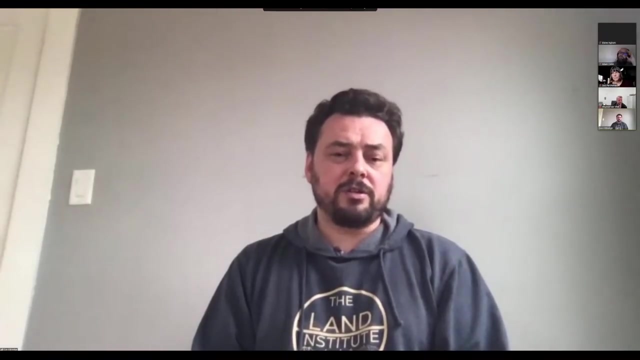 really profound effect is if we choose the food we eat every day based on its inherent quality. we understand that connects to soil health, to biological system function, to farm viability, to environmental health, human health. Most people are driven by their foundational 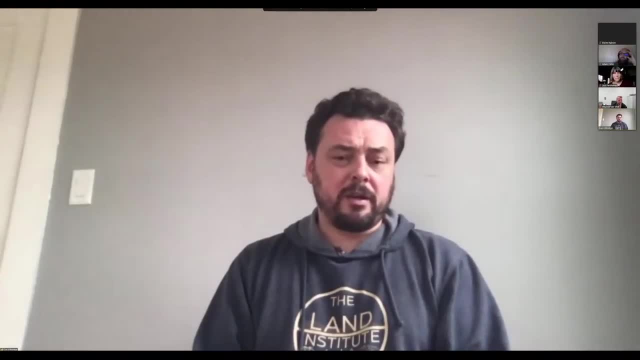 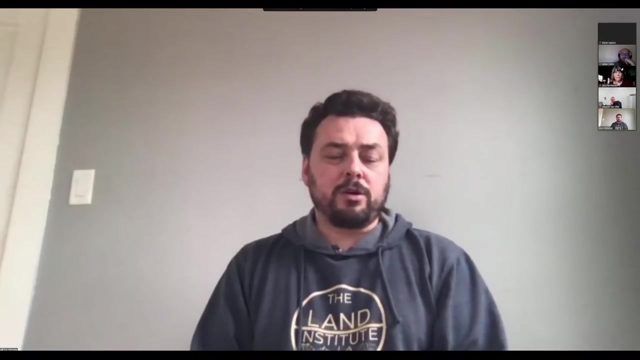 you know, dynamics of life and their health and the health of their children, I think for most people is actually more visceral and helping the environment. and so the question is for us: how can we engage the science, this understanding, um, and money and power and the world as it currently exists? so we, as an organization, 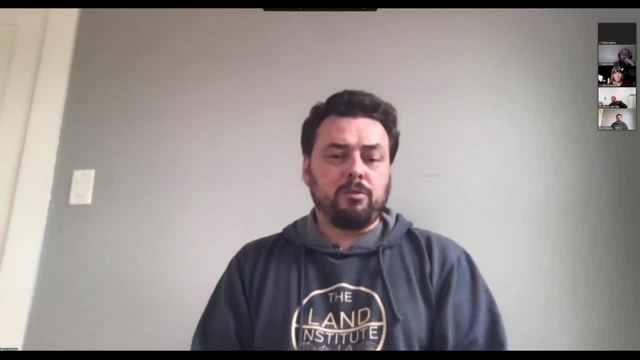 have been working for the past uh, five years on this really more proactive, you know, question of nutrient density: i think it's term that people have heard it. we've started to popularize it around 10 years ago or so, um, and the concept was that there's a variation in nutrient levels in 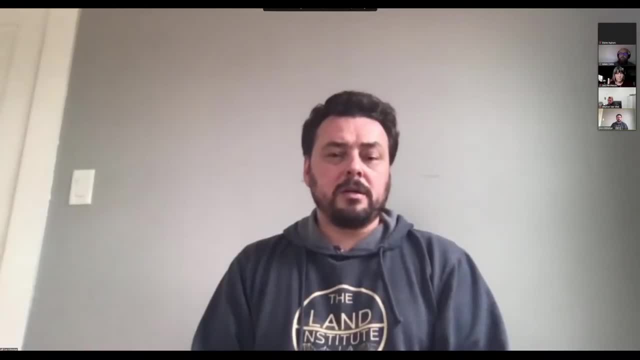 food. that's a foundational, foundational point. um, if you eat a tomato off the shelf from the grocery store in january, if you're living in the northern hemisphere, or a tomato off the vine from the field in, you know, august, again in the northern hemisphere, you know the variation and that's your. 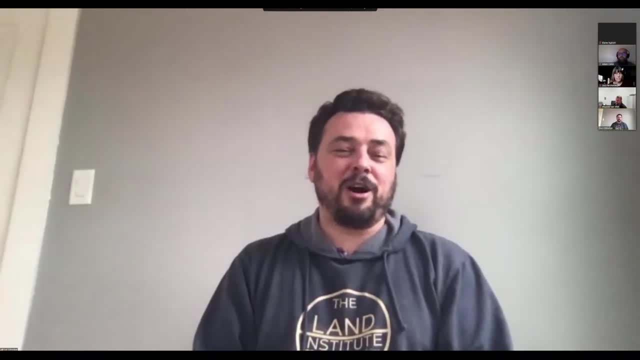 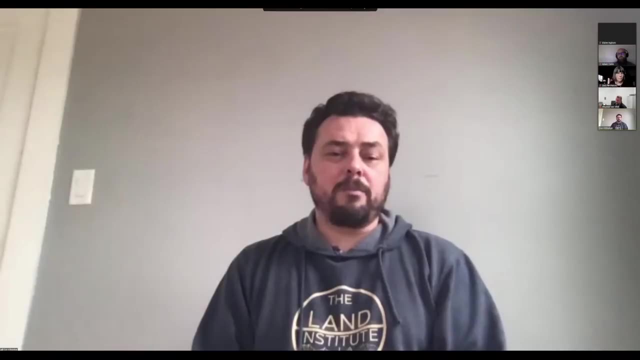 inbuilt nutrient sensor sensing hardware, your nose and your tongue and your body telling you this is different. um, so what we've said is if we could help people choose the variation in food that they are eating, you know, obviously help them grow it, but for those who aren't growing everything all the time with money, which actually is a power in the world- 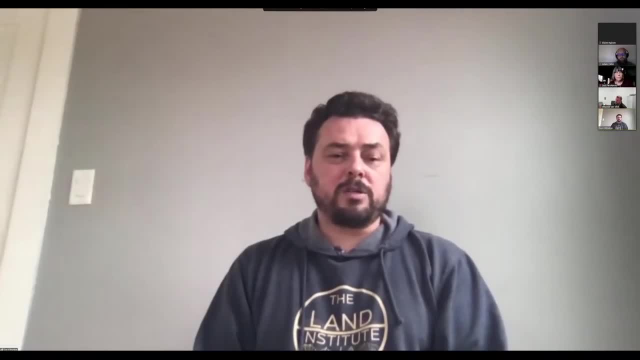 choose that what's better for them, we're actually facilitating what's better for the environment. that's a really powerful vector, because x number of billion hectares on the planet are managed through egg culture, and if we can inspire, support growers through better economic viability by choosing what they're producing on top of all the other things. 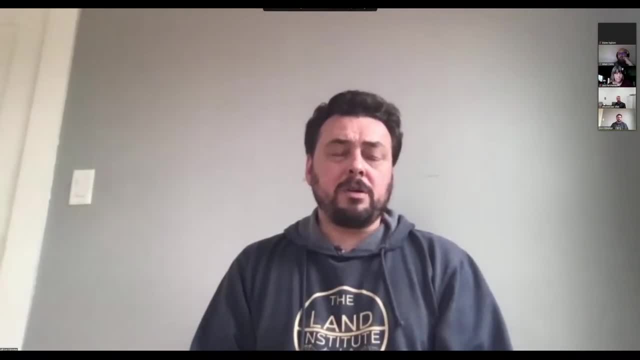 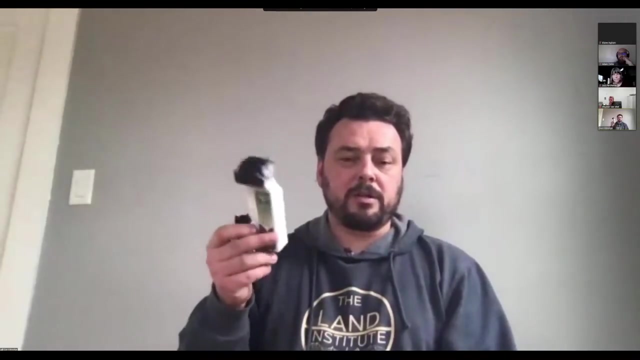 um, that can really help speed the process up. so we started five years ago- um, well 2016- with a concept that we need to identify variation, we need to connect it to the management practices and we need to build the ability to sense, to test in real time. um, we've got a, you know, a little meter. that's. 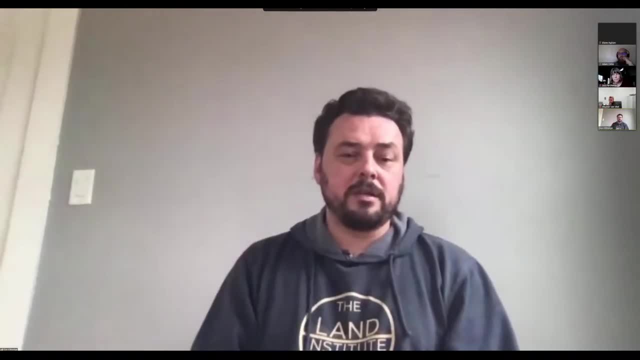 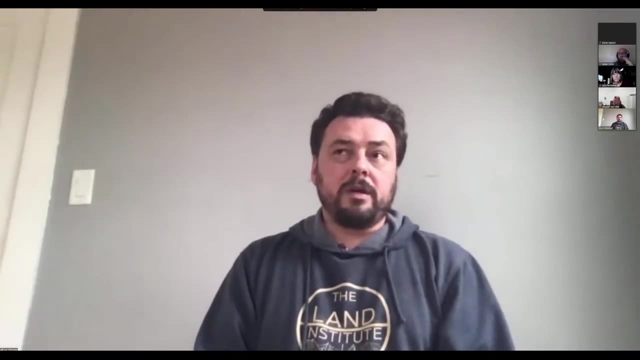 basically as a prototype. it functions for flushing light at things- wheat, berries or zucchini, squash or lettuce heads and getting readings um. we started in 2017 this year, so we're just kind of working with the lab and we tested um carrots and spinach we looked at. 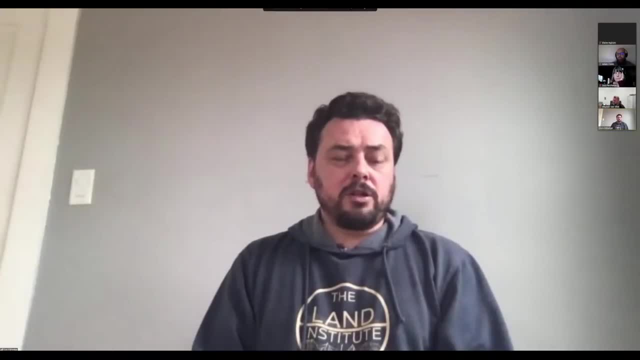 you know samples from grocery stores and farmers, markets and farms across the us um organic, not organic, etc. and we found variations. we were just looking at elements in a couple of compounds, things like copper and zinc and sulfur and phosphorus, and you know antioxidants and polyphenols and 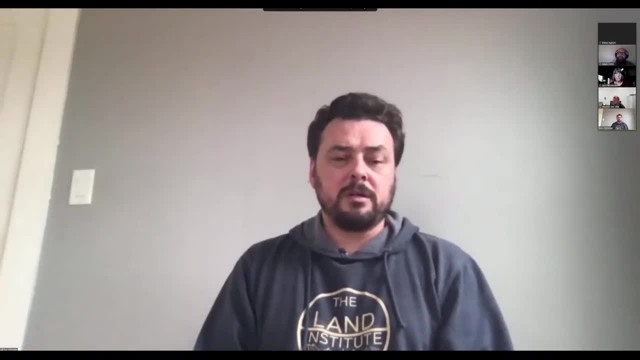 the variations were three to one to fifteen to one in minerals, which is massive, right, this leaf of has as much iron in it as those 15 inches of spinach. And then we looked at the compounds, the flavor, the health-giving compounds, polyphenols, antioxidants. 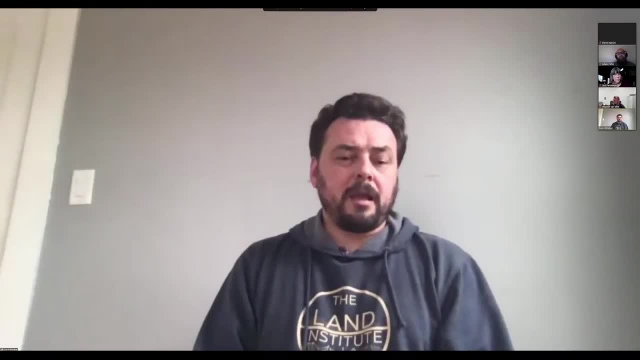 it was more like 75 to one. In 2019, we set up a second lab at Chico State and we started looking at a few more crops and also looking at the soil and the management practices and documented the practice soil type. 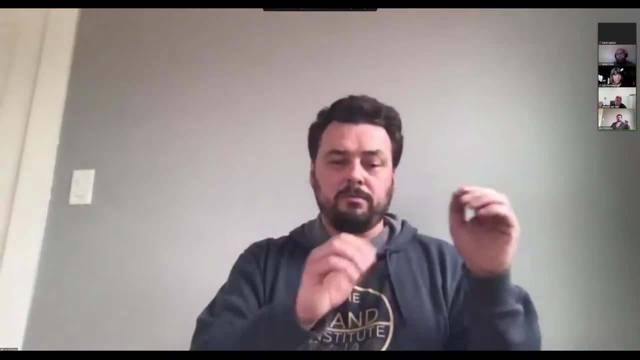 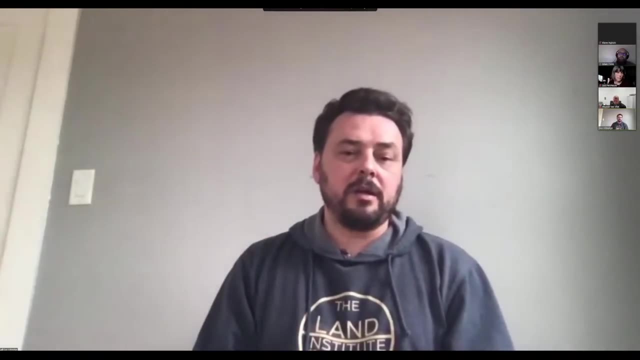 fertility program, tillage, inoculants, seed planting date, cover crops and the soil, so organic matter and minerals and phylogenetic activity, and overlay that on nutrient levels. In 2020, we had another lab in France. 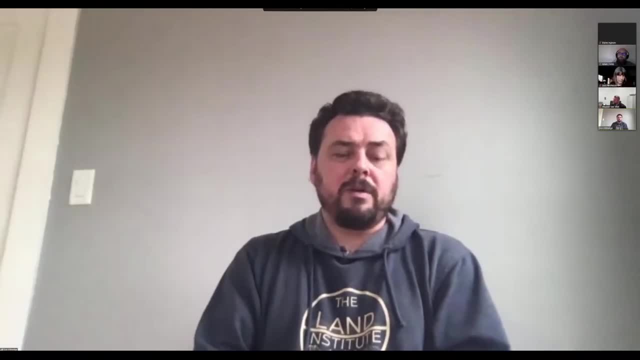 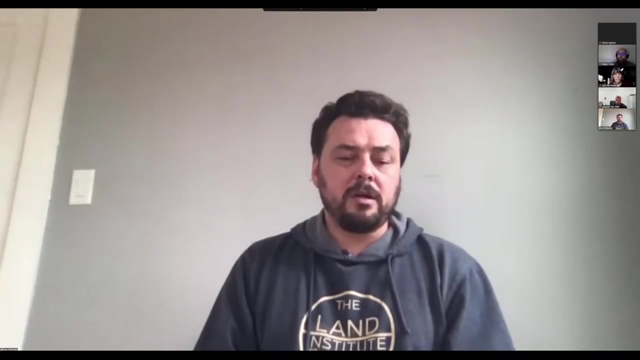 up to over 20 crops and we basically showed some really nice connections between management practices, soil health metrics like soil carbon and nutrient levels. So I'm gonna use the small time I have remaining to just run through a couple slides on that and then hand it over to Stefan. 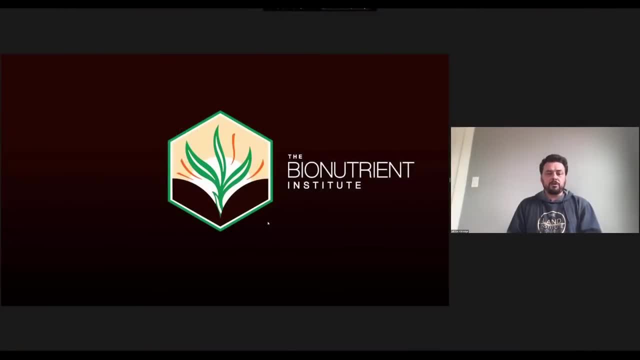 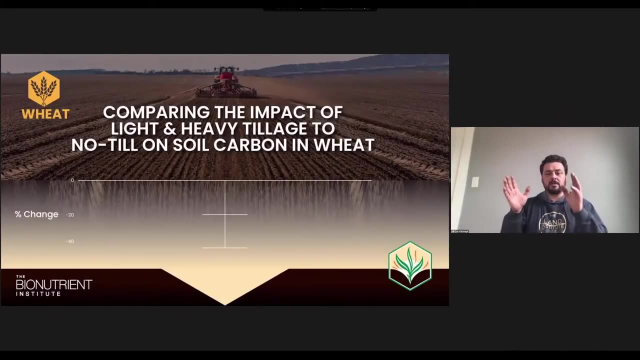 We have done basically this variation thing for roots, leaves, fruits and grains, and now we're looking to define nutrient density to be able to say: this is better, this is decent, this is not so good. So yeah, move it forward here. 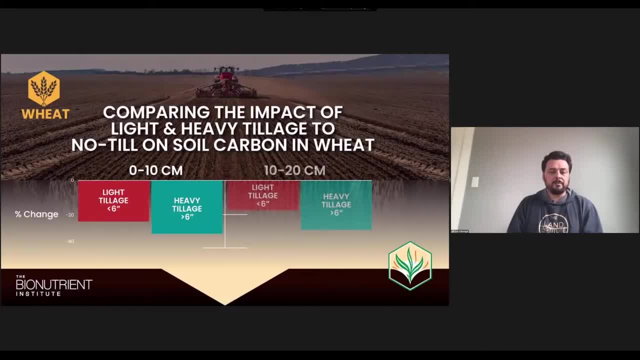 I think just forward on the yeah and keep going. So this is basically looking at tillage as one practice. Light tillage is less than six inches, Heavy tillage is more than six, And this is the effect of change on wheat in organic matter based on tillage. 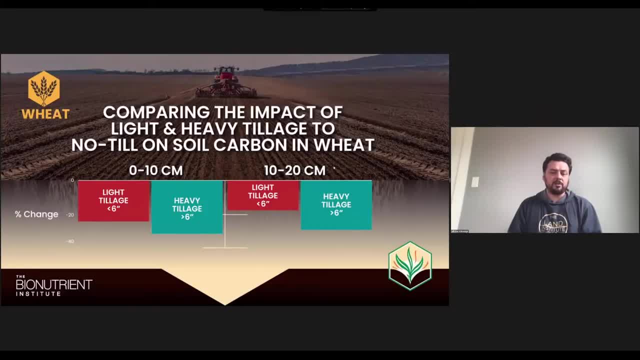 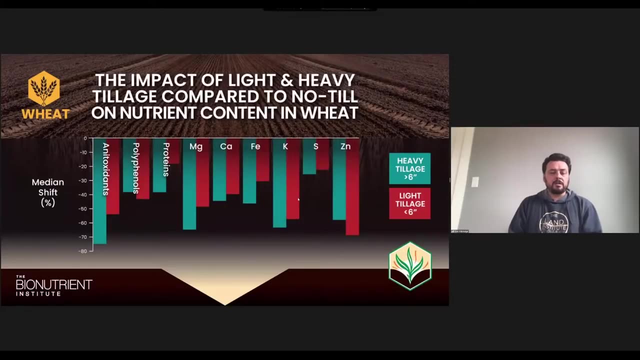 So look at that, It's obviously. this is. you know, average farm size was 3,000 acres, two continents, 13 US states, I think. Move it forward, Yep, proceed forward. So this is the connection between tillage. 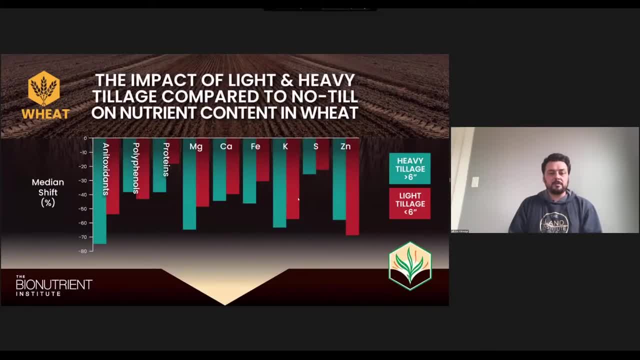 and nutrient levels decreases 20,, 30,, 40,, 50,, 60, 70%. You know, when you engage in that process of destroying the soil functionally, what you affect is a decrease in the nutrient levels in the food itself. 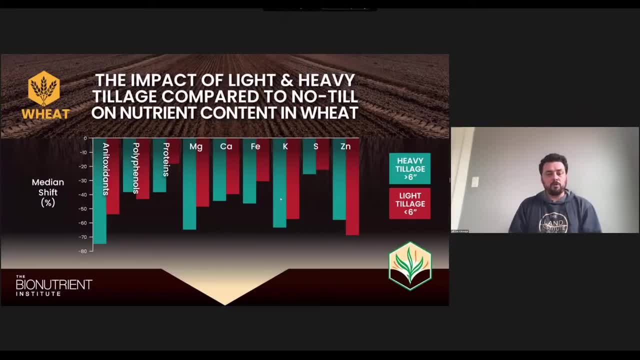 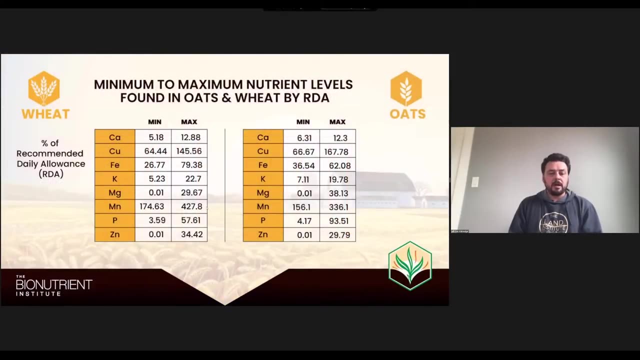 This is just one crop out of you know more than 20 we've done, but on scale and very good data. you know sample size, et cetera. Okay, keep going. This is the nutrient variations as defined by percent of USRDA. 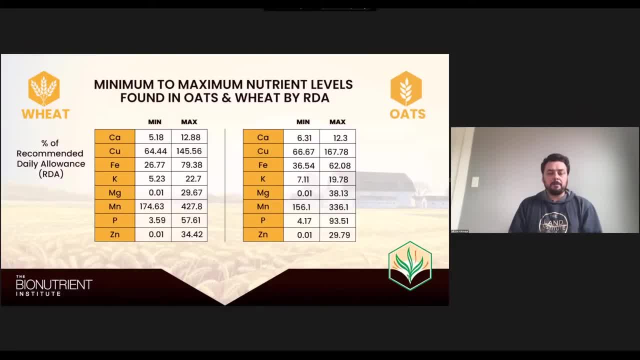 So how much calcium do you need per day, per serving? You know, how much do you get per serving of wheat. How much do you get per serving of oats? If you had bread or you had oatmeal, look at, we'll look at- potassium on wheat there in the middle. 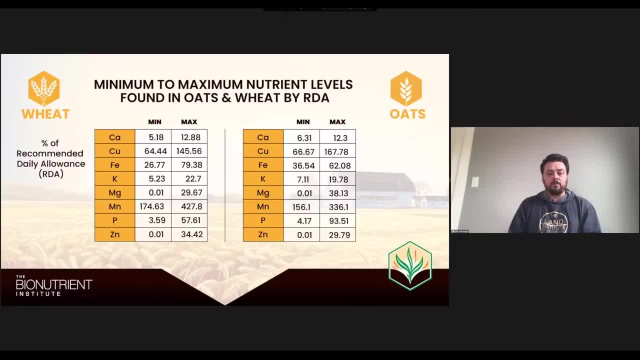 and okay, you know, one serving of wheat, one slice of bread, might give you 5% of your potassium. Potassium needs for the day are 22%. Magnesium: basically nothing, or 30%. People know what magnesium deficiencies dropped down to the bottom for zinc. 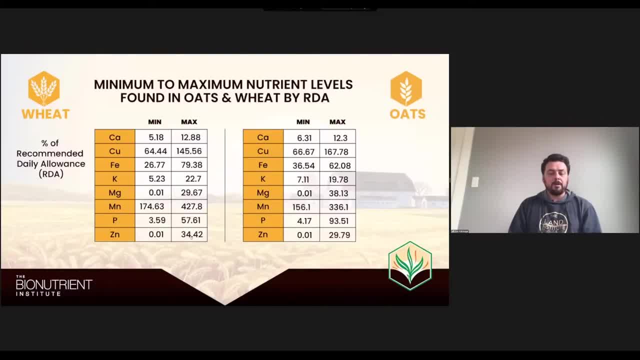 basically nothing, or 34%. How many people planet-wide suffer from stunting? You know you went serious dynamics here. This is the variation we found. The variation we found in crops that exist for cereal Rice is very significant from a nutritional standpoint. 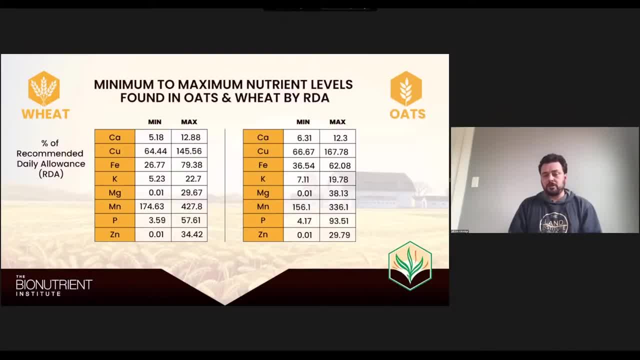 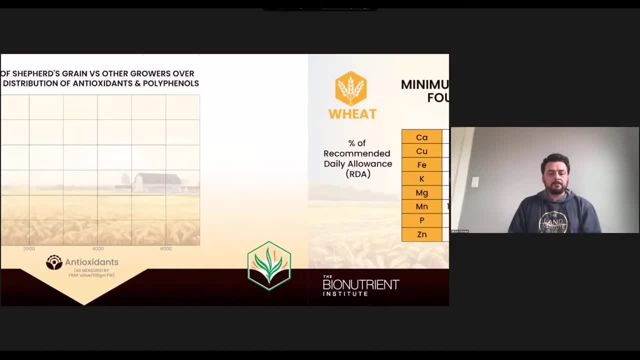 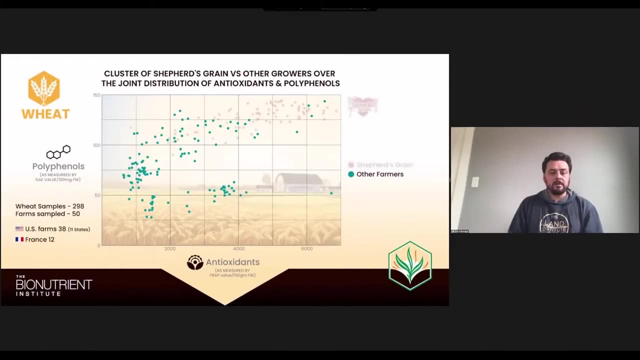 Over there on oats: same thing. Those are just. these are just grains. We did roots, leaves and fruits as well. Proceed forward. So this is a slide on wheat, Just one more step forward. So those red dots are growers that were working together. 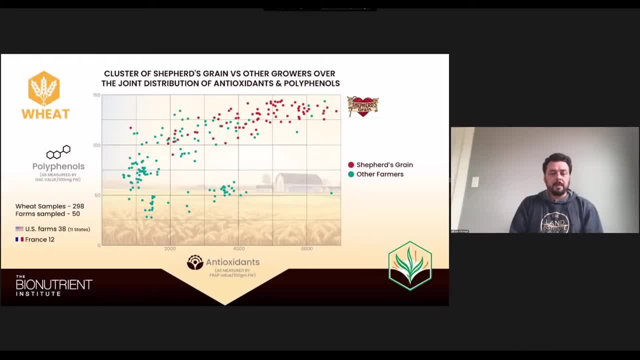 on more biological management. This is the global sample And the green dots is everybody else. I mean this is. it's a meta system, right? Biological systems have multiple factors, so we can't just draw direct connections, but we can see management practices, soil, carbon. 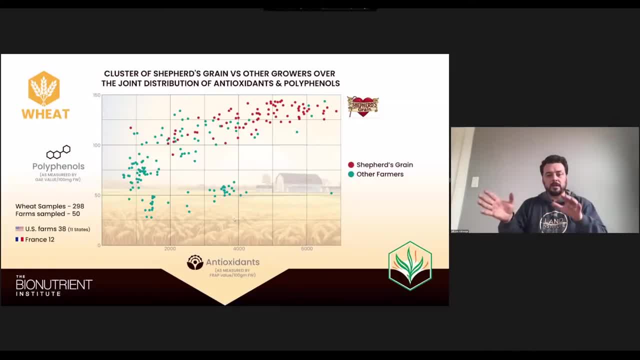 We can see soil carbon management practices, nutrient levels. We can see management practices, nutrient levels. It really looks like it's not so much about the variety you're using or the geography you're in. It's really about how you work with the land. 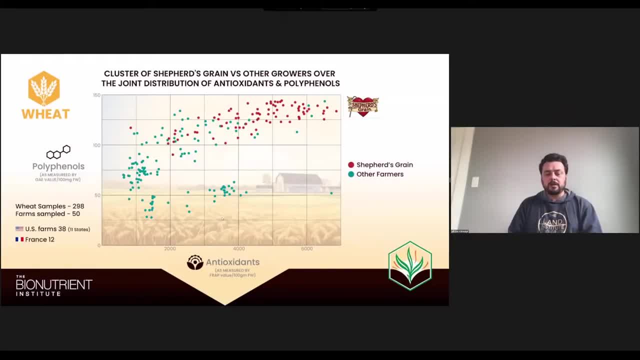 that affects what's in the food, So I'll stop there. I think we're. maybe that was my 10 minutes, but hand it off to Stefan. We have looked at these variations on roots, leaves, fruits and grains. I'll put in some links in the chat after I get done speaking. 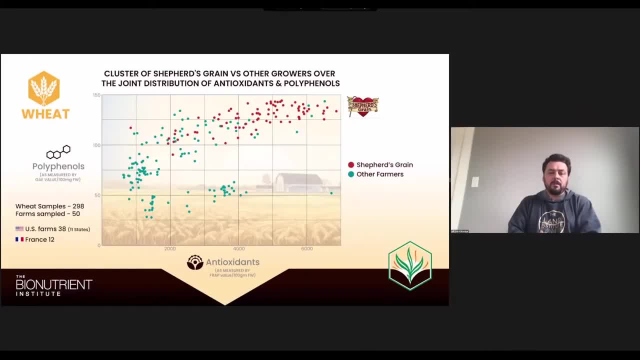 about where links are. You can see what we've been doing. Right now we're working on nutrient density, which is not just top to bottom calcium, you know, top to bottom polyphenols, but better decent, not so good. 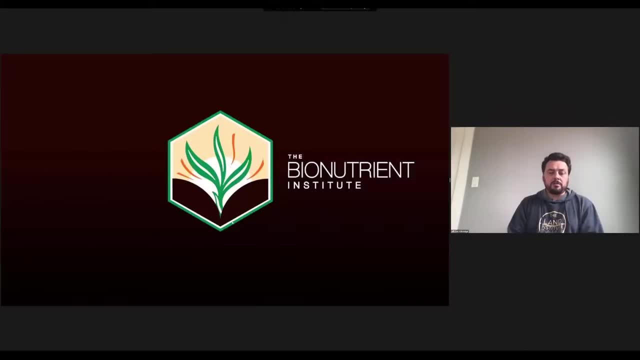 And we're starting with beef, because it's the crop with the largest market value on the planet and affects the largest amount of land on the planet. And if we can understand a way to provide consumers the ability to actually choose the burger, the steak, 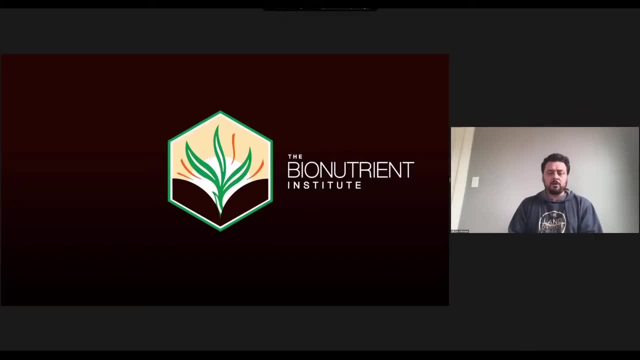 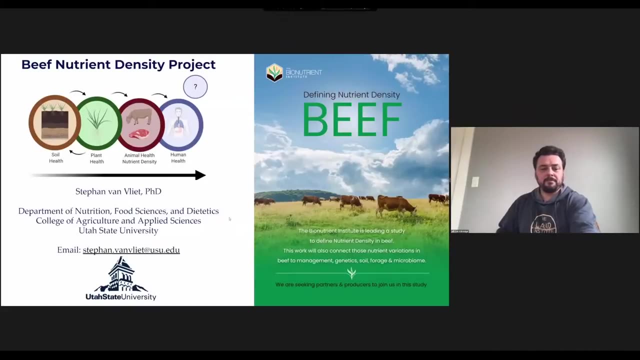 whatever it is that you buy, because people do buy beef based on quality- that should have profound effects on the landscape in short order. So I'll stop there. Yeah, thank you so much, Dan, And I will try to keep it brief, so we have plenty of time for Q&A. 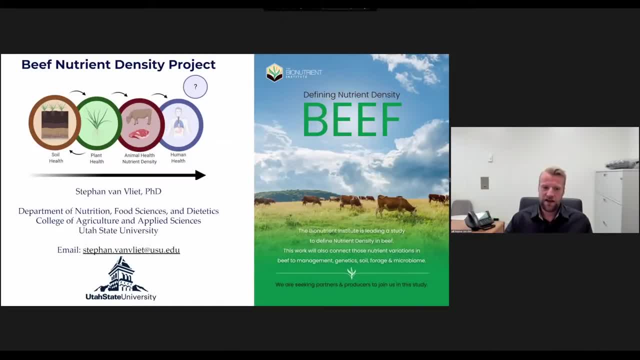 But I'd like to talk to you about the Beef Nutrient Density Project that we're doing. Oftentimes you hear this connection between soil health, plant health, animal health, human health. There's not a lot of systems research out there to suggest that that is the case, even though it intuitively 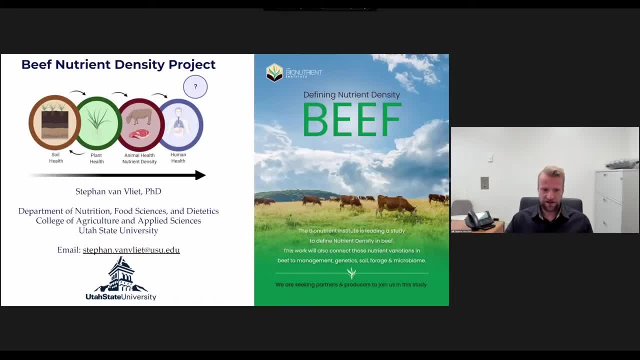 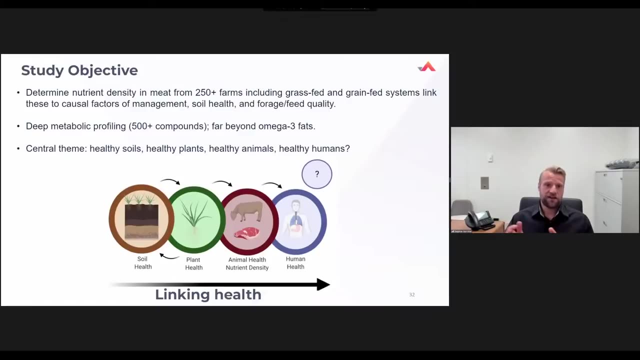 makes sense. So we're doing a beef nutrient density project. The goal is to collect sample samples- Yes- from 250 farmers over the next couple of years. please advance the next slide in beef. we are doing this in grass-fed and grain-fed systems and linking that to causal 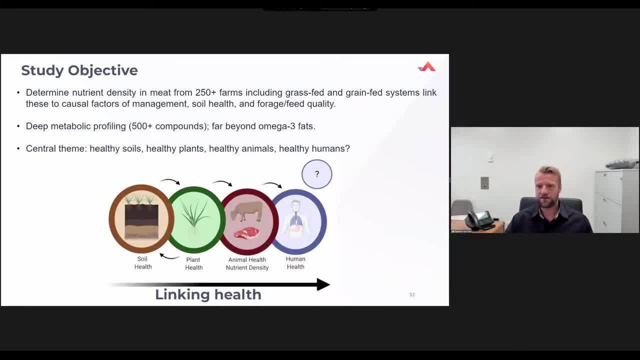 factors of management: soil health and forage feed quality. there's likely tremendous variation between more rotational grazing and continuous grazing. we know it's the case for soil health, so it would be expected it's the case for nutrient density too, and not all feedlot systems are. 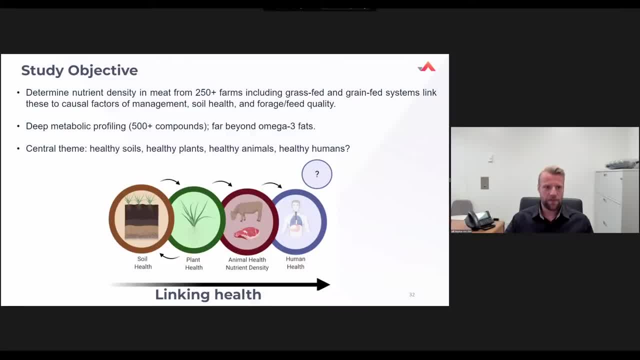 created equal either, is what we're finding in our data so far, and what really makes our analysis unique is that we do deep metabolic profiling, so not just looking at fats, omega-3 fatty acids, which is common, but we look at take a more holistic approach, because foods contain hundreds. 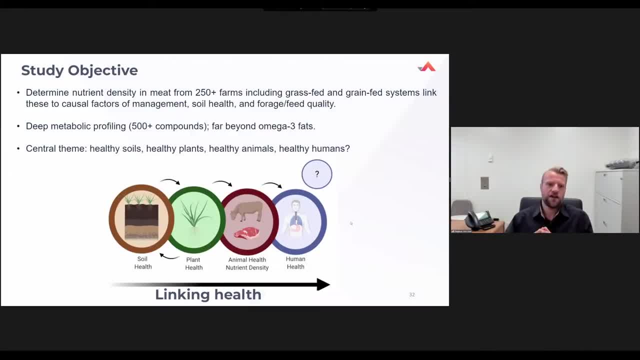 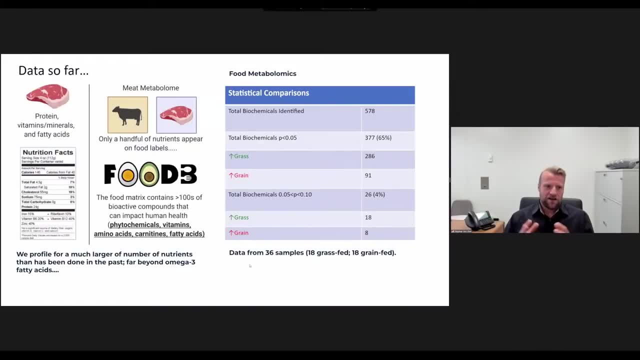 to thousands of nutrients and compounds that can impact our health and we're linking health along that continuum and please advance the slides. so just to talk about the data so far, if you are a consumer and you pick up a package of beef, you see a handful of nutrients appearing. 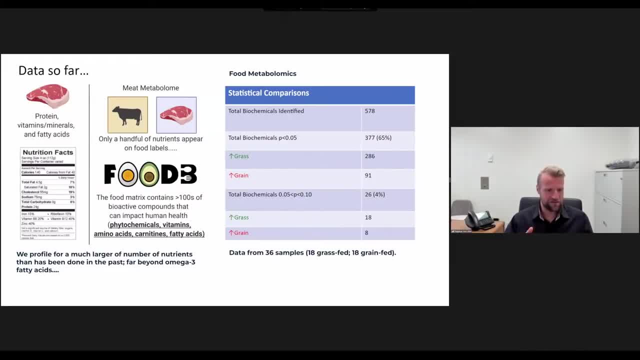 it's about 13 nutrients, your protein, fats and a handful of vitamins and minerals. a lot of our knowledge on how production impacts these small amounts of nutrients is obviously very, very powerful, but we need to take a more holistic approach, because the food matrix contains hundreds or thousands of bioactive compounds that have not 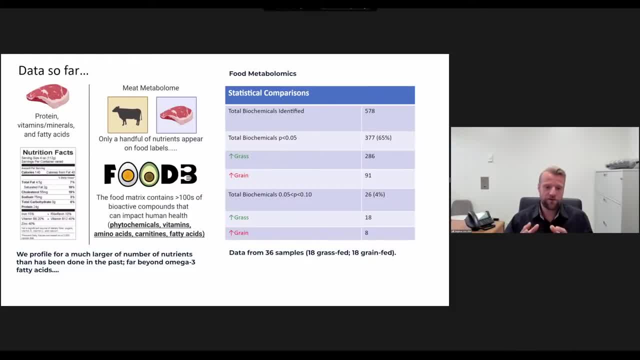 been at the forefront, but they do impact our health, so we profile for a much larger number of nutrients and if you look at the table on the right, this was a comparison of grass, fat and grain fed beef from 18 samples and we identified 568 compounds using our food. 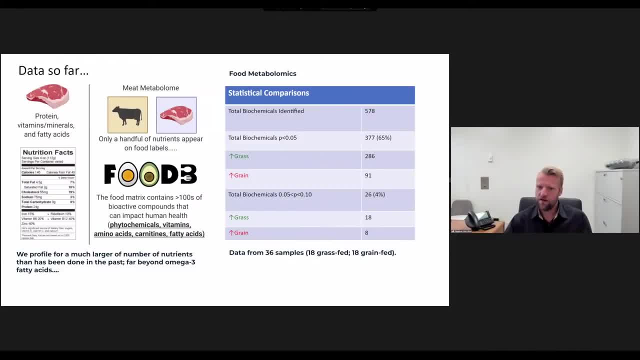 metabolomics approaches, which is much more than has previously been been done, and oftentimes we hear about the difference in omega-3 fatty acids, but you can see here the 65 percent of these biochemicals were different, so illustrating that the difference go far beyond omega-3 fatty acids. and certainly not all these compounds that we measure are nutrients, because 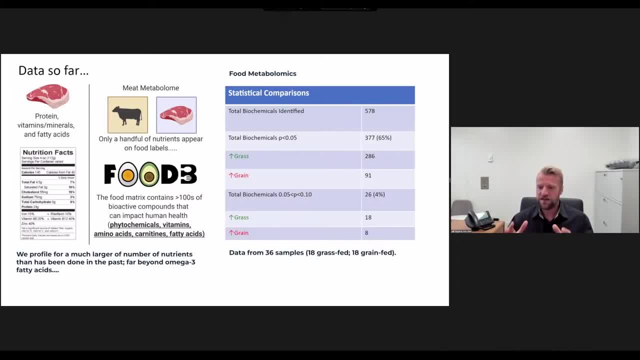 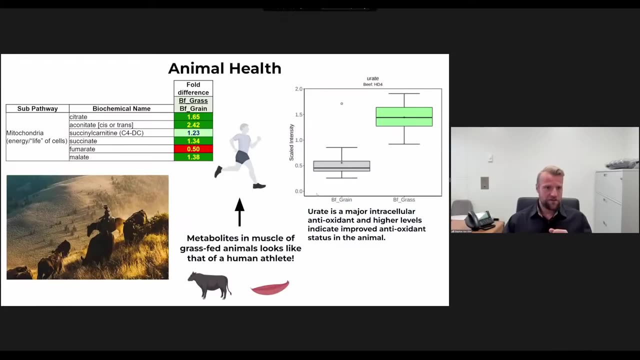 we also get insight into, into animal health. but, as you can see, there are substantial differences and arguably larger than i had even anticipated, and these differences are also arguably not known with the consumer at the moment. so if we advance the slide and we can see, this is a markers of animal health. so i'm originally trained as a human nutrition. 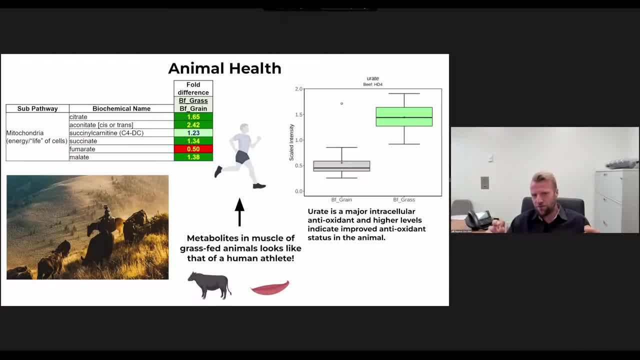 scientist and we do these studies on humans too. we take small pieces of muscle through a muscle biopsy and we've profiled that before. we've done this in individuals with metabolic syndrome, we have done this in endurance trained athletes, but we've also profiled meat samples, muscle of 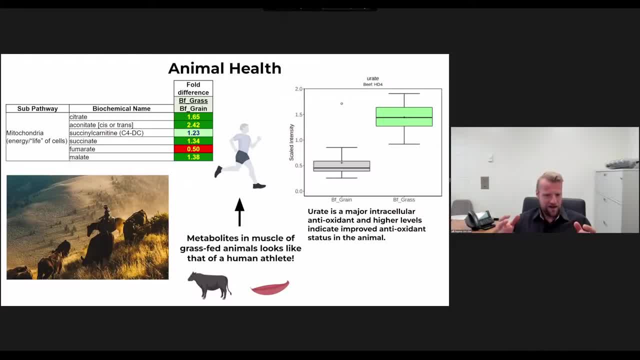 animals. and what is quite striking there is that the animals that have, uh, that are pasture, raised and move around a lot and and eat uh phytochemically rich forage, their mitochondria, which is the energy or the life of cells. and these biochemicals you can see citrate, succinate, fumarate, malate. 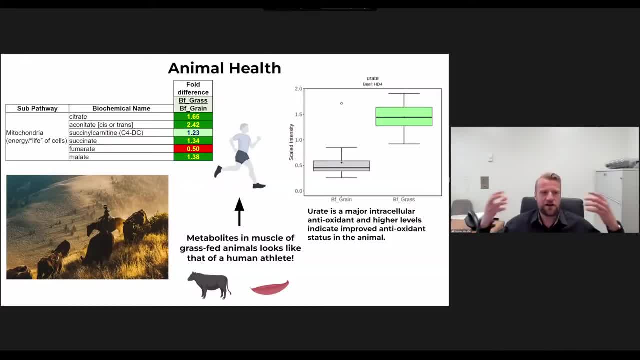 those are all intermediates in mitochondria. so mitochondria they produce the energy or the life of ourselves and we see that that life is higher in in grass-fed samples, so about one to one and a little higher in the in the green means higher. it was higher in the grass-fed samples. then uric acid: 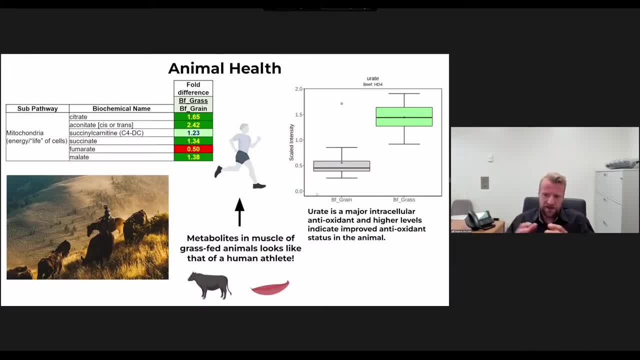 is a major intracellular antioxidant and higher levels indicate improved antioxidant status in the animal. and there's about a hundred more metabolites that all point to the same direction, suggesting that the pasture-raised animals display more of an athletic phenotype, not unlike you would see in. 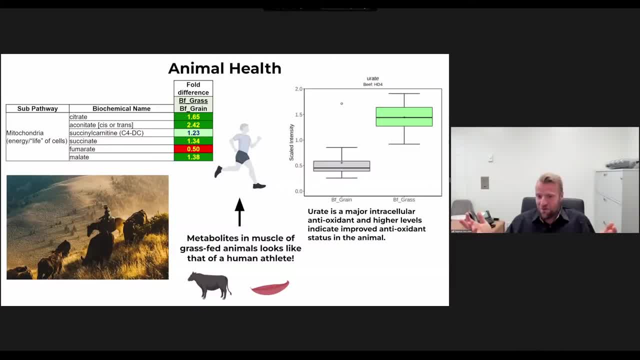 humans. after all, cattle and humans are more likely to be more active in the wild than in the wild. we're both mammals and uh. the differences in in that regard are striking compared to, we compare healthier phenotypes in humans and animals. so let's move on to nutrient density. 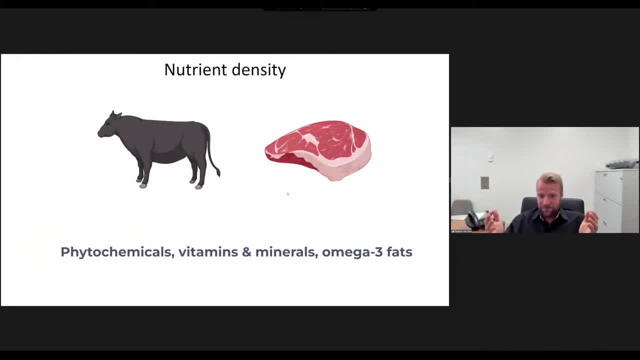 nutrient density can be defined. as we are specifically looking at phytochemicals, which are plant secondary compounds, antioxidants that are picked up from the forage and incorporated into the meat. a lot of these have anti-inflammatory effects, antimicrobial effects. various studies suggest that, at least in in in the lab, they can have anti-cancer and 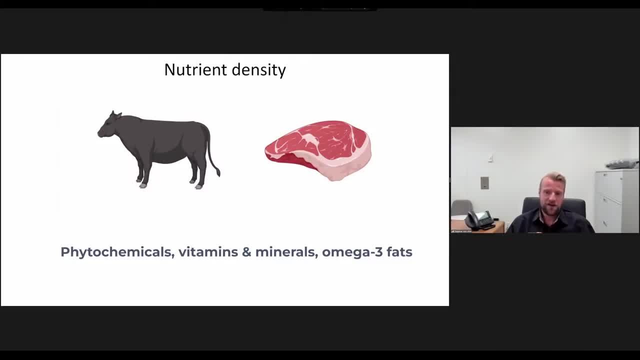 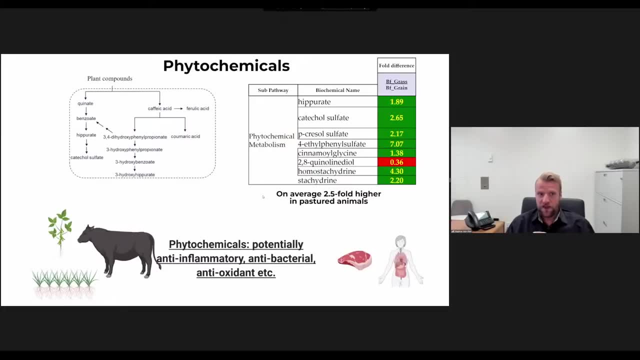 anti-diabetic effects. we also look at vitamins and minerals and, of course, fatty acids. so if we jump into that for the last few slides, so phytochemicals. phytochemicals are produced by plants. when animals raise these phytochemicals, these plant compounds, as you can see on the top left, they are. 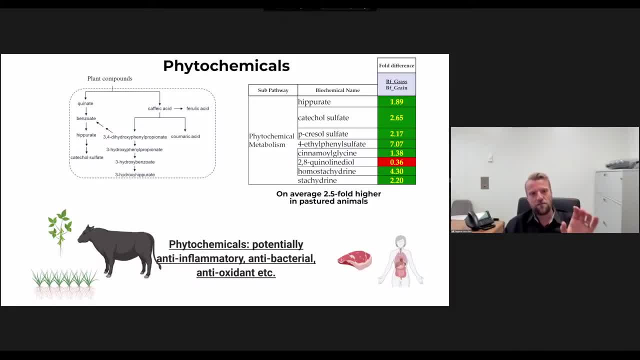 to a whole variety of of different compounds, and these compounds are compounds with potential anti-inflammatory and antioxidant effects. the figure on the right: you can see phytochemical metabolism and i've highlighted a few here. but what you can see here is that these phytochemicals 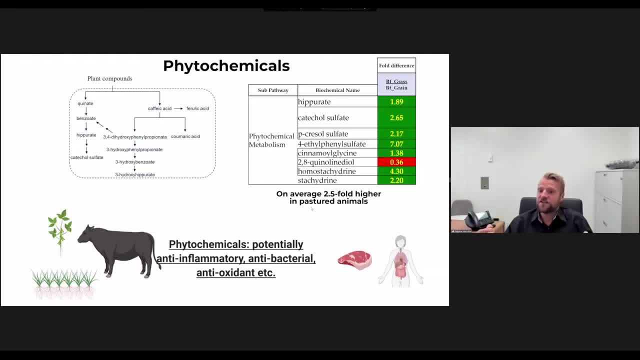 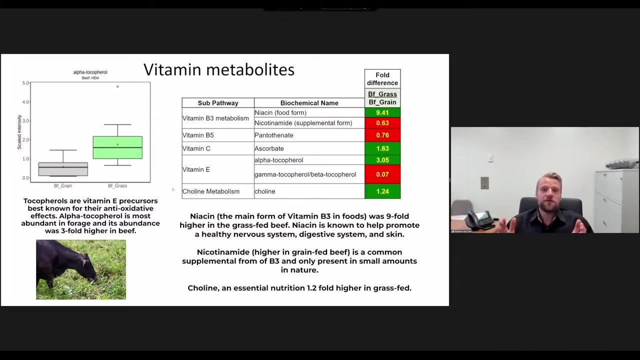 are consistently higher in the grass-fed animals, which is that the direct result of them grazing a wide variety and a diversity of plants, um so if we move on to the next slide, we see the same thing happening in these vitamin metabolites, which also have a relationship to. 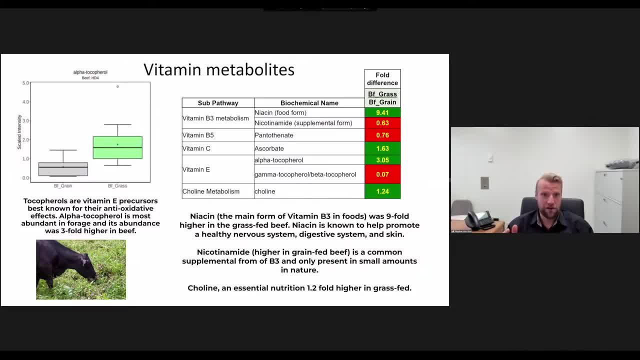 improved soil health and improved plant health. if we look at vitamin b3, niacin, which is the main form of vitamin b3 in foods, this was nine-fold higher in the grass-fed beef, which is directly related to the forage and presumably also soil health. um niacin and nicotinamide are both vitamin b3. 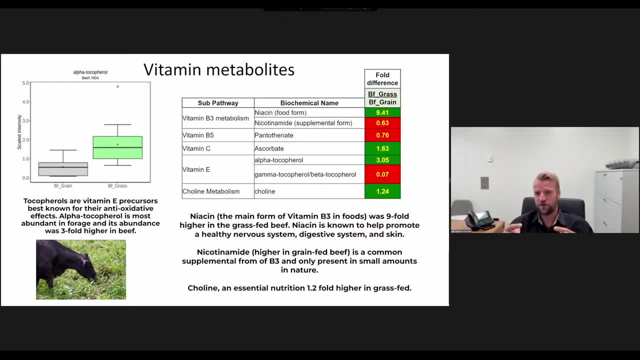 but niacin is the most abundant form in food found in nature. that was nine-fold higher in the grass-fed animals, whereas nicotinamide, the supplemental or synthetic form, was about twice as high in the grain-fed animals, which is likely due to the fact that this is commonly used in finishing rations. 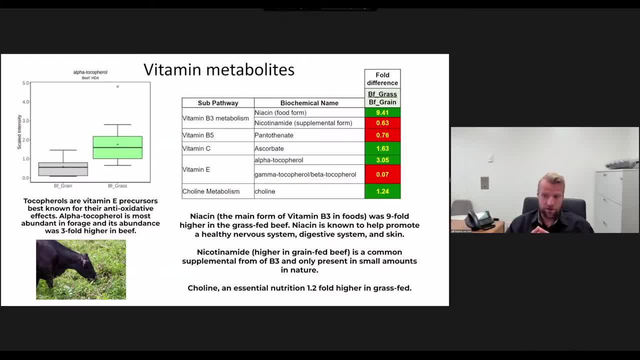 choline, another essential amino essential nutrients, 1.2-fold higher, and alpha dicophore and ascorbate vitamin c were also found to be higher in the grass-fed animals. the cough rolls of vitamin e precursors best known for the antioxidant effects, and they are. 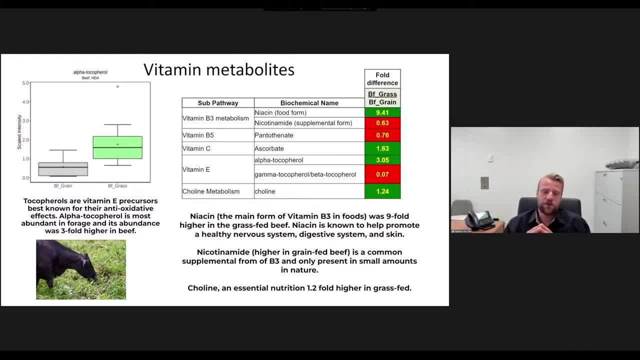 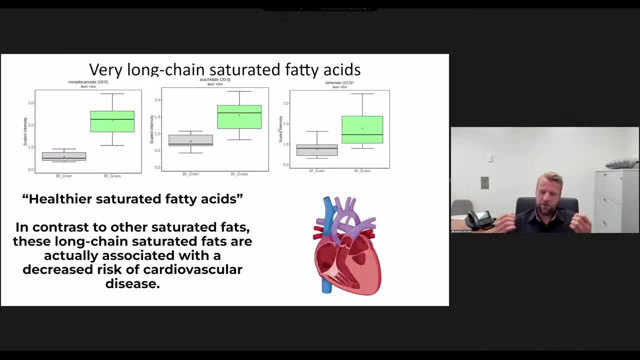 again directly related to consuming phytochemically rich forage. so we are seeing this relationship between more phytochemically rich plants and more nutrient-dense beef. so, if we go to the final slide- and i just want to highlight this because we often hear about omega-3 fatty acids- 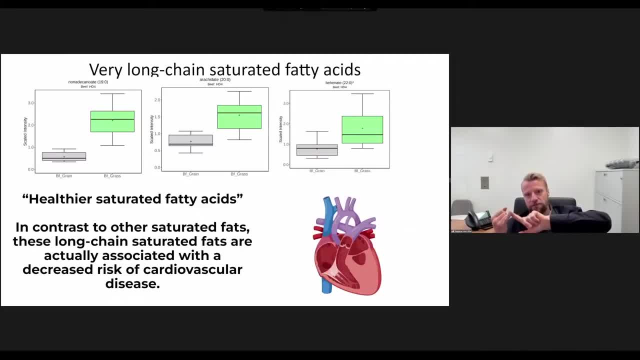 and the omega-3 fatty acids that would be epa and dha- are enriched in grass-fed beef. but what we are seeing in our data- and i think this is not well known with the consumer at the moment- is that within the saturated fatty acids often thought to be bad for our health, we actually see that within the saturated fatty 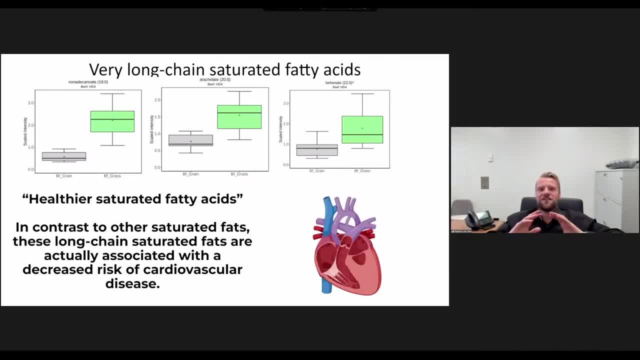 acids. it's. it's a broad category here. there are maybe 10 to 20 different saturated fatty acids and these longer chain saturated fatty acids that are actually associated in population-based diseases. so we can see that in the grass-fed beef the decreased risk of cardiovascular disease. 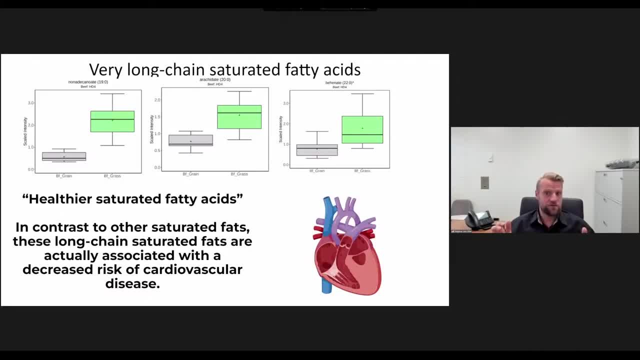 again become enriched in the grass-fed beef because of, uh, the forages that they consume. so, again, not all saturated fat is created equal either, and so we see these multiple patterns appearing where, if we feed the animal a more diverse and phytochemically rich forage, we see 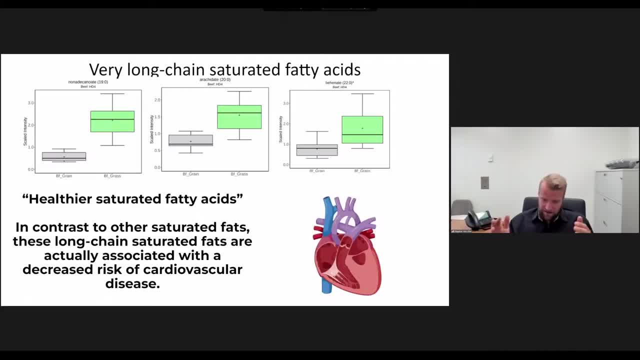 their health improving and their nutrients improving with that i want to say is that that, but as compared to grain-fed beef, grass-fed beef does have additional benefits, and but there are also nuances. and i must say this is that when we've done studies, when the higher amount of 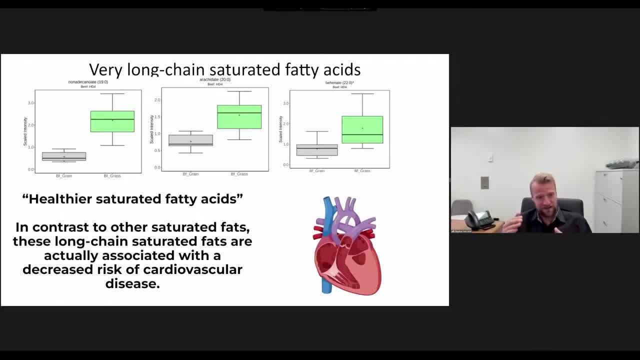 father or forage is fat in feedlot systems. we see that then the grain-fed beef or the feedlot beef also recovers some of that nutrient density. so it is certainly not black and white or a simplified narrative that this is good or bad, but the data is what it is. 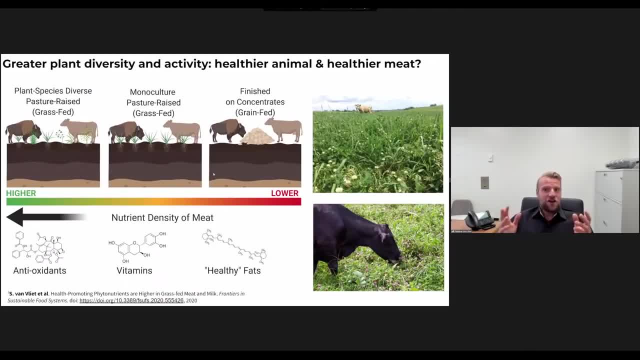 final slide. so within the beef nutrient density project, this is our working hypothesis. if we raise animals on more plant diverse species, we see a higher nutrient density of meat compared to monocultures or over grazing, with the lowest amounts of found in feedlot meat at the moment. but the goal of this work is to figure out this variation and 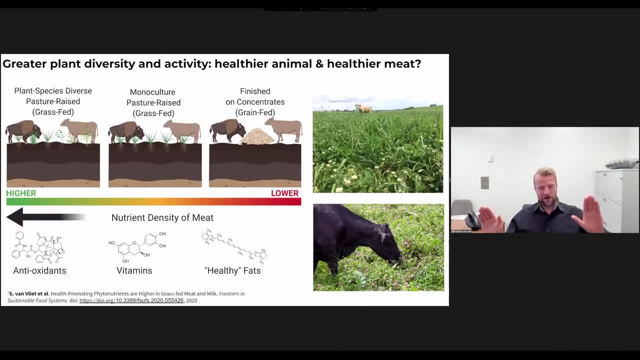 link it back to causal factors, because grass-fed beef isn't grass-fed beef, isn't grass-fed beef, grain-fed beef isn't grain-fed beef isn't grain-fed beef, and the goal is to improve best practices amongst each of these systems, and with that i'd like to end my part of the. 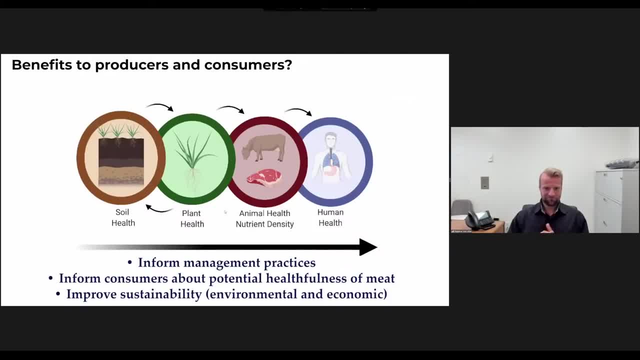 presentation and looking forward to the q a. finally, though, how can this benefit us or producers and consumers? well, we can highlight the best practices. so inform management practices. inform consumers about the potential healthiness of meat. so marketing death. attention to consumers when we know more about the nutrient density, and obviously the bigger 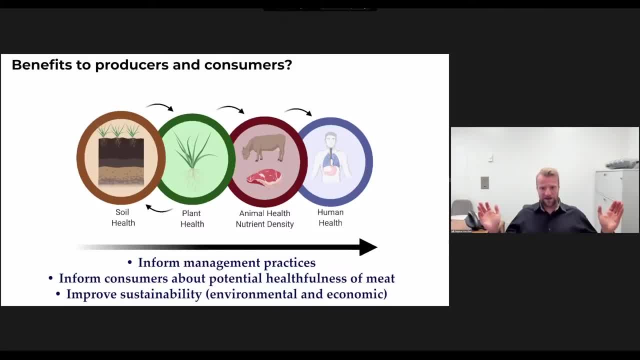 picture is: as we try to nourish a growing population, do so sustainably. uh, we must think also of environmental, economic factors, and i want to highlight the ipcc report that came out recently. yes, the report calls for moving towards, uh, more plant-based patterns and increasing our plant-based foods, but that report also stressed the use of agroecological livestock. 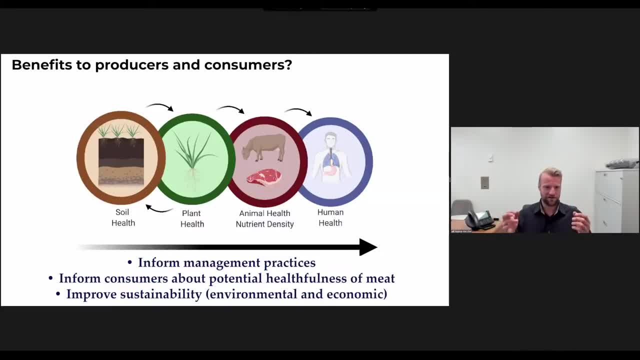 production systems, which means rotational grazing, integrated carbon livestock systems, silvopastoralism, which are the practices that we are investigating and are finding that they indeed produce more healthier soils, healthier animals and potentially also healthier humans, which will be studied as part of randomized control trials we do in the next few years. thank you so much. 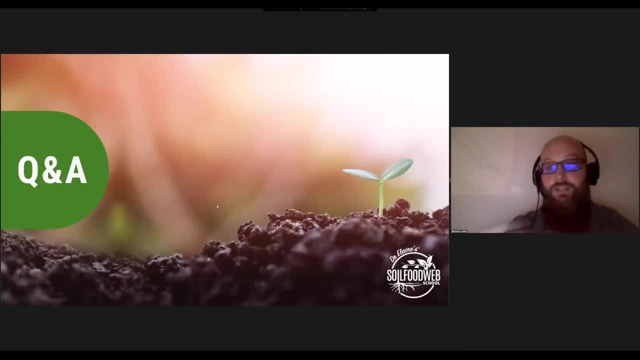 well. thank you so much, stefan and dan. um, and it's such a great point that you made there about the the value of properly managed rotational grazing systems where we've seen so much soil health benefit. um, in the long run. in fact, i know a few ways that i've ever read about to more rapidly. 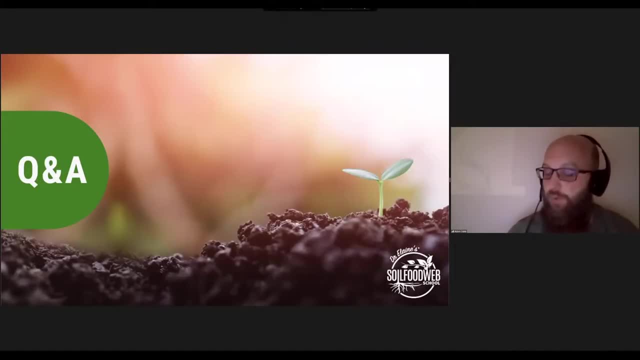 recover soil health than to use perennial pasture systems to do so. so we're going to move on to our q a session and we are running a little behind today. so in order to get the the webinar finished in time and make sure that the panelists are able to go to their next event, we have about 30 minutes instead. 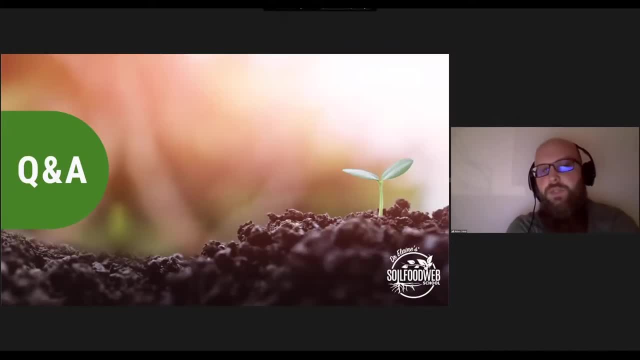 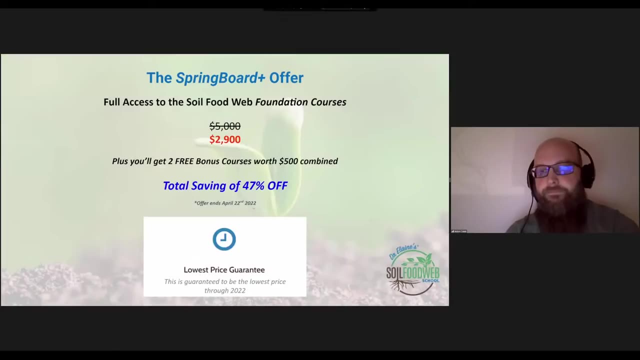 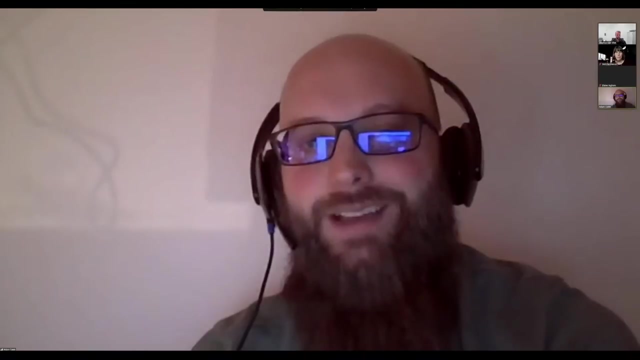 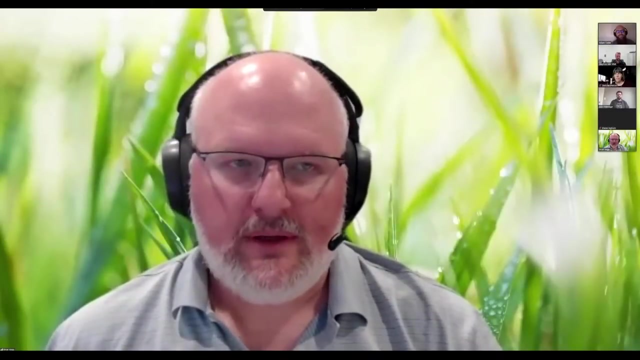 of 45 um. but let's, uh, let's, let's pull up our first q a, our first question. oh, i'm sorry, there are tech. we seem to be having a little bit of a technical glitch. will you take that away for us? sure, i'll read out the first question and then 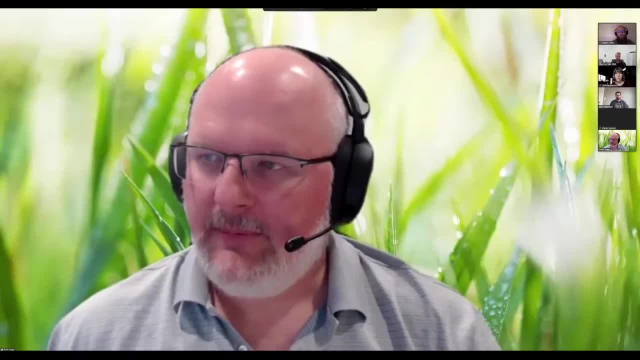 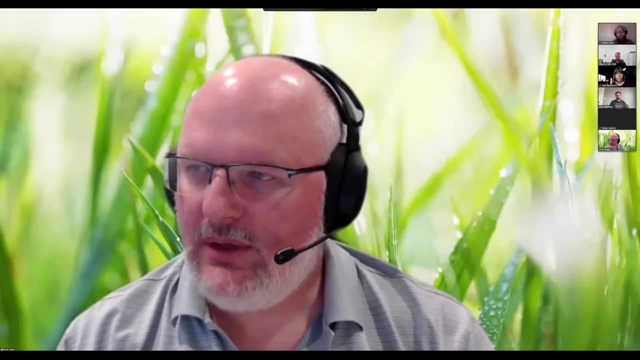 i'll try to get them into a slide form so we can- the participants can- see it. so the first question is from diane, and diane asks: i'm disheartened at people's apathy towards land regeneration as a tool to combat climate change, or towards climate change itself. what has been your most successful approach? 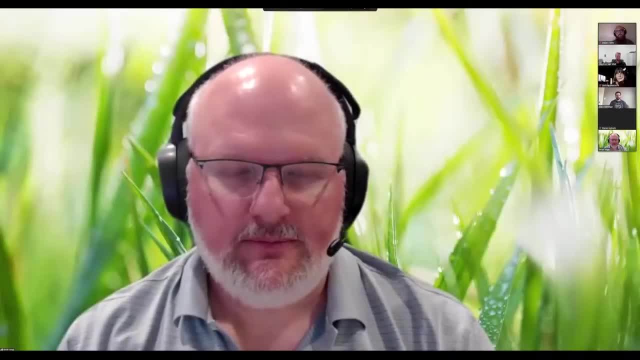 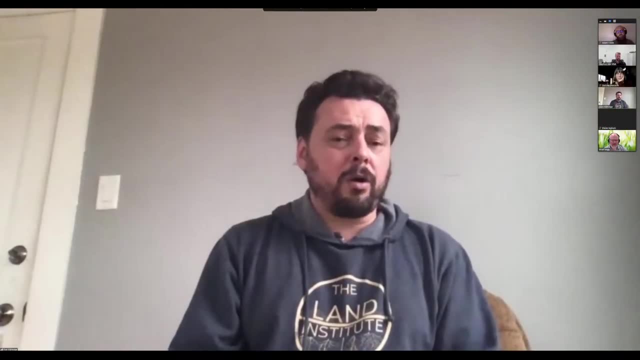 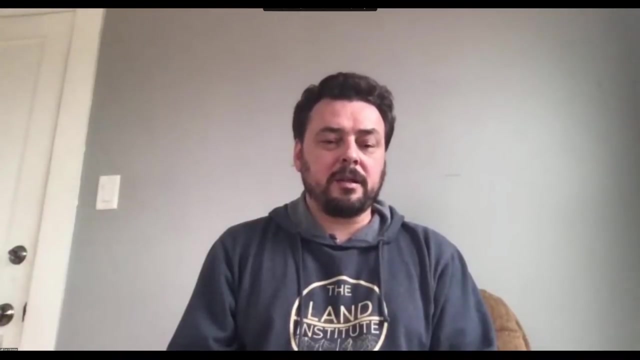 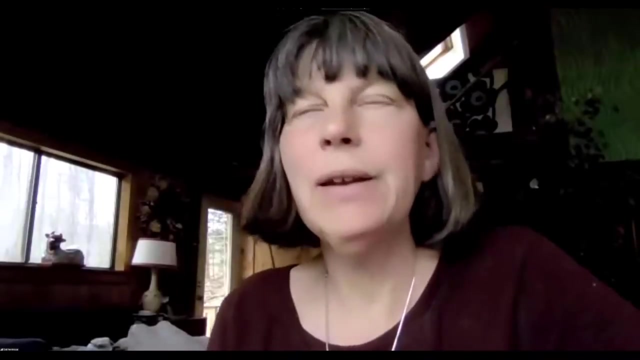 to influencing the average person on these topics. all right panelists would say you. i'll just say really quickly: um, our hypothesis is that if people care about themselves and their families and that connects to the land, then that's a really powerful vector and i i would say that, um, it's really key to get everybody moving toward the things that. 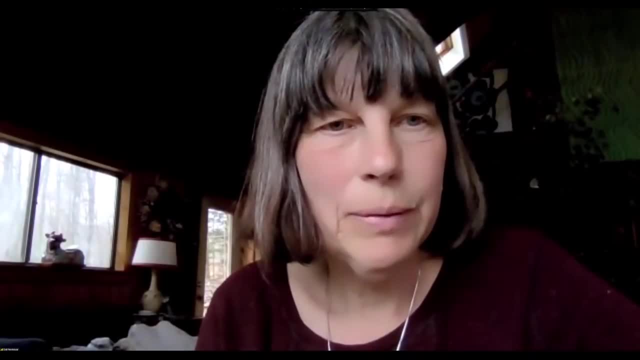 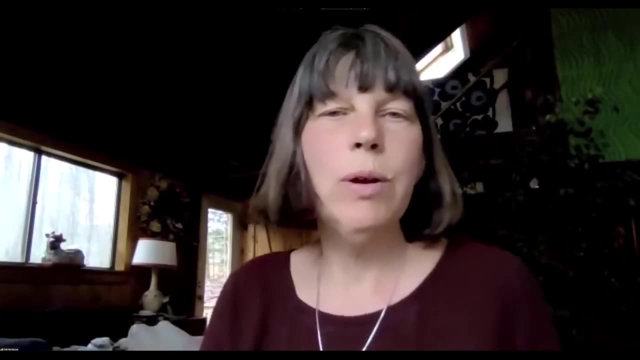 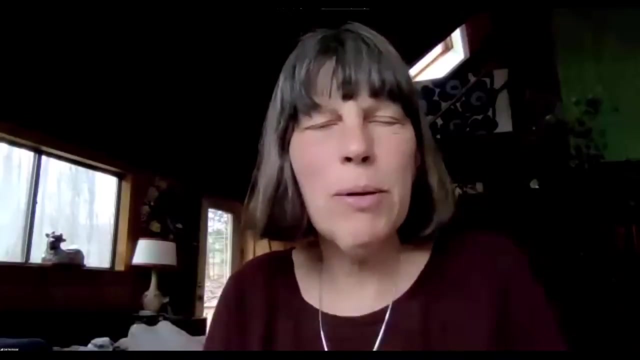 they all want um and so um. so anytime that we start using language- sort of fighting language or turning around and what fighting against? what we don't want, um is a, is um, getting people into arguing about what that is, whereas it's much easier to say: we all want regulated temperatures. 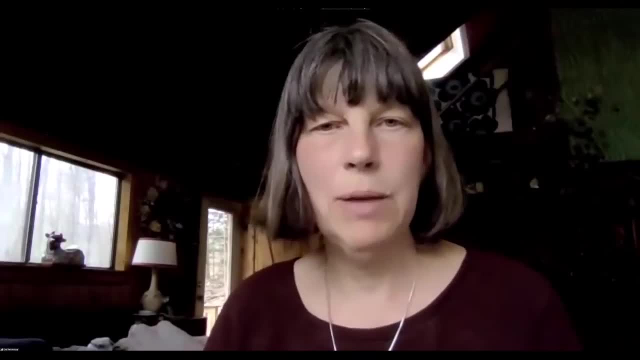 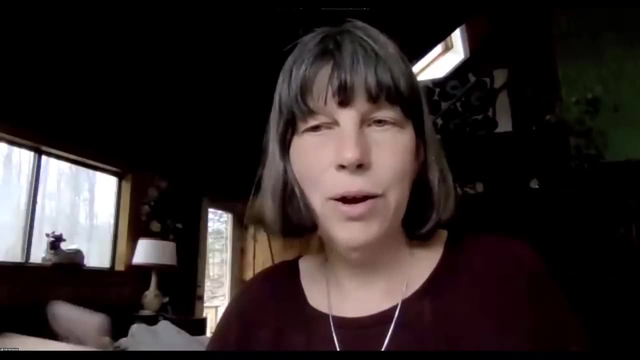 whether whether we think that an ice age is coming or we think that climate change is coming, we all want clean air, we all want clean water, we all want enough food, we all want protection from floods, whatever they're being caused by. so i found that soil health offers really an 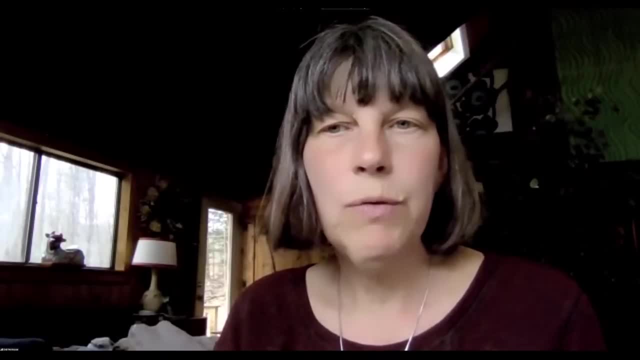 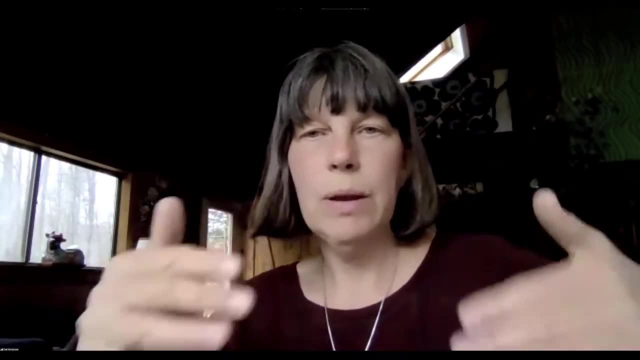 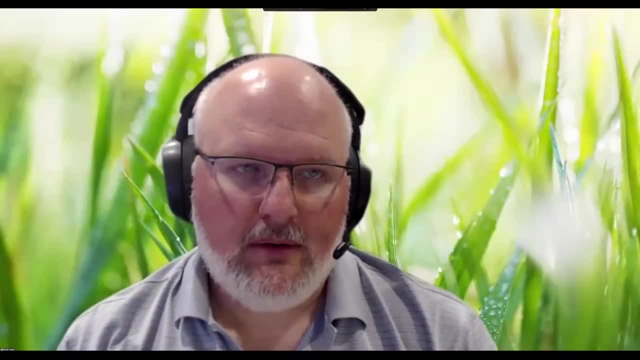 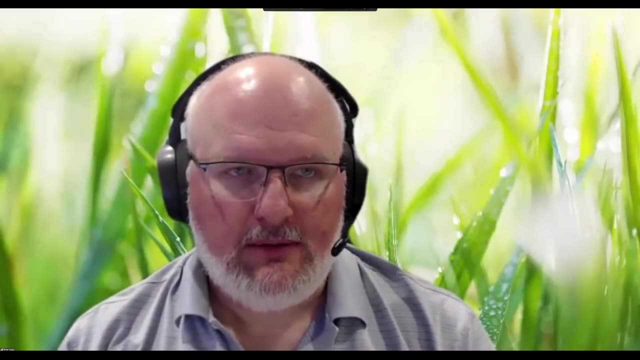 um, i'll just add my. my opinion is that knowledge is power, both knowledge from the consumer standpoint. so the more we can educate folks on the importance of soil health and soil biology and how that relates to human health is fantastic. but that's also informing the producers, the people that are actually, you know, doing the growing or the raising of animals. 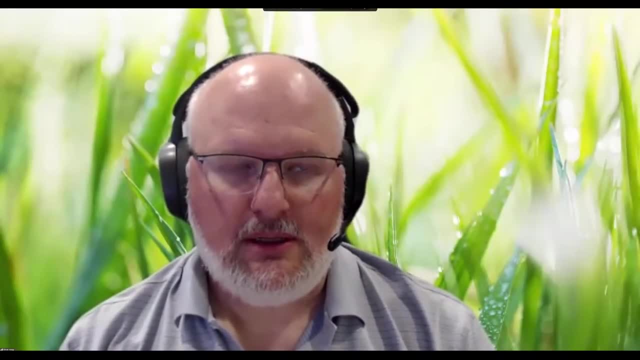 and so forth and making sure that they have the education and knowledge. and unfortunately, i think our university systems are lacking that sense but are starting to catch up and i think, as this really starts to to progress forward, i think we'll see a big momentum shift both from the producers and the consumers as well. oh, brian, i can really back up what you. 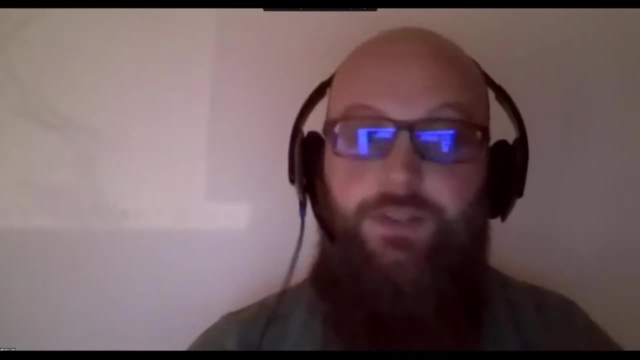 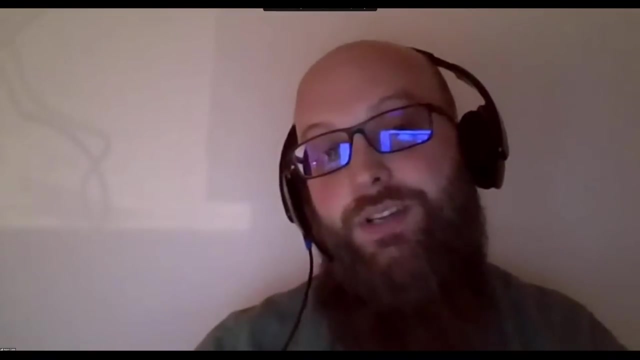 just said about our university system, the switch. um, i'm a product of the land grant system- my myself- but I've done quite a bit of talking to peers about the ingrained paradigms for the industrial kind of system of agriculture. And I'm actually here in Greece currently at a conference. 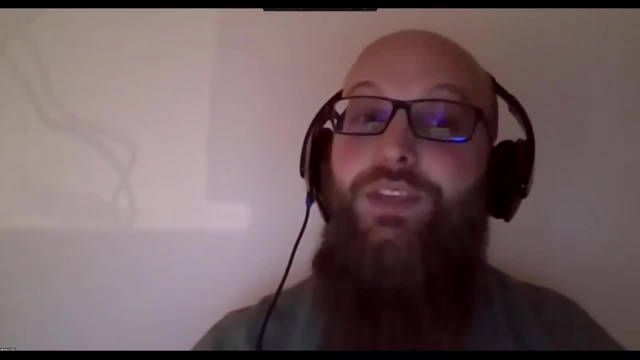 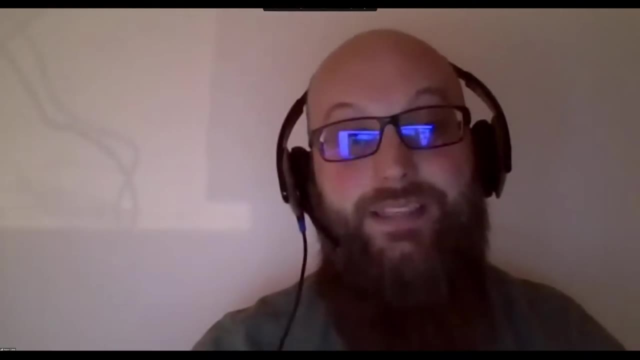 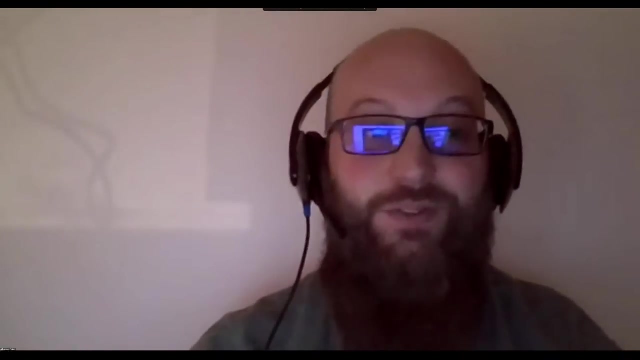 where, when I presented about that, I had a number of young faculty members across the land grant system come and have conversation with me afterwards about how ready they are for that shift to occur, And agroecology is being talked about by young land grant professors. 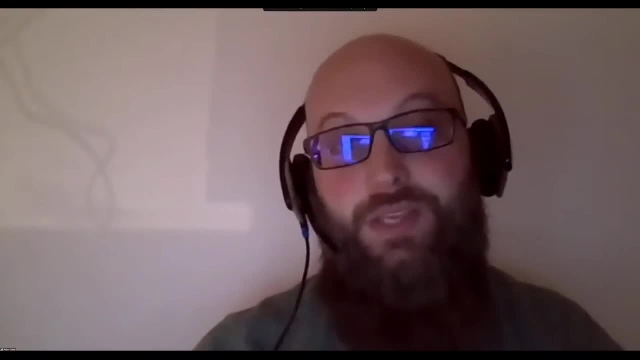 tenure-track professors. Regenerative agriculture is being talked about, And I think that's an exciting step, especially, you know, actually, it's in many cases the social scientists who work in community development that have seen the values of these kinds of systems. 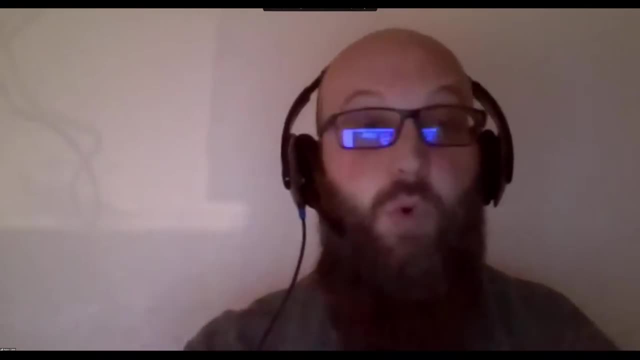 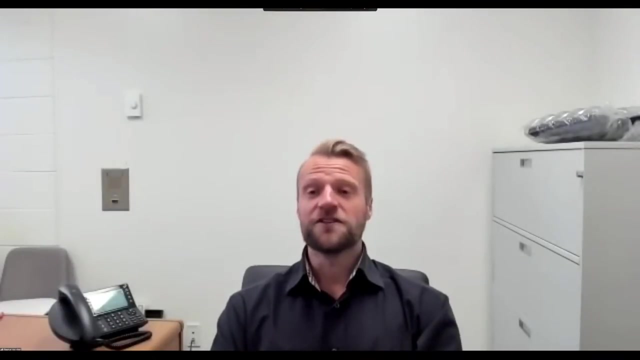 and their research is starting to reach more and more people. So, yeah, great Thanks for bringing that point up. Yeah, And to add to that, I'm an early career researcher myself at a land grant university, but it's also a matter of just doing it right, If you get to. 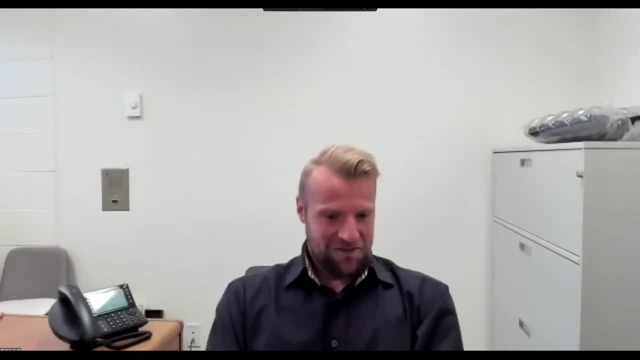 do the research and we obviously let the chips fall where they may and let the data show what it shows. but, yeah, it's just also a matter of just taking the plunge and doing it, And I think the younger generation absolutely is moving towards that And, yeah, it will become more. 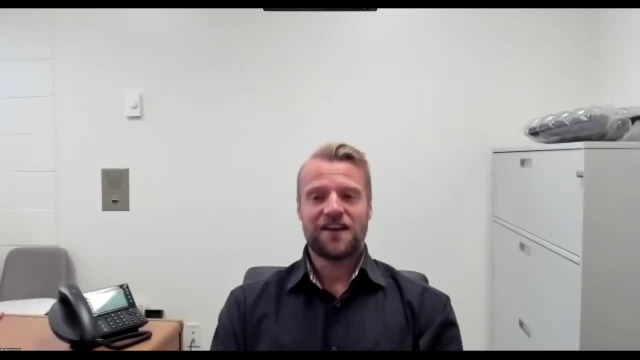 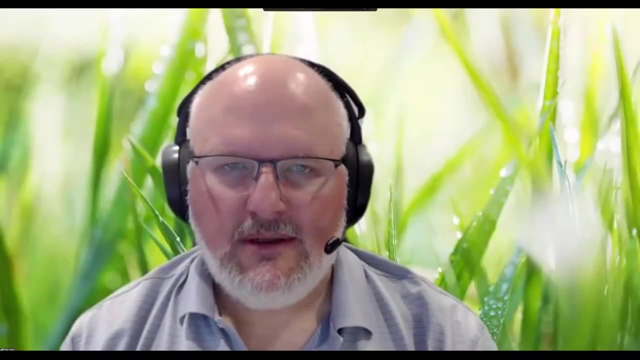 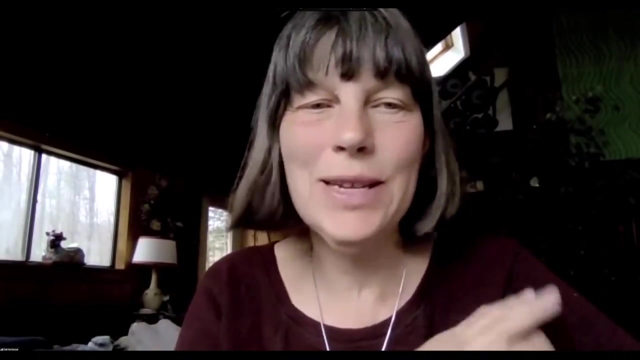 as the future wears on, So I think the time is also right to start investigating these things now. Great, Didi, Elaine, anything else you guys want to add before we move to the next question? See, Didi said no And Elaine, I will just say that that bread and flour thing is so easy I've 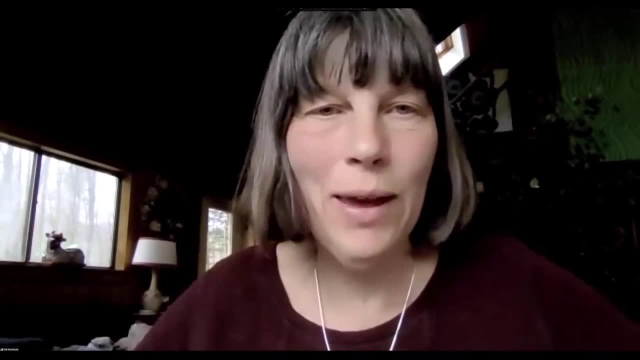 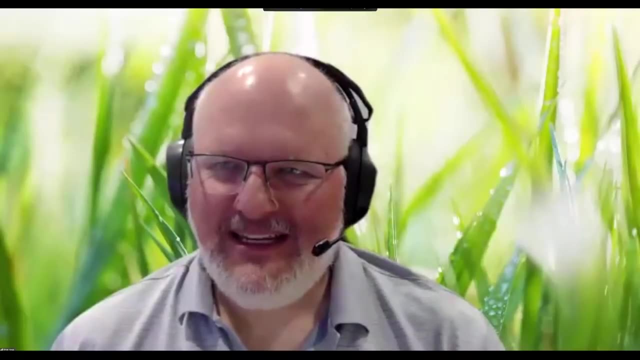 done it in kindergarten classrooms, I've done it on Wall Street, I've done it at the UN. Everybody gets it. So Agreed, Elaine. any closing comments on that question? Nope, I'm no, I'm fine. The other people have spoken for me. Go for it. 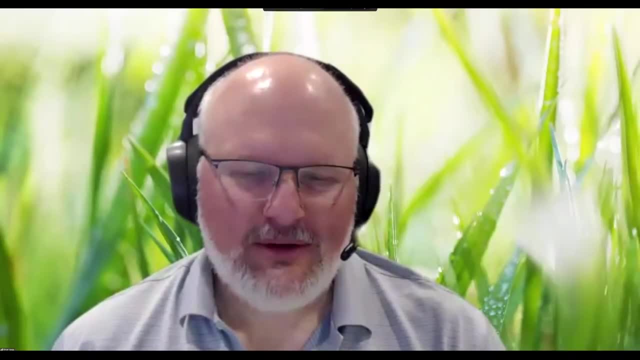 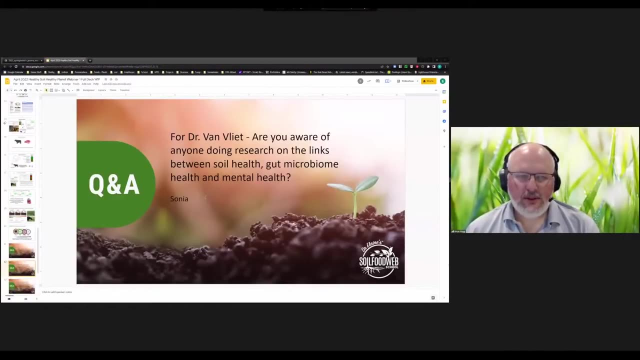 It got well covered. Yep, Yep, All right, Let me go ahead and share out the next question. So the next question was from Sonia and this is for Dr Van Velt. Are you aware of anyone doing research on the links between soil health, gut microbiome health and mental health? 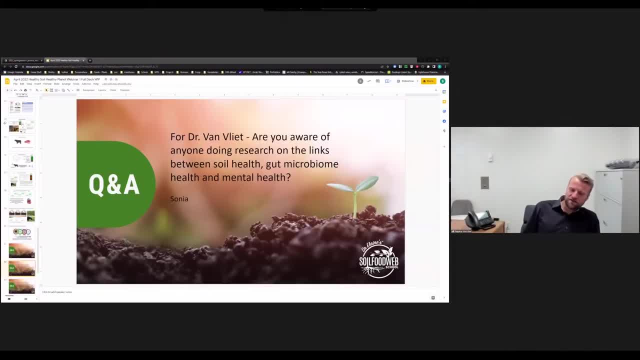 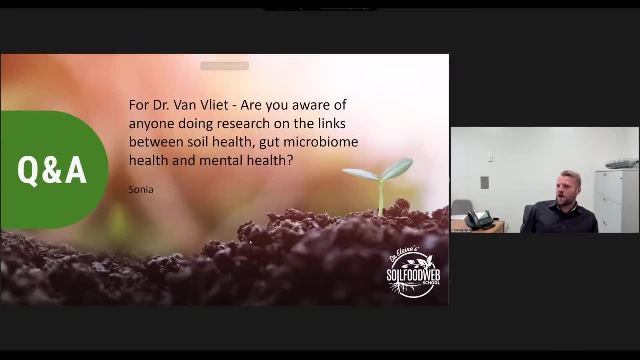 Thank you, Sonia. Yeah, that's a good question. I mean, certainly this work is starting, but and the systems research is becoming increasingly more important, right? So I have a background in human nutrition, in medical school, cultural schools or, not alone, soil health. 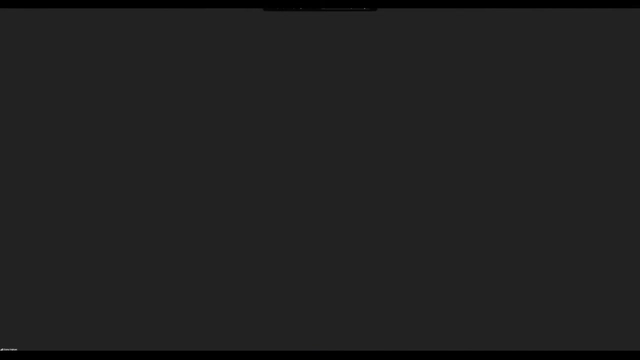 I think it's really hard to answer that question because we are almost assuming that there's a single value for soil health, And that's not true. If you're trying to grow brassicas, if that's the crop that you want, you're going to have to have a sort 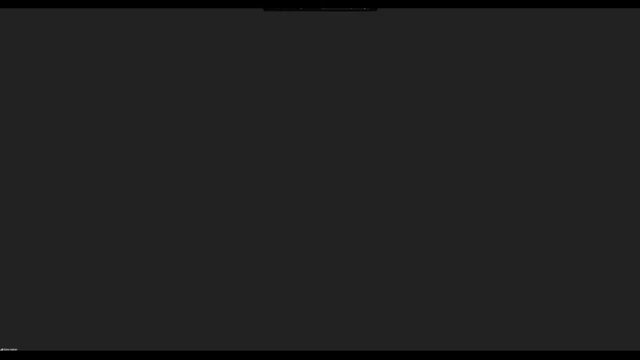 of food web that provides for that. you know, gives the does the right nutrient. cycling The exudates coming out of the brassica is going to be very different. It wants a different ratio of fungi to bacteria in the soil. It's going to. 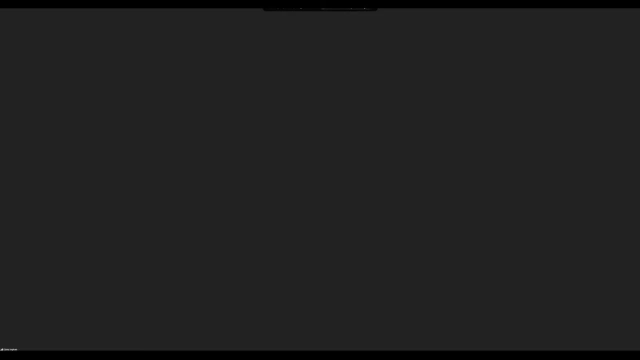 Yeah, Make certain that it maintains that ratio by the exudates that it's producing. Well, what if what you want to eat is carrots or corn, or blueberries or apples? The biology in the soil needs to be very, very different. 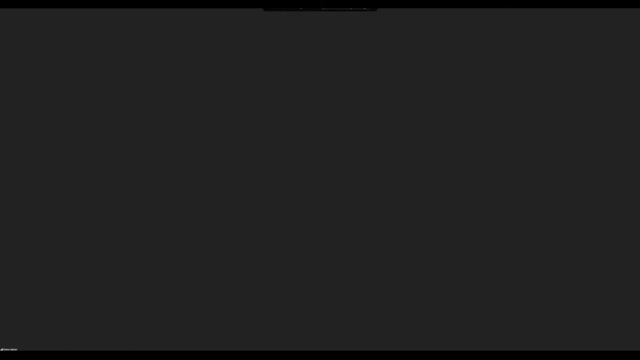 The ratios of fungi to bacteria and therefore the predators. As we go into different biomes, we have completely different species that we're dealing with, So it's not that easy to define soil health, because it's relative to the stage of succession. That's what you have to. you've got to have that comparison chart in order to make certain that the broccoli is going to be the best it can be and have the most nutrients. 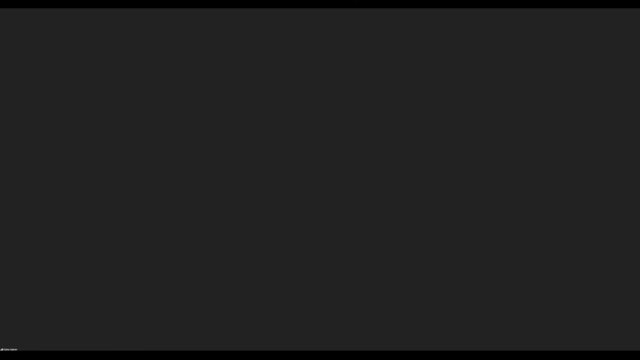 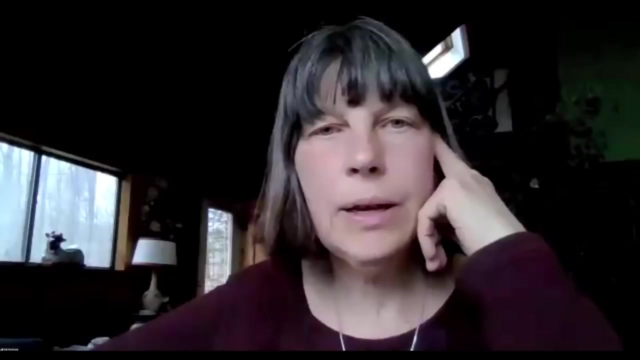 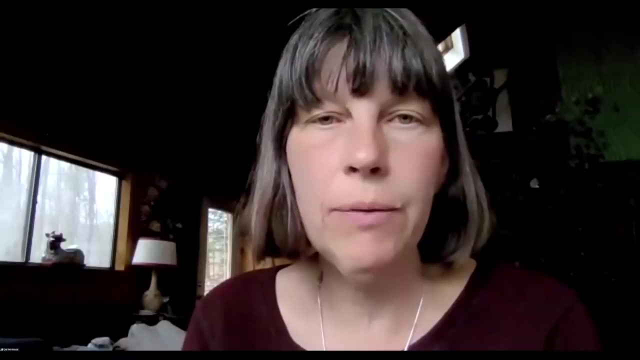 Or the corn is going to have all the nutrition it needs, or the apples are going to have all that it needs. I'll just say that two things. One is that in the first third of my book, The Ecology of Care, that is a lot of what the topic of that part of the book is about. 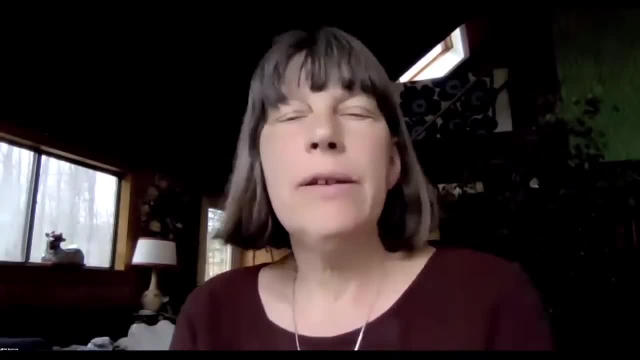 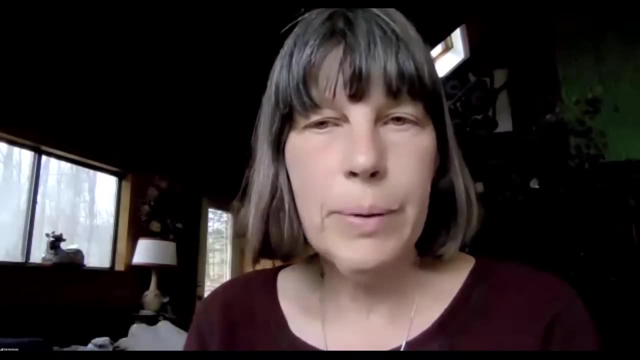 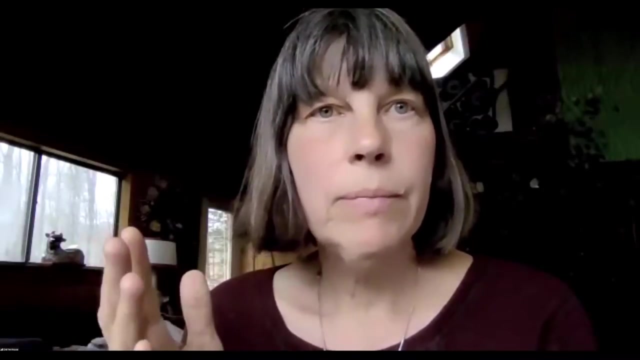 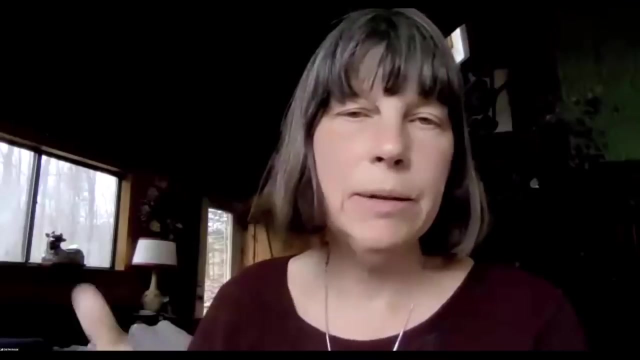 And the other thing is that glyphosate or Roundup was patented As both as an herbicide and as a broad spectrum microbial and antimicrobial or antibiotic by Monsanto. And the reason it works as both of those is because it interrupts something called the Shikimate pathway that exists in plants and in bacteria, but not in animals or insects. 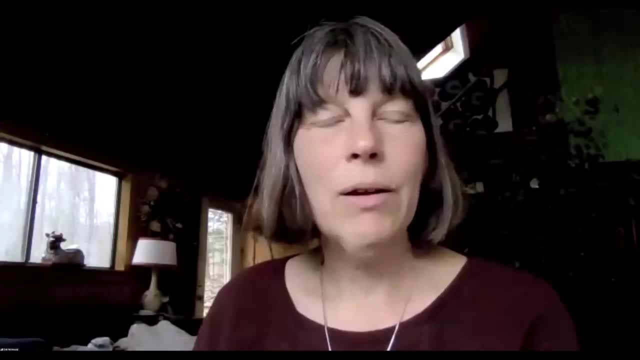 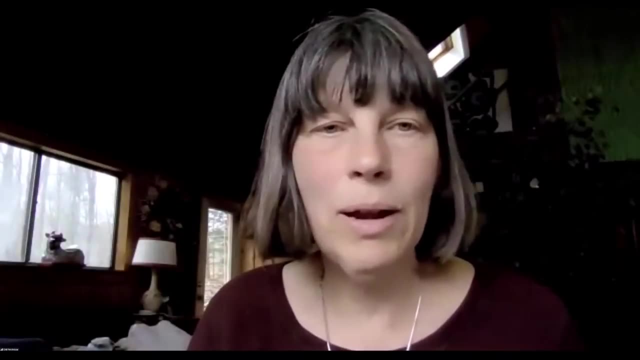 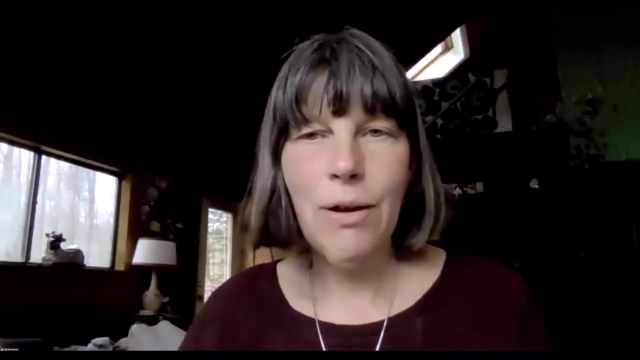 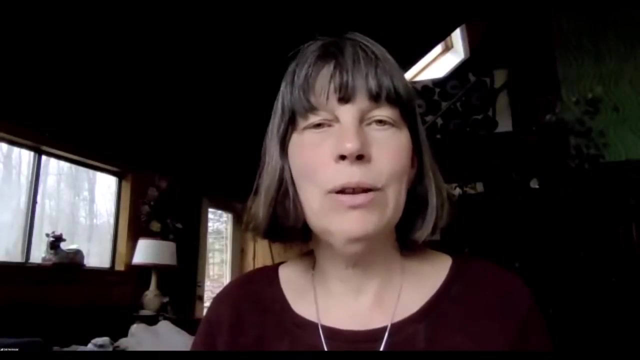 However, what we know is that our gut microbiome And our skin microbiome and our uterine microbiome and all you know, all the microbiomes that exist in our body, even our blood, For for all animals, It regulates our entire system. It produces our brain chemicals, it produces, it produces, you know, regulates our digestion, it regulates immunity, etc. So, if we take something, if we use something in agriculture, 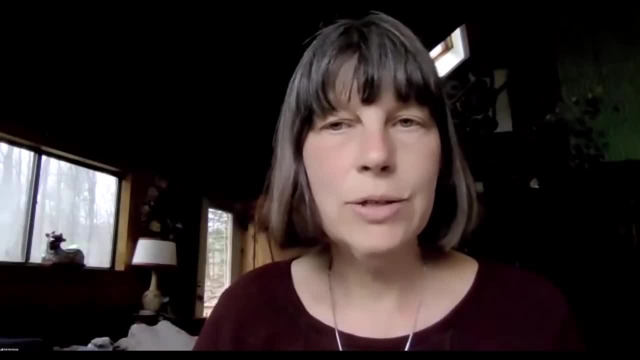 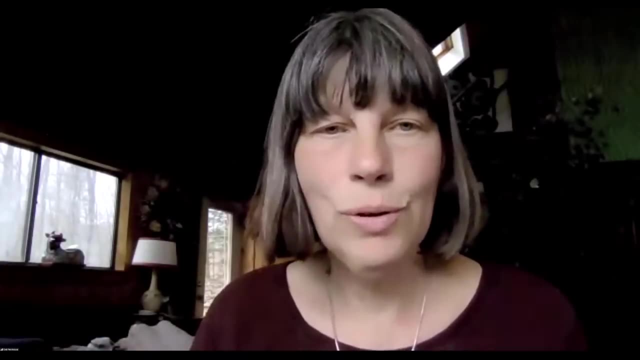 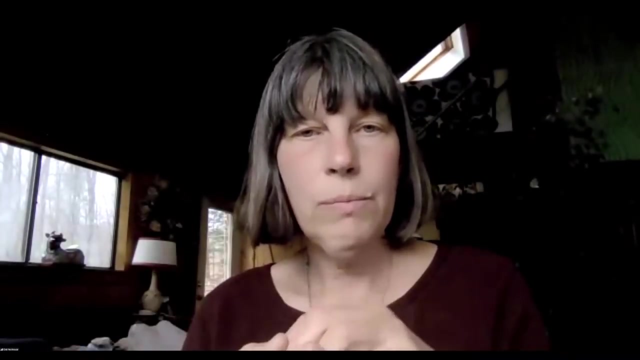 Or even on our lawns. that is an herbicide, That's also a broad spectrum antimicrobial And it's now in our water and in our air and in our food, For not just for us but for all of life. We are disrupting that microbial animal symbiosis. 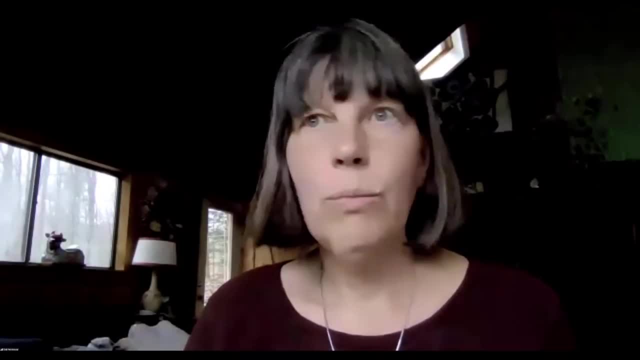 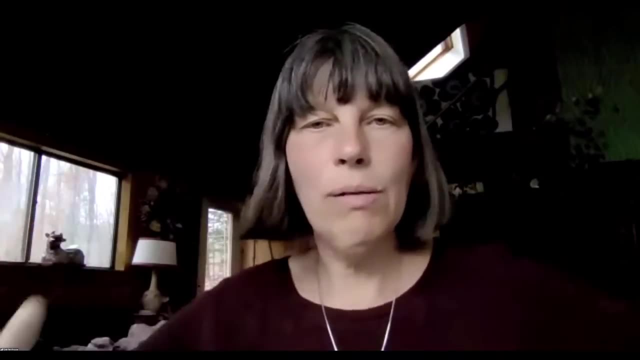 And we're deeply disrupting One of the most basic things that makes us who we are. like we are, we are, we are moving bubble for microbes. That's that's that's how. That's how our whole body works. 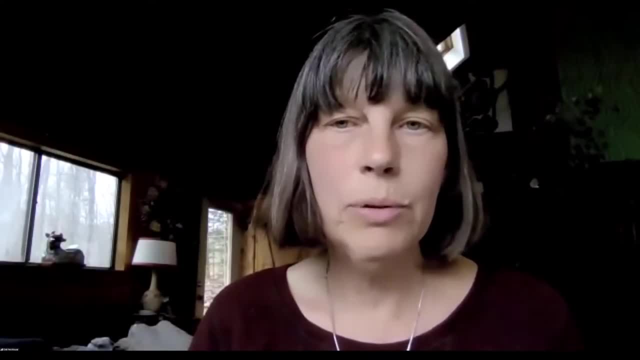 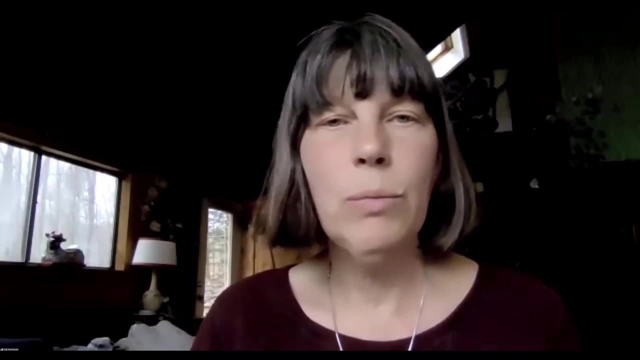 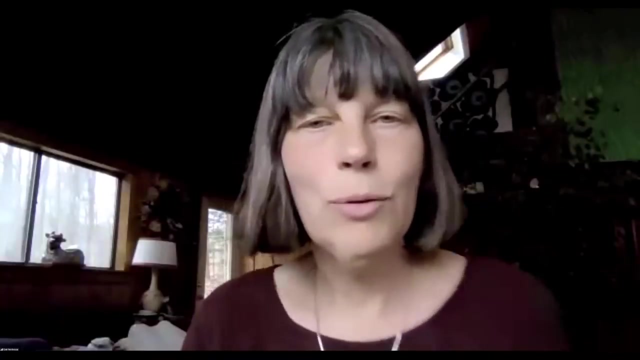 So so that's a very direct link between soil health practices, that that eliminate that particular herbicide, And we know that, that all the other biocides, basically, you know, all the other pesticides, I don't think, I don't think that pests exist. 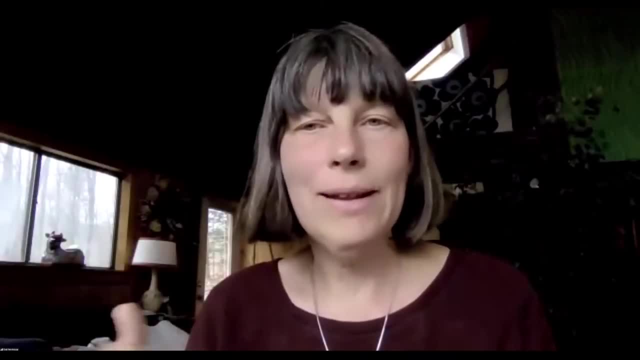 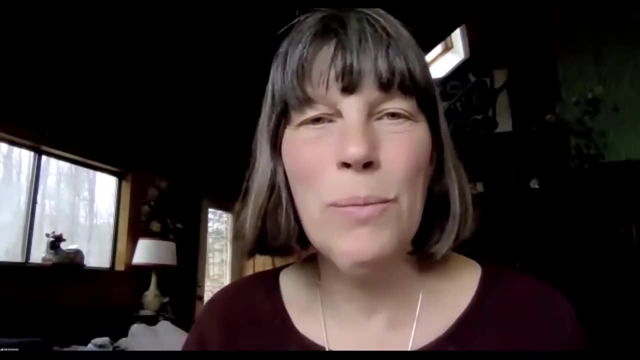 But all the other biocides are killing off something that is part of our whole ecosystem. So fungicides- we have fungi and yeast, et cetera, that live in us too. So so that's that's one direct link. 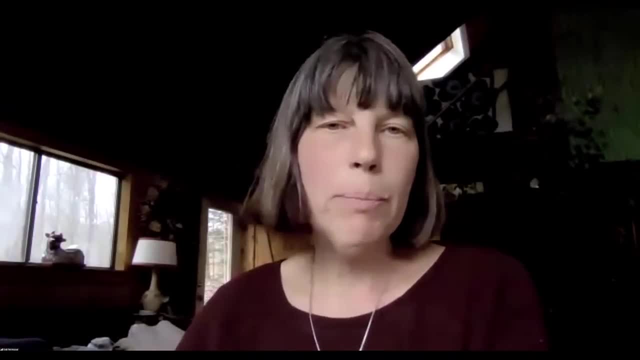 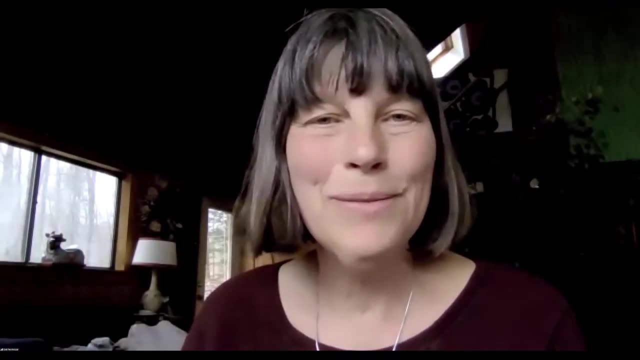 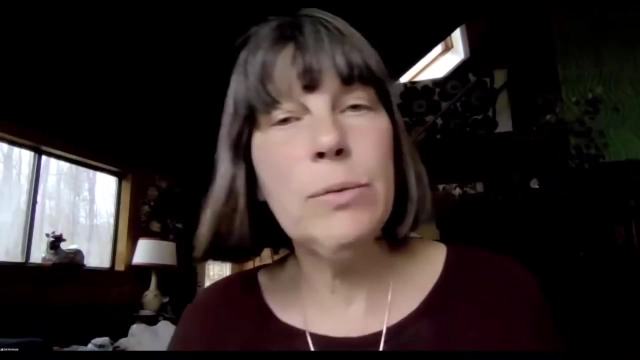 And then there's a lot of research about that. people who grow up on farms or around soil et cetera, playing children who grew up playing in in relatively healthy dirt, have have healthier microbiomes. And we know that taking dewormers, dewormers- So so worms in the body perform a role. They help our immune system from overreacting to things. So yeah, there are a lot of links that may not, may not. people often think, oh, it's just about eating soil, you know, and it's not. it's not quite that direct, but there's a lot of links there. 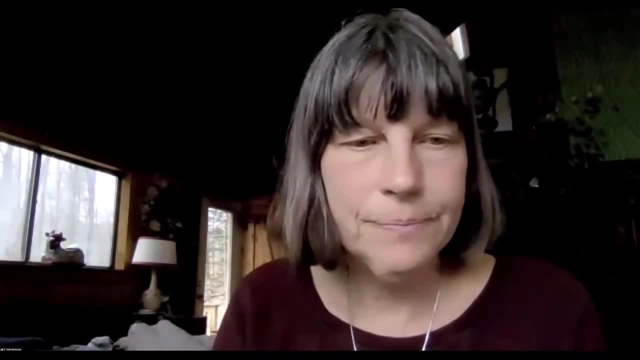 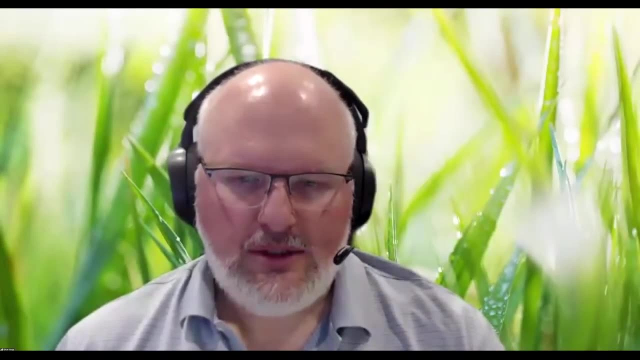 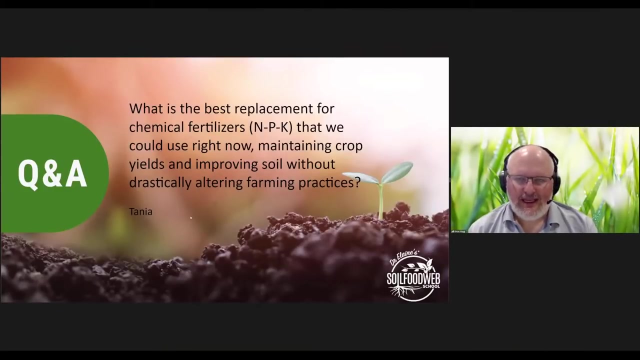 So the ecology of care gets into all of that. Okay, Thank you, panelists. I think we can move on to the next question, Next question. Next question is going to be from Tanya: What is the best replacement for chemical fertilizers- NPK- that we could use right now, maintaining crop yields and improving soil without drastically altering farm practices? 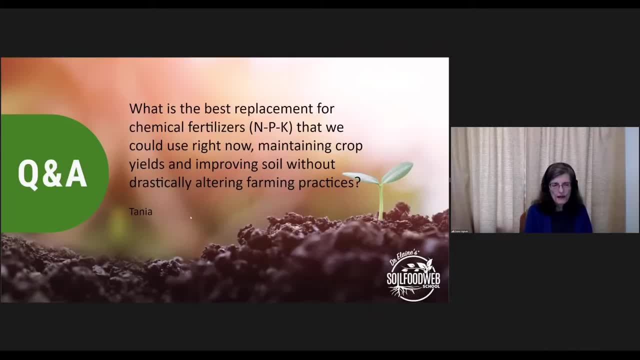 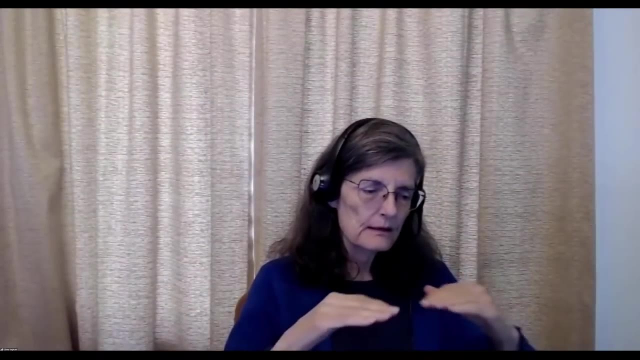 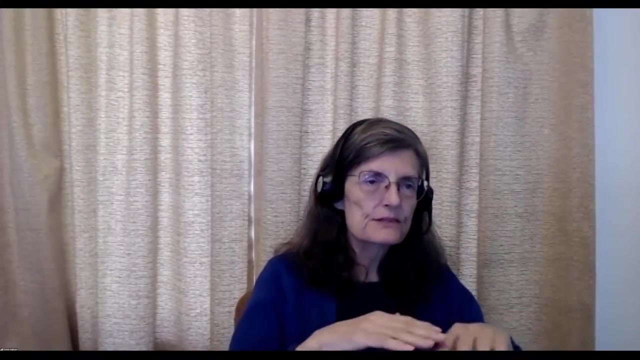 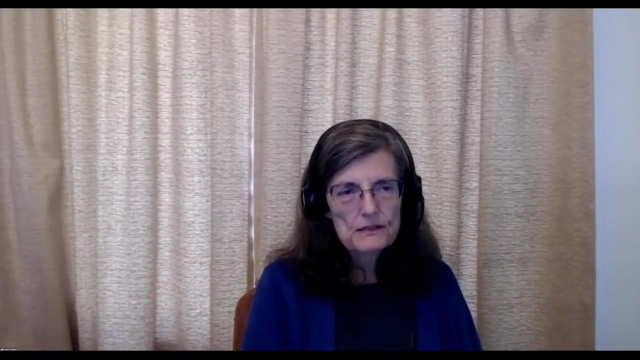 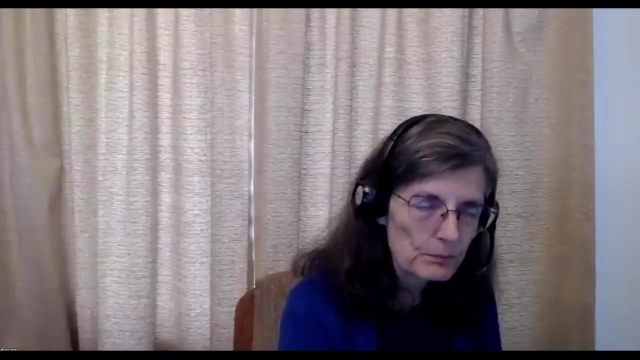 Well, the best replacement for the chemical fertilizers is a well-made compost that has all of the different organism groups that your plant might require. We have We started to develop kind of a rating scale for that compost. We have to have a minimum of this number of bacteria and fungi and protozoa and nematodes, this kind of diversity present in those groups, to know that it's going to be able to deal with all of the needs of your plants. So you've got to have a minimum value of these organisms in your system And then you've got to balance your fungal to bacterial biomass ratio, And it's really pretty easy. You put the appropriate foods in along with the properly made compost. It has to be aerobic. That's a really important aspect. You cannot let it become anaerobic, because these anaerobic conditions are where the disease-causing organisms thrive. So, starting to grow your own compost- Or buy it from somebody locally, that is, you know- has looked at the minimum levels for a biologically complete compost would that would be my suggestion on the way to go. And that means you can delete all of that inorganic fertilizer right from the very beginning. I don't know how many of you have noticed, but inorganic fertilizers have increased in cost by something, like I was told earlier this morning, $800. $800 increase in inorganic fertilizers. Where are all our farmers going to find the money to pay for those inorganic fertilizers to go out? We need to be making compost for these folks. We need to be helping them out by giving them an organic, alternative way of putting fertilizer back in their soil. 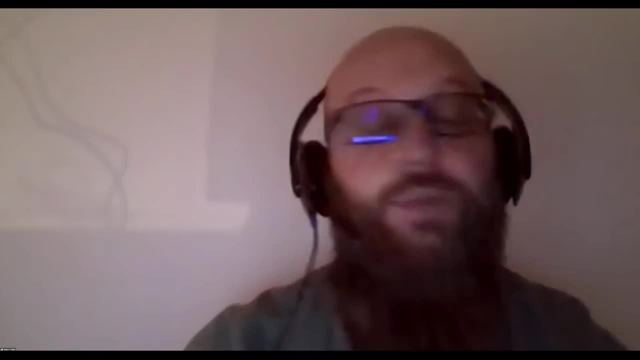 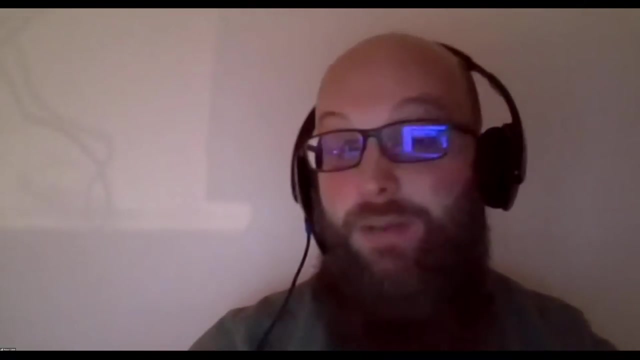 I'm so glad that you have brought that up, Elaine, because it gives me the chance to thank you publicly, as I've done a couple of times, for bringing this knowledge to me at a point in my career when I was desperately looking for such a strong point of leverage. 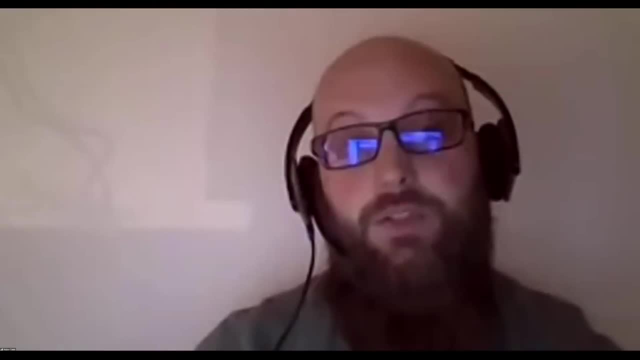 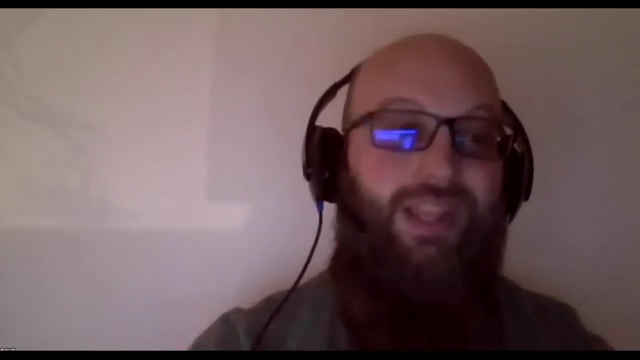 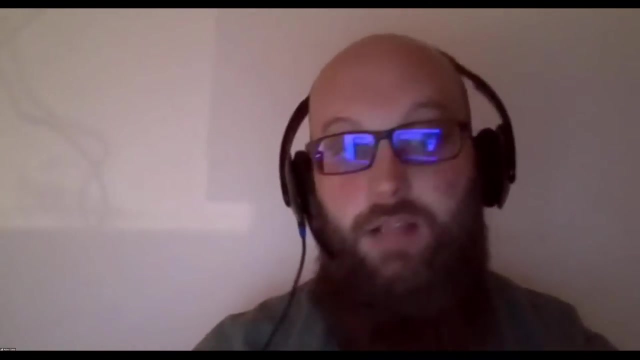 If you look back at the papers I was writing as an academic two or three years ago when I was still a postdoctoral researcher, I was trying to find a way to replace inorganic fertilizers because I saw how devastating they were environmentally in the world, ecologically to the soil. 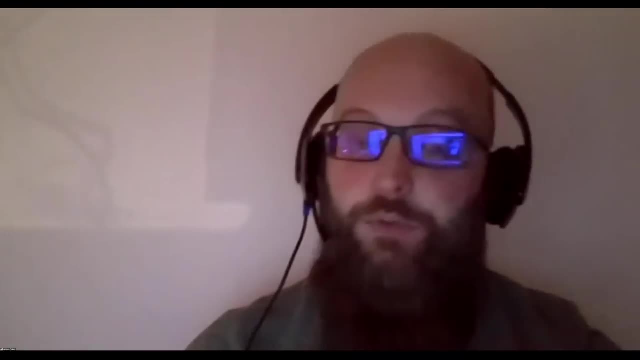 And so with mycorrhizal fungi, with biochar, with worm compost. I was toying around with all these different little mixtures of things. 50% the normal rate of nitrogen, can we get by with that? and looking for the efficiency? 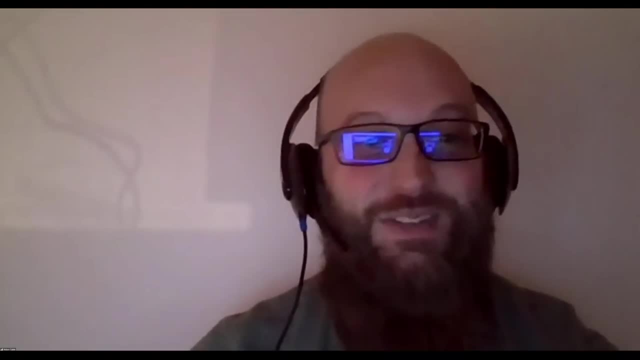 And then seven months ago, when I joined Soil Food Web School and took the foundation courses, I said: aha, this is what I've been looking for for a decade And it's just. it's been awesome to see the way that. 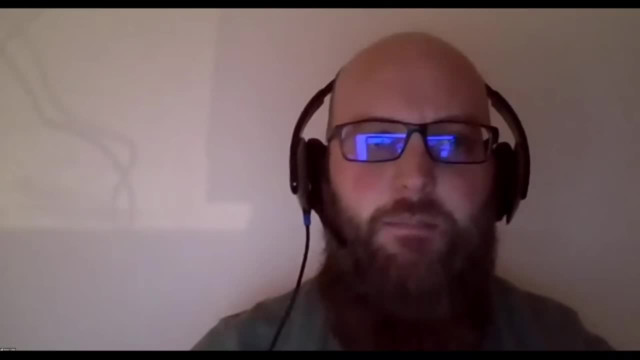 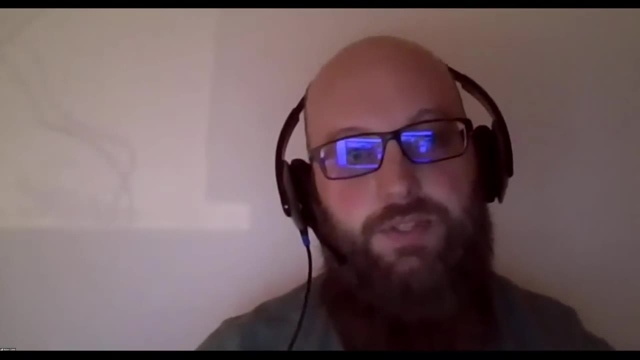 We've had farmers on here like Adam York who have done this on a massive scale and that it's really the foil to that entrenched paradigm from the industrial system that says you have to have agrichemicals, you have to have agrichemicals. 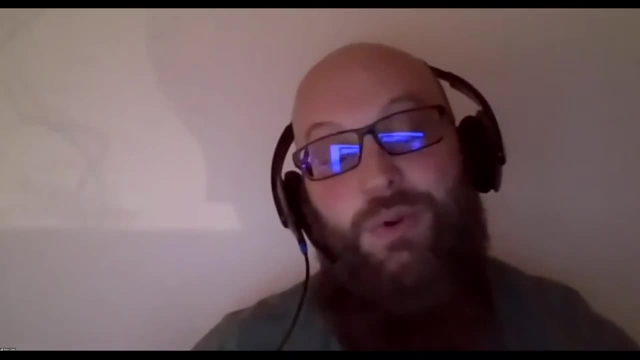 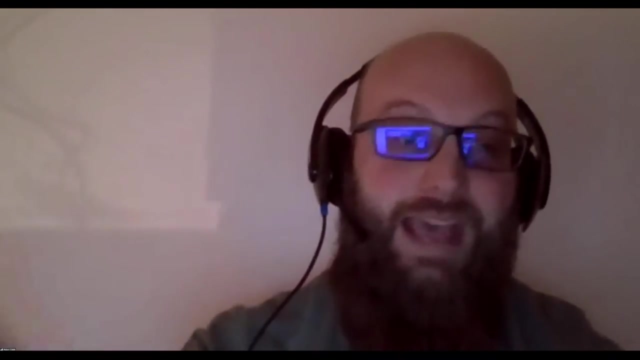 You know, every time I wish every farmer in the world. if I could send out one message is: if you reach for a chemical, think to yourself: how could this be the last time Any chemical on your shelf, How could this be the last time I need this? 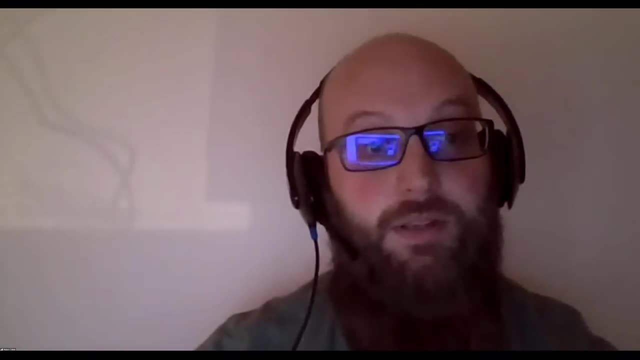 And I fully believe that it's the Soil Food Web and the other principles of regenerative agriculture, agri-ecosystem management that can help them abandon those chemicals forever. Yeah, I'm glad you came in the last with your statement there around management. 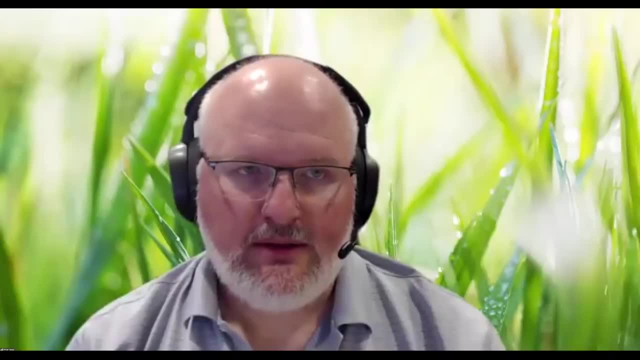 You know, as Elaine mentioned it's. you know, getting that Soil Food Web reestablished back in the soil is really important. We use compost and liquid amendments like teas and extracts and so forth to do that. But the other important thing is the farmers have 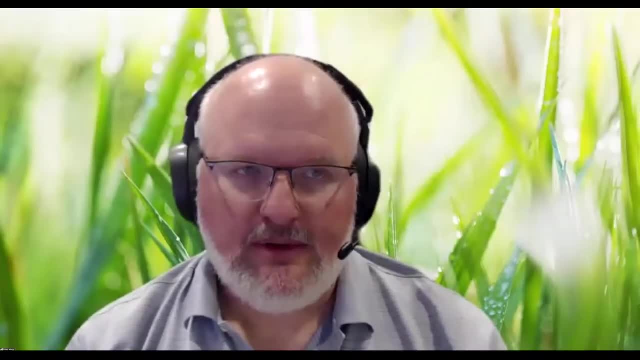 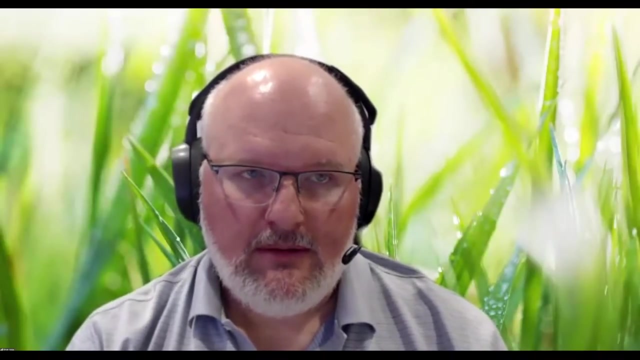 You know they have a significant role in the practices that they do. Tilling is a good example as a management practice that you need to find an alternative for, because you're really going to be interrupting those microorganisms in the soil. You know I tend to go through this exercise with a lot of my clients, which is: let's look at your management practice and identify: are they harming soil biology, are they neutral to it or are they beneficial? 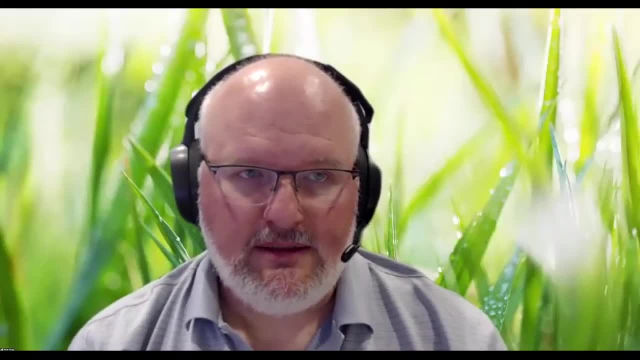 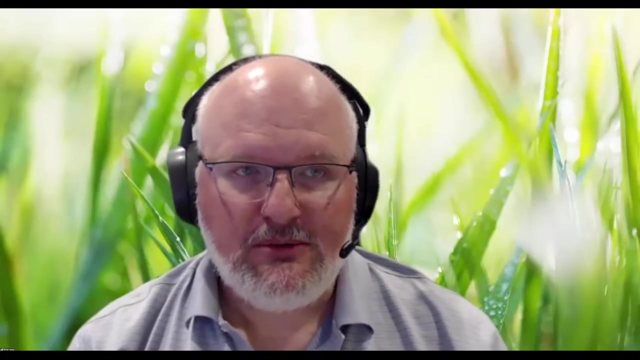 And what we really try to do is prioritize any of those harmful practices to the soil microbiome. how can we find alternatives to those management practices to move it either to a neutral or a beneficial soil microbiome And then, once you do all the harmfuls, then move into the neutrals until you are able to change the management practices that the farmer uses to help support that microbiome in the soil? 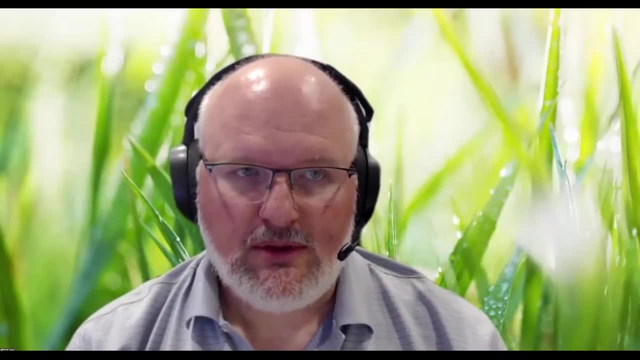 And it's really kind of an educational process you have to go through with your clients as well, with the farmers, the producers. Anybody else want to add on to this question before we move to the next one? Okay, let's move to the next question. 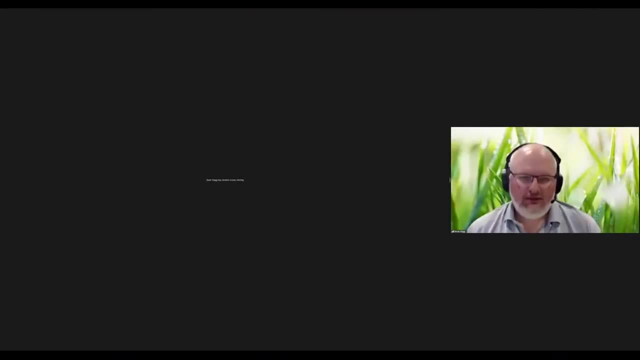 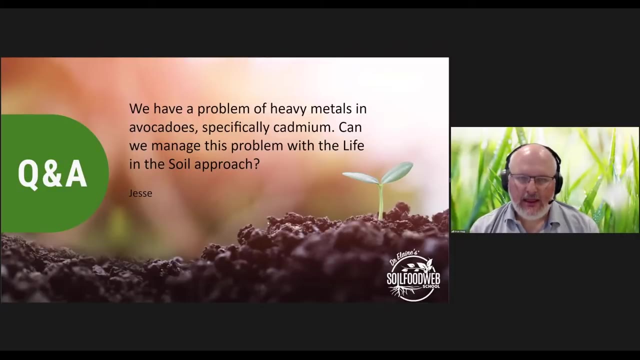 Next question is- This is going to be from Jesse, And Jesse asks: we have a problem of heavy metals in avocados, specifically cadmium. Can we manage this problem with a life in the soil approach? Yeah, sure we can. 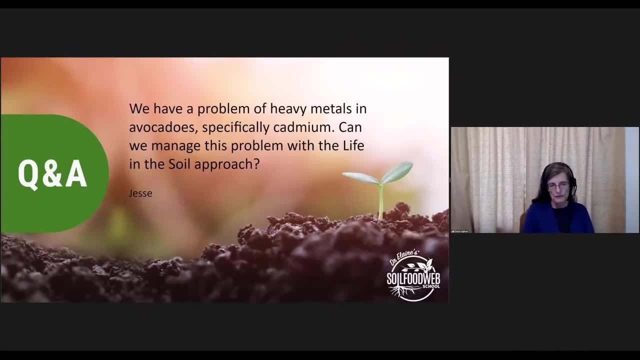 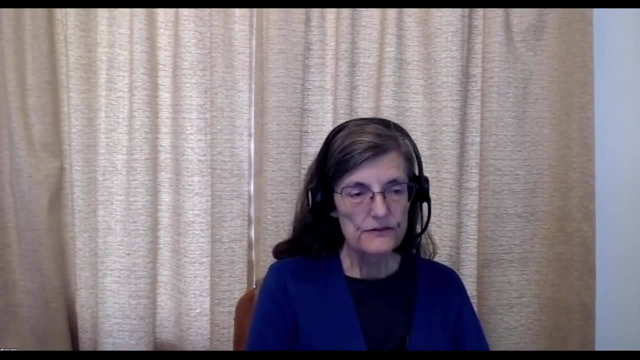 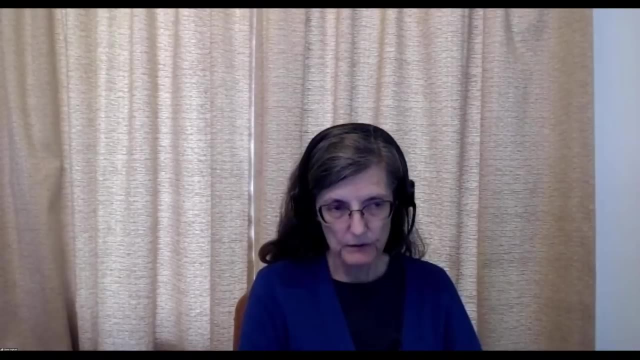 What we've got to do is tie up that cadmium that is present in your soil and put it into a not plant available form. So it would be working with composts. So we get the organisms back into your soil that will put that cadmium back into a biologically viable place. 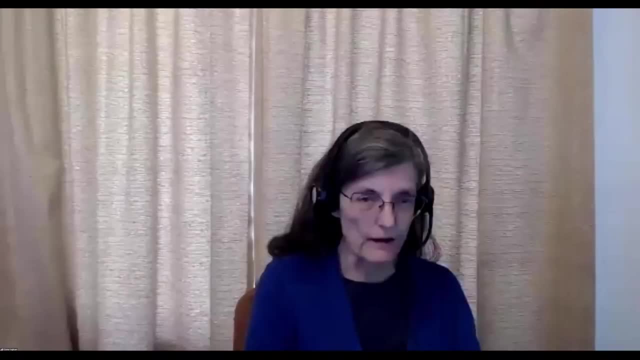 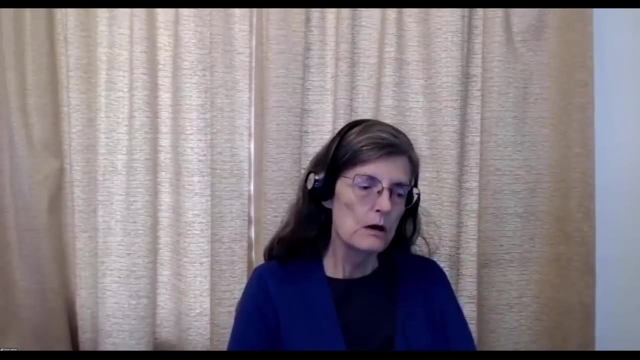 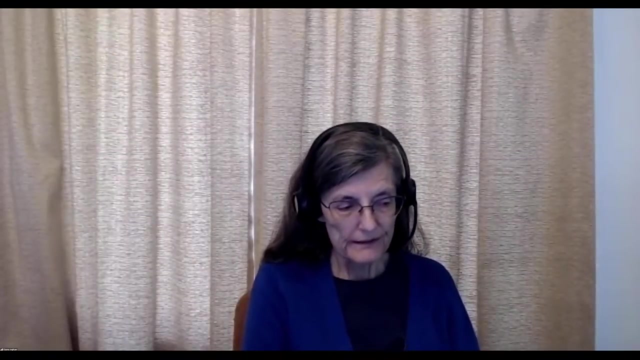 Your plant requires some cadmium, but not a lot. So we don't want to be removing all of the cadmium from the soil, but we have to get it down below a level that is not going to be available to your plant Or it's actually physically removed from the system. 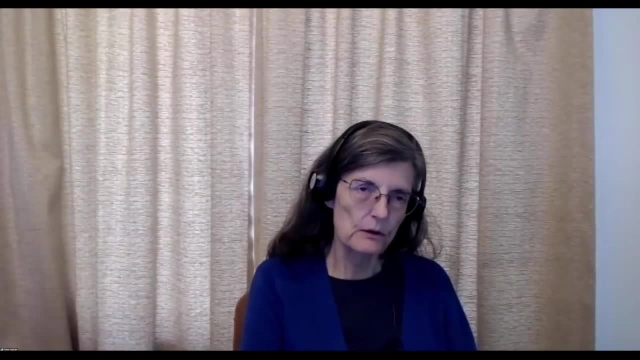 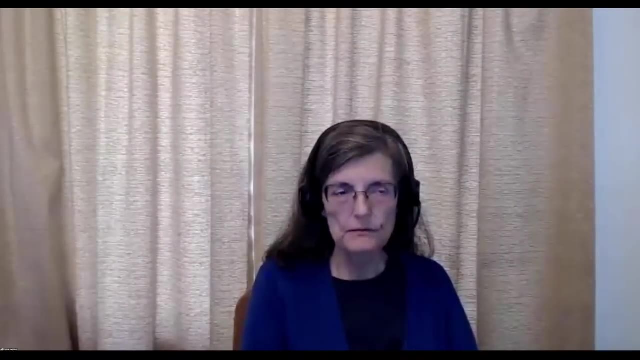 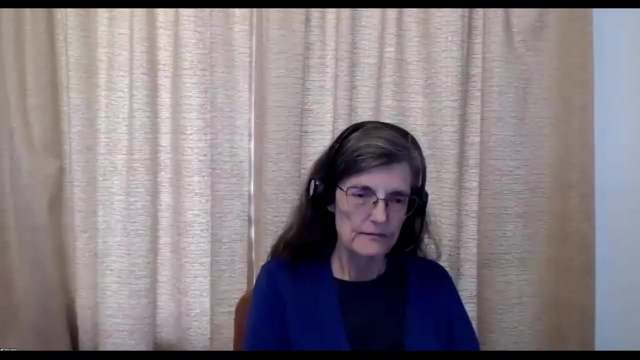 And so we'd have to sit down and chat and talk with you about what the most, what the easiest way is to get things put back into the, get the cadmium put back into the structure of the organic matter. I have nothing else to add. 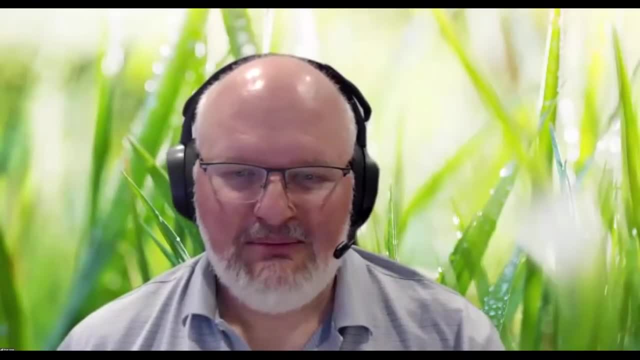 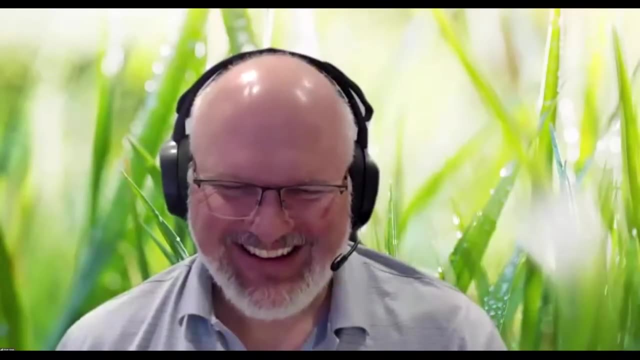 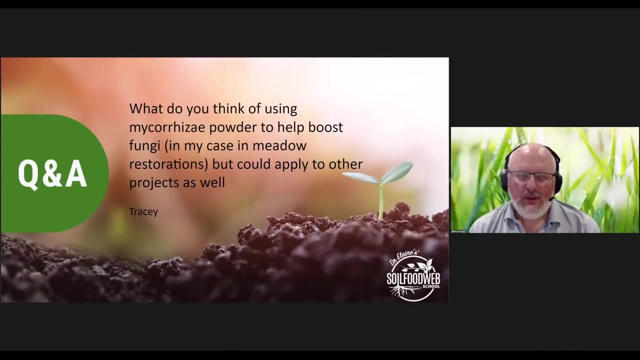 Anybody else? Pretty succinct answer here, Elaine. I didn't know I had it in me. All right, let's go ahead and move on to the next question. So the next question is from Tracy, And Tracy's question is: what do you think of using mycorrhizae powder to help boost fungi, in my case in metal restorations, but could apply to other projects as well. 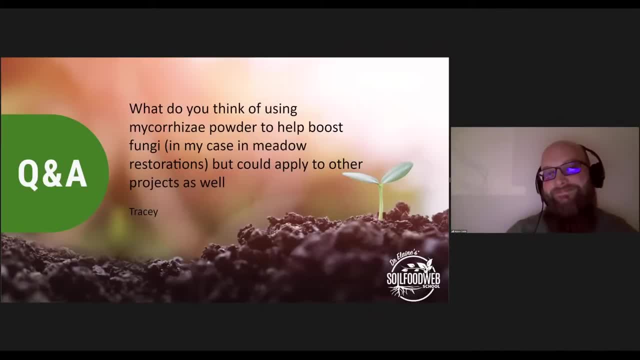 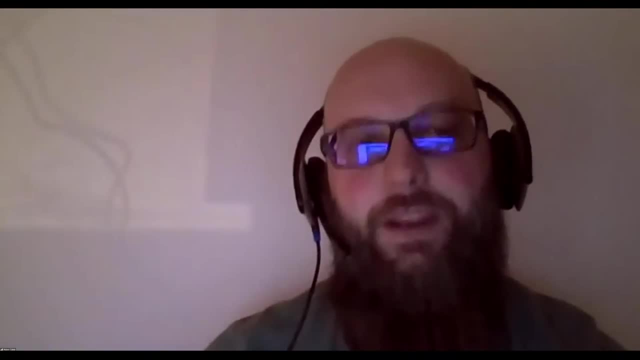 I'd take this one. Oh yeah, I think it's right up your alley there, Adam. Yeah, I've done research into mycorrhizal inoculants- commercially available mycorrhizal inoculants, And I'm very, very skeptical of the claims. In many cases we found no living mycorrhizae. Some researchers have done work and they have not even found mycorrhizal DNA in the products sold as mycorrhizal fungi And we turned those products- in some of them that we assessed- into a soil testing lab and found they had very high amounts of nitrogen and phosphorus in them from some kind of other carrier, say fish meal or something. And so, instead of getting a locally adapted, viable mycorrhizal strain that would partner with your plants- you know where you've paired the soil that you have with the mycorrhizae that have evolved in that soil, You actually could be disrupting the relationship right by putting heavy amounts of something like phosphorus onto the plant early in its growing cycle, so that the plant doesn't signal: hey, I need some mycorrhizae here. 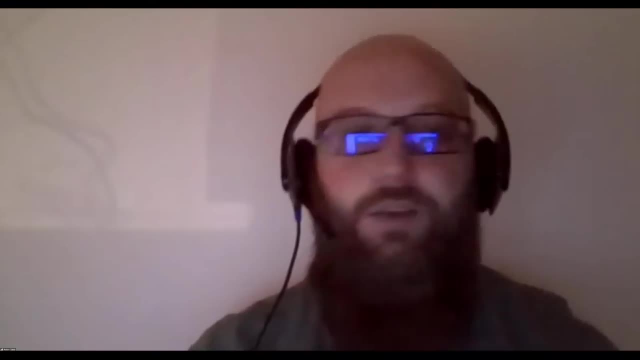 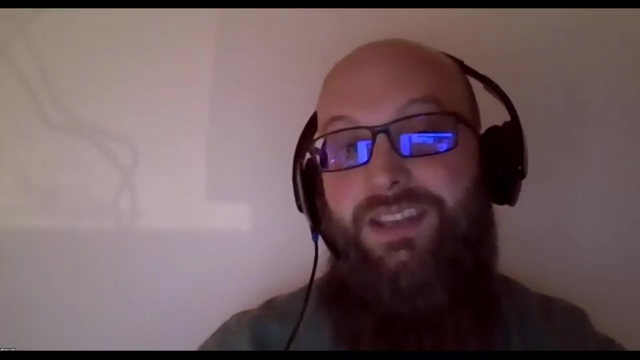 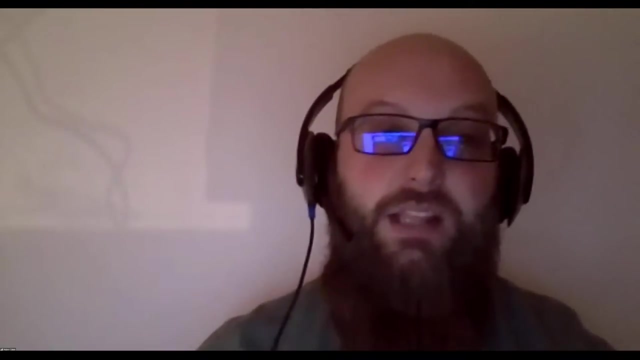 I'm looking for some help getting a little zinc or getting a little, You know, water out of the soil system. instead it's it's shutting down that communication, that chemical dialogue, when you have high rates of something like phosphorus. so it's just a very unregulated market, and I've used this metaphor before, maybe on another webinar. but if we think about you know, if your goal is to say, oh, we want to increase. you know something? in the Serengeti, let's put out millions of poodles in the Serengeti. Let's put out millions of poodles in the Serengeti. Well, you'd have a bunch of poodles in the Serengeti for like a week and then they would all get eaten. And if you put out these non-local mycorrhizae, one of the things that could happen is that they could die out. Another thing that could happen is that they could become invasive in that system, right? We just don't know the long-term effects. and you know, sometimes I see where one region is producing mycorrhizal inoculant. It's a commercial product, say in the Pacific Northwest, where I live, and farmers are using that in Oklahoma, farmers are using that in Florida, farmers are using that in Connecticut and I'm like that's probably not the same kinds of mycorrhizae that should be in those places, especially not in terms of their genetics. 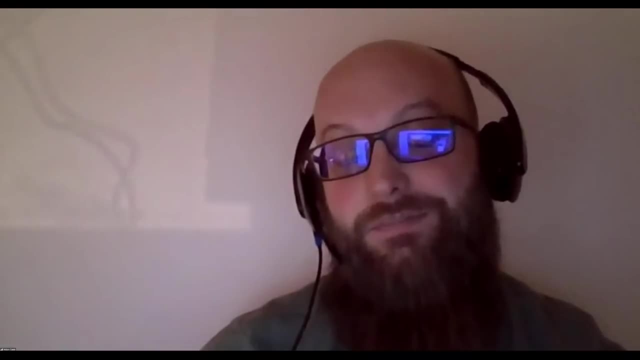 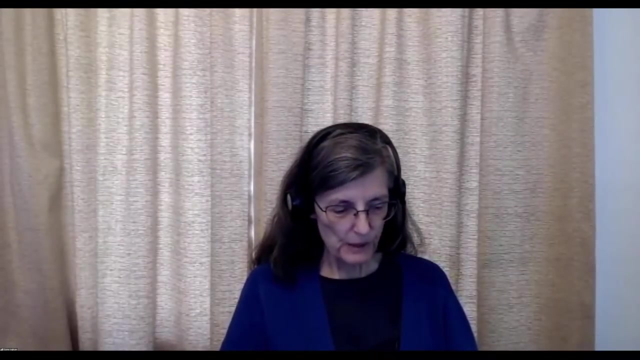 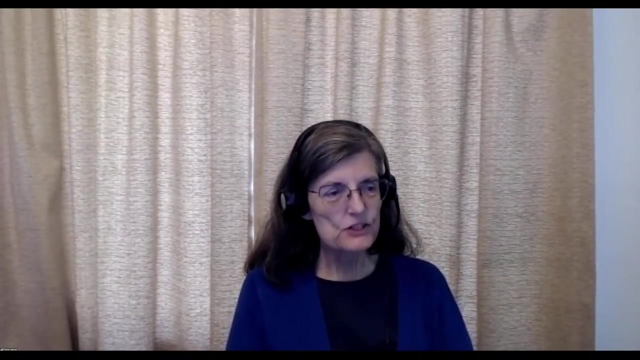 So I'd very much like to turn people away from that idea. Yeah, that's why we like to make the compost. We make sure that we're going to use locally so that all the starting material comes in, with the indigenous sets of organisms. We make sure the conditions in that composting process are going to select the beneficials and against the diseases and pests and problems. So it's not that difficult to get these organisms back into your soil. if you are paying attention to the soil, Yeah, I think. 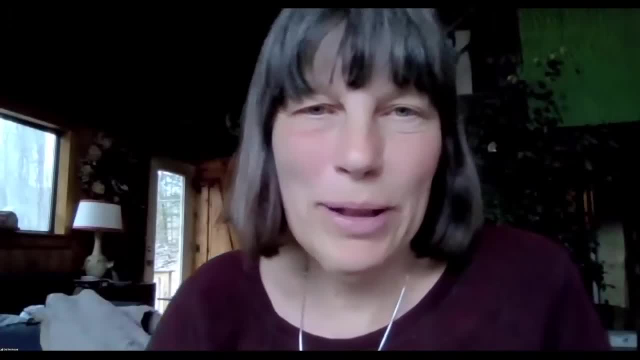 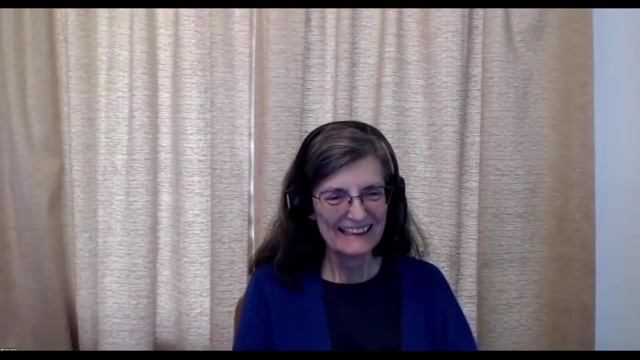 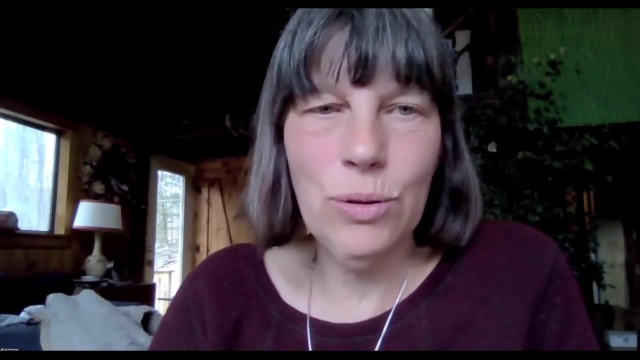 I love that example of putting a poodle out. The mental image- You know that's another thing- is just like with probiotics. I mean, as soon as someone figures out that there's something that could be patented and sold, it will happen. 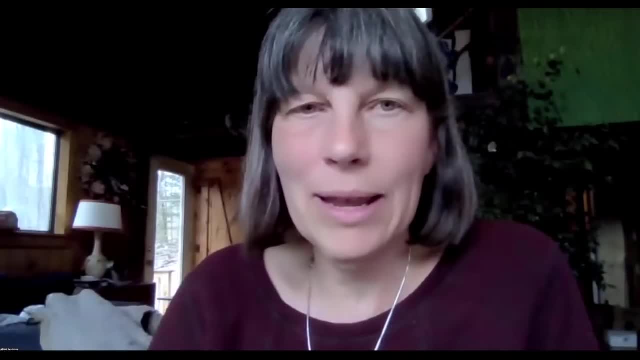 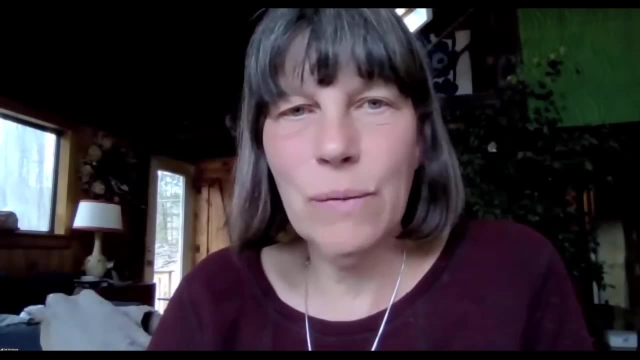 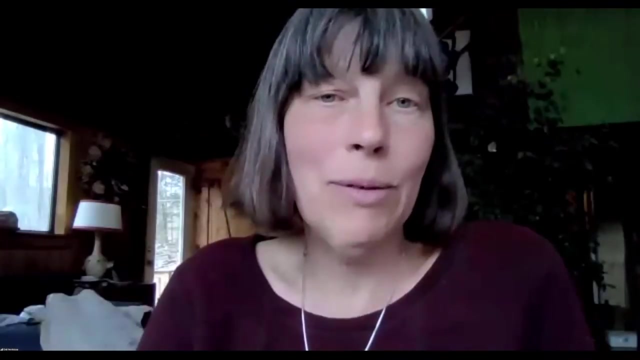 And most people don't think like: well, where can I get this? You know, where can I? Where where would this be happening? naturally in my food system or in my land. So we just always have to keep an eye out for that, that extractive paradigm that creeps in everywhere, because everybody's you know kind of societies are collapse. 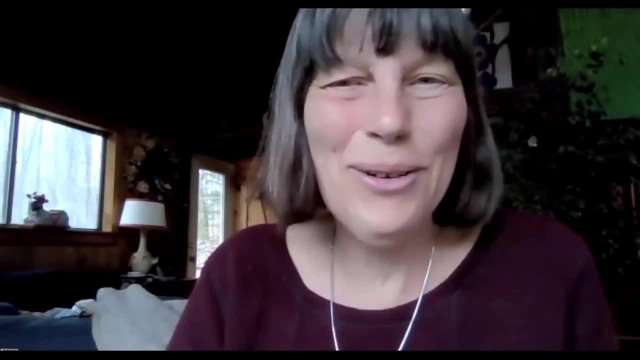 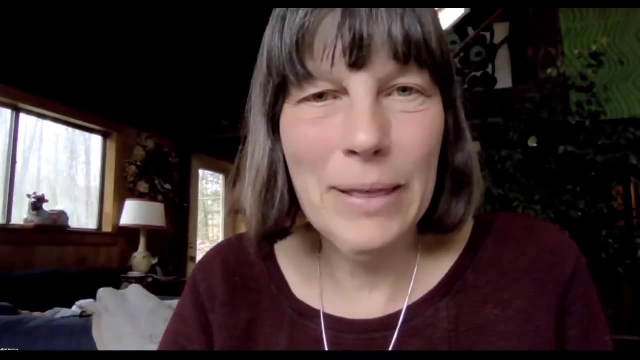 Capitalism are kind of an end stage, And so everybody needs money and and everyone's trying to figure out how to make things work. So but but I think there are better ways. Well, you know there's There's a whole movement about going local. 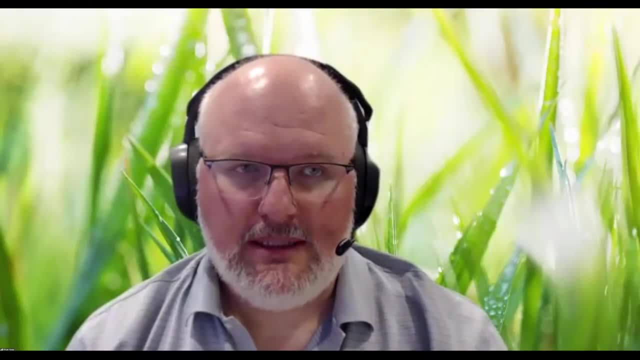 And this really particularly applies to the work that we do. You know, as Elaine mentioned indigenous microorganisms and Adam you mentioned as well, the indigenous microorganisms are would have, of you know, evolved over the eons in that particular bio climate to be able to thrive for the plants that are growing in. 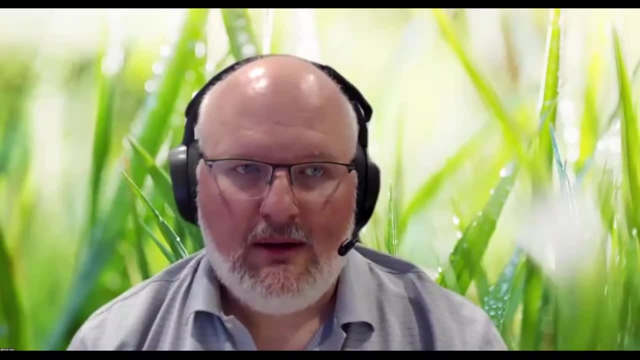 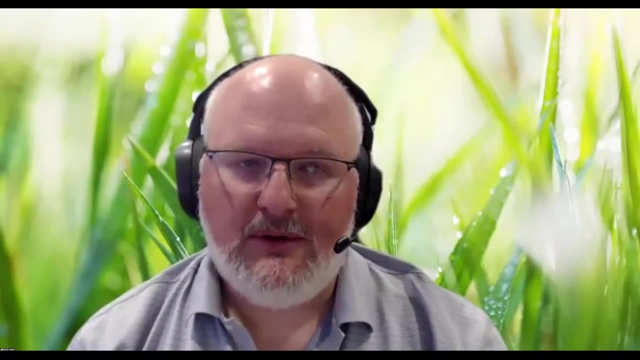 those systems And you know, I think there is going to be a lot of movement towards creating these hubs of making compost- you know, on farm compost- and making, you know, liquid amendments. They're going to be servicing the local area. 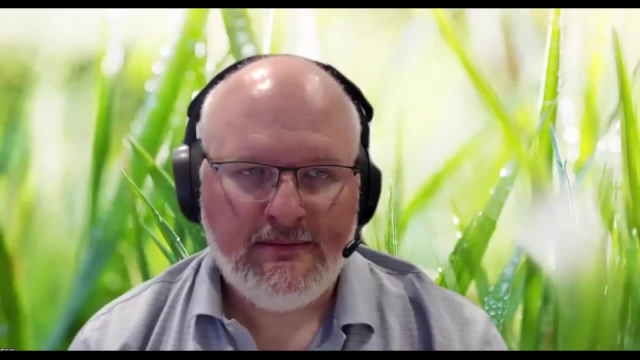 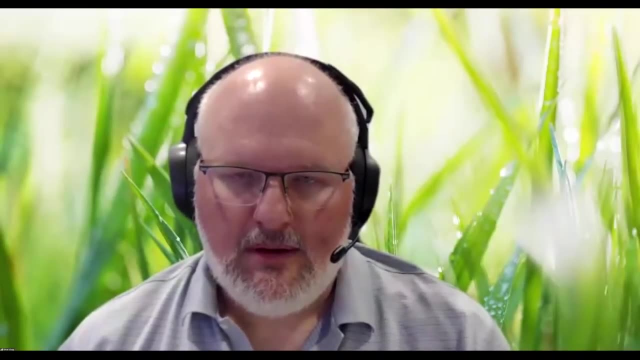 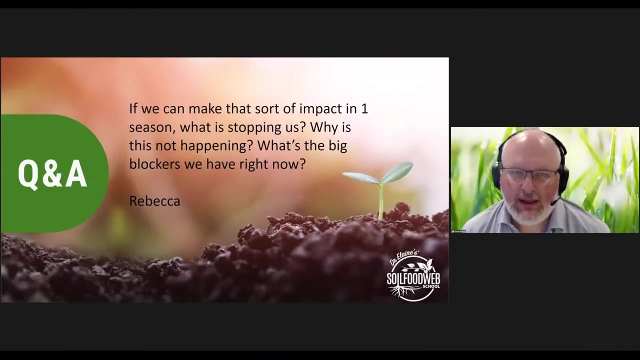 That's really where I think this is moving towards in the agricultural space. OK, any other comments before we move on to the next question? All right, I love this next question. this question is for Rebecca. if we can make that sort of impact in one season, what is stopping us? 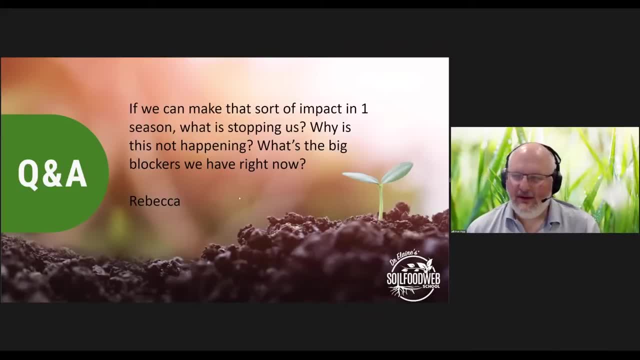 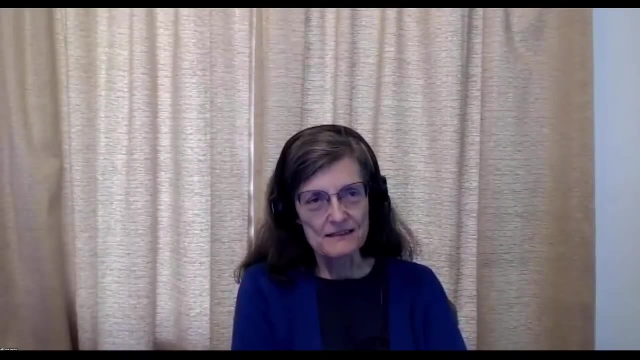 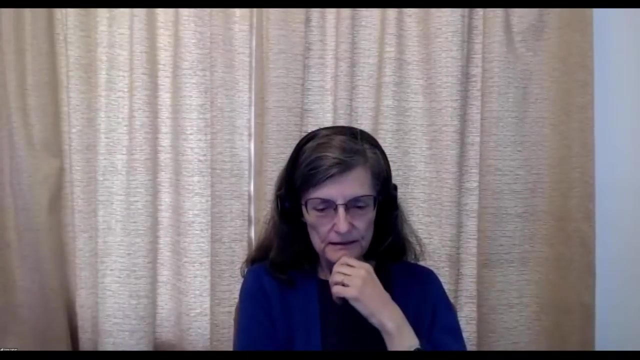 Why is this not happening? What is the big blockers we have right now? What say you panelists? Uh, don't get me started, It's uh, you know, you go to grower meetings and give a presentation of all of the benefits that could come from giving getting the right sets of microorganisms. 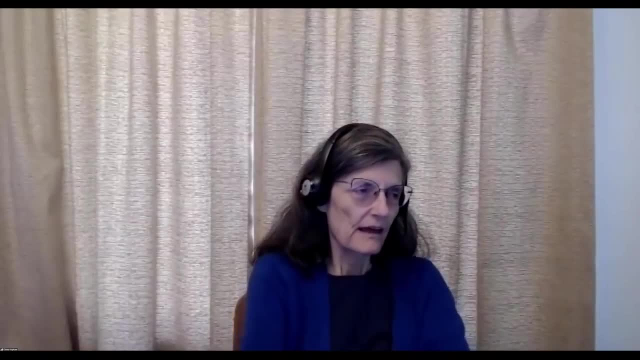 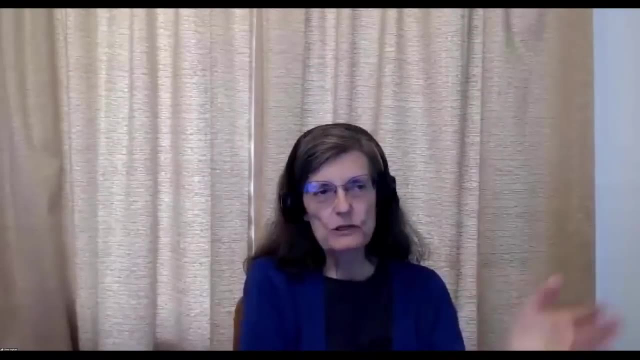 And you know, the first thing you hear when you're at the coffee break is: you know that woman's crazy. She just doesn't know what she's talking about. If it, if it, Actually, if what she was talking about actually worked, then we'd already be doing it. 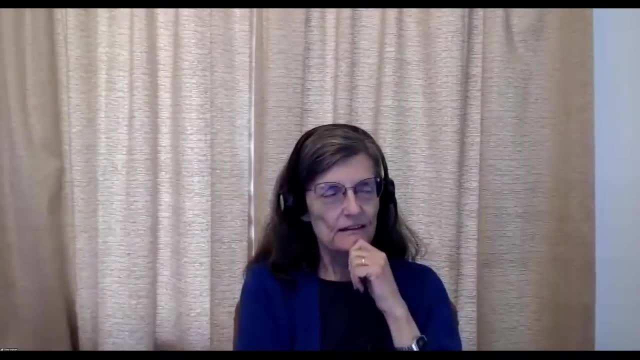 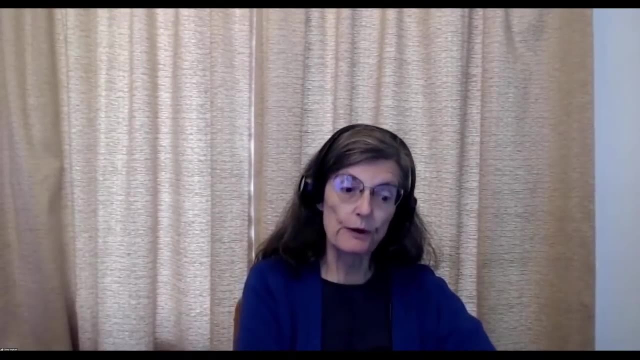 And it's just an aggravating thing that at least we're having a lot more, a lot of success, because people are actually following directions now and getting their compost made properly so that they have only the beneficials present and you're aiming things for the specific plants. 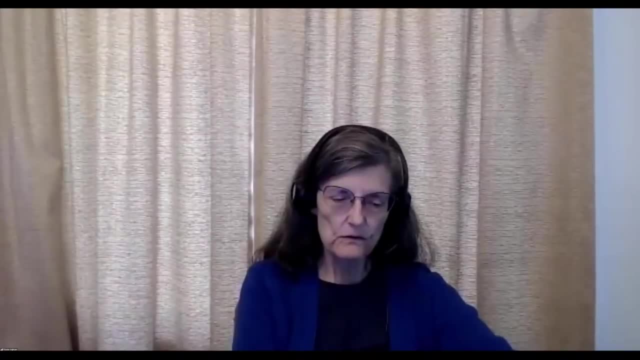 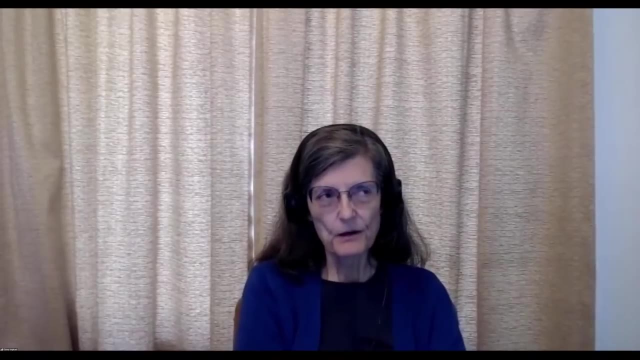 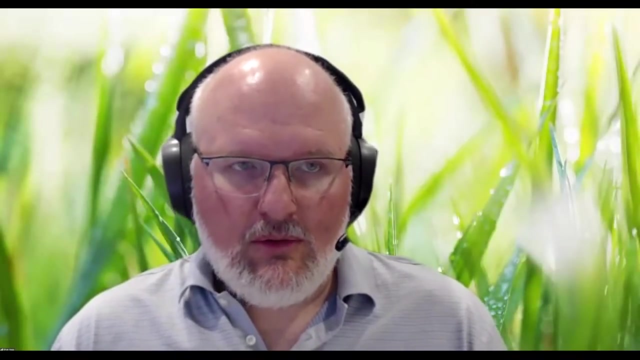 It's that you're growing, so you're optimizing your soil for that crop in that place. So I think the chemical companies are still a huge problem. This is something I see all the time. Um, you know that. you know a grower is some producer. 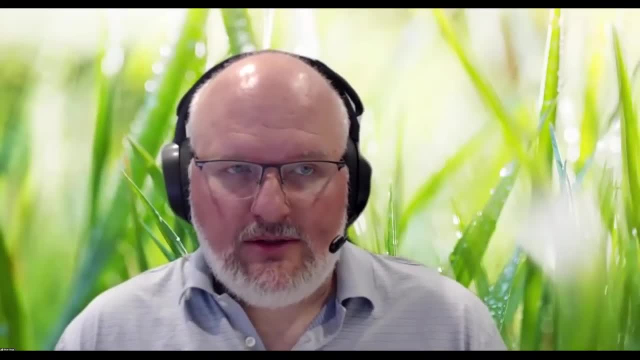 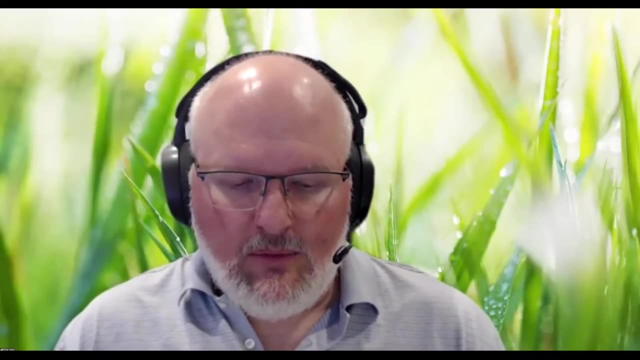 They typically have a lot of different what they would consider trusted advisors- This comes from the university, the extensions, their PCAs, their fertilizer salesman, I mean. the list goes on and on and on, And Yeah, And the farmer knows. hey look, I can see the writing on the wall. 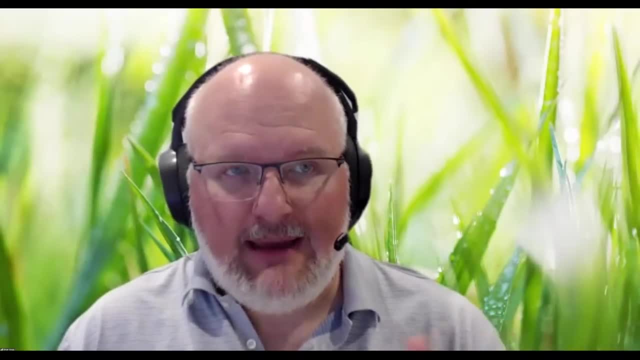 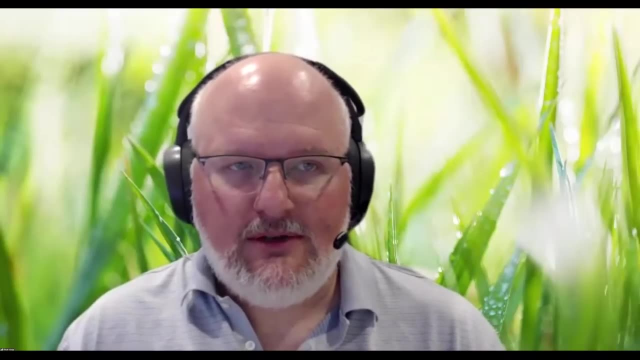 You know I'm going into negative territory. This is something I have to make a change in my farm. The people that are supporting them sometimes are very resistant to that change, And so they're hearing a lot of different voices, And so for a lot of these producers they want to kind of dip their toe into it, which that's OK. 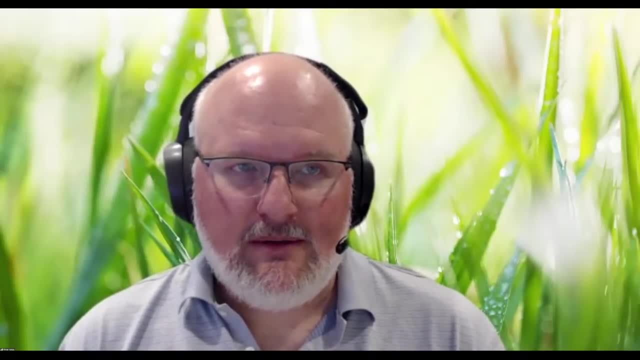 I'll take a farm that's willing to do a trial and you know I'll tell them: give me your worst block, give me the bad, the worst performing area that you've got And let's go ahead and tackle that and try to make those changes. 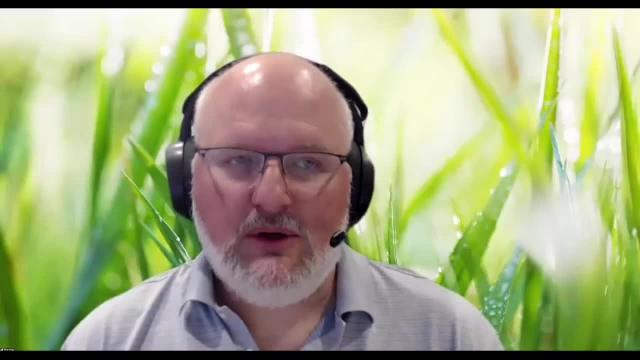 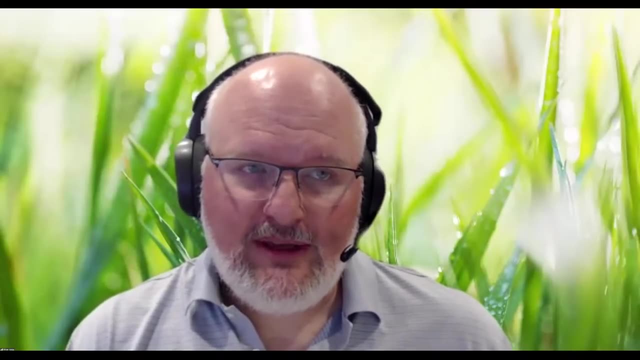 And so they can see firsthand, you know, how these systems can work and what it's going to take to actually do this, this kind of work, And then that starts to make the changes. And then I also see that once farmers become successful, their neighbors start to pay attention. 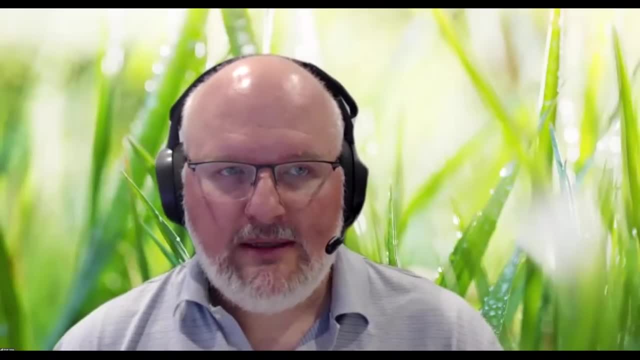 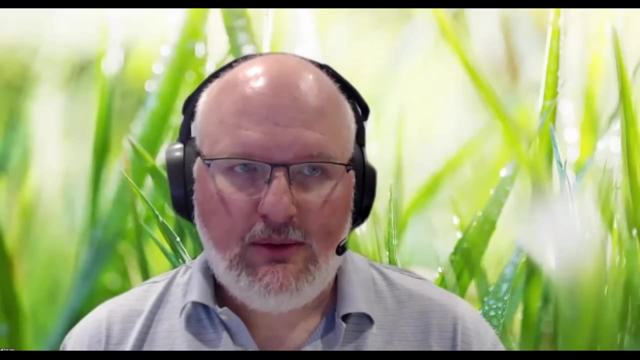 The resistance becomes less and it starts that momentum shift. So it's just going to take, I think, having a number of those farmers being pioneers, going out there making those changes, Everybody else is going to start to pay attention And then we'll see that ball rolling. 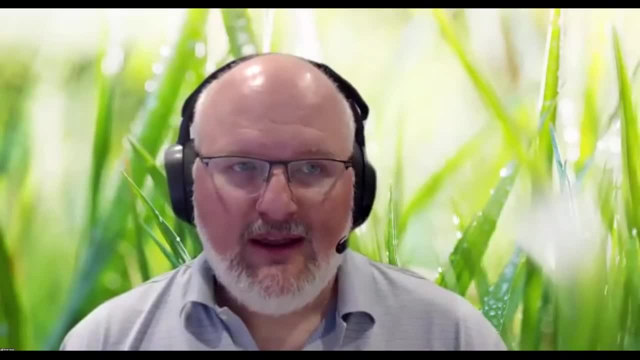 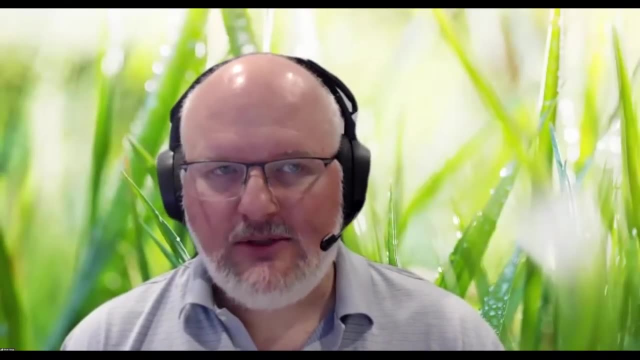 And that's really kind of what's happening right now in the field. I'm seeing a lot of hey. I'm a neighbor of so-and-so where I've talked to this farmer and he's had some success. Tell me more, Right. And that's where I think the big change is going to make. 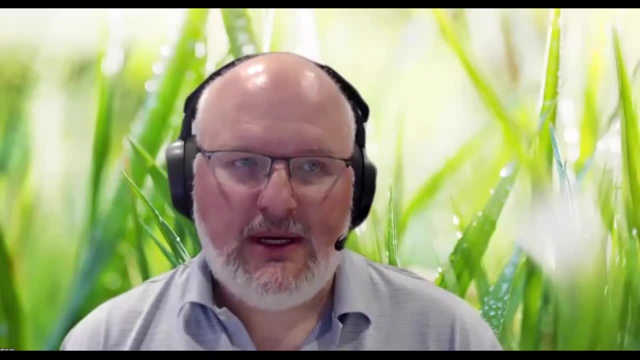 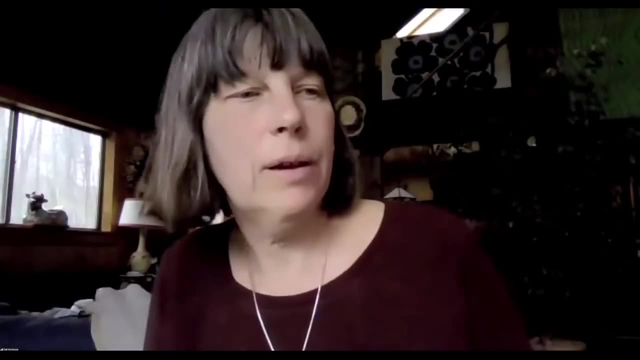 And then once we get that, then I think it'd be a much quicker adoption of these practices and we'll be able to convert a lot more land a lot faster. One of the things that I hear a lot in the United States is what people call the coffee shop. 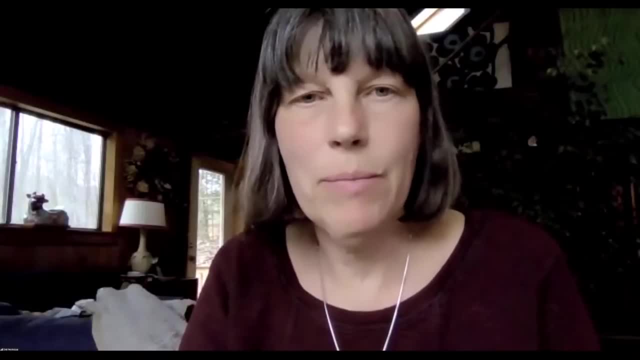 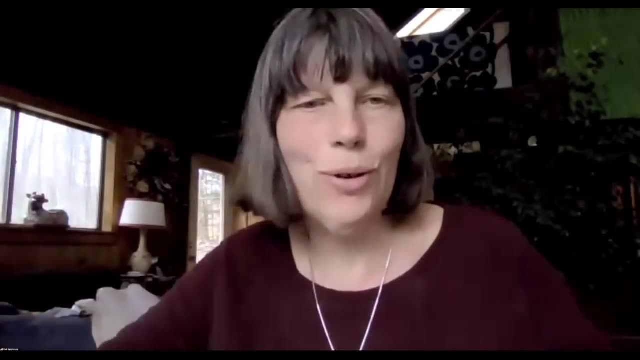 It's a conversation where kind of like what Elaine was describing, But for farmers you know they've made a change, They've planted maybe a diverse cover crop. So there's all these things there that aren't corn or soy and they go into the coffee shop and everybody starts talking about them very rudely. 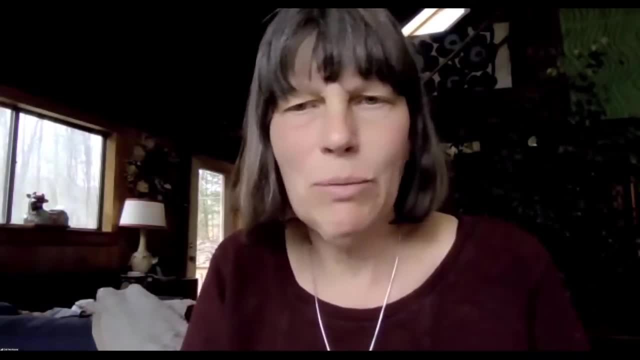 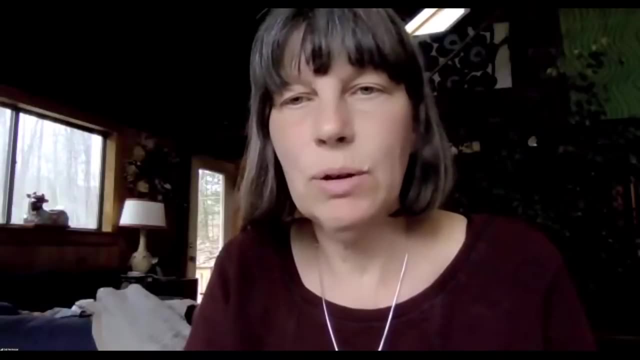 And I'm saying, oh, look at that, You know they're so messy And what do they think they're doing? Who do they think they are? And especially in small rural communities, those relationships are really important And so 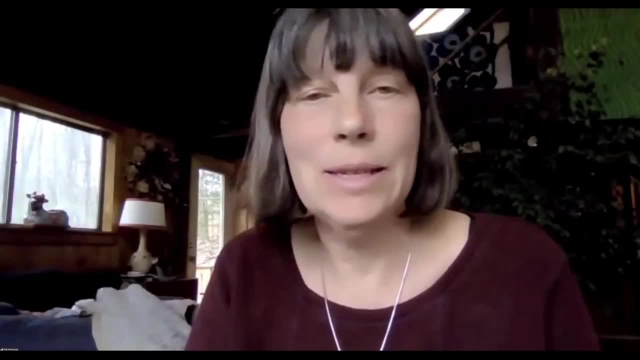 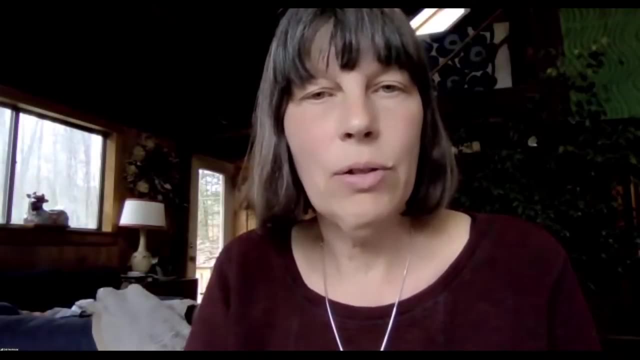 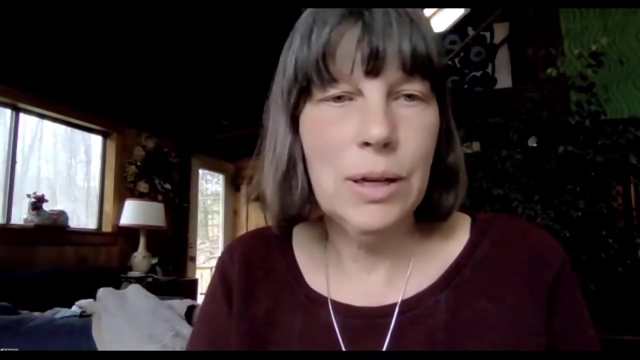 Figuring out ways. for me, I think one of the key things that has made this work in India and that is working in other places is people who have figured out how to have a long term learning network, a long term learning community of people who can support each other, are interested in listening to each other and can define their own questions and figure out ways to research them. 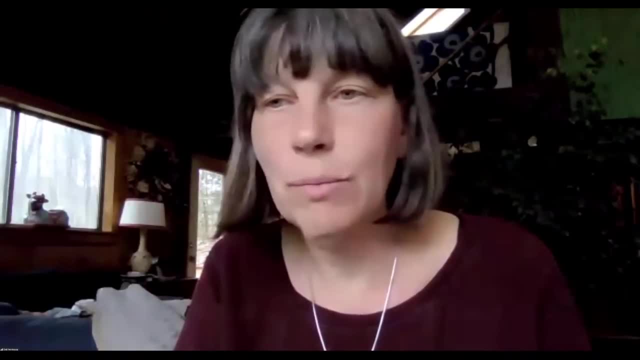 That's what the farmer field school approach is, which isn't used much in the US, but is used in many other parts. That's what the farmer field school approach is, which isn't used much in the US, but is used in many other parts of the world. 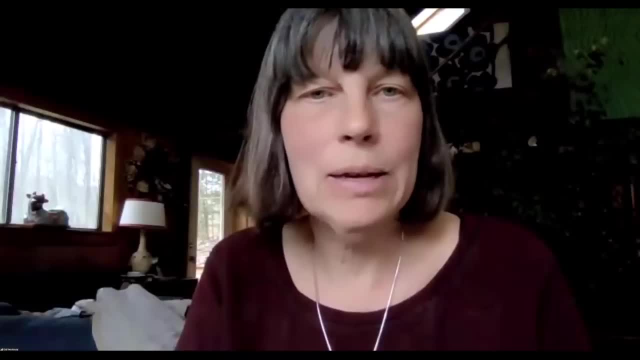 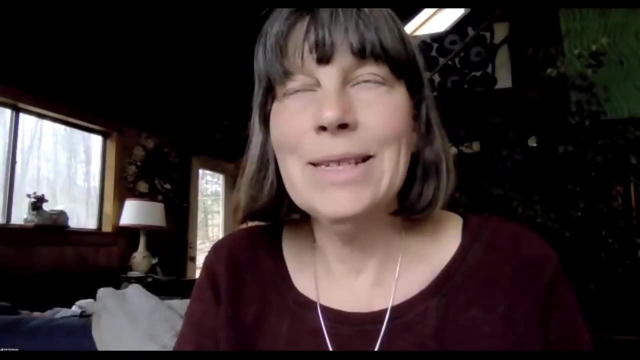 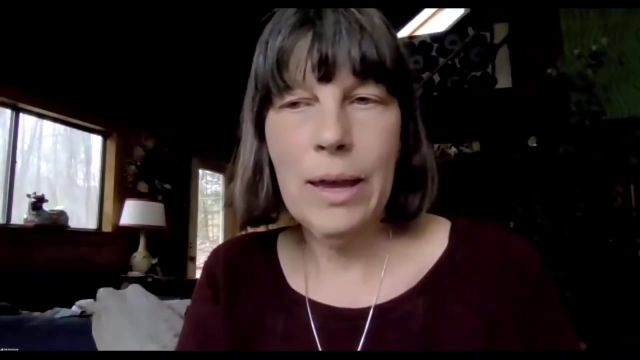 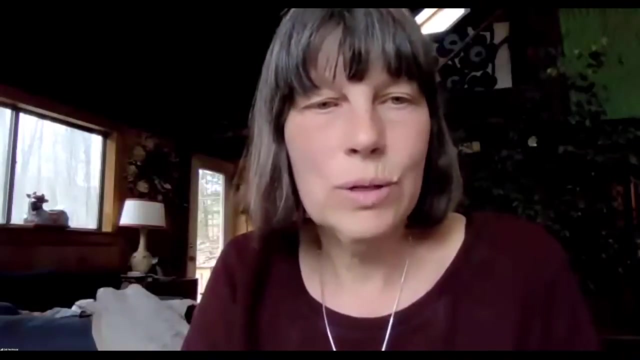 And holistic management support groups do that. At Landon Leadership we're working on long term, long term communities of learning. That's part of what that does is it breaks us out of that paradigm of relying on experts, as if somebody who's over here, who's not working with your farm, knows about you know, knows more than you do about your farm. 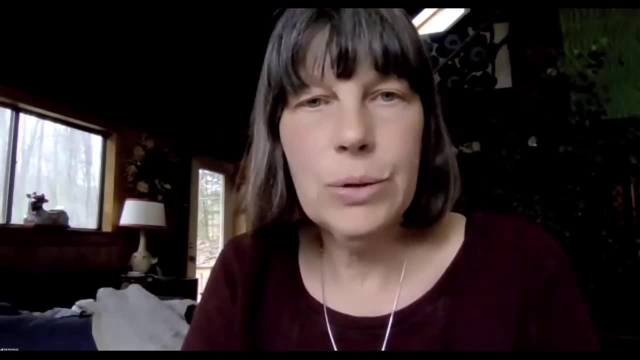 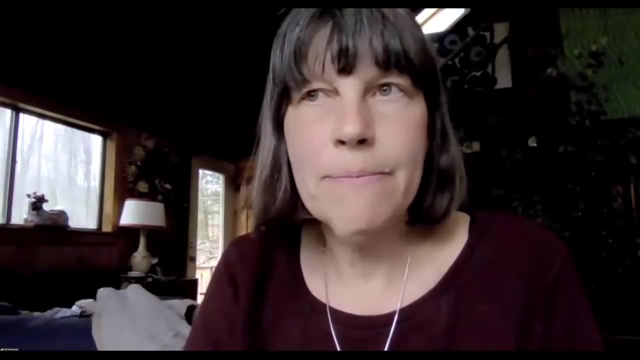 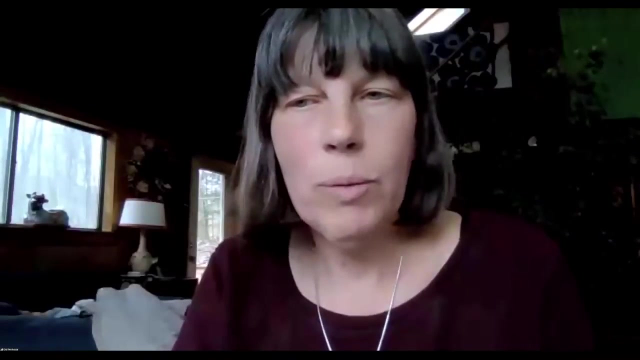 Or about your area Or your context. So I think I think a lot of this is about building strong relationships between people so that they feel more supported in their innovation. They know that if things- you know something- doesn't work out, they have people to talk to about it. 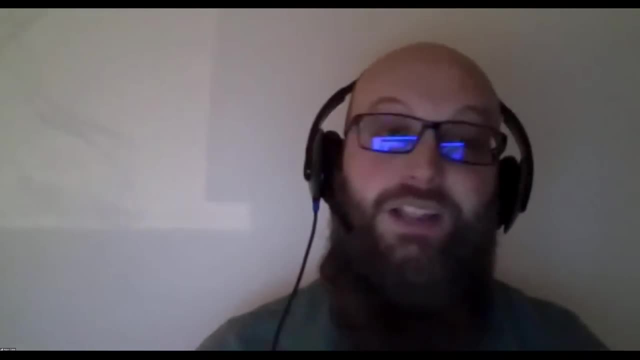 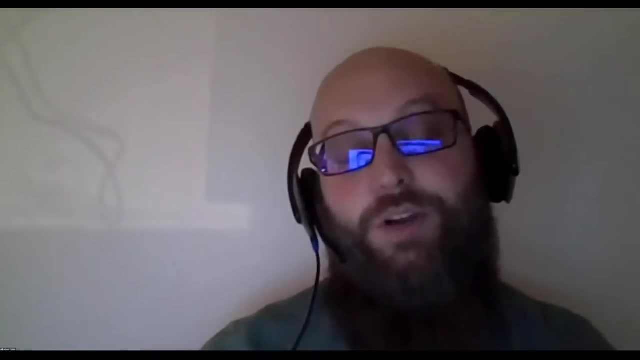 Oh, I'm so glad you brought that up, Didi, And it's like something I love as well to see those farmer to farmer sharing situations. Stefan, I don't want to get you in trouble, But I'm so curious if you've presented your research to traditional animal science professors at land-grant institutions and what their reaction was. 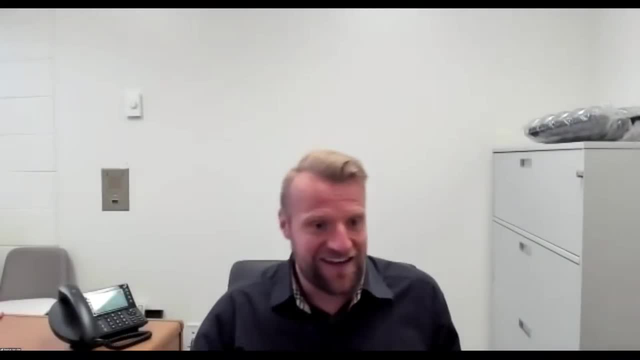 Yeah, no, we have presented that. And I mean I get a comment such as, like you know, thank you for challenging the status quo or presenting this information right. So I think I think people are open for the idea. 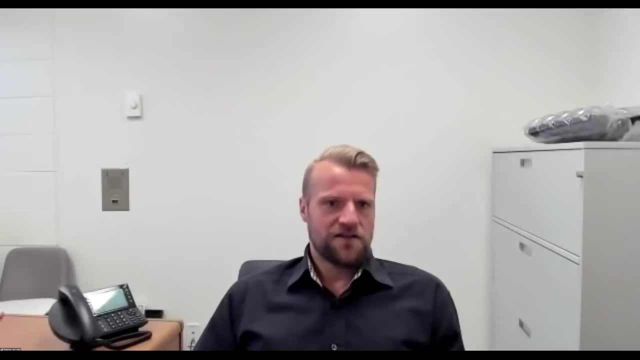 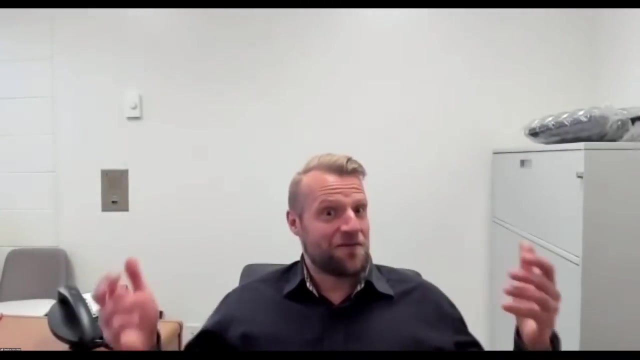 Yeah, And You know certainly sort of these nature-based solutions. that field is growing right, And we're also not per se saying, and it's not realistic right To say, well, we're going to stop finishing a feed loss and things like that, right. 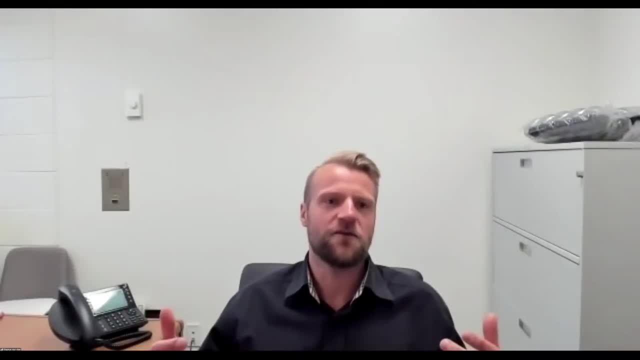 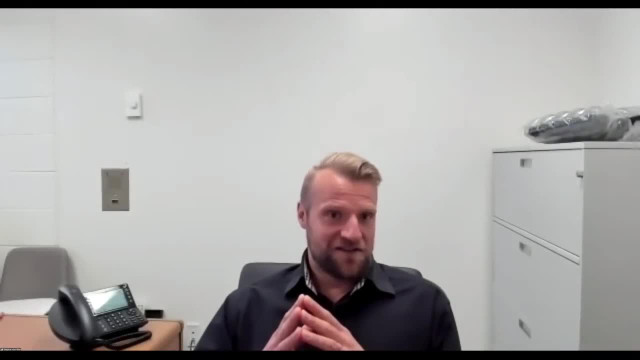 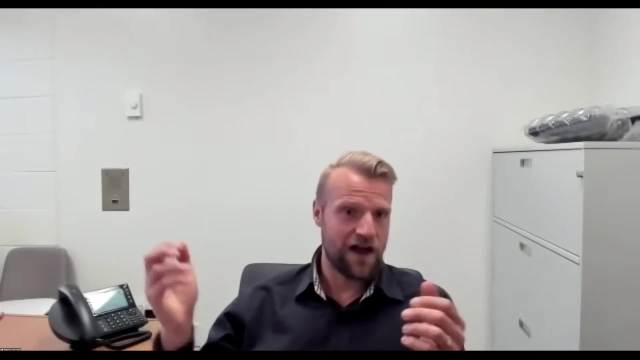 Yeah, Yeah. I see many farmers making a transition because it's beneficial for them, because they got back their input costs with like 30, 40, $50,000 a year. So maybe they're not producing more, but they're producing a similar amount, but they cut back their costs so much. 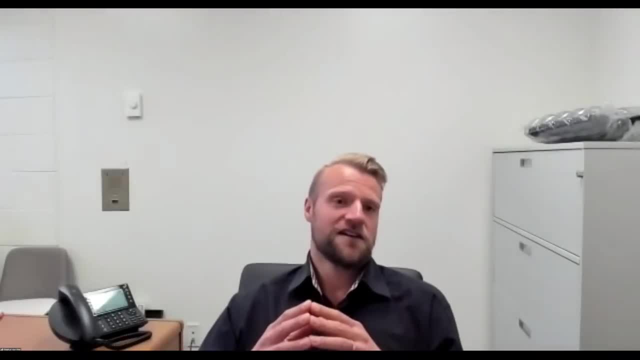 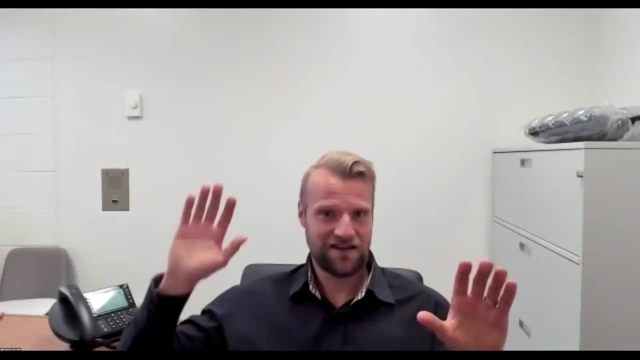 And, as a result, they improve profitability and quality of life. And I think we absolutely need to support small to mid skill farmers, And that is what we're focusing on. But we should- And that doesn't mean we cannot- have the big sort of, you know, industrial food system either. 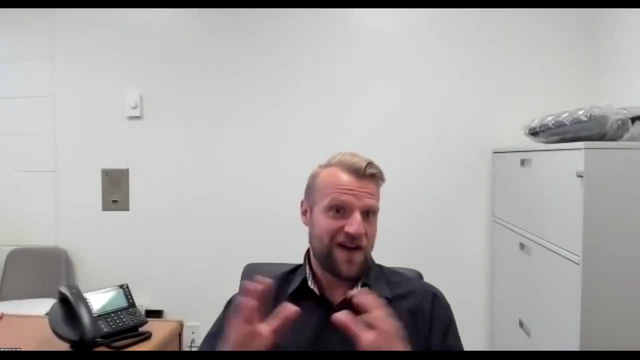 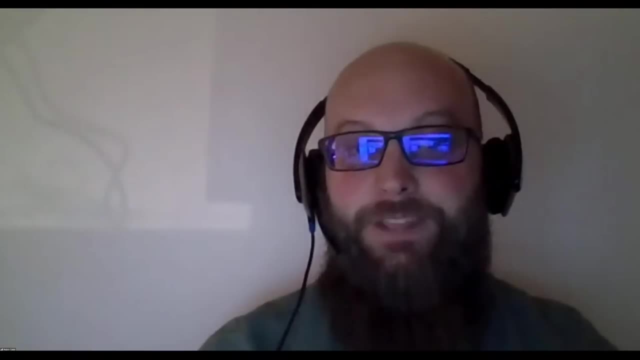 I mean, I think there's a combination of both, So it's finding sort of a middle ground in that, I think. Oh, thanks so much for sharing that. Yeah, that's, that's kind of the thing I've been talking about a lot lately is the messy middle between a lot of what's out there. 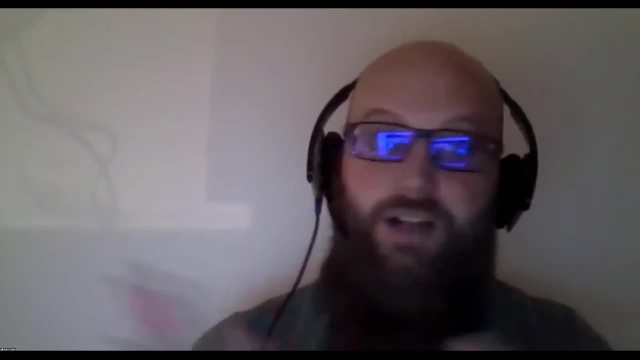 And the fact that we don't necessarily want to set it up as a fight between sides, but we want to say, you know that, not that the truth is always a An average of two extremes, but that there is a kind of like a mosaic that we can pull and put together from some different things. 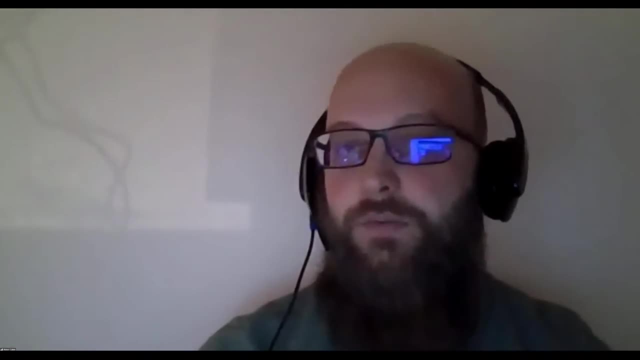 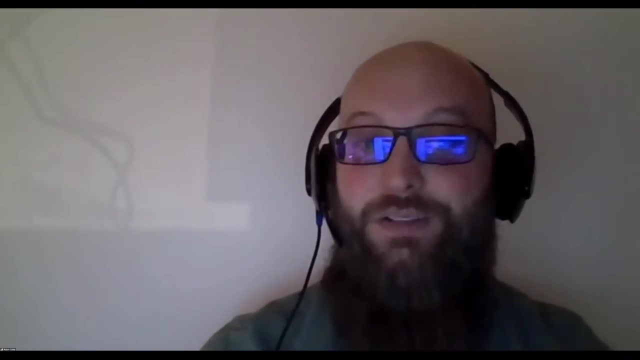 And it's not going to work the same way everywhere, especially in terms of, you know, different countries and the food systems that they have. But yeah, thanks so much for fighting that fight in the land grant system. You know I still am doing some publishing but that guy got a little, a little tired of. 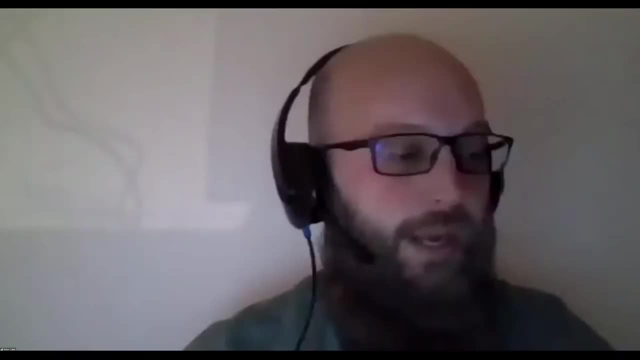 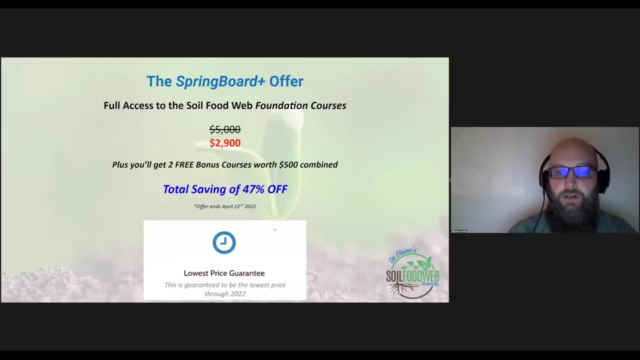 Edwins: Yeah, So I think we're Brian. we're probably going to have to shut things down here just because we're over time, but We wanted to put up our- our marketing promo one last time here and then and then thank the panelists for their time today. 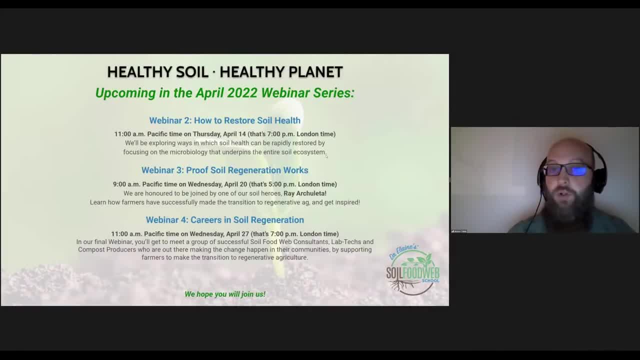 It's been really great. I've learned so much from all of you and I'm really looking forward to attending the next webinar, which will be on April the 14th. You can see that we have a series Set up here and so yeah, but I just echo the comments coming through on chat that I'm glad people are finding it so inspiring to hear from these voices across the you know sort of alternative agricultural spectrum and- and we want to- it's so great that here at the soul food web school we can- we can bring people together to share these advances. 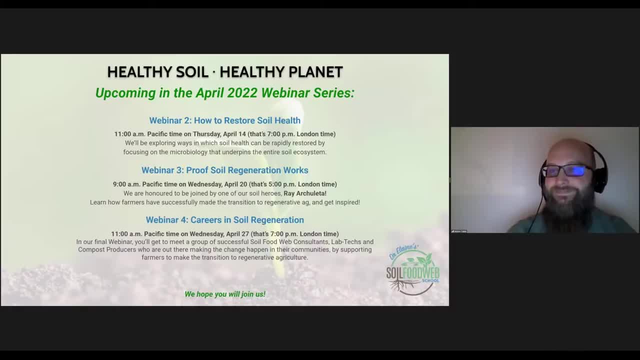 All right, was anything Anybody, anybody's like, heart heavy to share. one last thing. I have one last thing to share about your question, Adam. I think, talking about the land grant, you know the powers with the farmers and the community and the consumers. 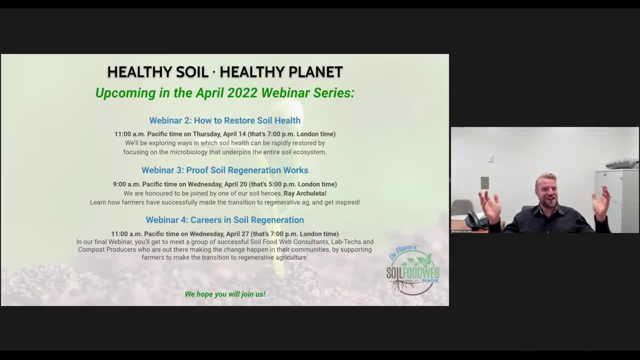 If they change, We will change to as land grants. right, I love it. We are focusing on that. Oh, thank you so much for that. that makes me feel optimistic- and I still am- and maintaining so many relationships along across university systems and I. 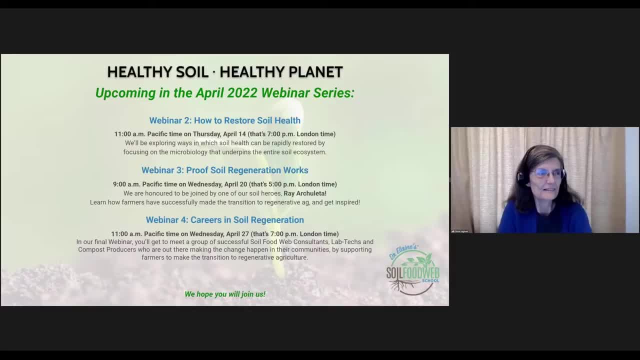 I can't wait to be Part of helping it change A little bit of different attitude, I think from younger folks, because over the last 15 years started to see a shift In the people that are being hired by land land grant universities, So there has been more willingness to look at studies that have been done that don't line up with the 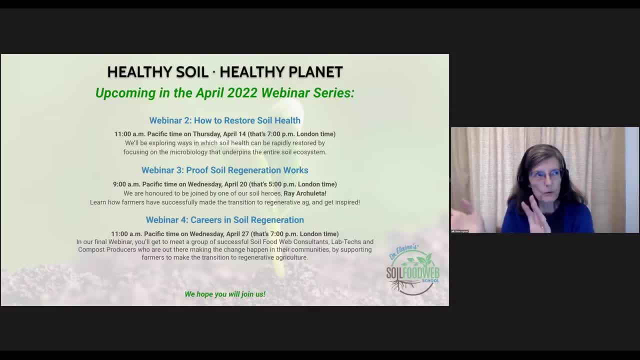 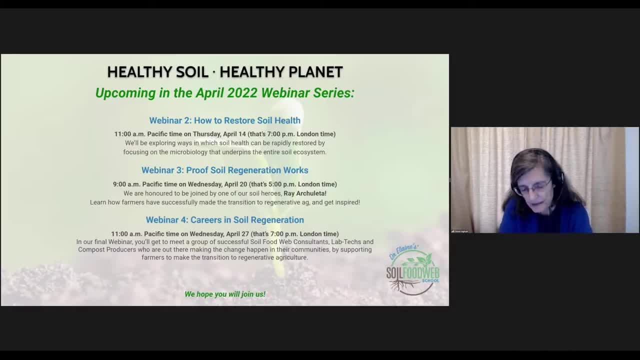 So the change is happening. It's been a long time brewing Awesome. Well, let's, let's sign off here so that people can get about their daily activities. but I just wanted to thank all the panelists one more time, and I know Dan had to leave already for personal reason. 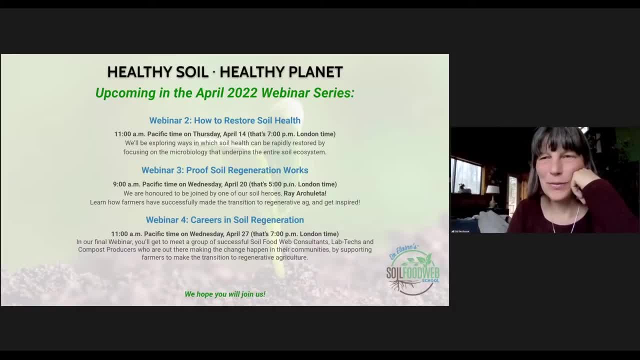 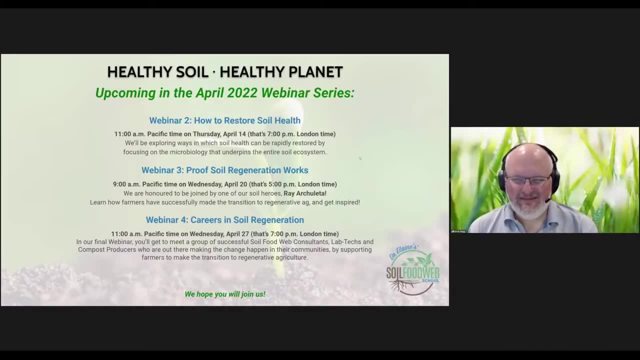 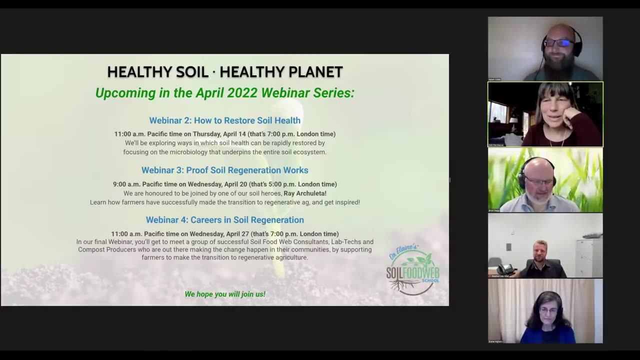 It's great to be here and really, really fun, fun, even if a bit distracting- to read the chat. There's just so many great comments and questions. And yeah, we are, we are. we are building the community right here and I'm looking forward to meeting some of you in the next course. 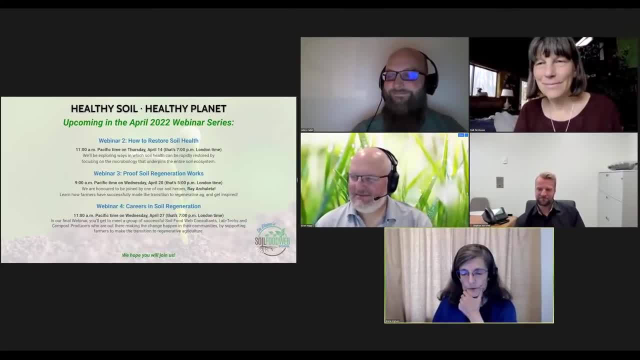 And I want to thank all of the support people who have behind the scenes have made it possible for us to put on these kinds of webinars, and you know so, Sammy and Alex and Heather and Luke And everybody back there, please are take our gratitude for the effort you put in. 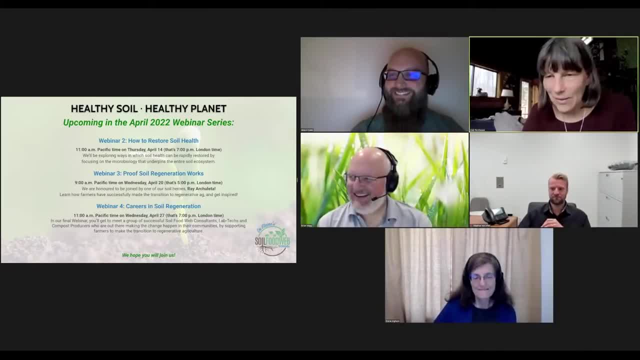 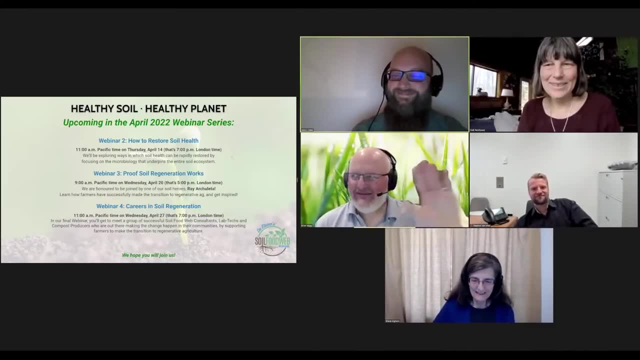 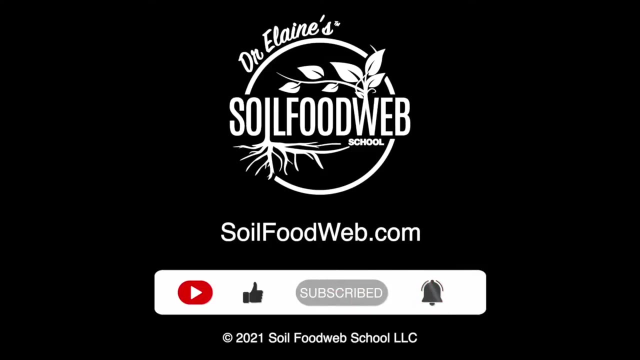 Absolutely agree. Our essential, our essential workers and David Yep, Awesome. We'll see y'all next time. Okay, everybody, Ciao, Don't forget to click that like button, subscribe to our channel and ring the notification bell to stay updated with all our new videos. We'll see you next time.